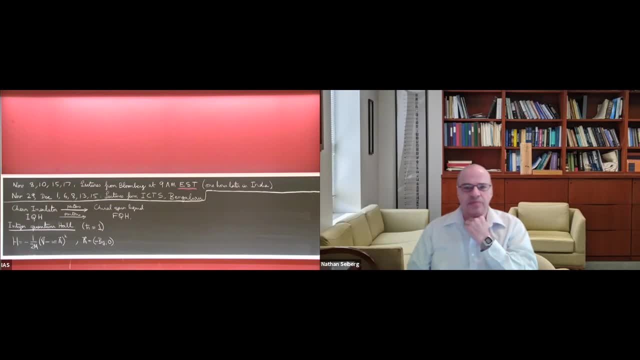 Oh, what time is it? It's almost 2 minutes past. All right, so good morning, Let's see. OK, hopefully you can see me and I'm on the right screen. So we're back at Bloomberg. So a couple of announcements. 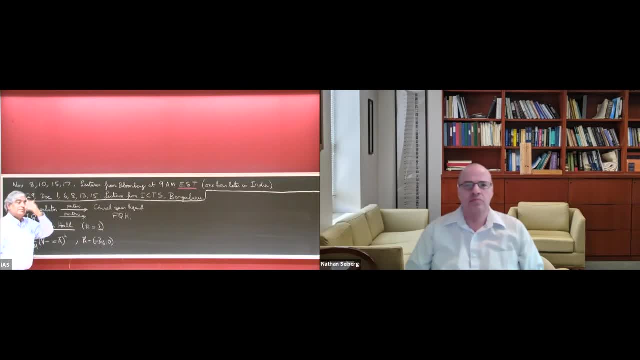 So there's going to be a change in time in the US at the end of this week. So next week we're going to continue at the same time in the US, Which is 9 AM Eastern Standard Time, which will be one hour later in India. 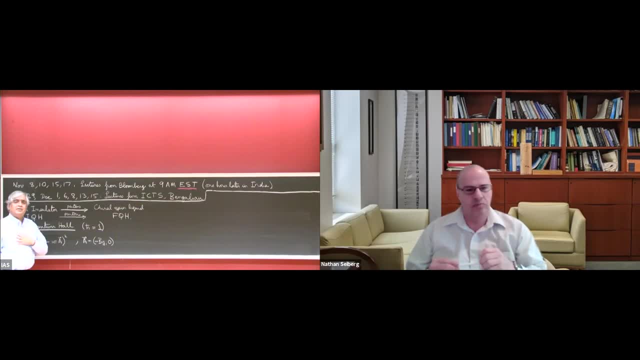 So please be aware of that. Can you hear me, by the way? Yes, we can hear you. All right, great, OK, and then. so that'll be the next four lectures, And then there's a Thanksgiving week here in the US. 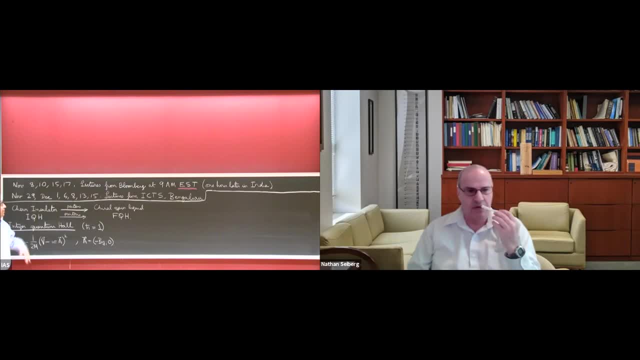 where I will not lecture during that week And the week after that I'll be in India, in Bangalore, And I'll give six more lectures over there. So at a time to be determined- I'm not sure exactly when- It may end up being quite early in the US. 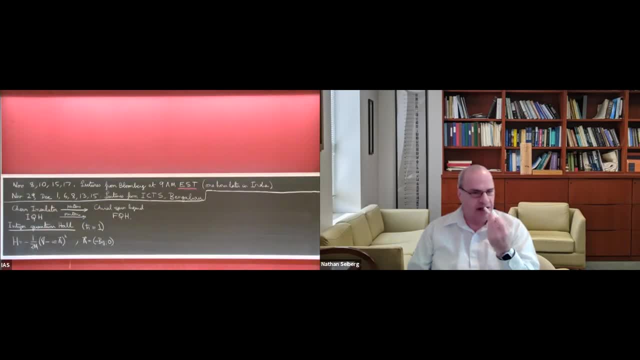 but you can be in here at home and watch it. OK, yeah, So in your previous lecture you discussed how you start from maybe some spin system and then go to the Spartan picture. Yes, For example, Trans-Simon's description. 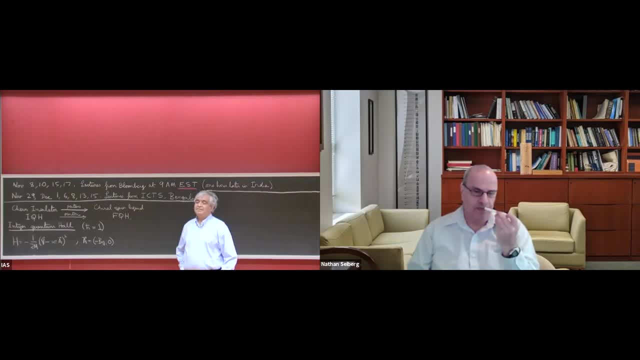 Yes, yeah, And the chiral spin liquid Right. yeah, Is it possible to just go there To go directly to the Trans-Simon's description, Because that's what you really care about: the very known, actually, description. 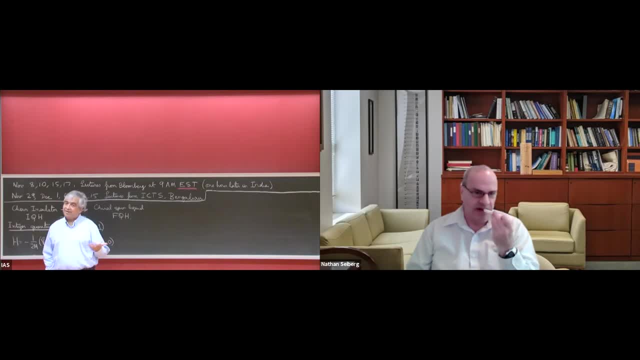 To go directly. I mean, you still have to solve the spin problem somehow. So another way to do it, which is, I guess, the way Laughlin and Kalmar did it: you take the spin problem and you think of spin up as nothing. 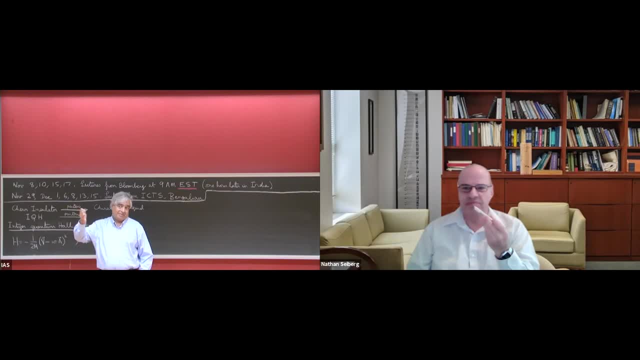 and spin down as a boson, Then you can think of it as a hardcore boson problem And then postulate it that the hardcore boson problem for a boson system should be in the nu equals 1 half fraction of quantum power state. 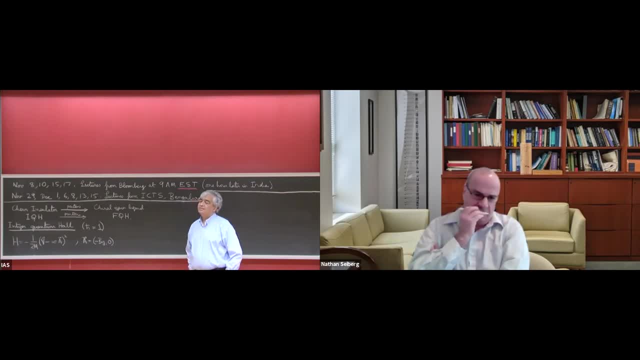 OK, Yeah, I'm just thinking of theories like, for example, the CPN model, where you have an immersion gauge field, Right That there is a simple. Well, that is exactly what we did. right, We wrote the spin in terms of fermions. 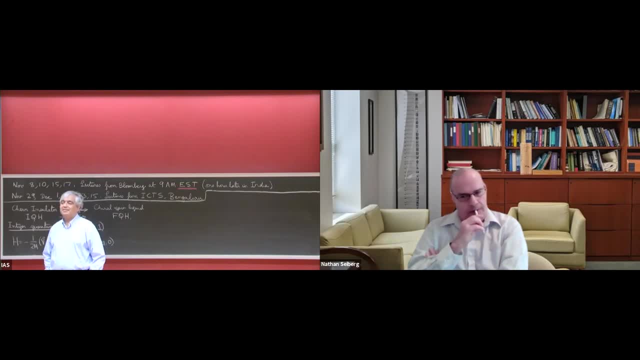 Yeah, yeah. no, I realize that, But there was the intermediate step of the part of this. Well, anyway, it's just a Yeah. So the partons, I mean the CP1 theory, is also a theory of partons, because the z particles 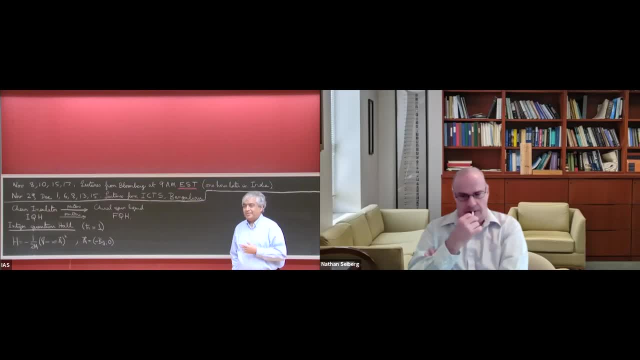 have a gate charge. It's also a theory of partons. The physical operator in the CP1 theory, the gauge-neutral operators are spins z, star sigma z. Those are the spins. so you're not doing anything different from the CP1. 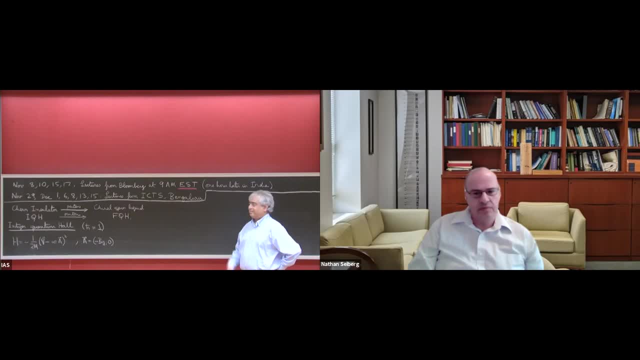 Yeah, there's no gauging. The z's are not gauge-invariant objects. So similarly here the partons are not gauge-invariant. I had to put the partons in a churn bag to get the churn silencer. 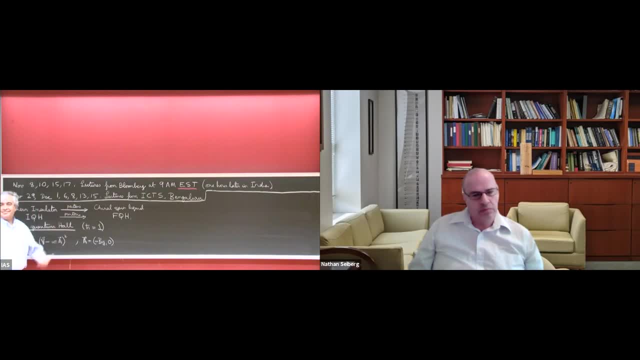 But, as we'll see today, you could equally well put them in a magnetic field, and it'd be very similar. Yeah, I also have a question from last time. Yeah, go ahead. This is the role of time reversal symmetry. OK, 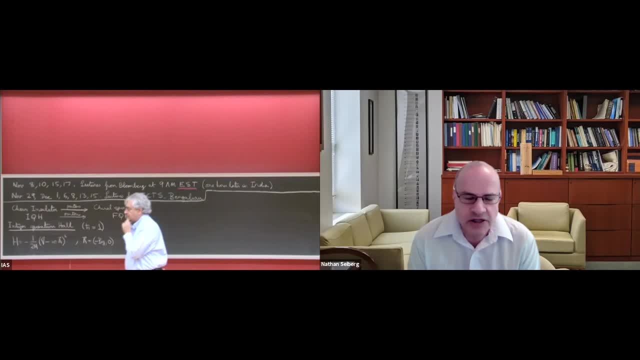 Was it there microscopically and then was spontaneously broken, or was it explicitly broken? And if it is spontaneously broken, are there any consequences of that? Like too bad for our Actually? your first question is: it can be either. 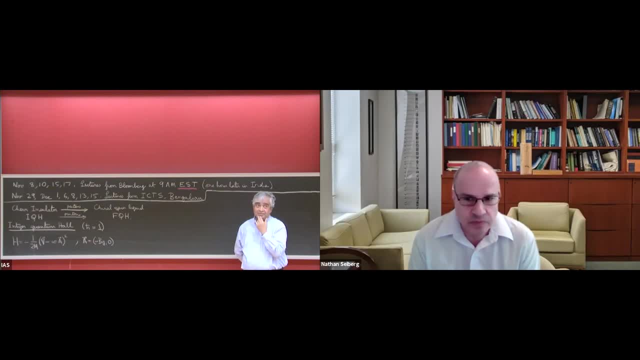 It can be either spontaneously broken or broken explicitly by the Hamiltonian. It won't make any difference to the theory of the phase. That's the phase where you have of the chiral spin. you get exactly the same theory in terms of the quasi-particles and all their properties. 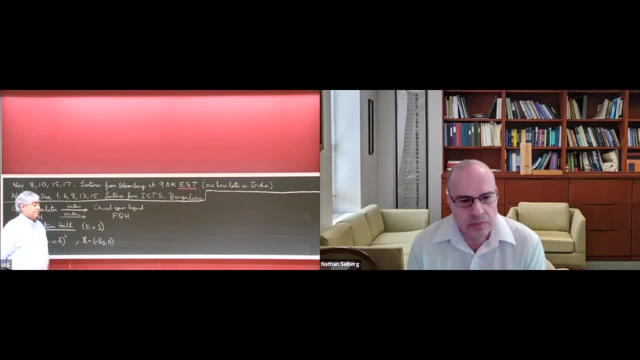 and the edge state properties. But if it's been spontaneously broken, well, there is a scalar which is gapped, And that only becomes important near a phase transition. So suppose there's a phase transition where the symmetry is being restored, And then you would have to worry about the fact. 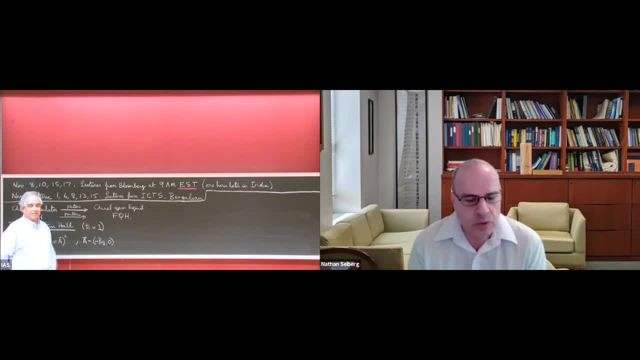 that the time reversal was spontaneously broken And there will be extra fields associated with light field, associated with the fact that you're restoring the symmetry. So that would be an interesting point And based on vision which I haven't addressed, you first have to decide what the other phase is. 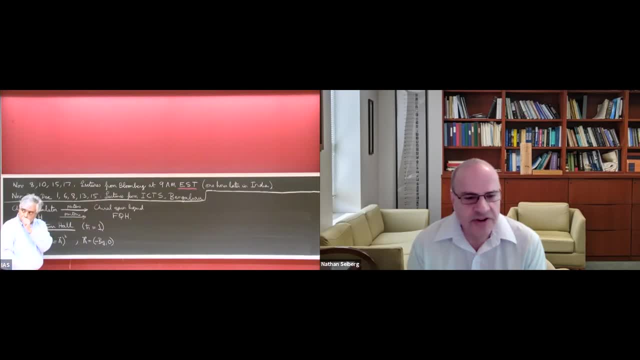 on the other side that you're going to. Are there any? But if it is spontaneously broken, won't there be domain walls where you have the different vacua on the two sides without going to a phase transition? You're right. Yeah, there could be such configuration. 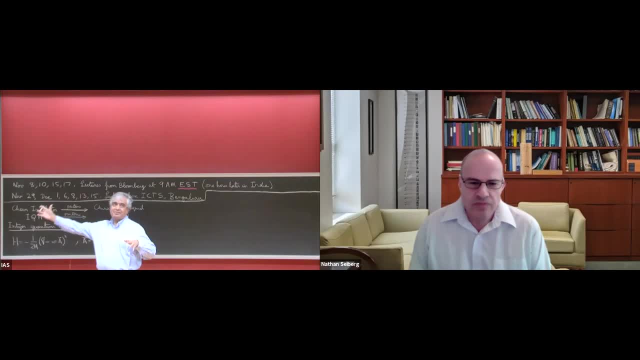 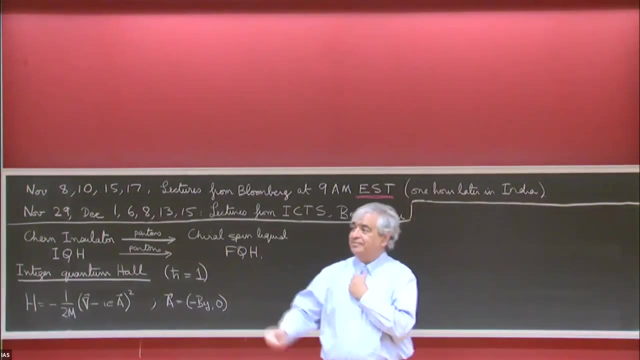 Yeah, so that would be like going from churn plus one to churn minus one, And yeah, then there'll be some edge states in the domain walls for sure. Yeah, Thank you. What were you saying, Tom? 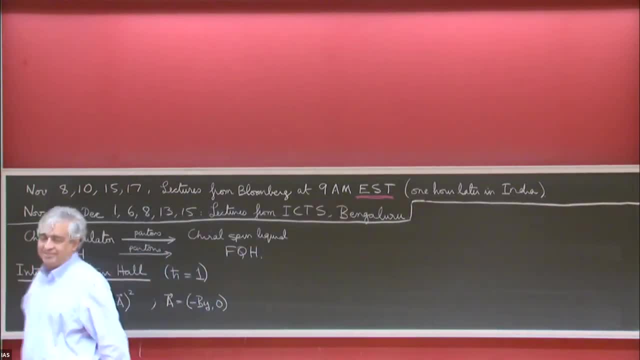 Exactly. OK, yeah, all right. Yeah, that's correct. Sure, All right. so we talked about this connection and which we've just discussed. Are there any other questions on the last picture on the churn insulator and the current spin? 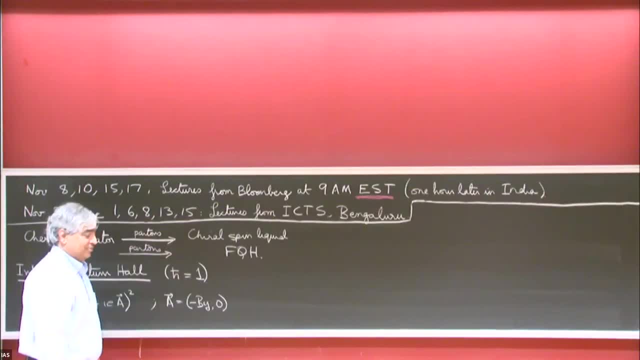 liquid. I've updated the notes on a lot of that on the website, so please download the latest version, And all the details on how the churn number is quantized and how it relates to the Chen-Simons term or the Hall of conductivity are in the notes. 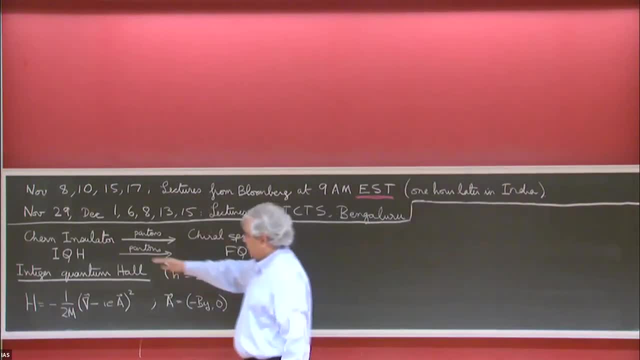 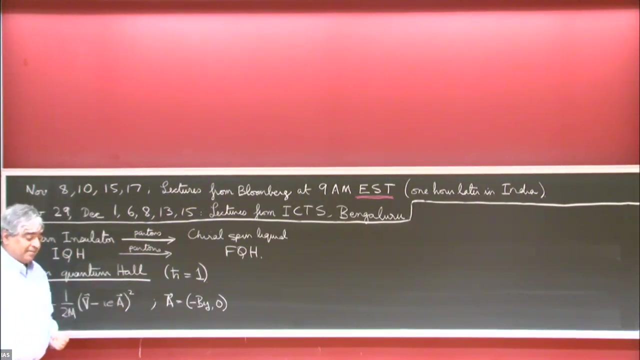 All right. so today I want to establish the same connection, But in a slightly different setting. This is the setting of the quantum Hall effect. So now you have electrons moving in two dimensions. They're not spins, They're electrons, They're allowed to move. 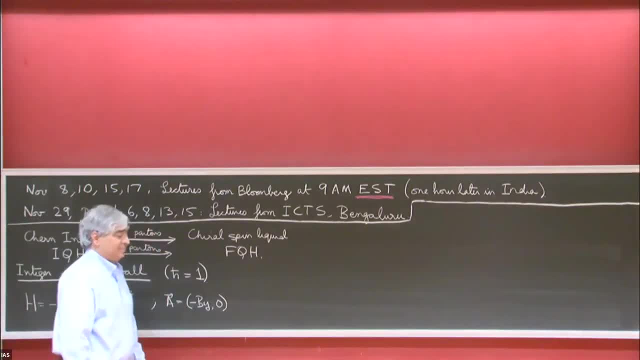 So there's no local constraint that they have to be exactly. in the case of the current spin liquid, there was a local constraint that the number of fermions on each side had to be one. There's no such constraint And initially we'll just take three fermions. 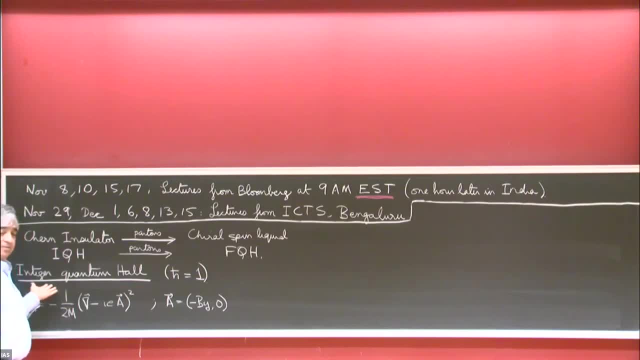 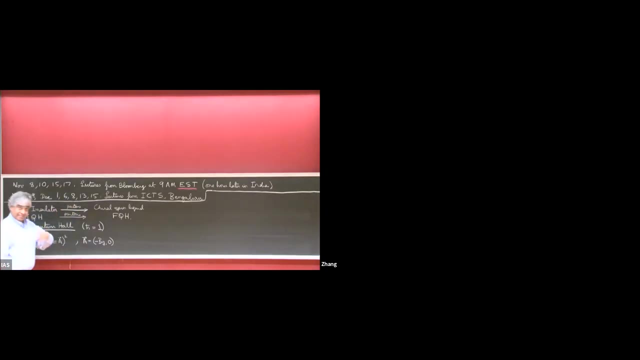 moving in a magnetic field, That of course leads to integer quantum Hall states. OK, And then we'll do a part on description and describe a few fraction quantum Hall states And hopefully, given all the stuff we've already covered, this will be relatively straightforward. 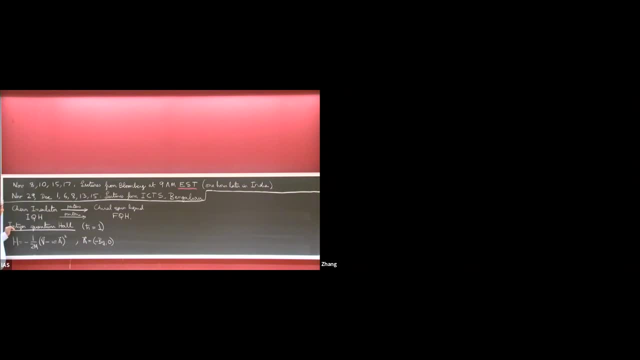 as you see. I hope OK. so we consider the integer quantum Hall case. I'm going to take h bar equals 1. This is important because many results are expressed because of h, not h bar, So always remember it's h bar. 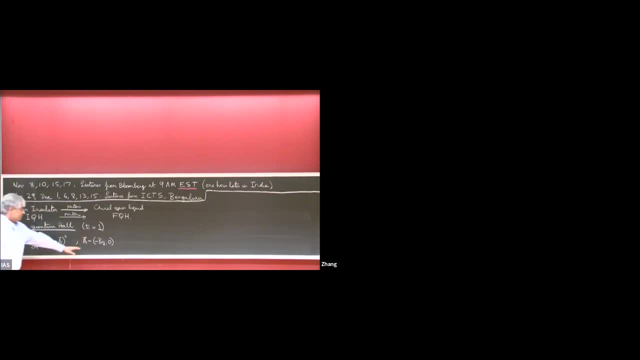 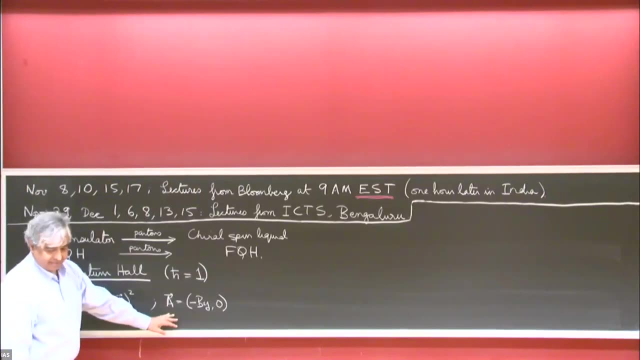 That's 1.. OK, so this is just a free particle and a vector potential. I'm going to use this particular gauge because that will be useful when we look at the edge states. So that's what I want to do. today is also explicitly show. 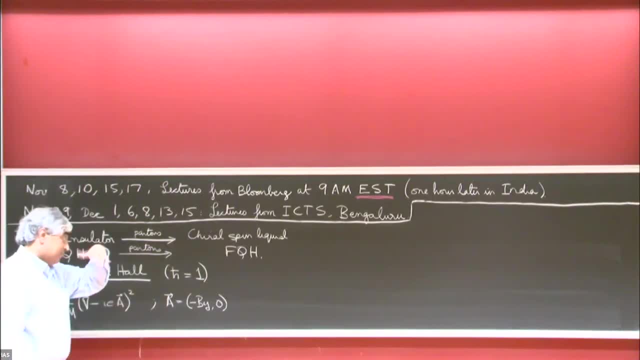 you. in this case it's a bit easier- as was shown first by Alvaren, actually before TKNN, that there are chiral edge states on the integer quantum Hall system. OK, So now we just go ahead And solve this equation. 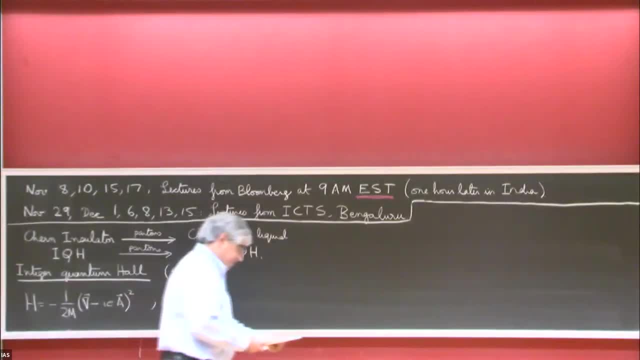 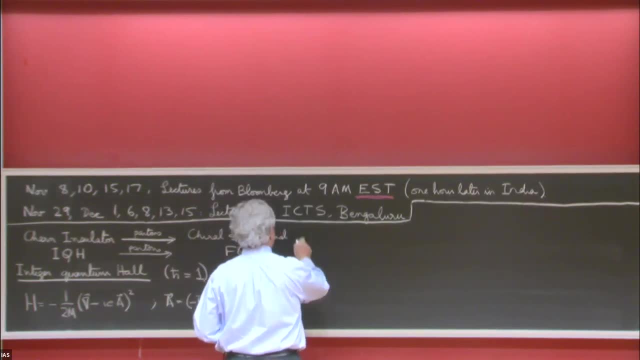 I'll be very quick about it. I presume most of you have seen it somewhere. It needs to land our levels, So let's put that with notation. We introduce something called one of the various quantities that you will see if you read papers on this topic. 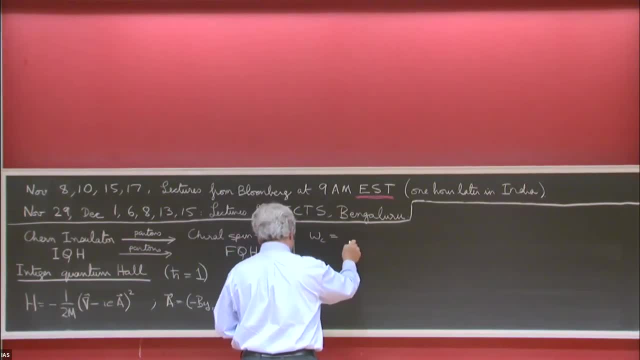 There's something called the cyclotron frequency, which in these units is eb over m, And there's a magnetic length which is 1 over square root of eb And there's a magnetic length which is 1 over square root of eb. 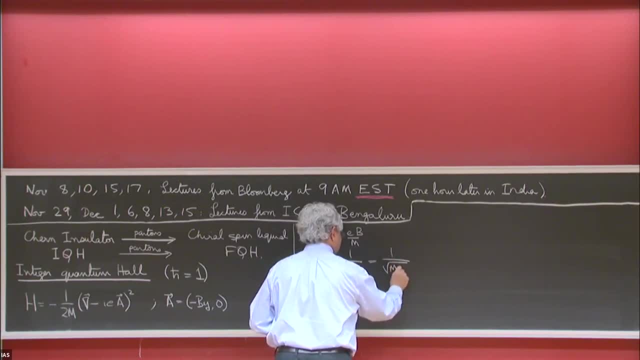 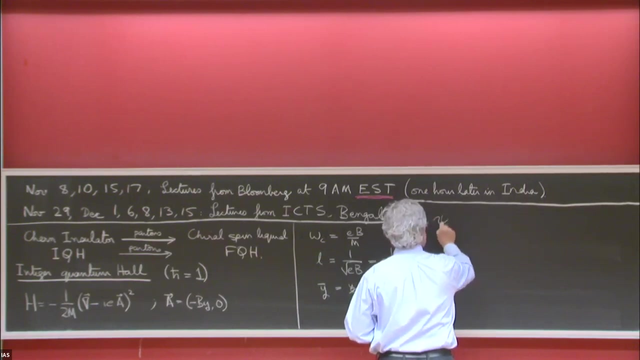 And also 1 over square root of m only to c, And then you can introduce a dimension that's coordinated in terms of the magnetic length, y minus y over L, And then if you take your wave function, so I could have a label n and the function of x and y. 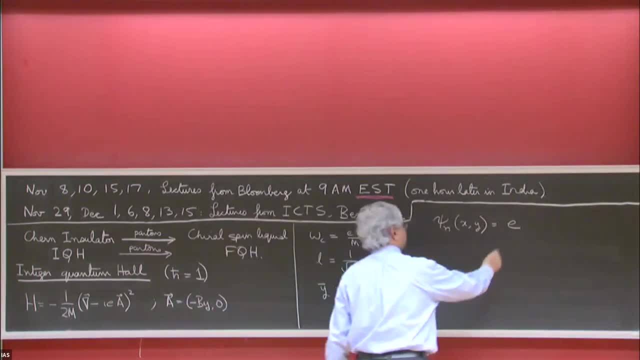 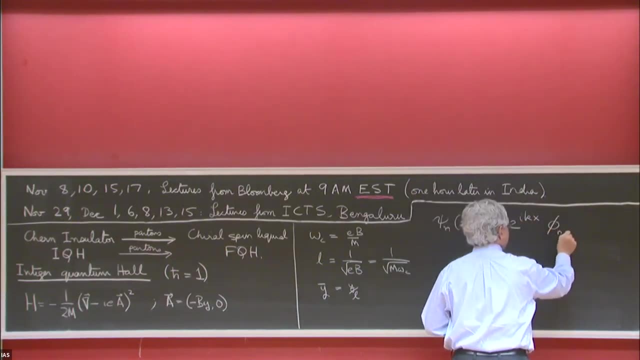 Well, since you have a translational symmetry in the x direction, it can be a plane wave in the x direction And it will be some function, pi, of n and k which will depend on y, And this function just obeys the equation. 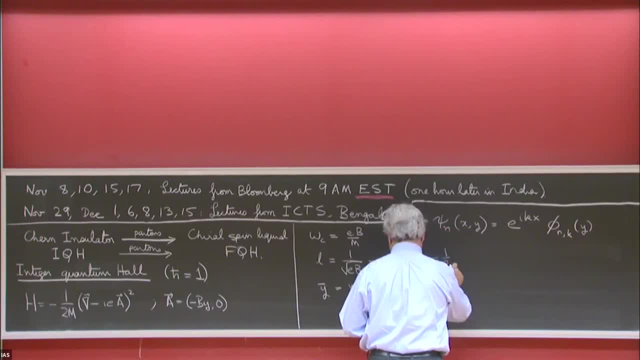 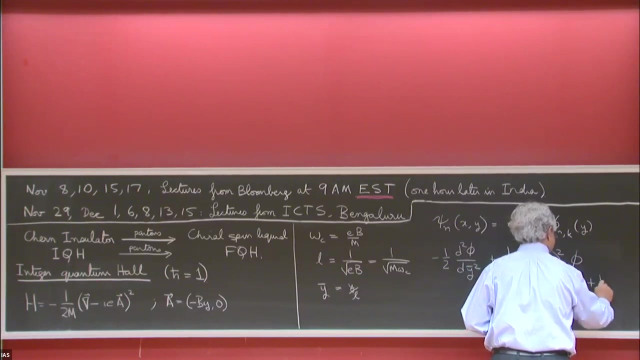 of the harmonic oscillator. So in appropriate units, d squared, pi over d, by bar squared, that's 1.. That's 1 over pi over d over pi, which is 1 over square root of eb. And so we have n over square root of x squared. 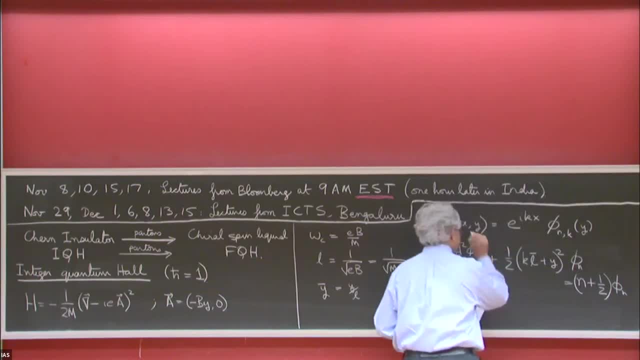 And again, theopex trainers are actually actually the same thing. So it looks like we're not necessarily going to be getting any more m over square root of x, but we see that if we just use the type of the value of the你们 that we were going to get. 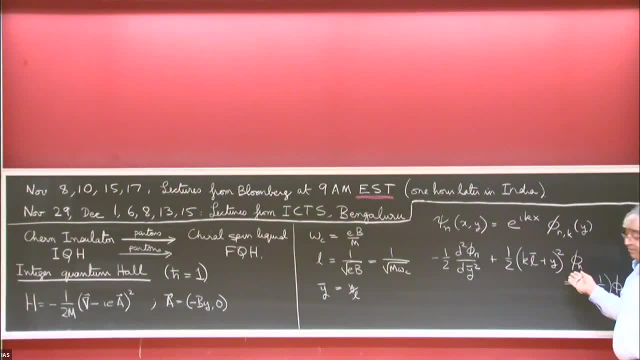 we'd be getting n over pi over x squared, because there is a point here, whereas the momentum that we were getting would have been the momentum. So we would have nearly n over pi over x squared, and then we would have no volume. 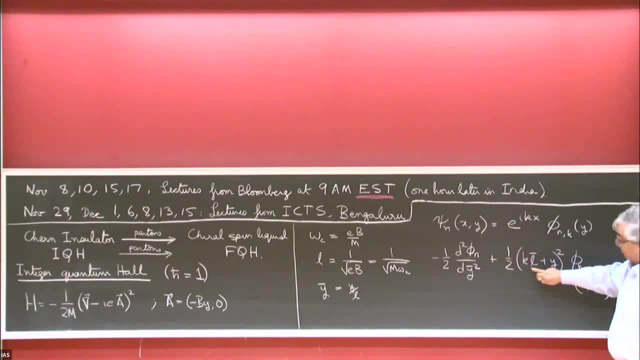 and then we'd have no mass, And so that's something that's really important. So we're going to just start from here. That's a little bit of a shout out of mass of the harmonic oscillator shifts with K, So momentum in the X direction is the same as coordinate. 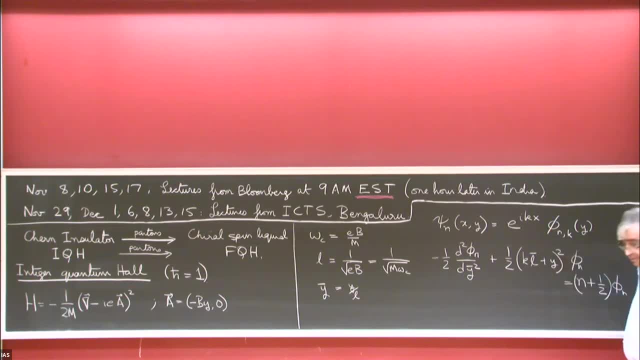 roughly same as a coordinate in the Y direction, So that's a very useful semi-classical picture to keep in mind. Sorry, what's L bar? Maybe it's L square, perhaps Yeah, or it's Y bar, Or it's K L bar. thank you, 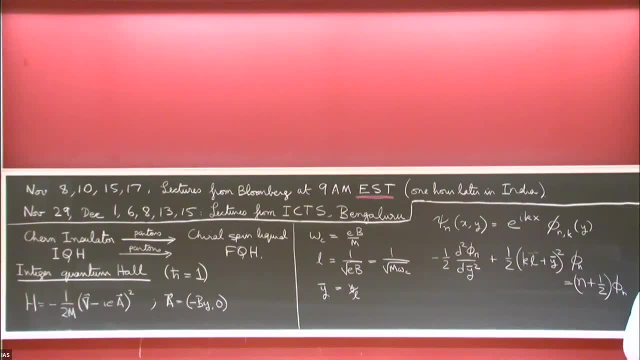 Yeah, so K, L is dimensionless, Y bar is dimensionless, so it's all all right. Okay, so the very important property of this equation, which is different from the Chiron insulator, is that the energy, the eigenenergy. 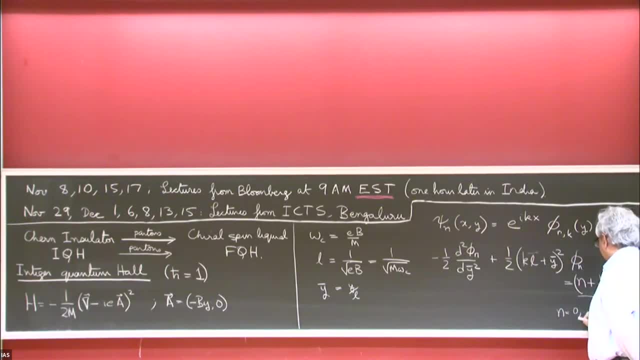 that is the harmonic oscillator states. and here of course you can see that N is zero, Y is two, it's an integer. The energy is completely independent of K. So we have a very large degeneracy of states. It's independent of K. there's no dispersion. 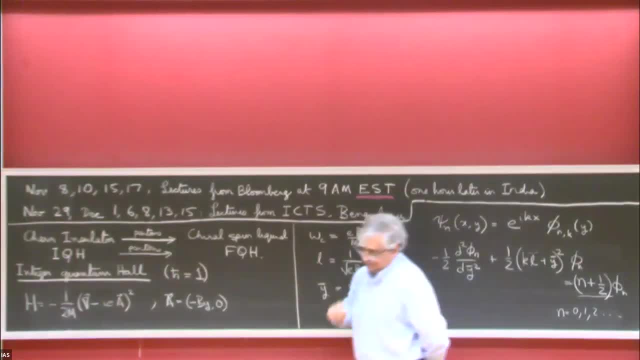 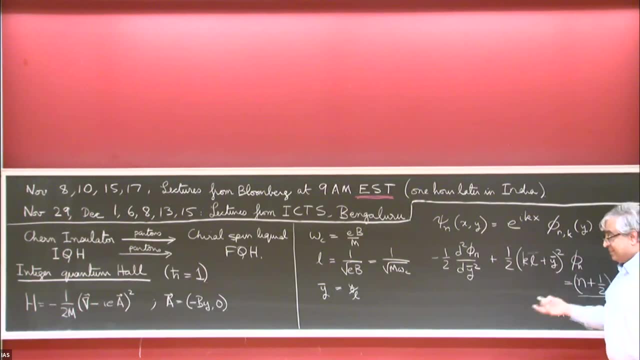 as a function of K And that's very different for the Chiron insulator. but it's a simplified feature. But in many ways it's also a confusing picture because it makes the band flat and things like Chiron number are not so easy to define. 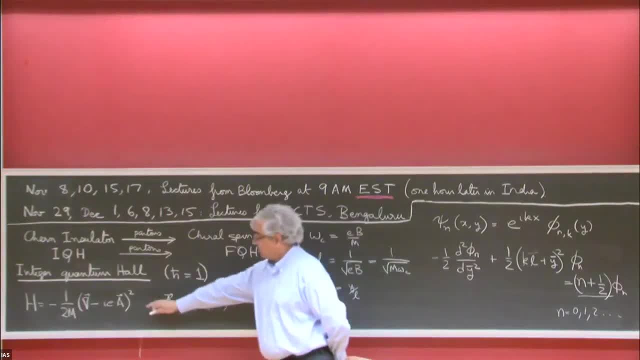 So you can imagine a more general problem, that you added a very small theory of potential here, and then it'll become exactly the same set of problems that you solved there, but that the algebra becomes more complicated and you have to go and draw a theorem and all of that. 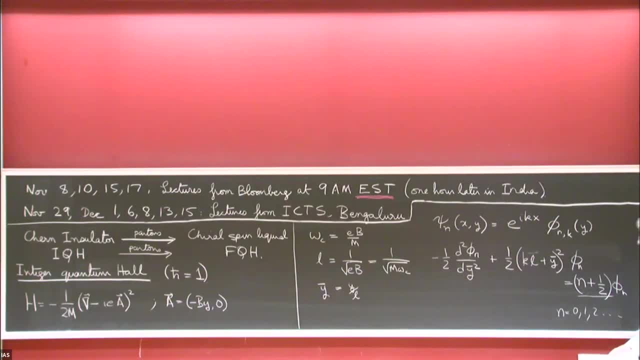 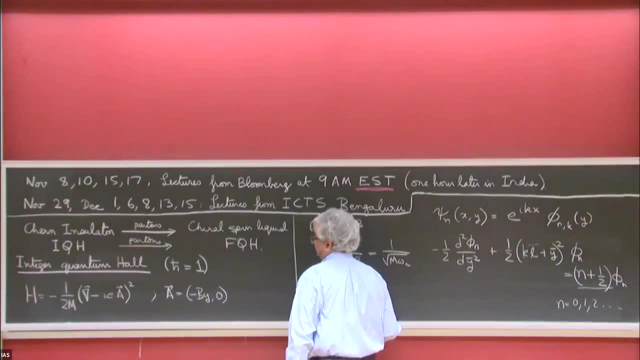 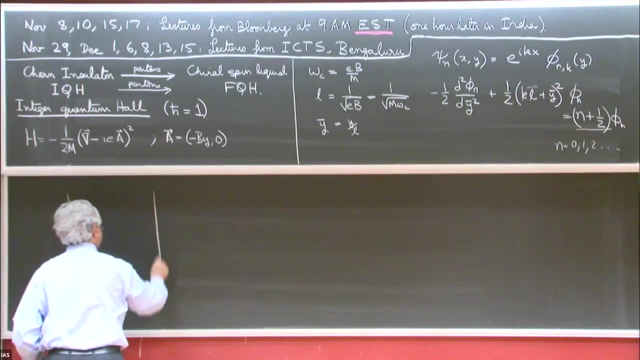 Anyway, Okay. So then the question is: what is the degeneracy of the states? So this is the other important point. So, if you take a geometry there, so that's all this, Okay. so this is LX and this is LY. 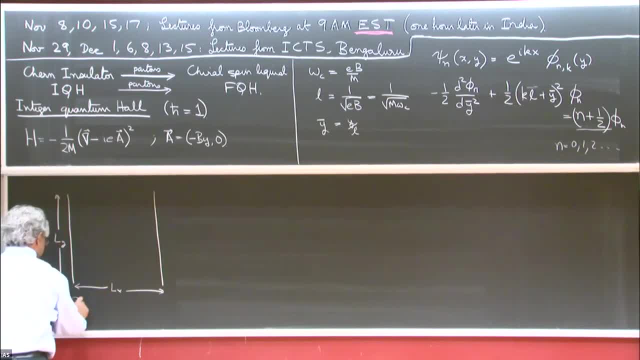 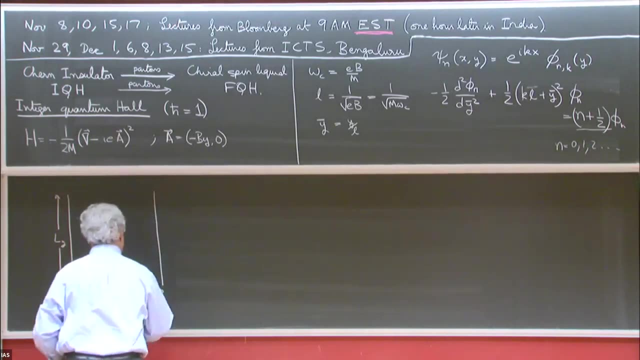 So my K is some integer multiple X over LX, And then the center of mass coordinate here, Y bar, is. so the average of Y is of course then minus KL. So the way you can think about this is that you have a whole bunch of states. 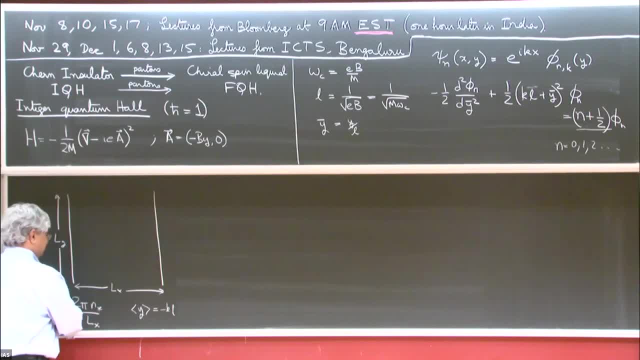 and then you have states where K is positive and Y will be negative. So those are states that are running here with very large momentum. And then you have states with smaller momentum, which- so this is just a basis of states. The larger the momentum, the more the negative Y coordinate. 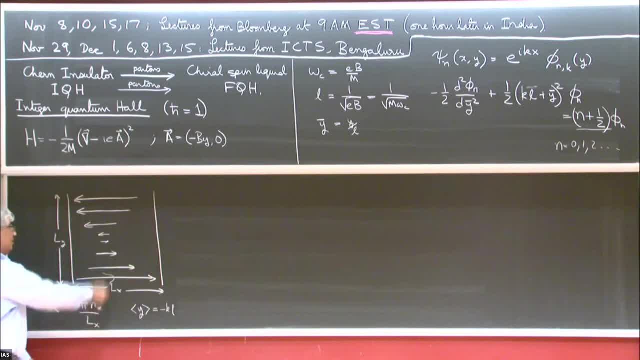 And they're basically Gaussian functions about in the Y direction, harmonic oscillator functions: Okay, In the lowest Landau level they got six Okay. So another important point is that if you well occupy say the Landau level, so let's say here are the Landau levels, this energy. 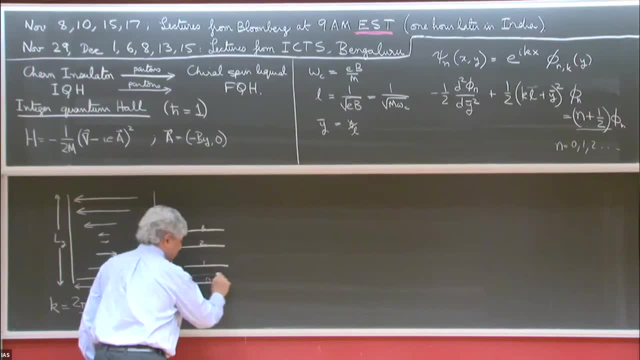 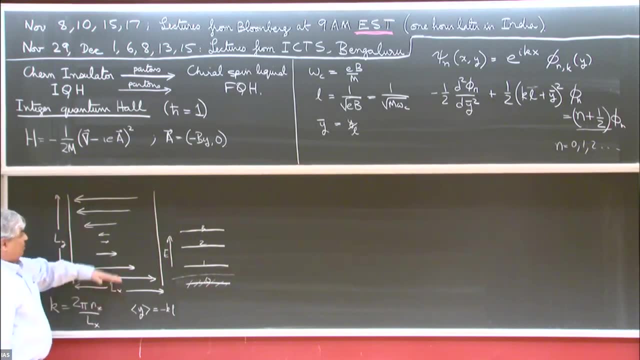 Zero: one, two, three. If you occupy all states in the lowest Landau level, which is the most important case we'll be interested in today, then you occupy all of these states And, in fact, at any point in the center. 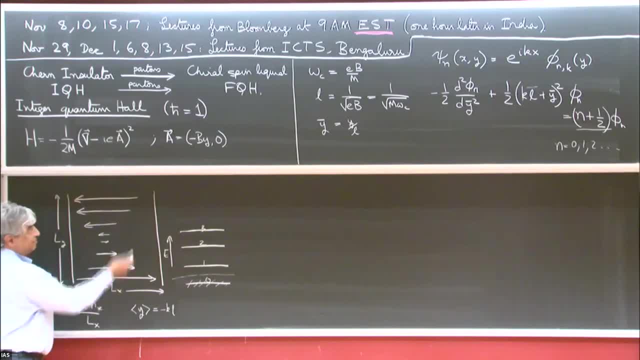 the net current is zero If we just compute it carefully. and it's done in the notes that there is no current. So if you pick a point here, you get a current from here and there and they all cancel out. These are just. this is a set of basis. 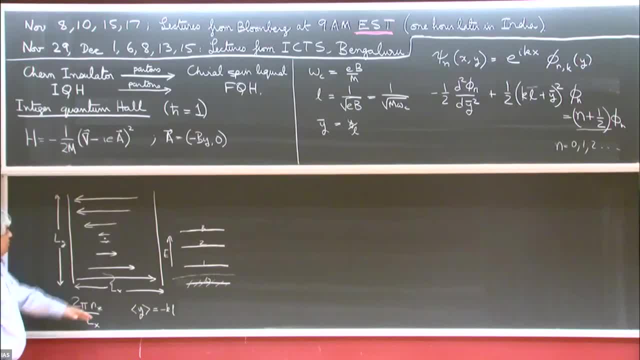 that you've chosen to describe these states All right. So this particular basis is very useful to figure out the degeneracy of states. So first thing is, how many states do we have here, And then, how many states do we have here? 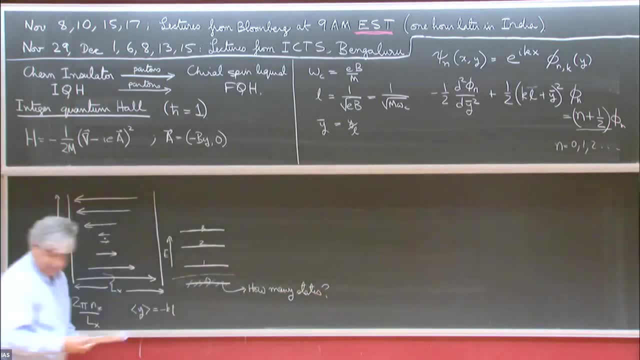 What's the relation between the value of the state and the function of the state in the Well? so the number of states, easy to count, It's the number of. you know the model. So the question now is: what is the maximum value of N sub X? 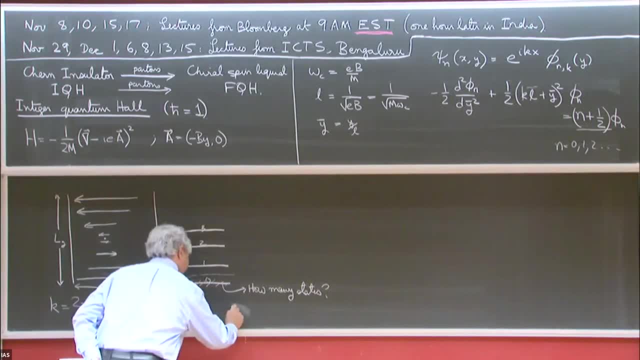 So how does? what distance is N sub X? What are the values? a lot of values- of N sub X. Well, N sub X is given from here, so it's got a number here. so we know that K minus KL, or let's say KL, is between 0 and LY. so let's just call this: 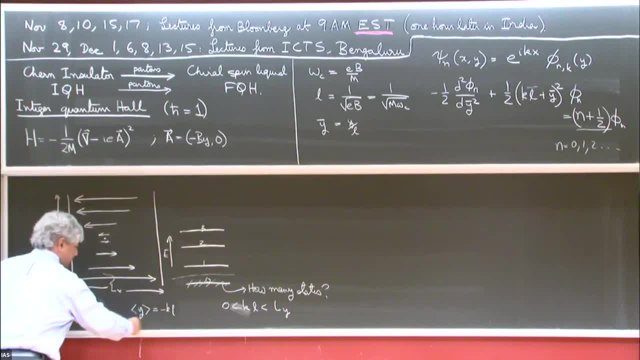 yeah, so this distance is LY, so the range of Y, which is KL. yeah, so this is Y bar, right, thank you, is that right? yes, thank you, all right. so then you get ignoring things near the boundary. you will all get all of these states. 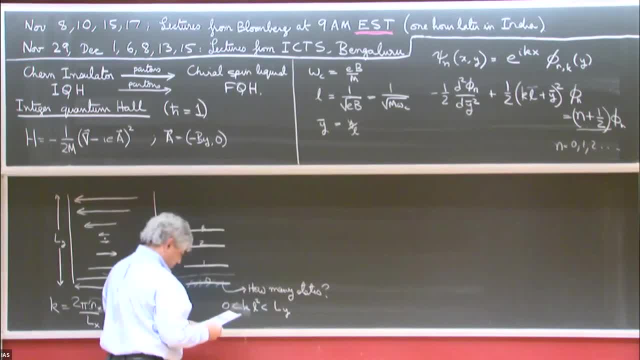 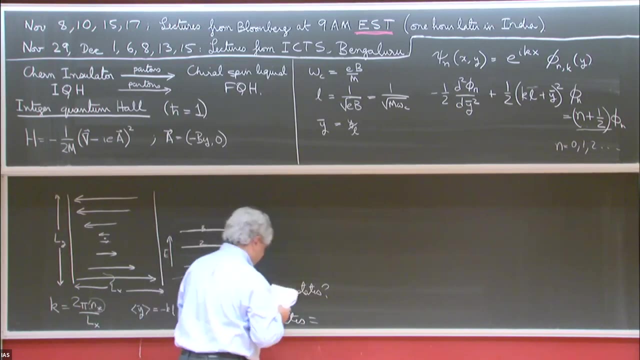 in this region, and so this tells us that the number of states here is combined to this, which is actually degeneracy, so the number of states is equal to LXLY over 2 pi L squared. and another way you can write this in the original units. 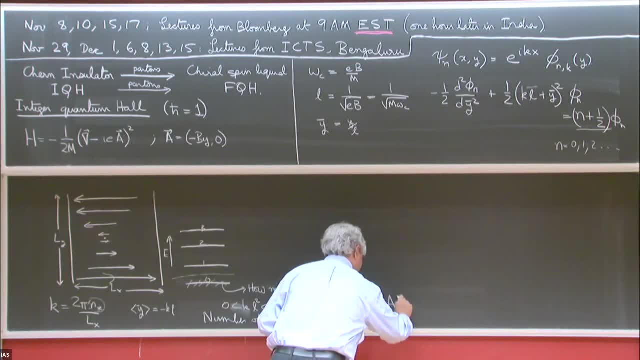 is the area of the sample that is B divided by phi naught, and phi naught is the flux quantum H over. so here A is LX times L. so notice that's H, not H bar, and that gets rid of the 2 pi over here. 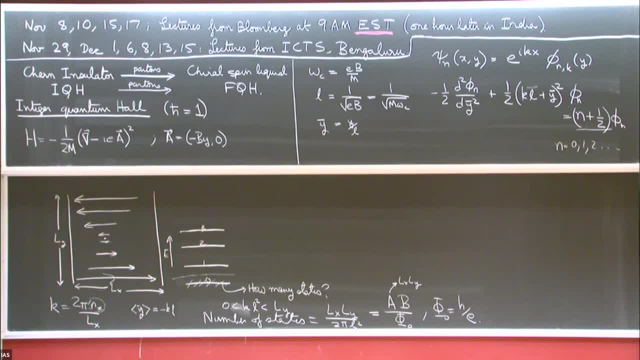 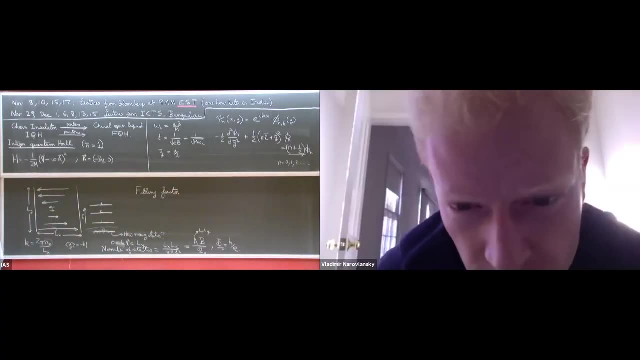 okay, that 2 pi comes from this 2 pi. all right, so that's the degeneracy of the states. and another very useful thing we're going to define is the filling factor, which is, in this case it will just be an integer, we will consider a fractional. 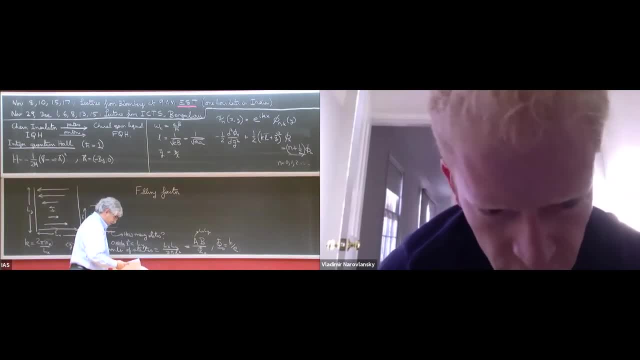 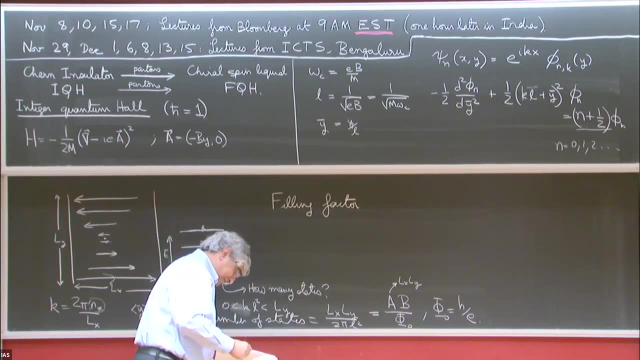 let me make sure I get this right: all the factors of 2 pi. this is absolutely crucial to get this right for this lecture, so I want to make sure I have it. the new filling factor is defined as mu, which is rho over B over phi naught. 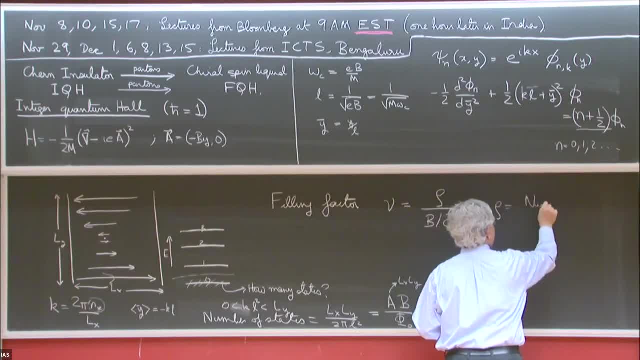 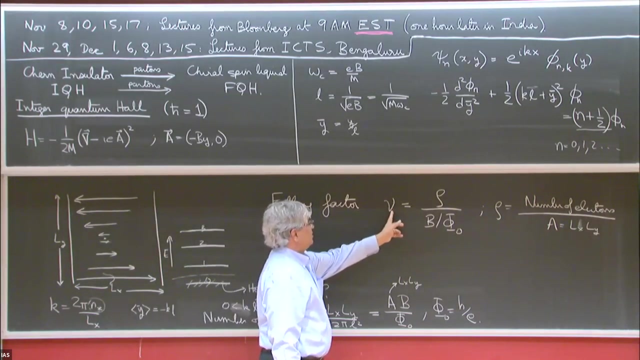 we have rho, with the number of electrons divided by the area, which is a, l, x, l, y. Okay, so in the image of a very large sample, then you don't have to worry about the edges, and all these are also exact. and so nu measures the density in units of the number of flux quanta. 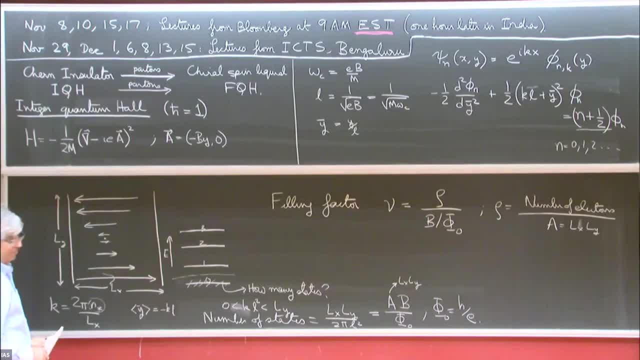 So that's one very easy way to remember it. and it's inversely proportional to p Um. okay, all right, all right, so then, okay, I'm not considering the spin of electrons. No, yes, thank you. so no spin in this entire lecture. So we assume here it's a very high magnetic field and the spin of the electron is polarized. 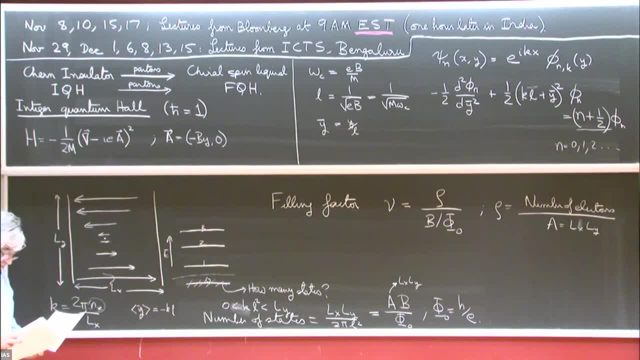 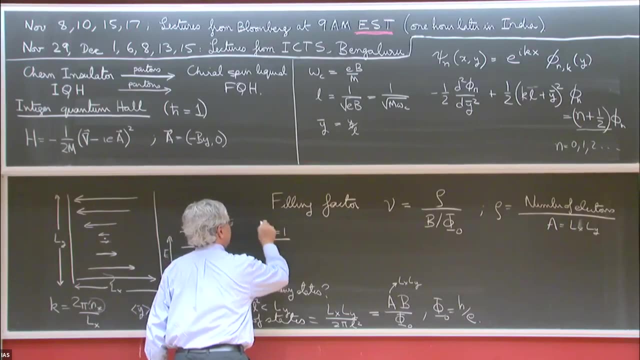 Of course, it could be other interesting states where you worry about the spin. Okay, so we'll be interested now in the case where nu equals one. All right, so let me, yeah, so let's consider nu equals one, Um, and now, in fact, I'll write down the wave function, and now you can write down the wave. 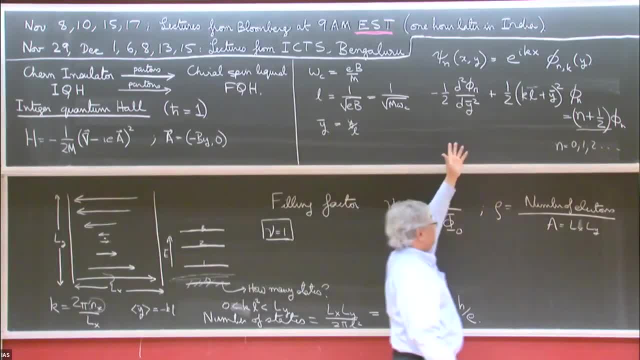 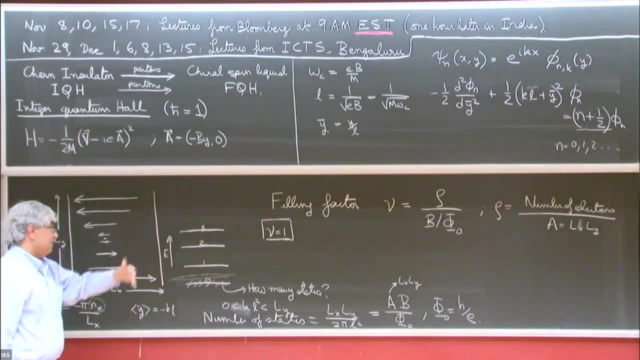 function, if you wish, by looking at occupying all these states at n equals zero, for nu equals one, and that will give you plane wave status, Gaussian, and you'll get a big determinant to write down the full wave function. but it's very useful for later purposes at least. 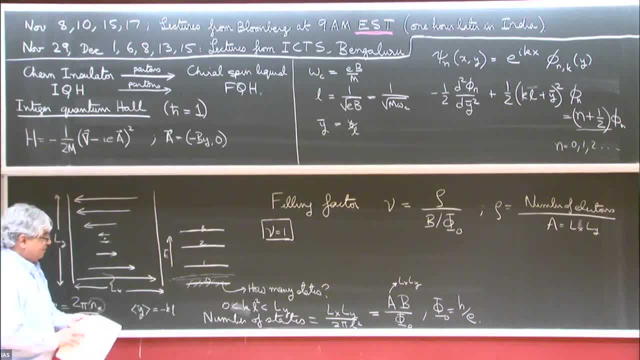 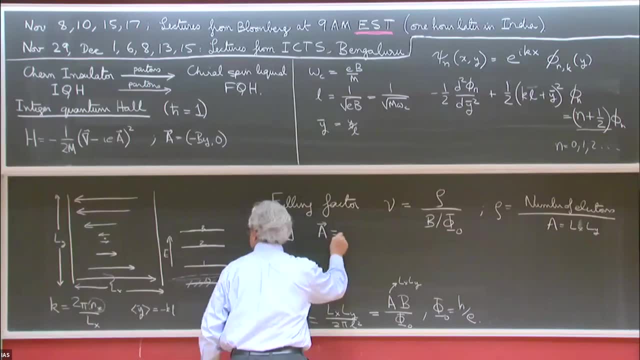 briefly so you can connect with a lot of other work. uh, to write the wave function in a different gauge, so we choose a different gauge where a, instead of having this value here- uh, we're going to now choose a- is minus one half r plus b, so this is going to be a different rate here. 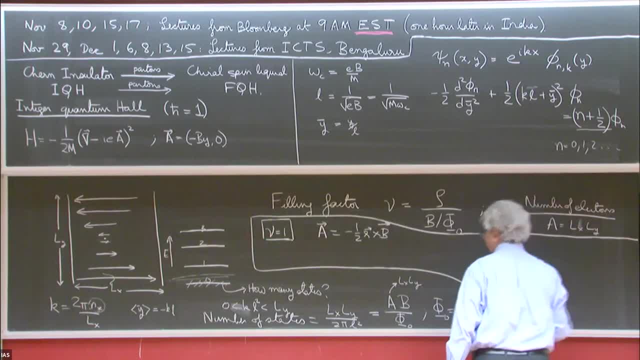 So we write down the wave function at n equals zero, and then I'll write down the value of r over here and we'll just try and think about some of the other phenomena as well. Then all the lowest lambda wave functions: 10 equal 0 wave functions: 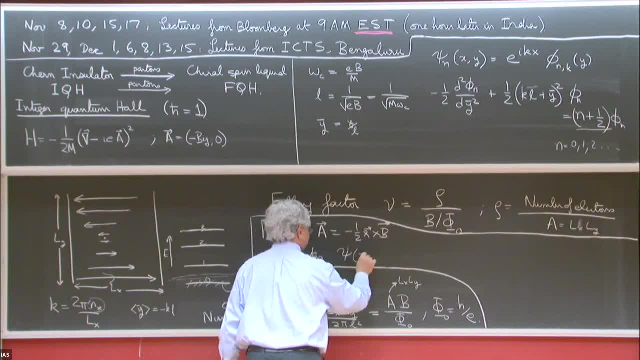 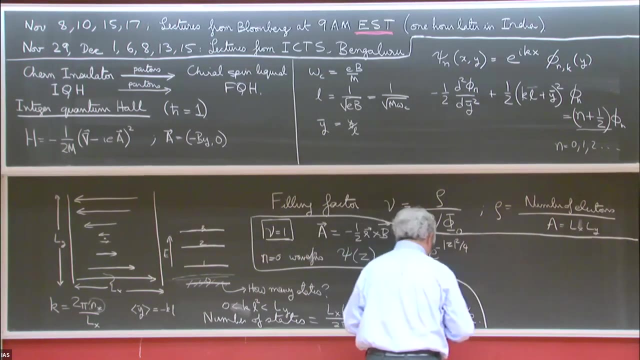 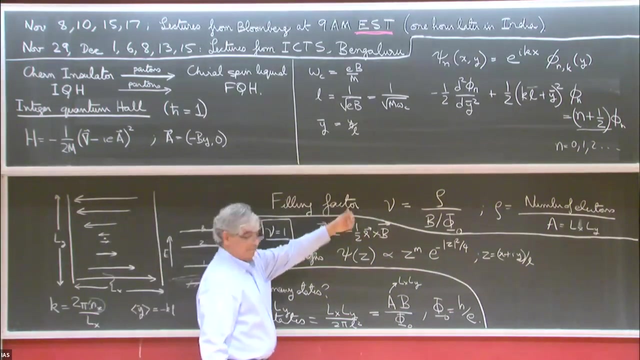 become very simple. they become analytic functions of z, psi, of z, which is uh proportional to z to the m and e to the minus mod c squared over 4, where z is plus iy. So in this particular gauge, which is explicitly preserved- rotational symmetry, in a sense angular momentum- the weight function has this very simple form And m is an integer. 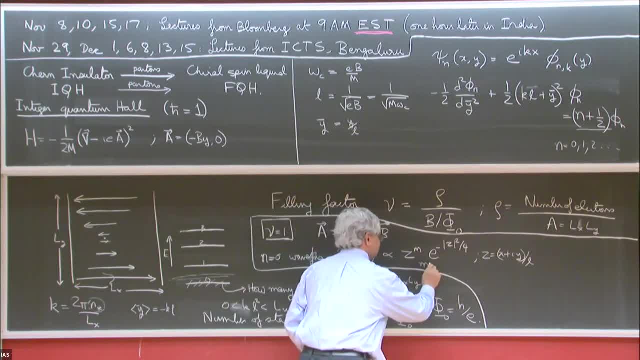 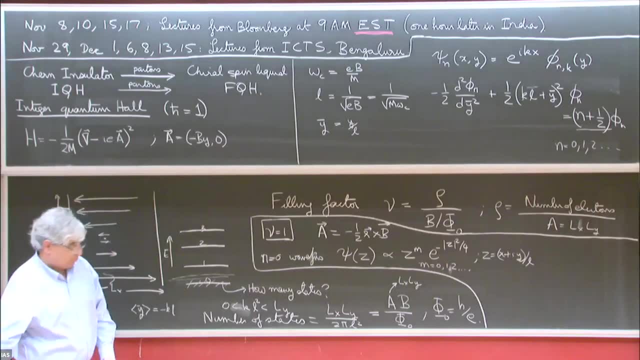 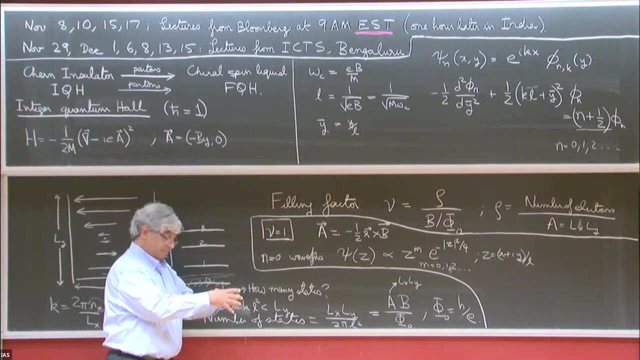 and in fact has to be positive, and so on. And so these are the so-called circular states. You know, the n equals zero is just a Gaussian. And then you take higher and higher values of n. you get states which go farther and farther and farther out. So if you fill up a lot of these, 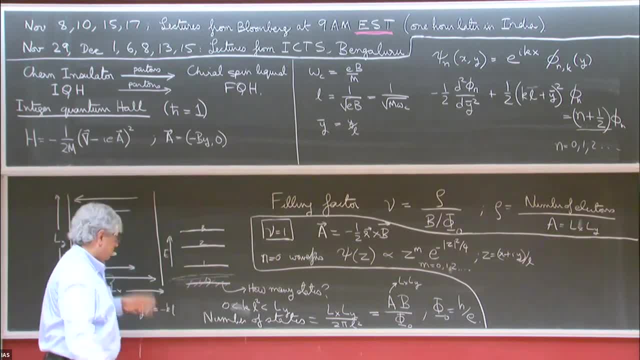 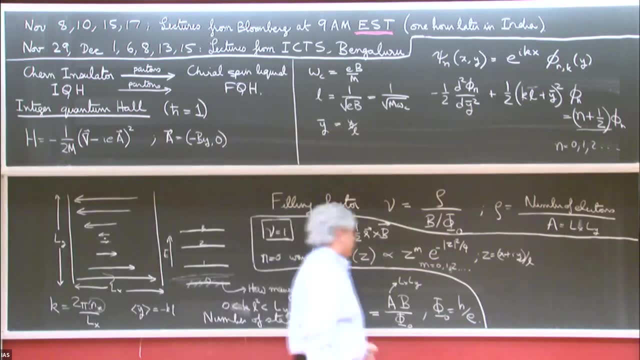 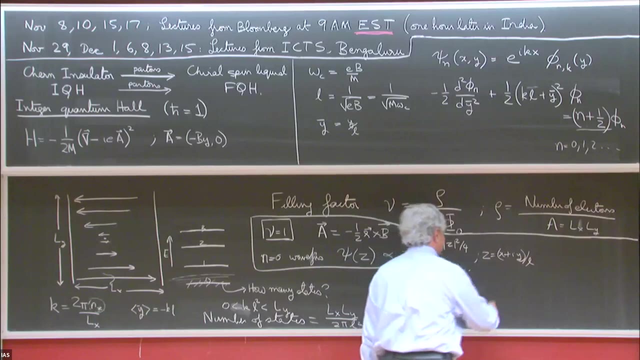 states, you'll get a sample which is the shape of a disk here, which is the shape of a strip. Okay, So one very interesting result here is: what is the actual wave function? So suppose I fill up all of these states in the lowest lambda level. What is the wave function? size of z1,, z2, all the 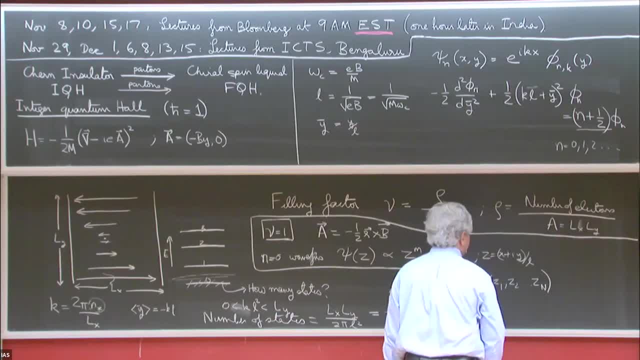 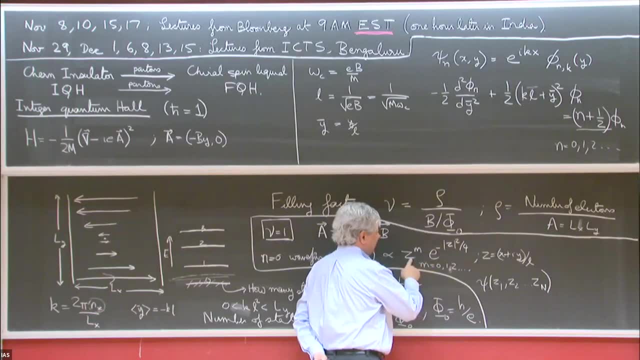 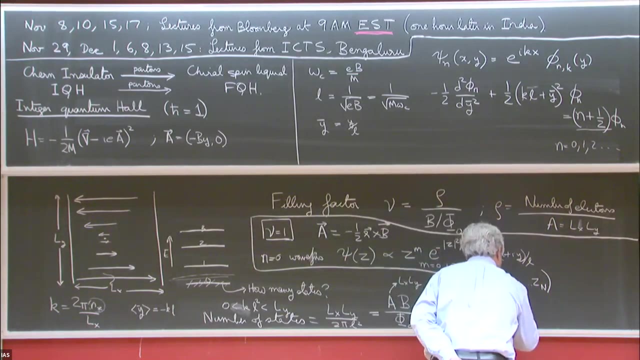 way up to zn, And there's a number of particles. Well, each particle will give you the same factor here, So we don't worry too much about that. But they have to have different values of m, So the answer will be the Slator Determinant. the product on i e to the minus z, i squared over 4.. 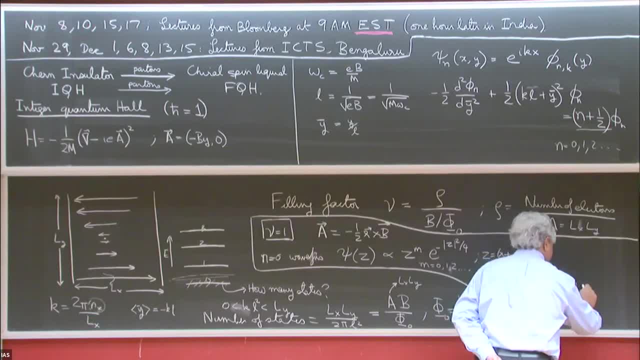 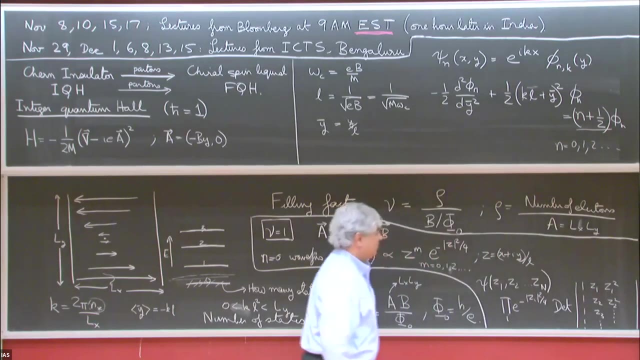 And it's a determinant of you know, 1, 1, 1, 1, 1, z1, z2, z3, z1 squared, z2 squared and so on, And that's the determinant if you fill in the lowest n m value. 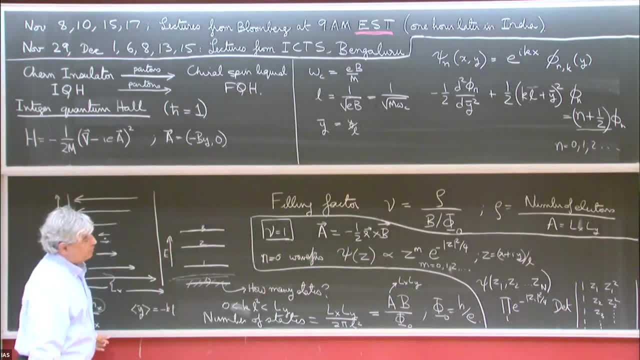 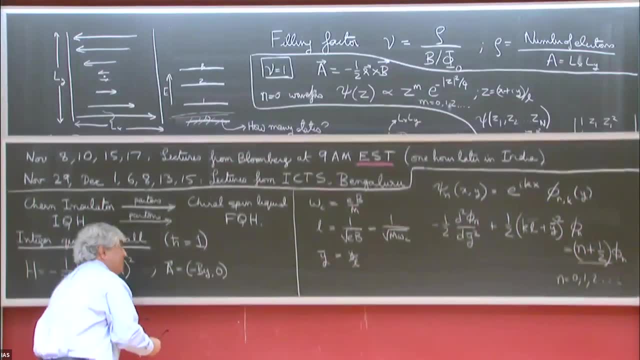 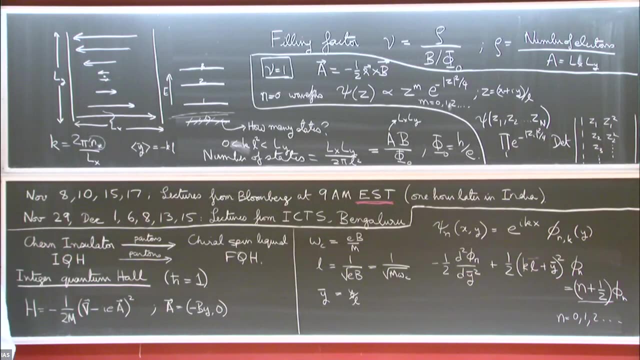 Of these single particle states. Okay, So that determinant is called a Vanderbilt Determinant. It has a very simple expression which will be of course much more useful in the in the fractional quantum hall case. So you can just evaluate that determinant and write a much simpler expression for it. 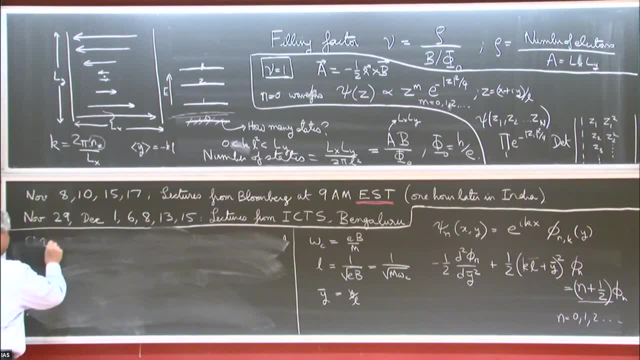 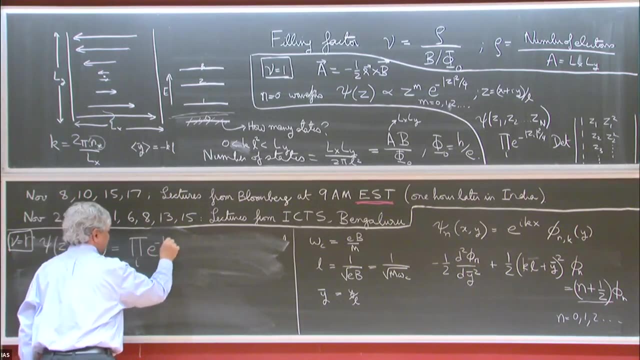 So this is a new equals one wave function. The term is psi, So this is a mu equals one wave function. The product on i e to the minus z i squared over 4, and the product on i less than j of z i minus z j. 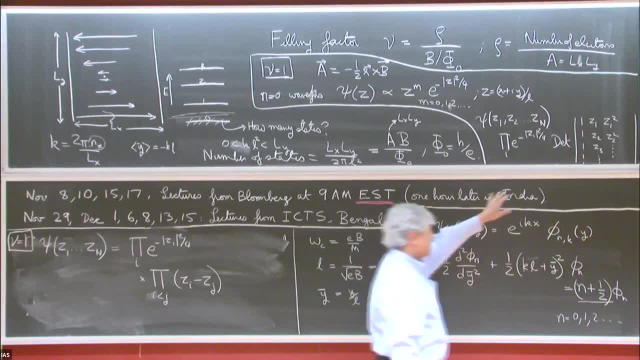 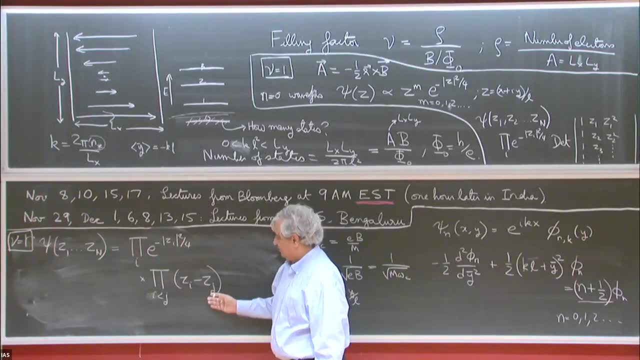 So this expression here is identical to this expression, this data determinant, You know. this form seems to suggest there's some correlations between the particles, but it's a product of pairs of particles. This one makes it clear. well, any correlations there. 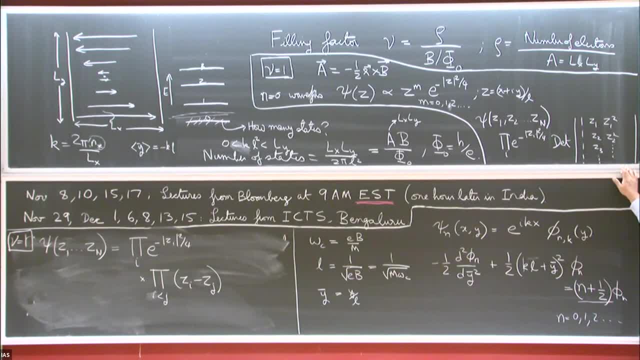 are purely due to Fermi statistics and nothing else. And why is the determinant equal to this? Well, it follows from the fact that this is a polynomial of a certain degree, And this polynomial vanishes any time any two of these z's are equal. So when z2 equals z3,. 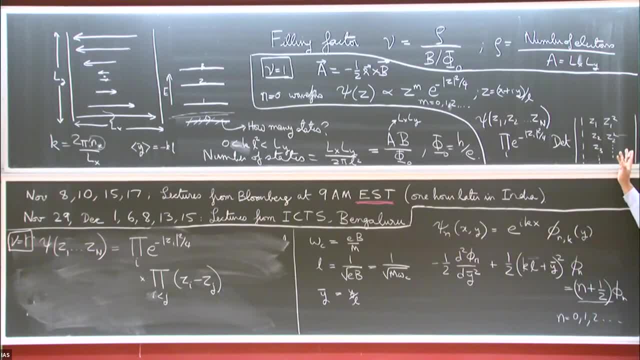 then these rows become identical and the determinant vanishes. And if you just count the degree of the polynomial which vanishes at those points when any pair of points are zero, then this is a unique polynomial that has that property. All right, I'm just. I'm a bit confused. So this is the weight function. for what? For? 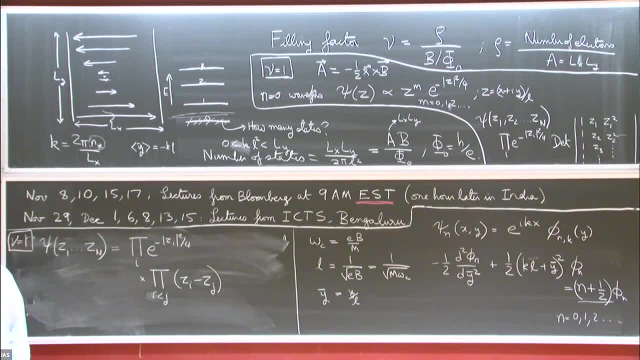 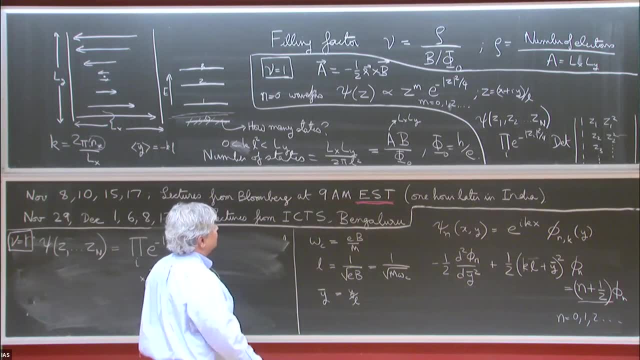 n electrons? Yes, n electrons Or n times m electrons? No, they have n electrons. There may have been too many n's here. n is the total number of electrons, And each electron is n equals zero, and that's some value of m. 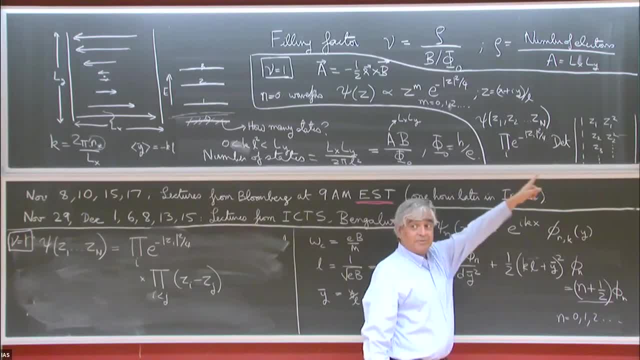 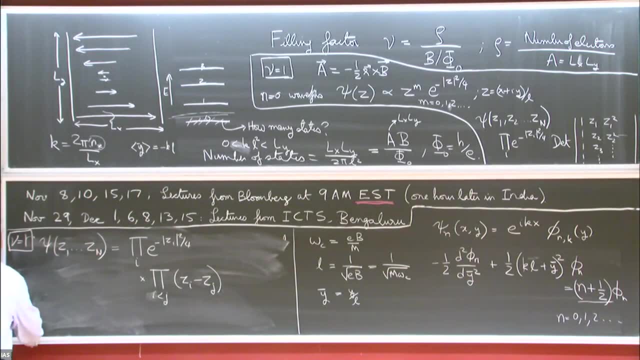 That's right. So the electrons are from m equals zero all the way up to m equals n minus one. So this wave function, you know, if you actually look at the density of particles, you look at the density average value of the density. 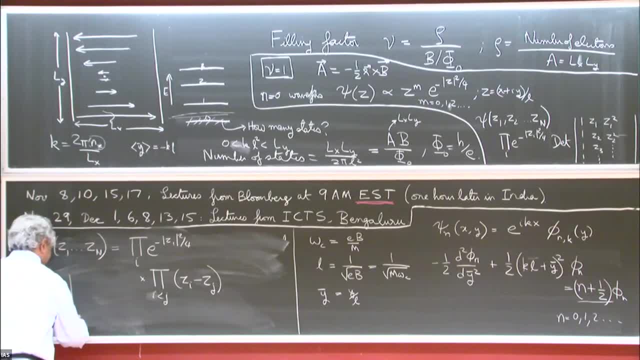 for this wave function. you can compute it on a computer if you wish. So this is. it's of course angularly symmetric. It has something looks something like this: It's essentially flat here, The density here is rho, But it has an edge, and at the edge it goes very exponentially down to zero. 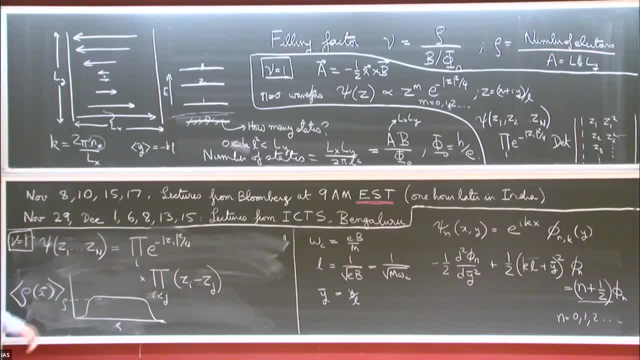 So that takes a little, you know, work to prove it, but it can be proven. Take the modulus squared, the wave function. this becomes the typical mechanics of a Coulomb gas in two dimensions with log interactions, which is the Coulomb interaction, two dimension And from properties. 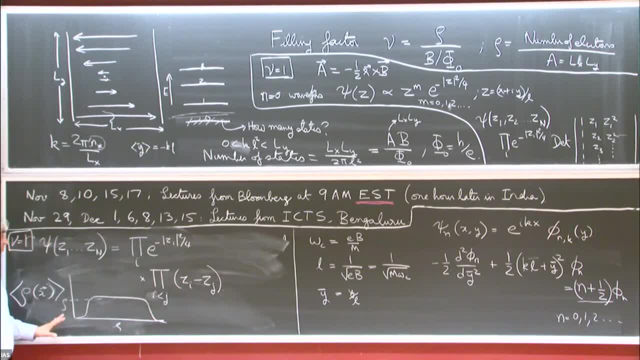 of the electrostatics of charges in two dimension you can prove this wave function. even though it doesn't look, it is actually a state of uniform density, except right near the edges. So this is this distance here. Well, it's whatever the distance you need to. 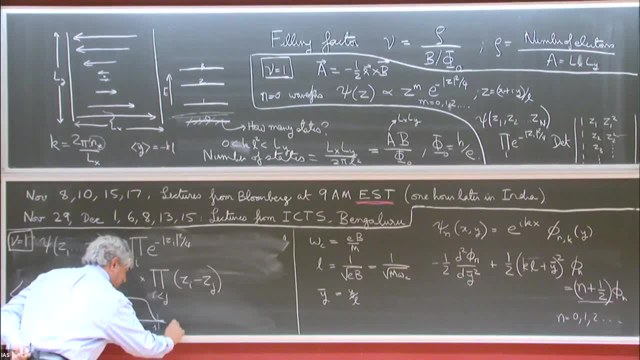 you know, call this r, then Pi r squared times n. look, Pi r squared times, the density times n number of particles. All right, And rho is the inside of r. So I have a n, number 4, which is equal to. 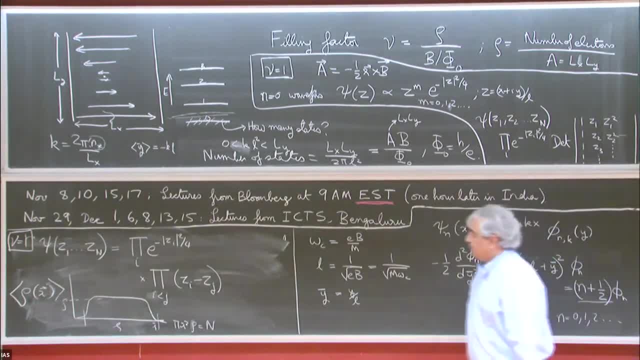 Alright. Alright is the density of a filled band. that's right, rho. is this density, here, this value? of course, here the density will look rather different. it'll be the same in the center, but on the edges it will fall off and we'll have the rectangular shape. 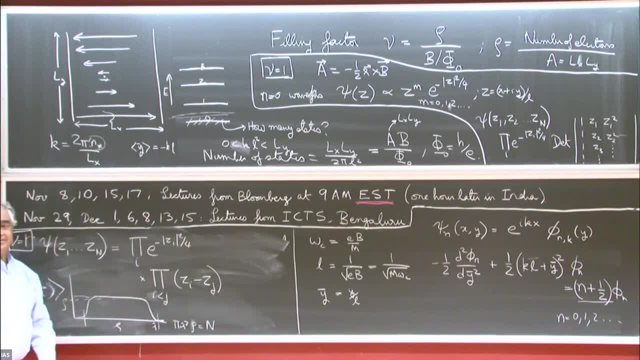 if we took those states here, you get a circular shape. okay, all right. so what I want to consider next, then, is: go, I'm going to go back to this rectangular shape and look at the edge states. we go through the application, okay. so now we are back to the, the other gauge. 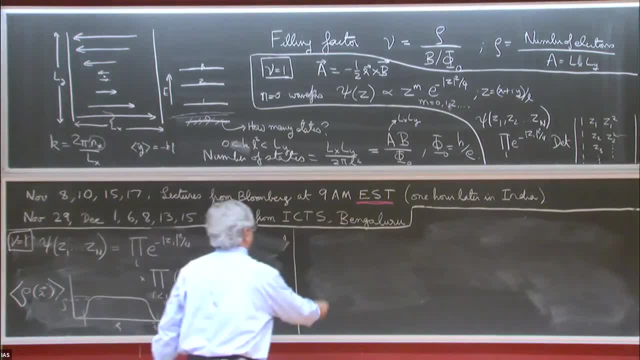 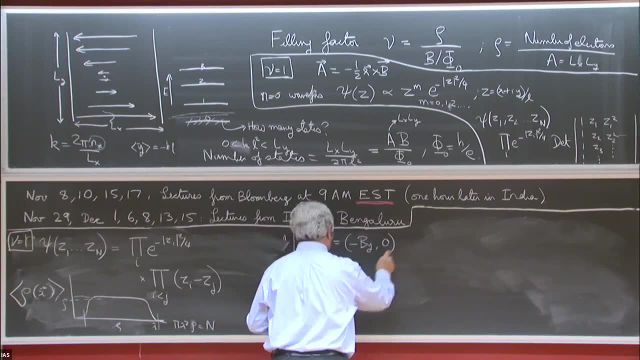 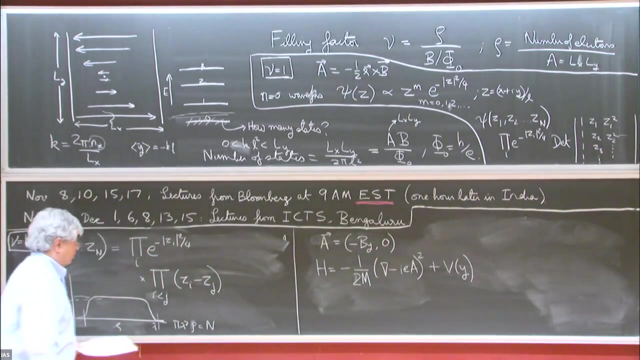 okay, so we're back to the gauge. a equals minus e, y and zero, and I'm going to consider the Hamiltonian h is equal to minus 1 over 2 m. okay, so I have. and now you'll see why I choose that particular gauge: because if I had a potential in this, 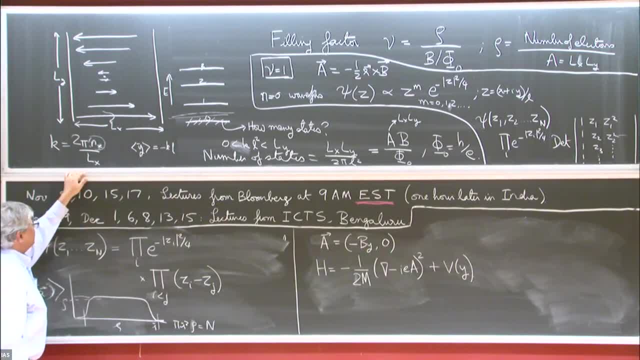 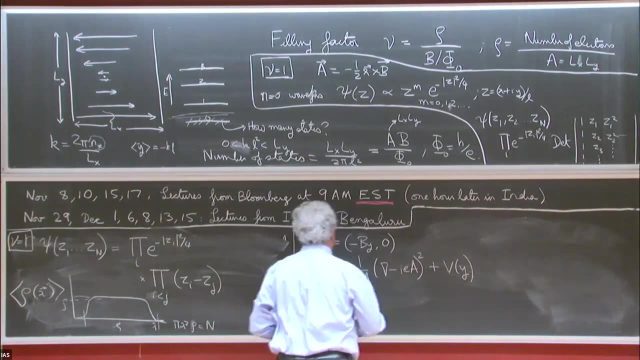 direction. so there are walls or something towards the ends. so it's a very slowly varying potential at the bottom of the sample. but towards the edge you have a boundary. but I still have a conservation of momentum in the x direction. so if I write down the Schrodinger equation now, 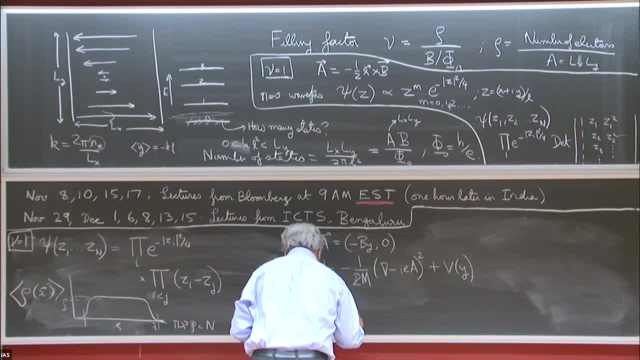 minus one over two m, and now I'm dropping the bars here- that was equal to one over two m plus one over two m, plus one over two m, state m plus, I'll have one over two m of k plus k, the moment in the x direction, plus b, y squared as we had before. 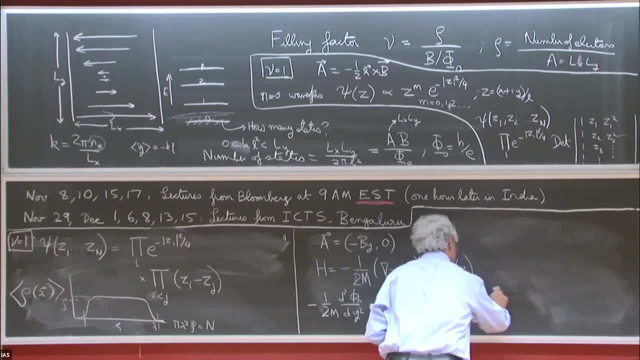 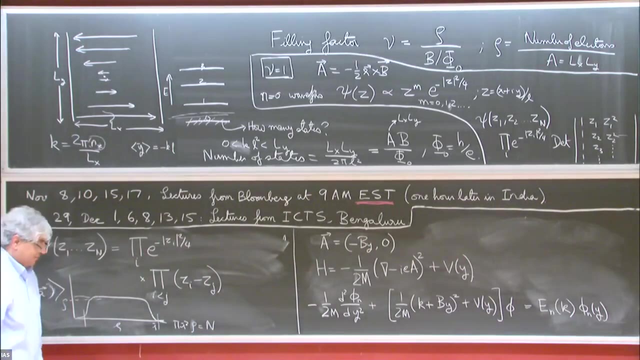 but we don't just add in the potential v of y. y will be some eigen energy, which will now depend on k times five and a fourth. okay, so this is still a one-dimensional Schrodinger equation and you could have taken v of y equals just a quadratic function of y and it's still solvable. 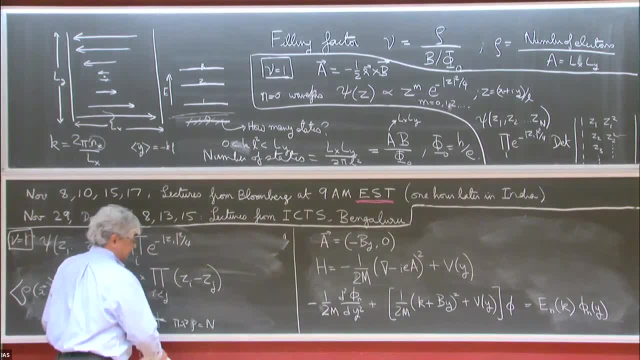 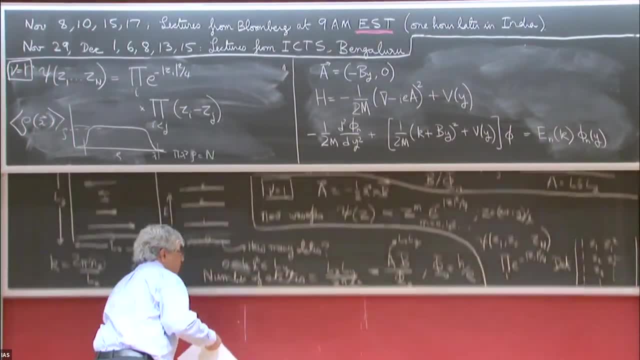 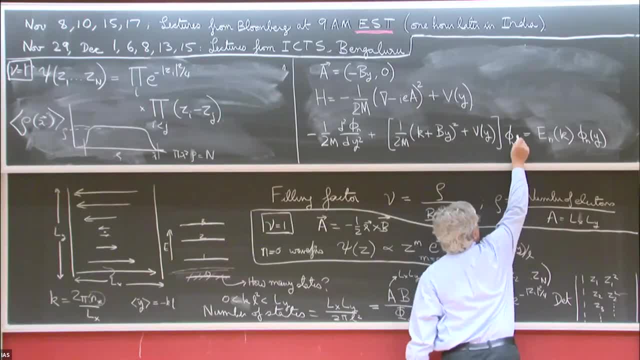 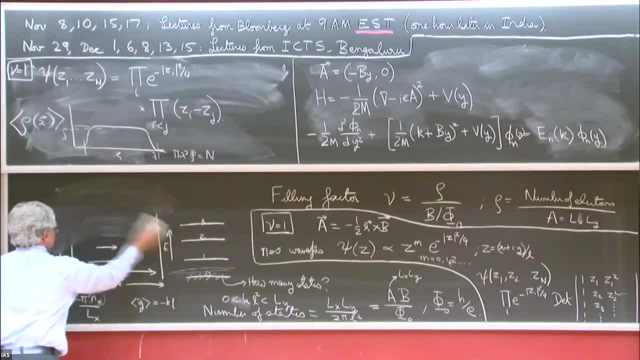 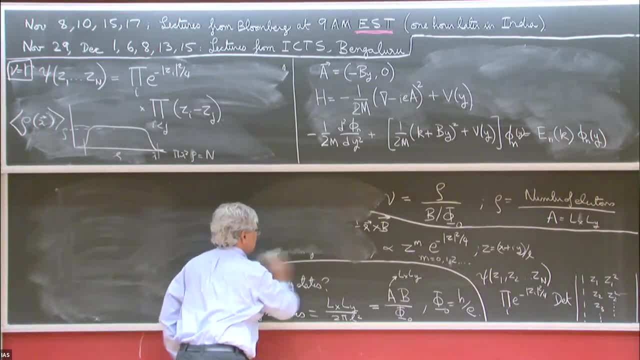 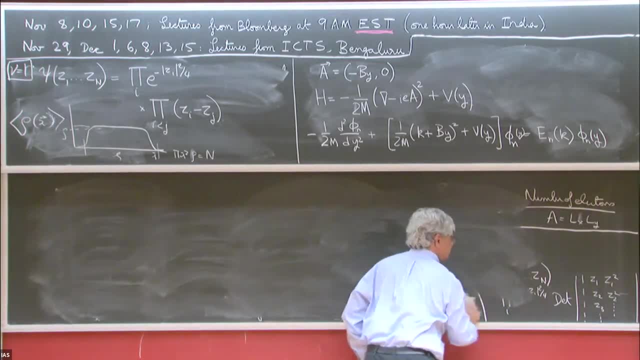 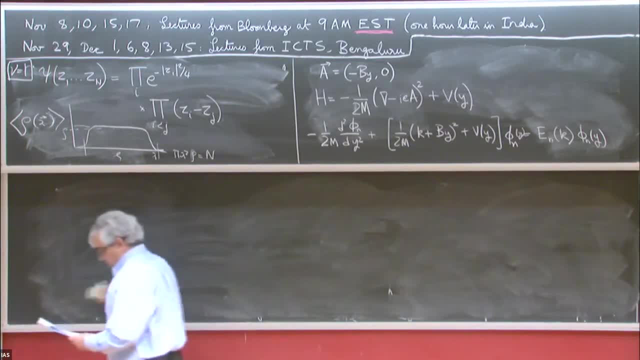 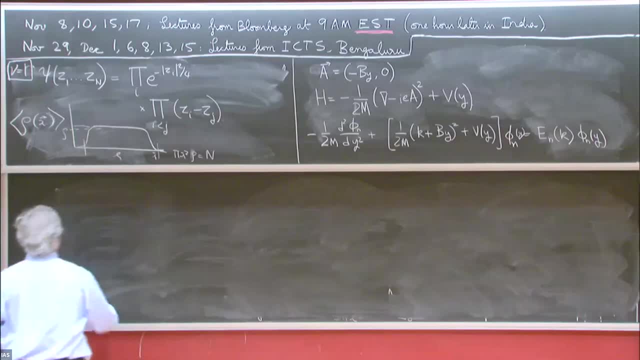 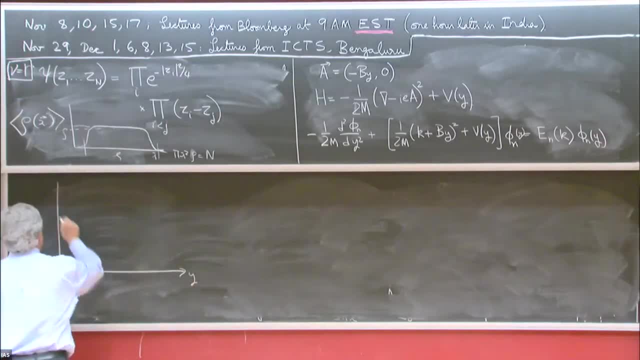 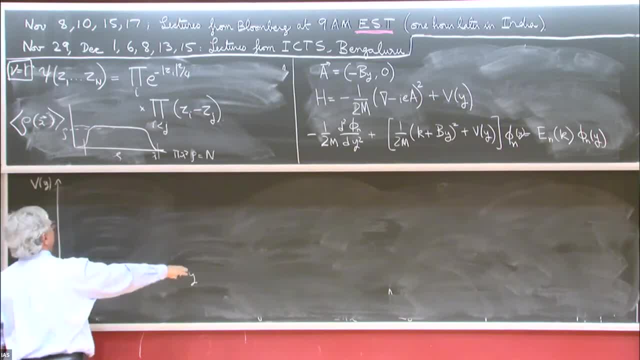 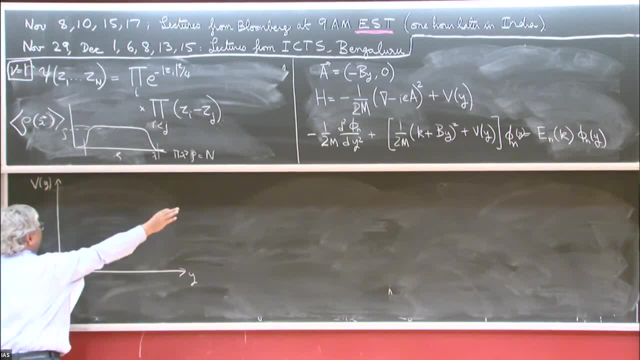 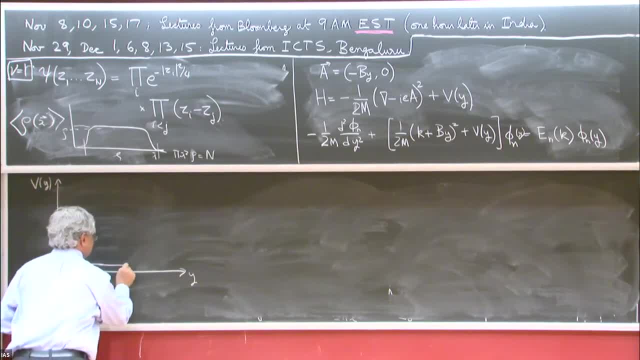 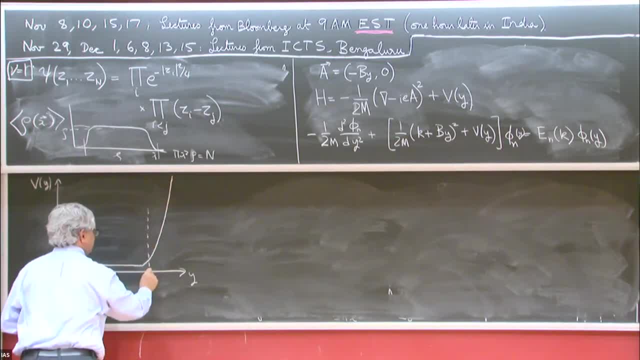 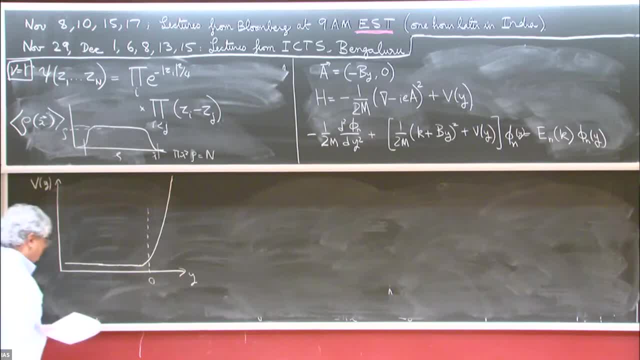 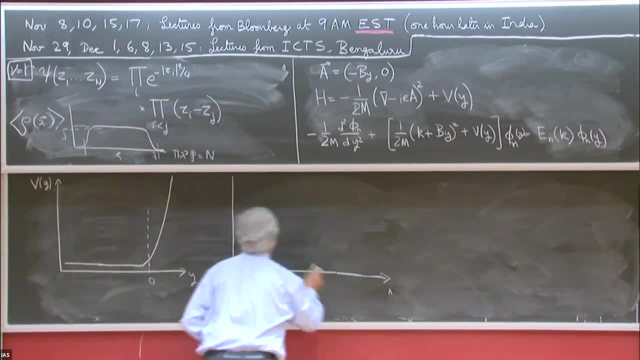 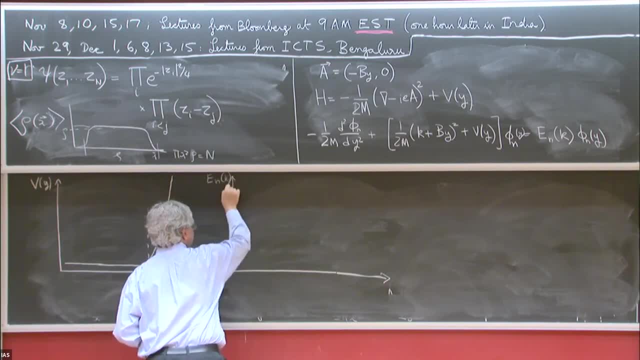 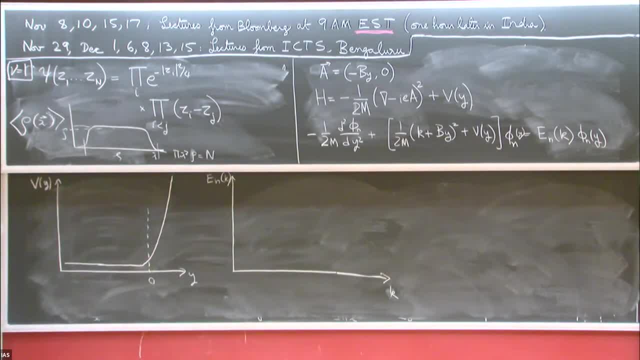 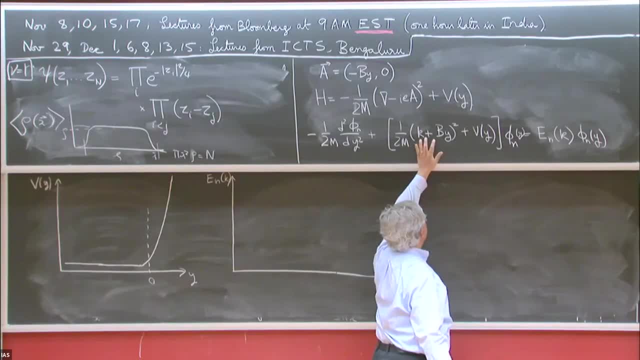 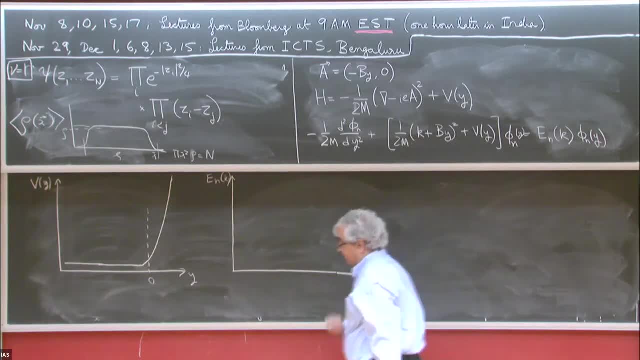 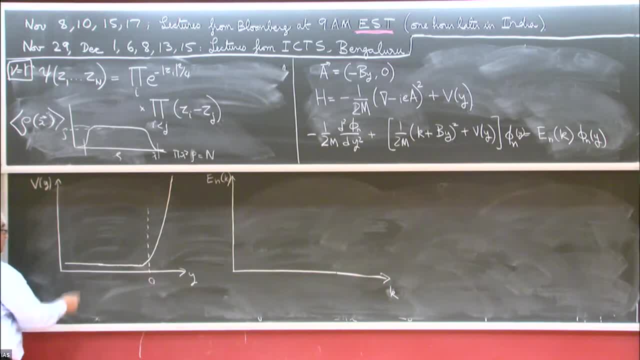 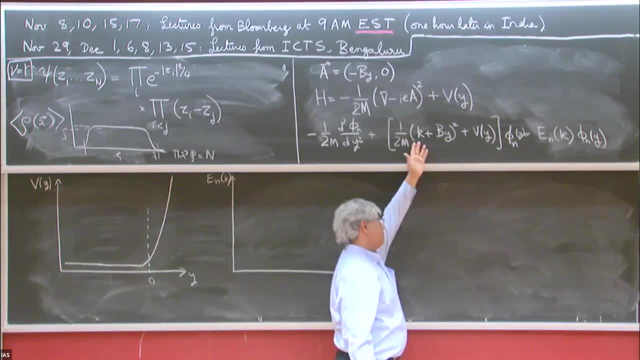 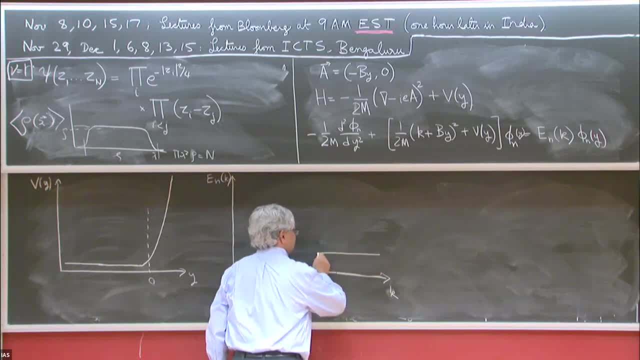 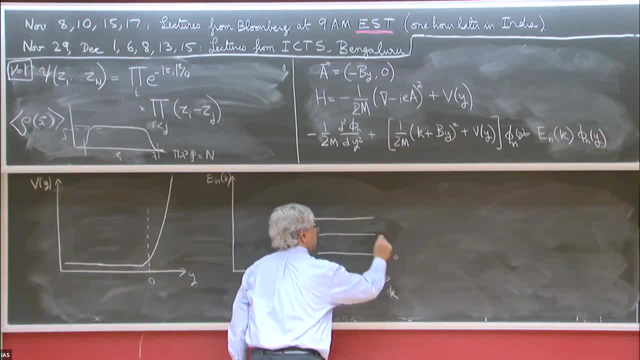 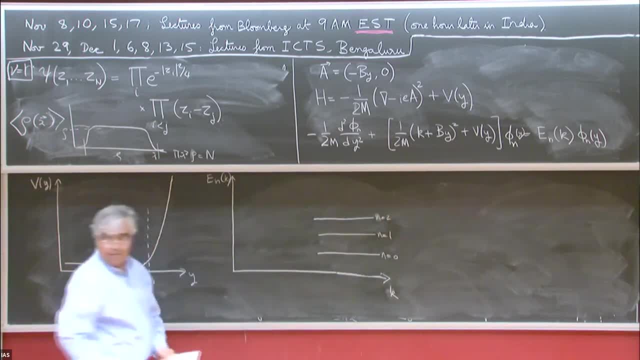 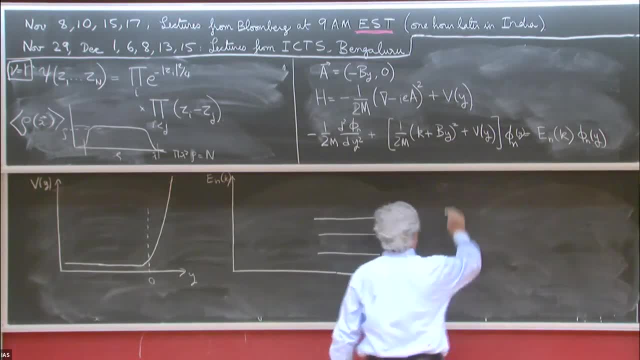 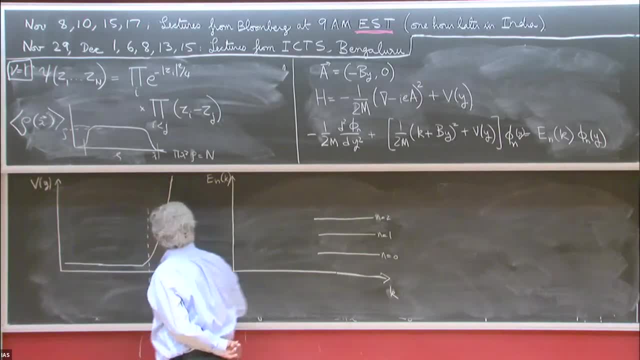 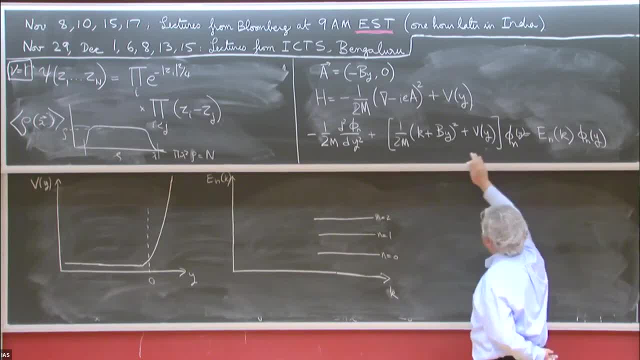 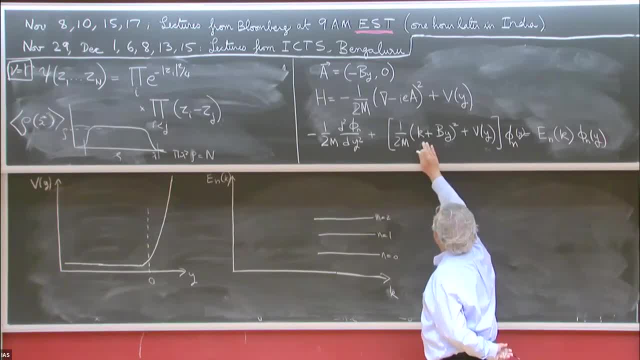 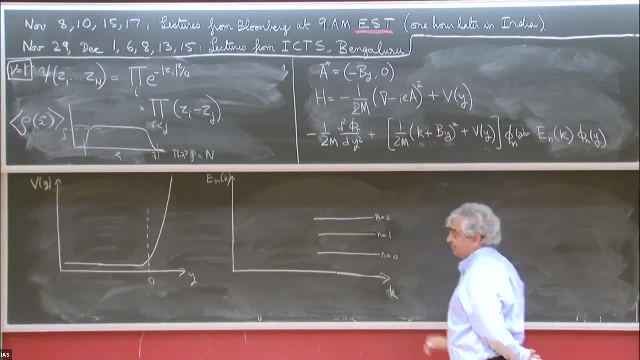 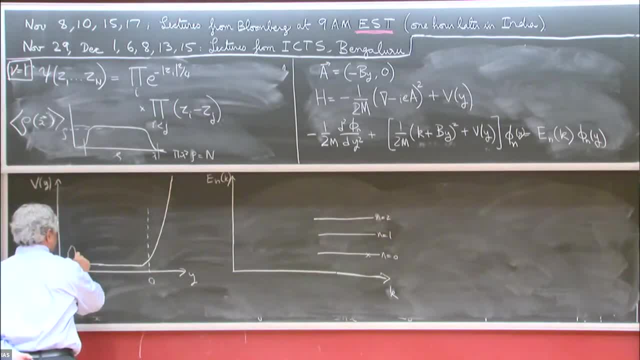 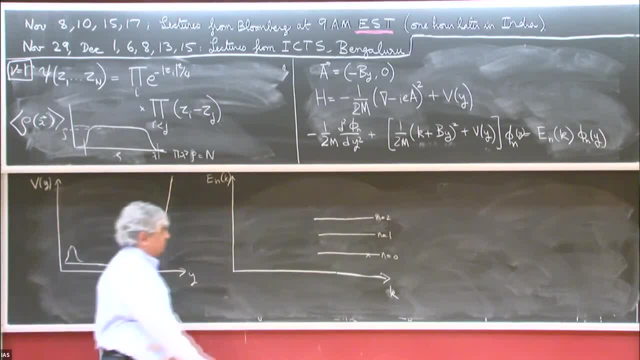 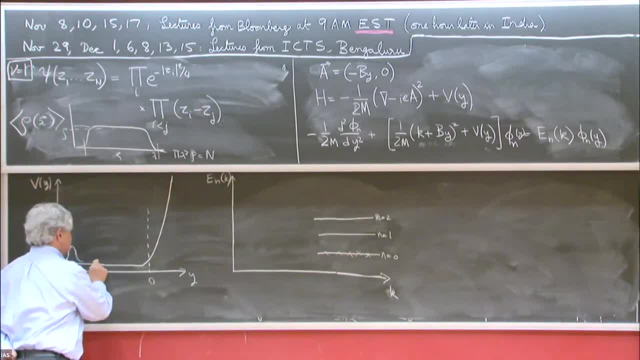 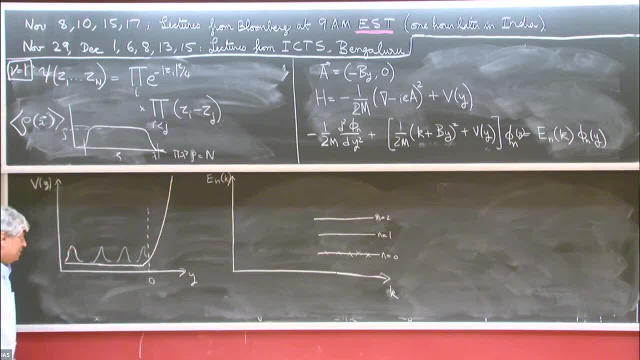 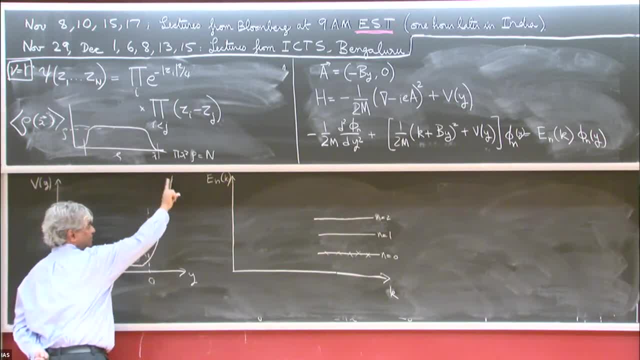 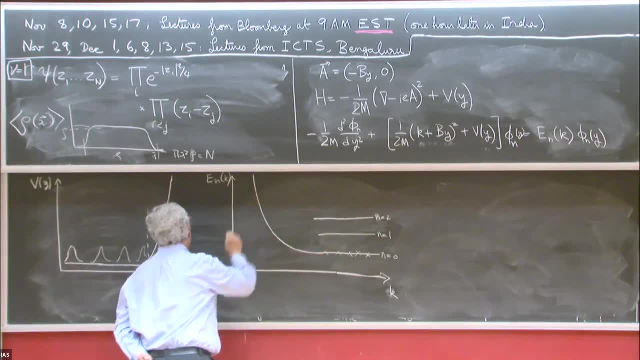 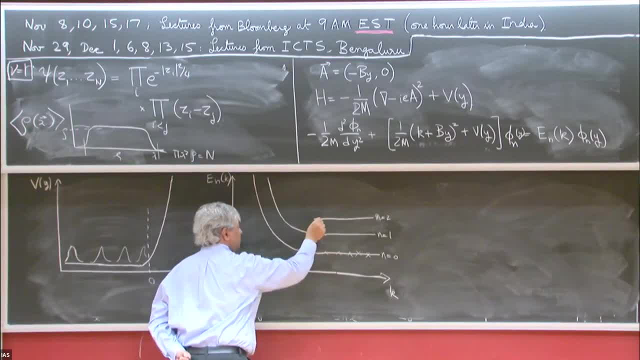 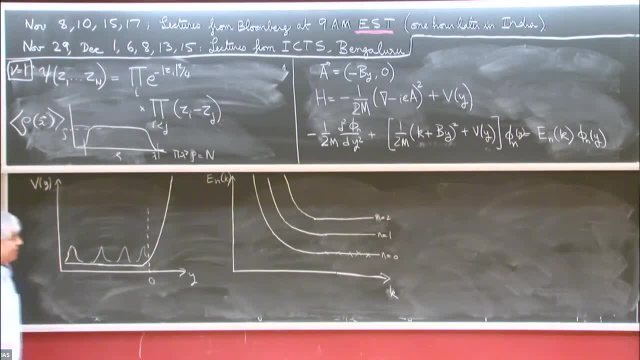 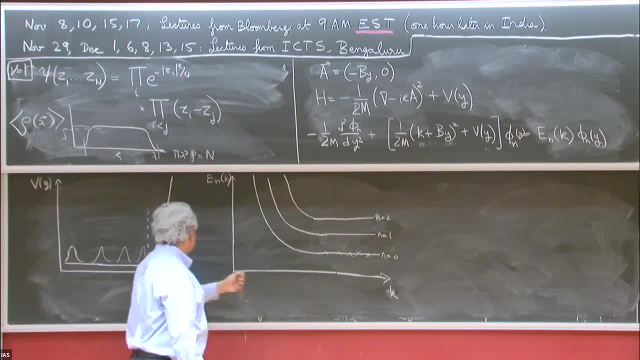 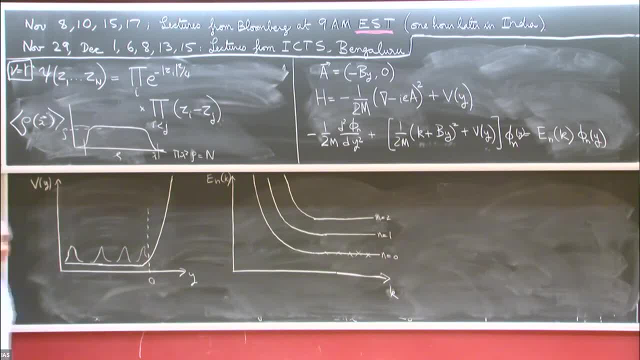 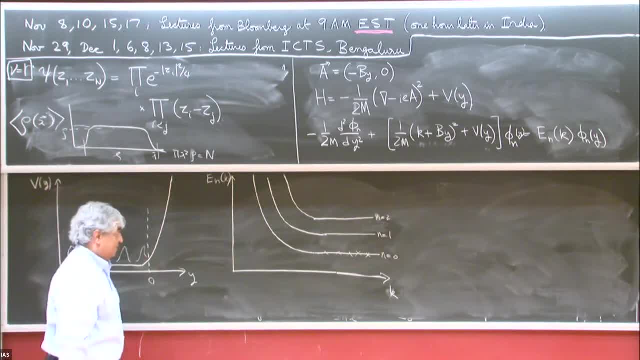 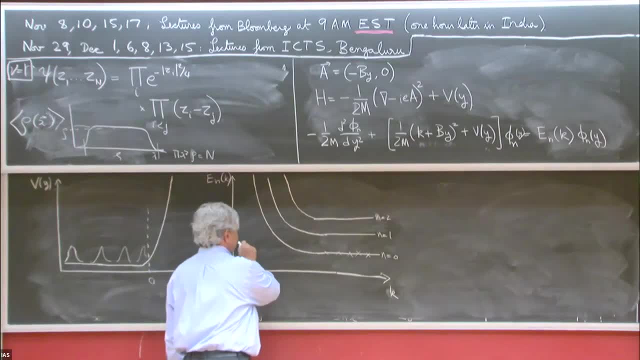 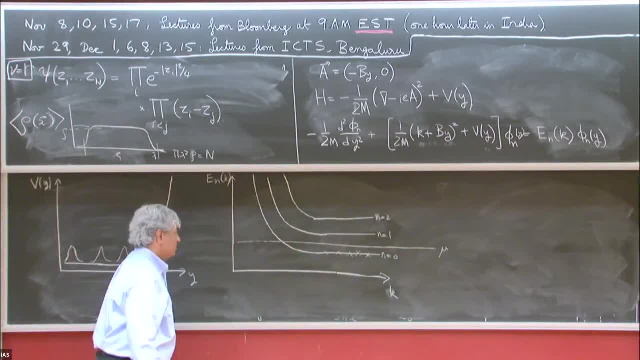 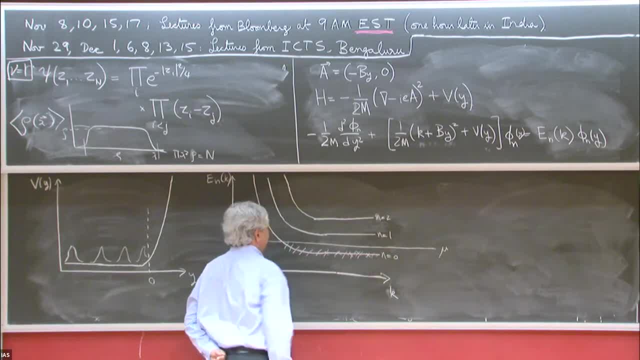 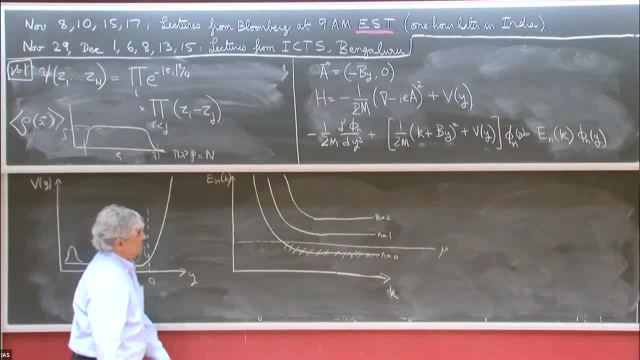 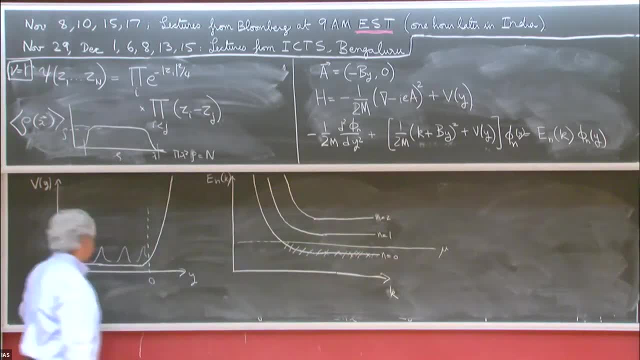 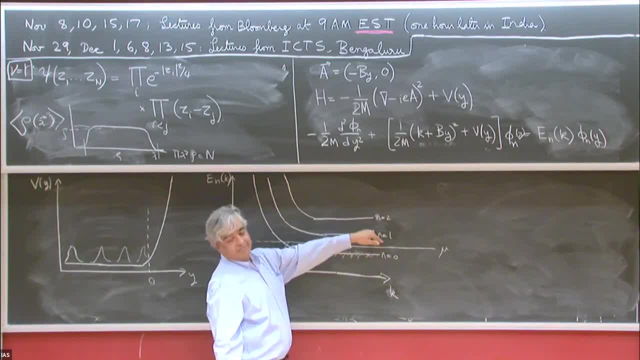 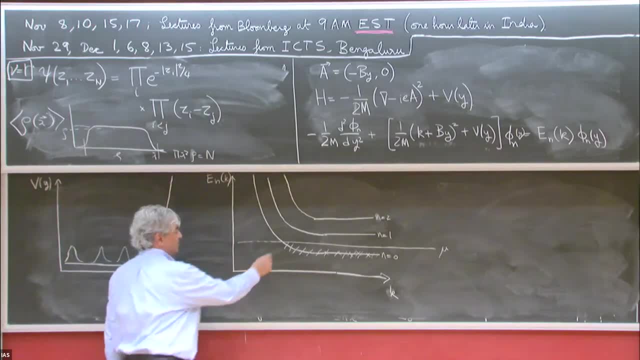 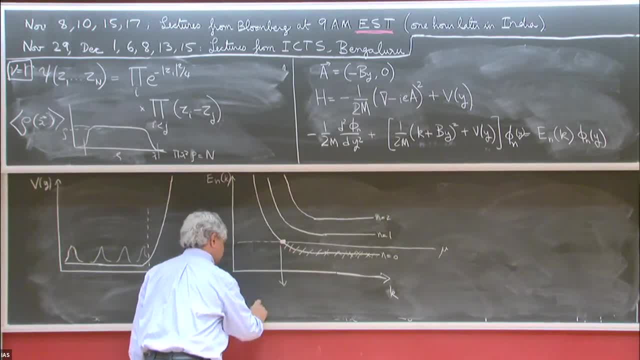 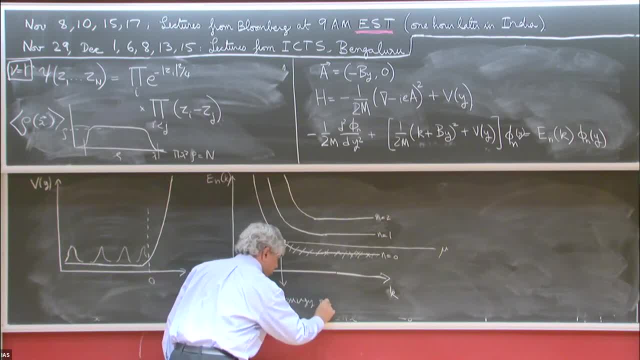 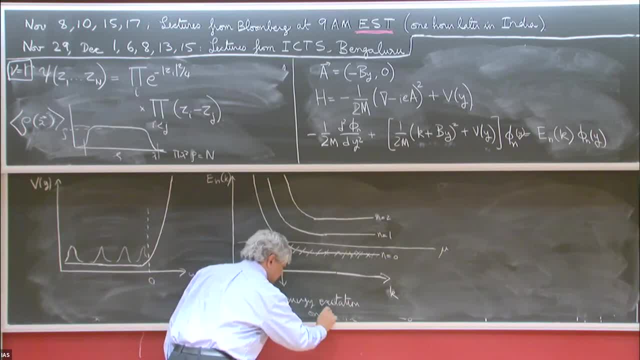 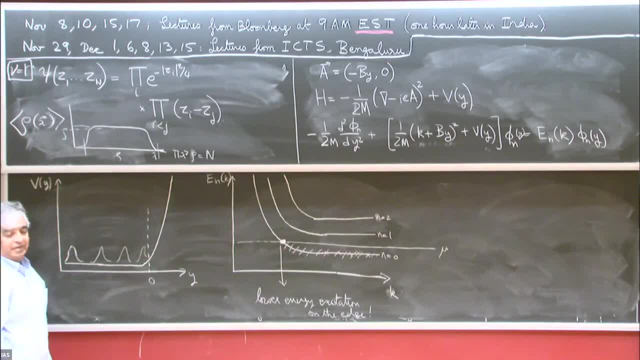 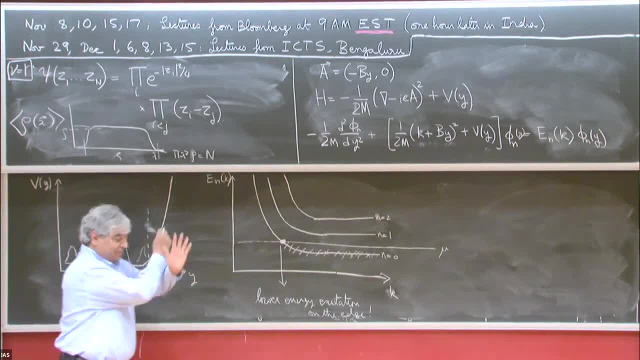 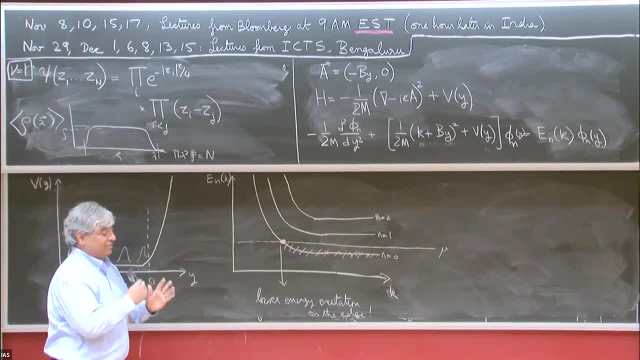 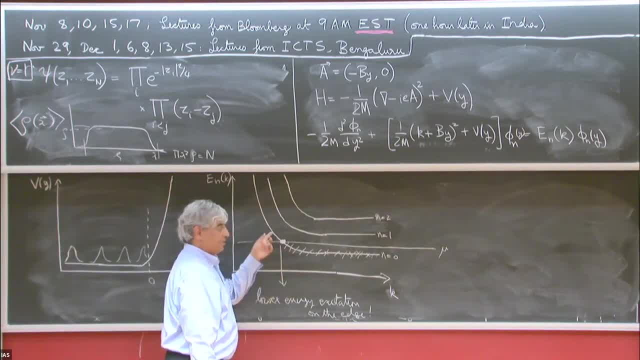 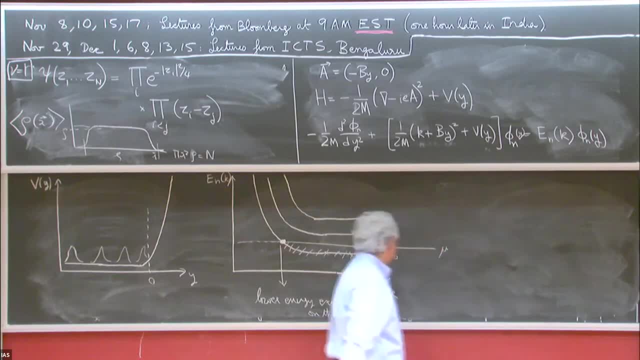 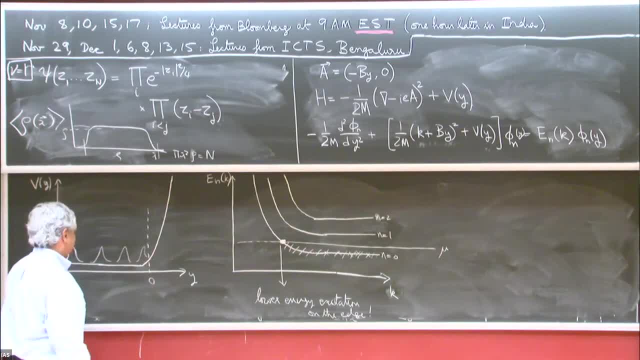 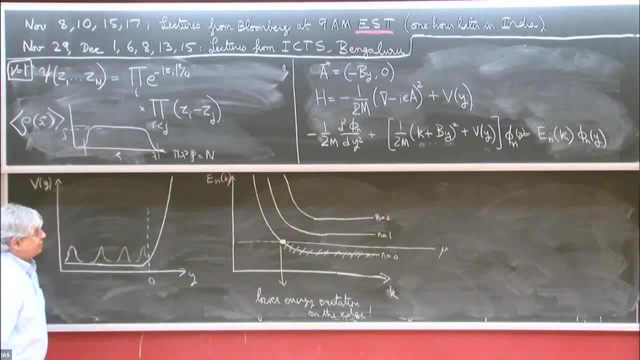 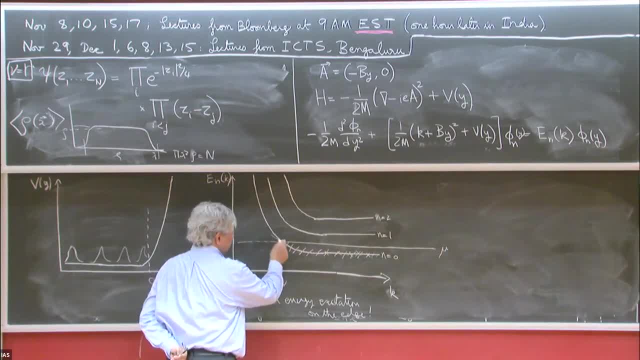 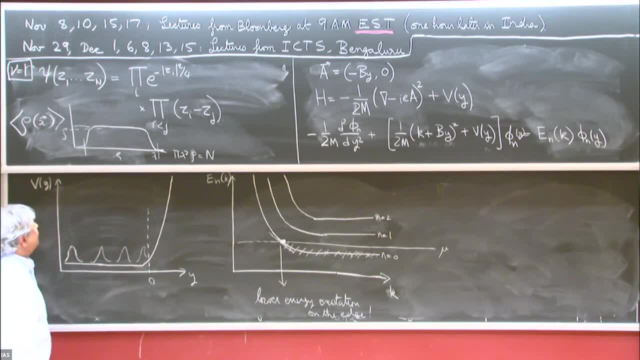 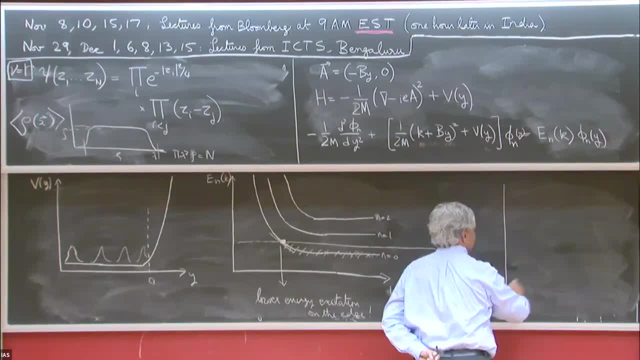 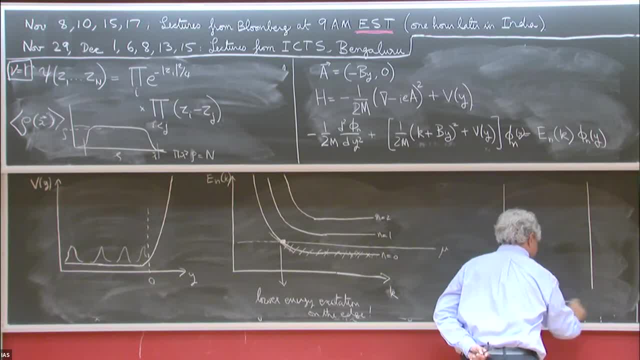 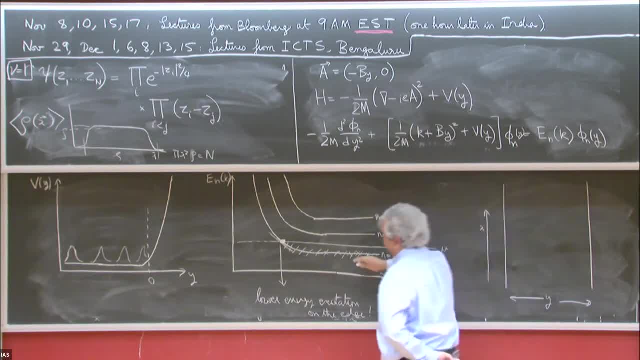 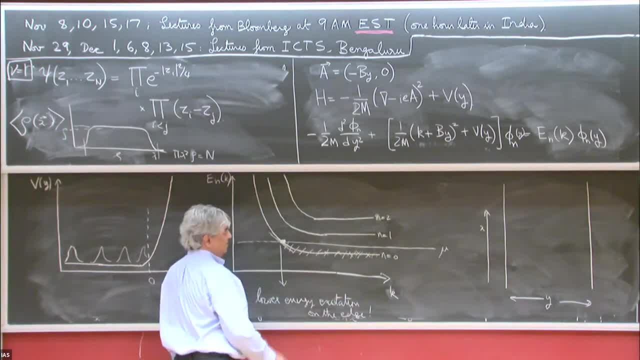 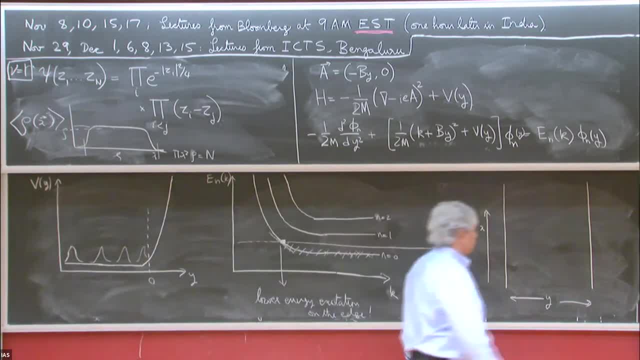 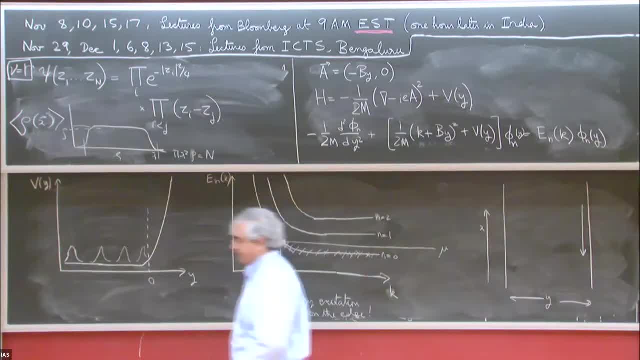 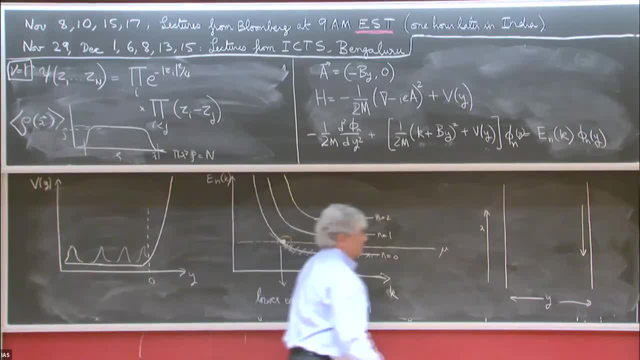 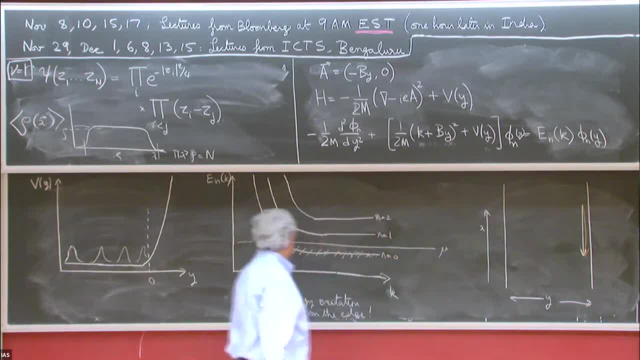 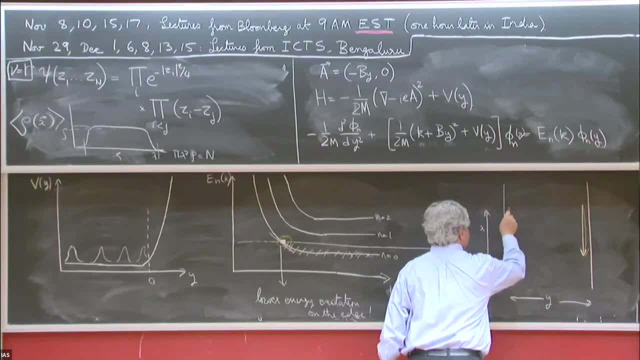 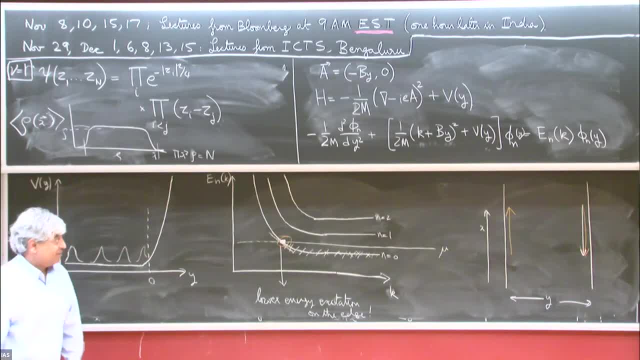 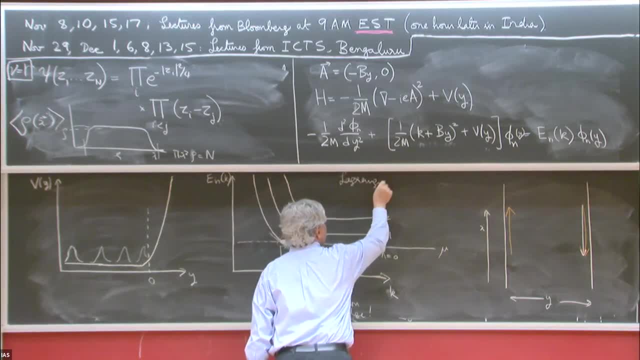 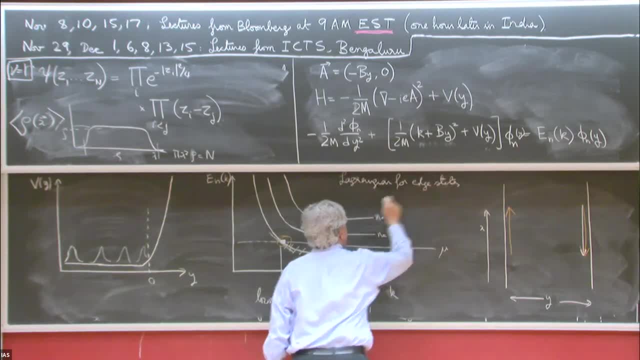 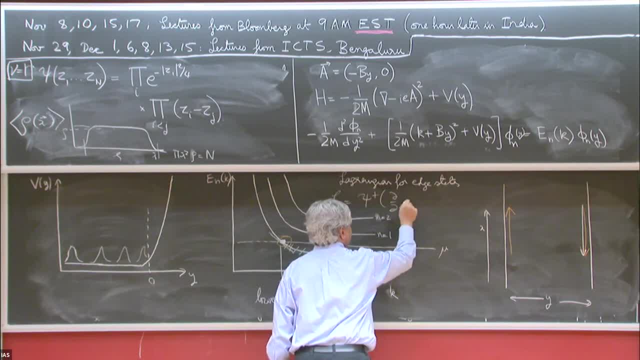 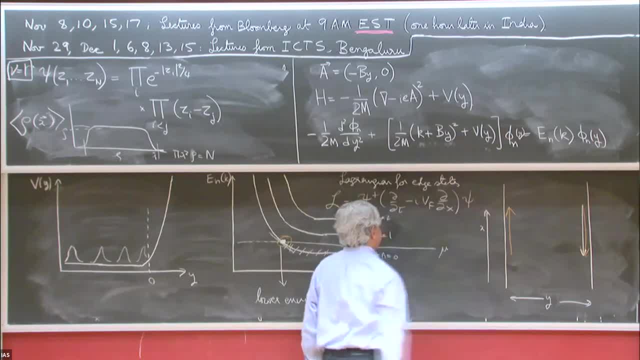 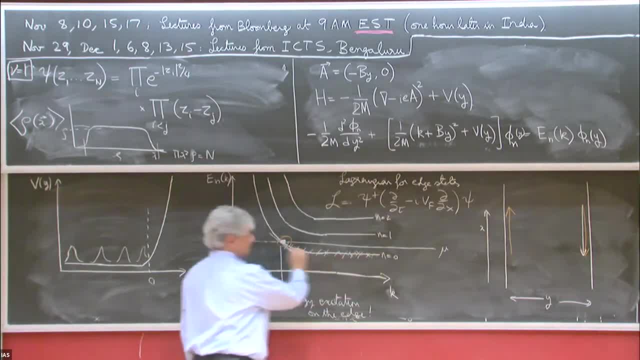 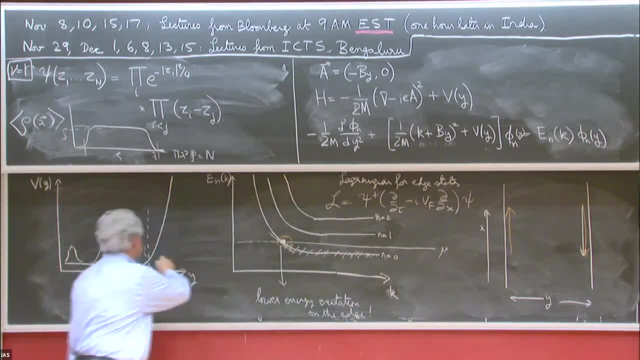 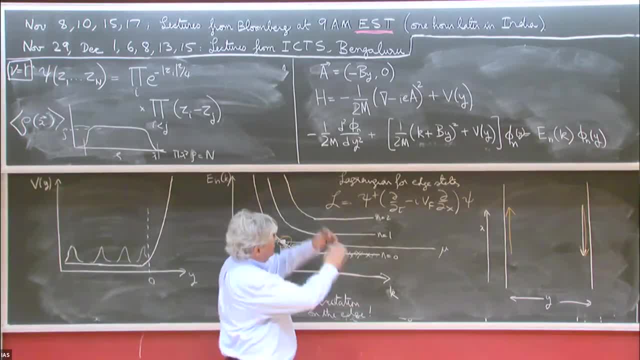 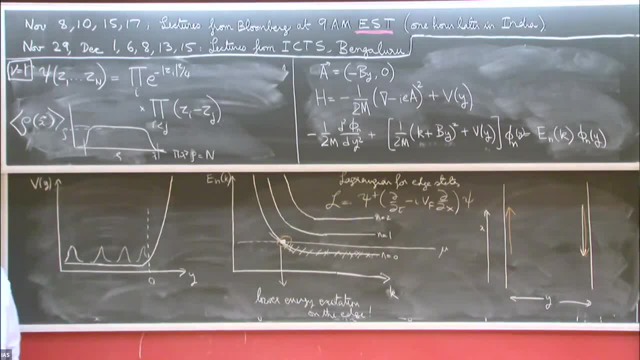 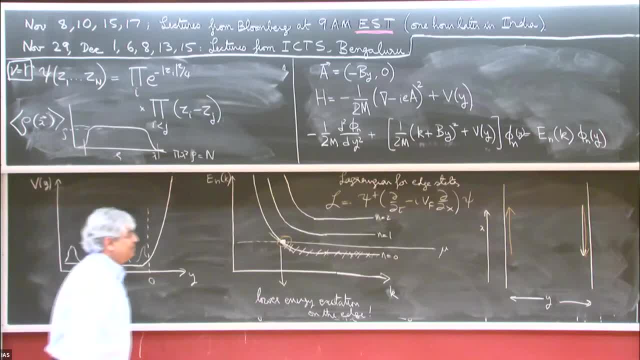 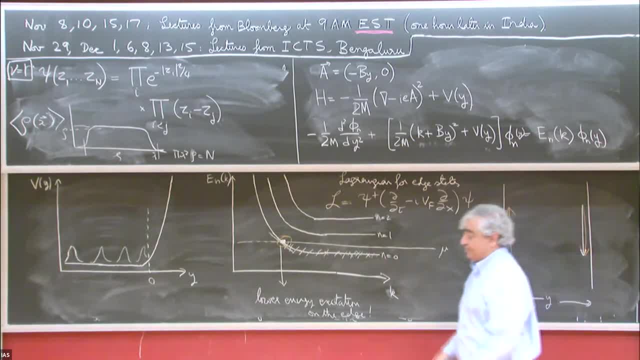 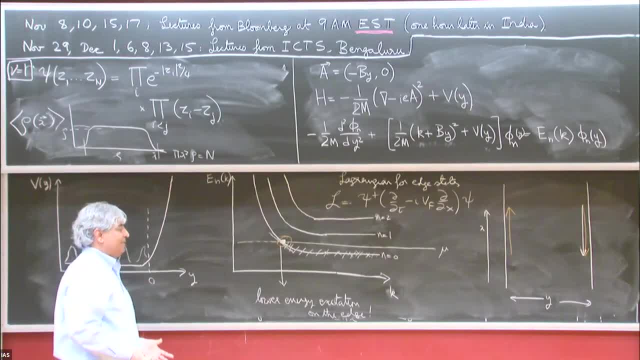 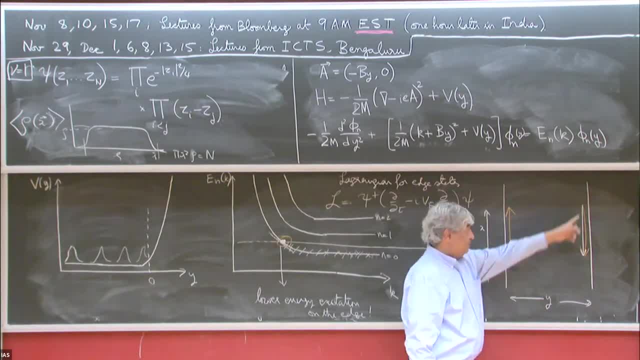 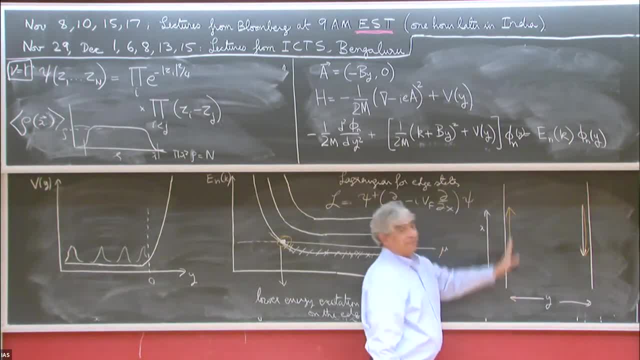 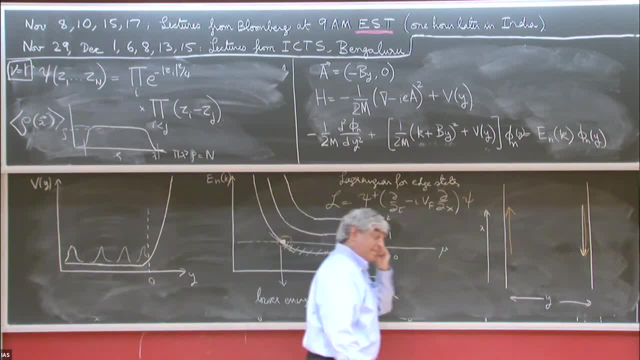 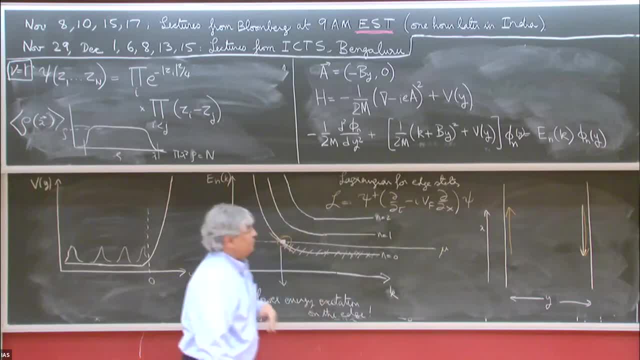 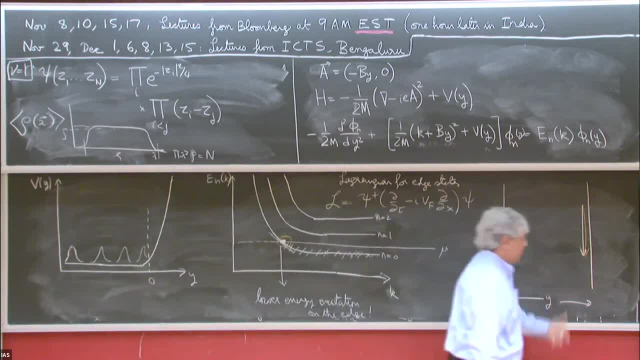 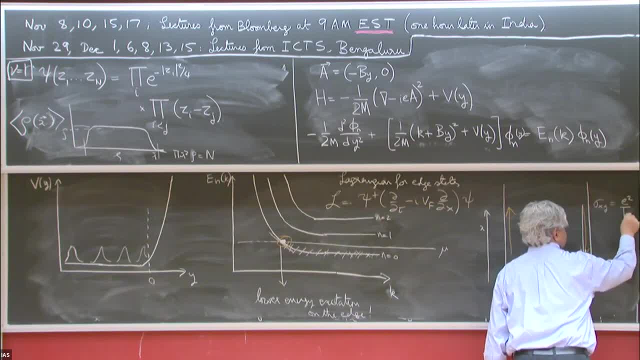 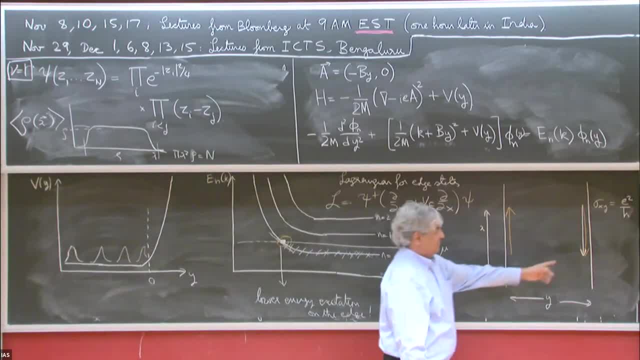 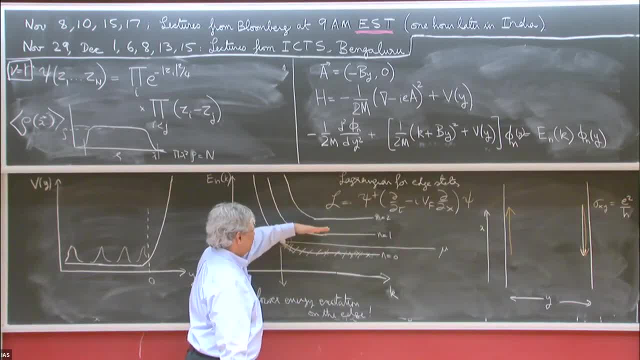 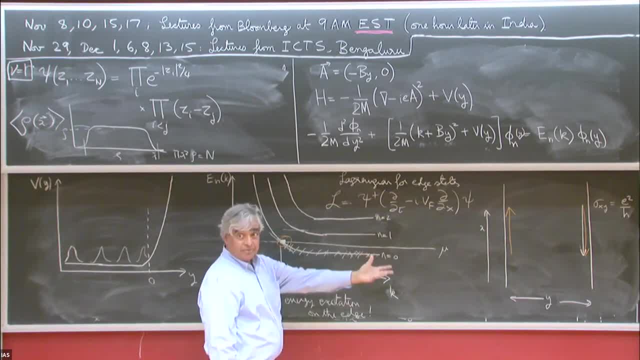 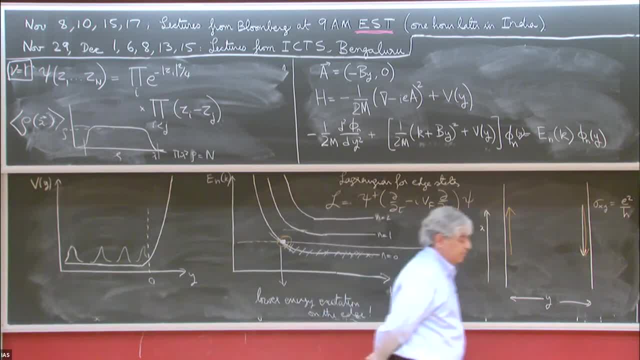 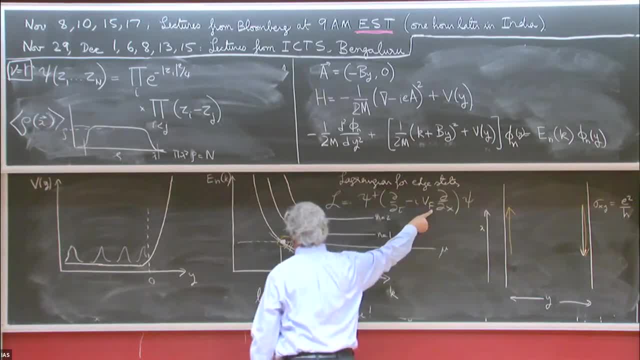 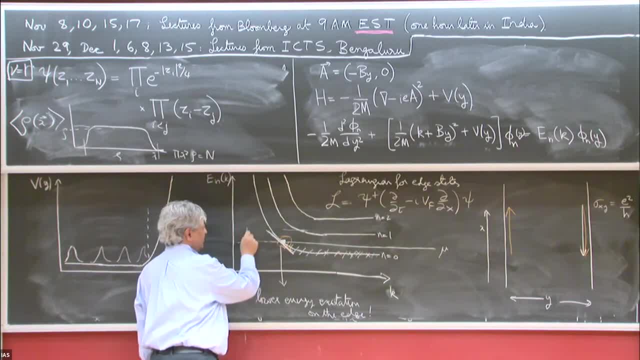 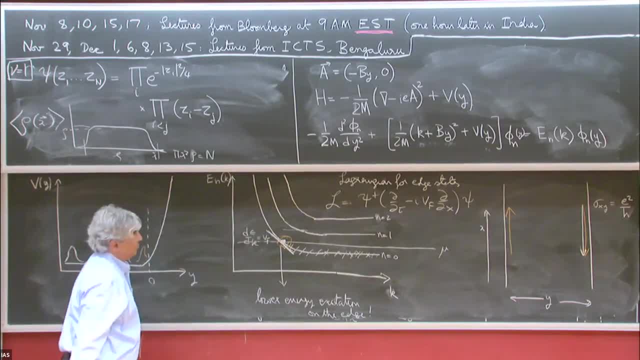 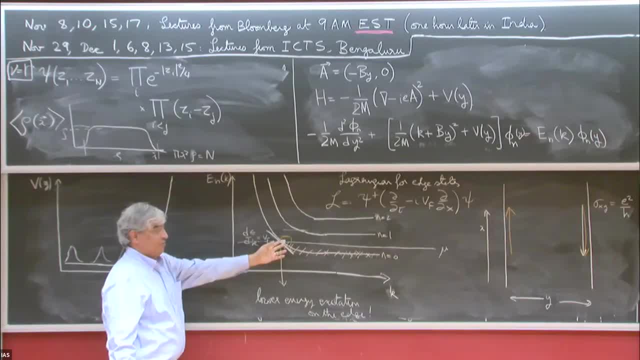 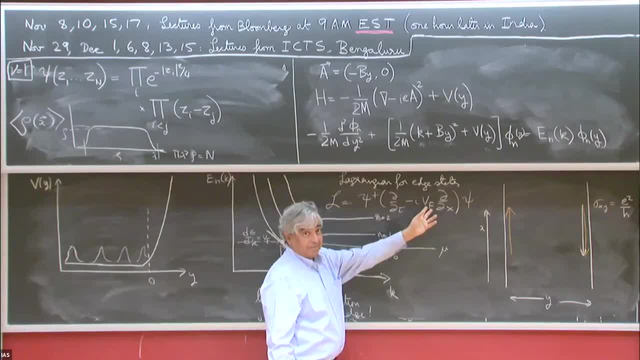 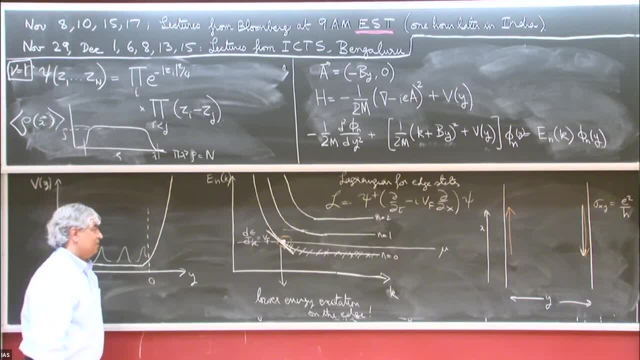 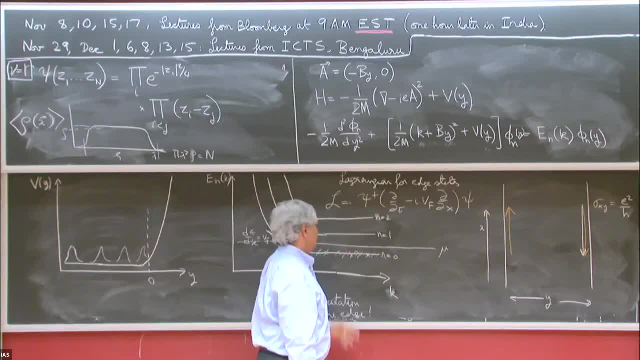 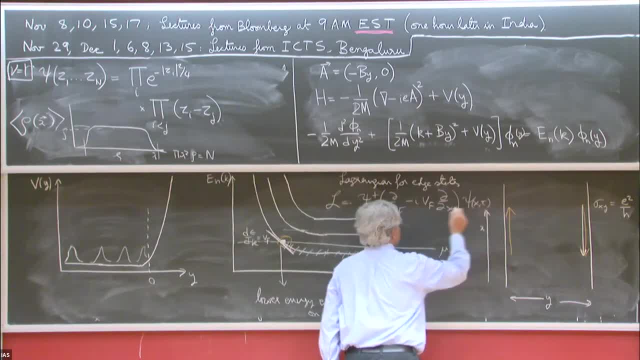 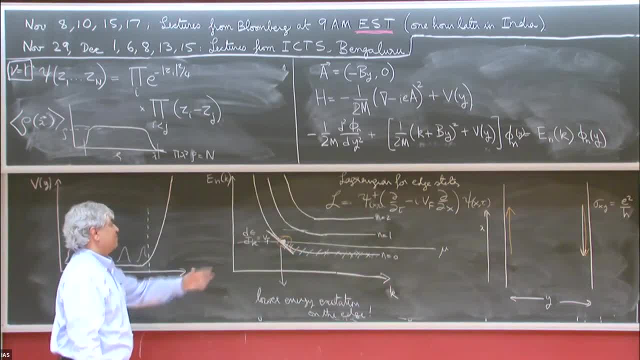 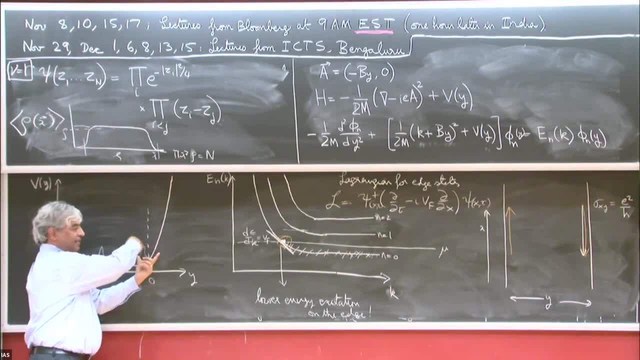 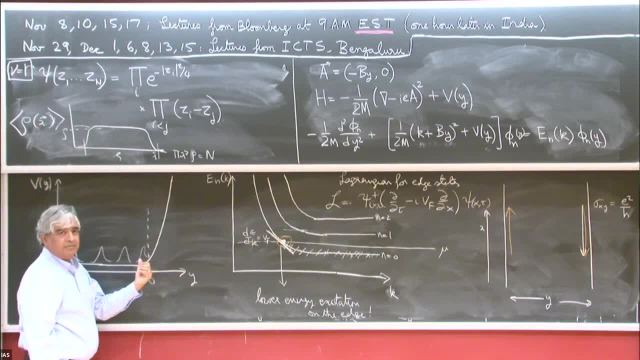 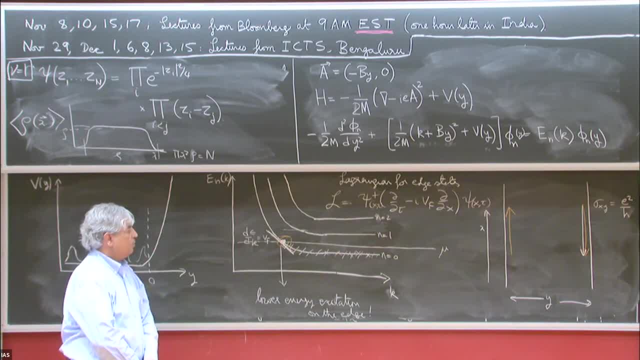 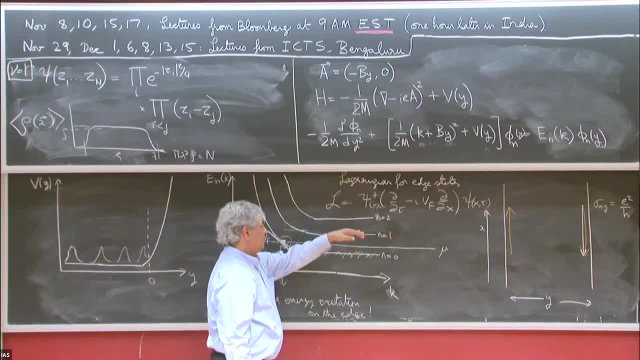 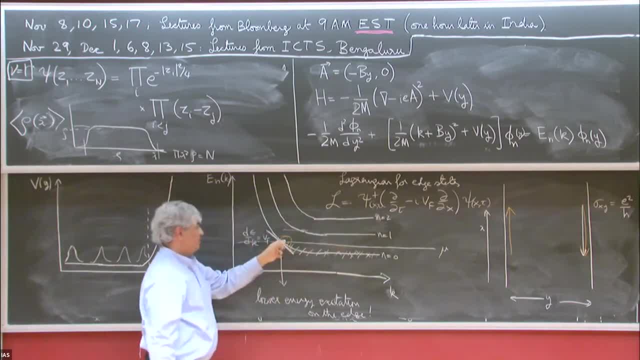 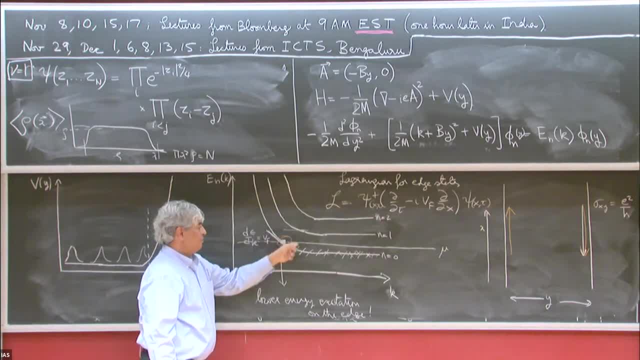 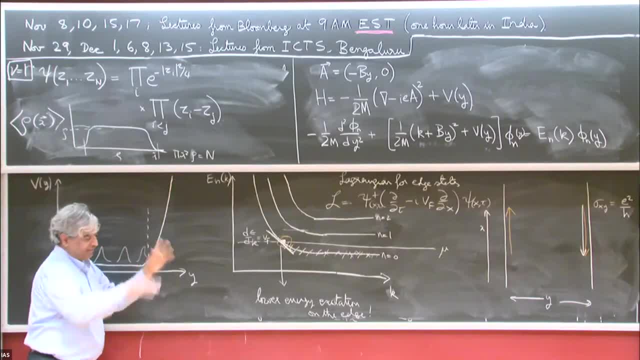 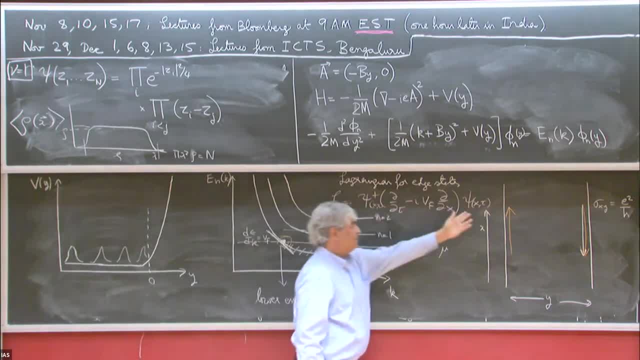 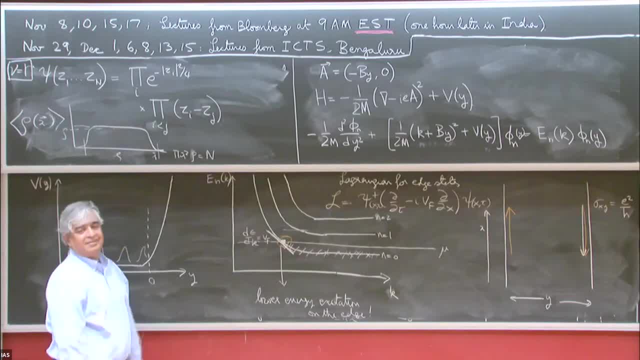 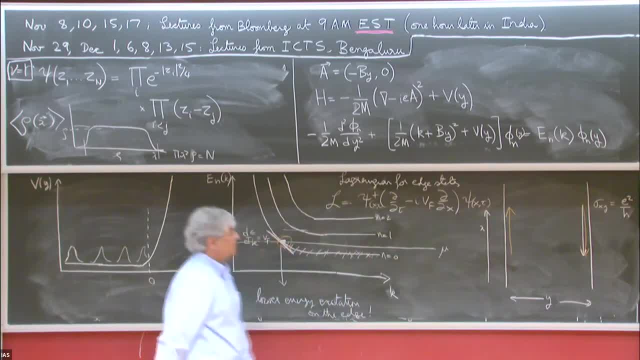 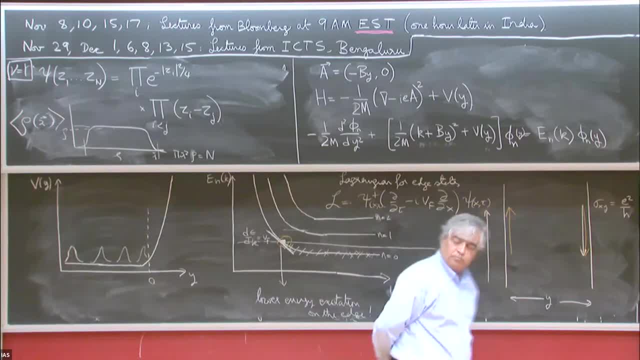 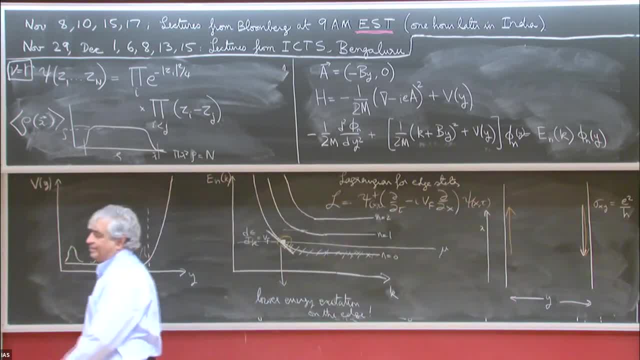 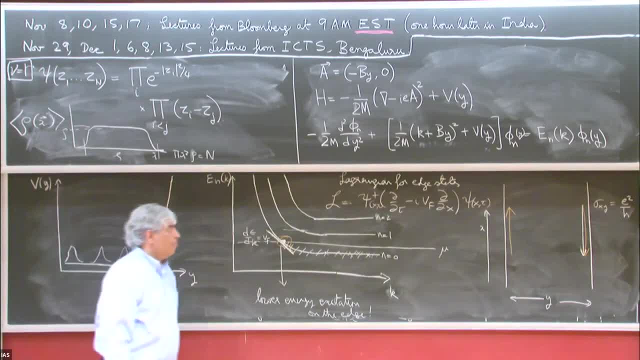 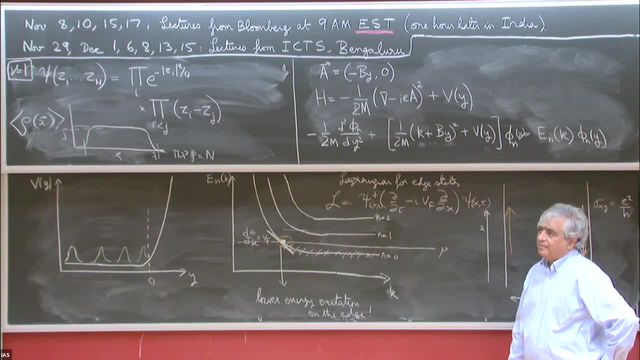 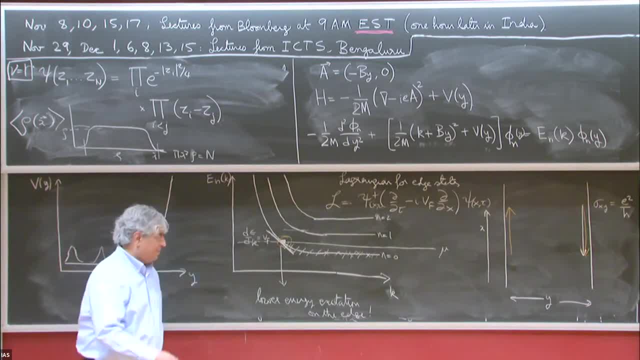 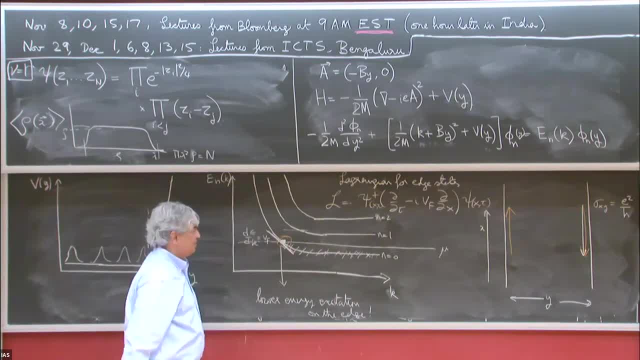 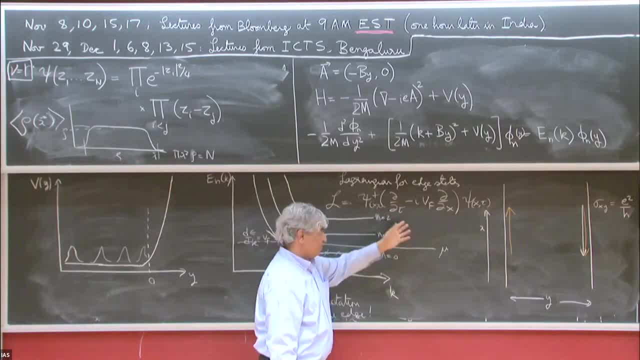 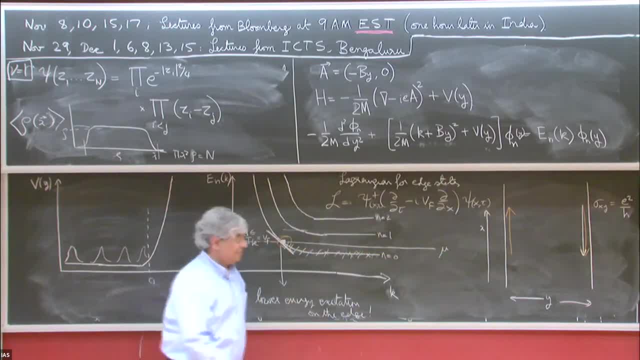 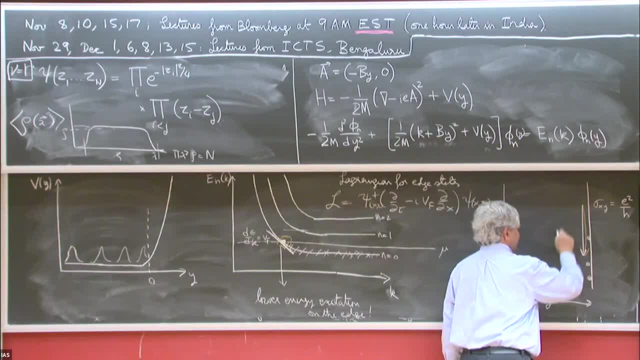 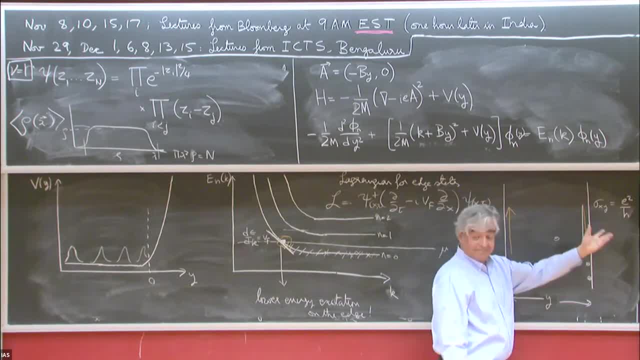 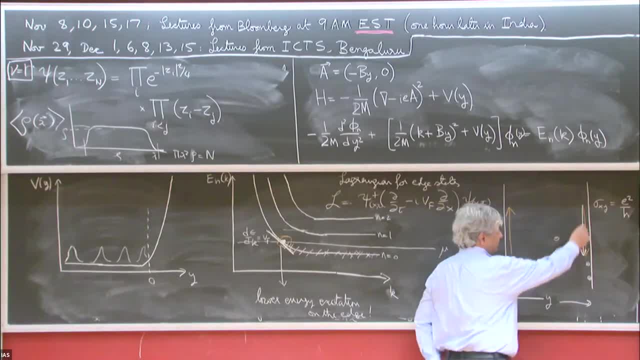 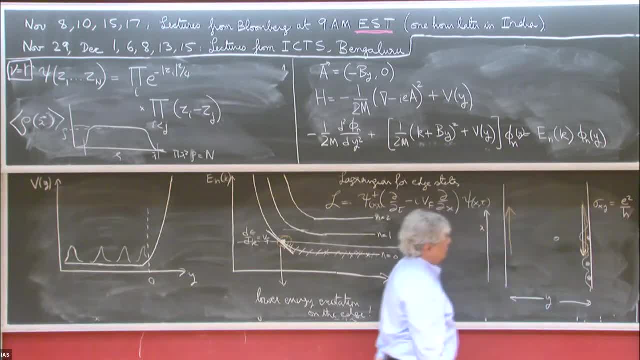 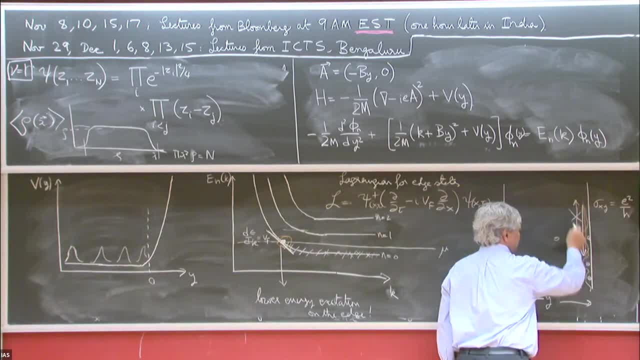 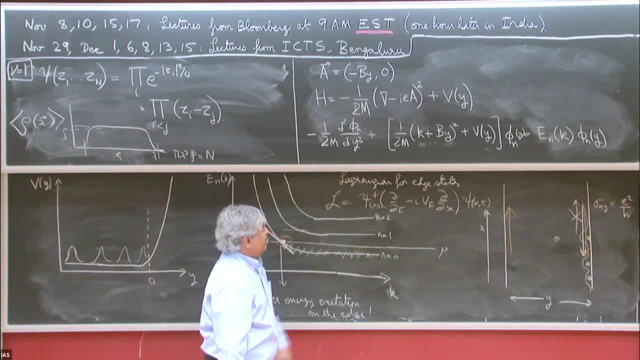 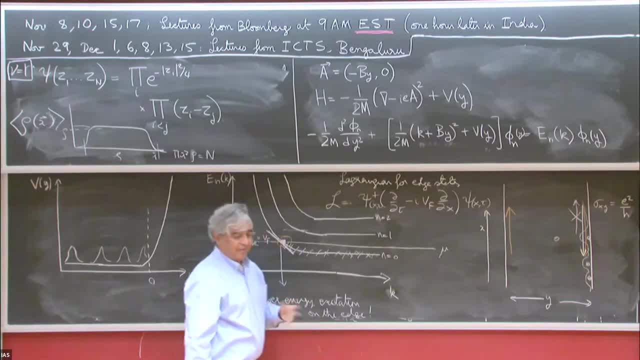 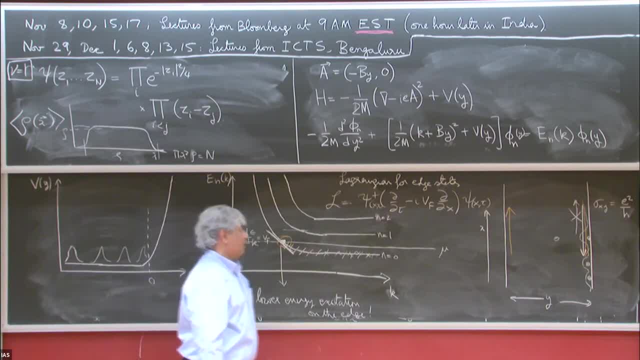 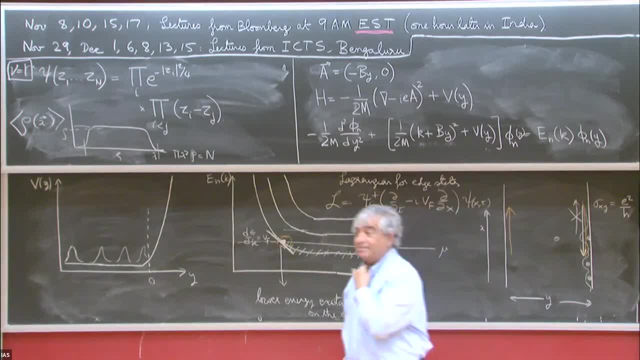 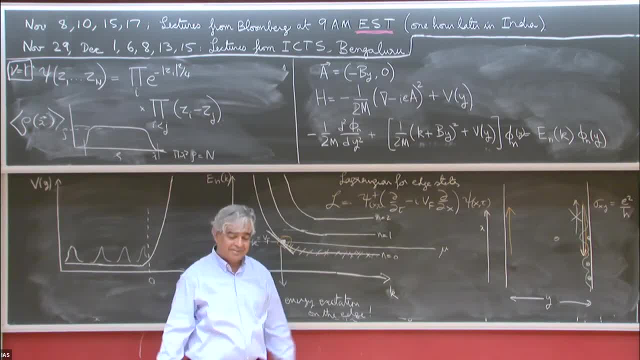 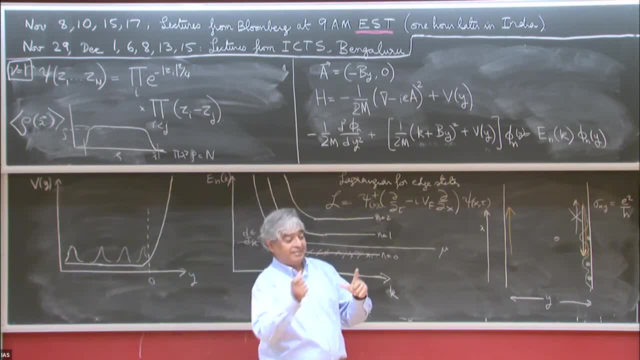 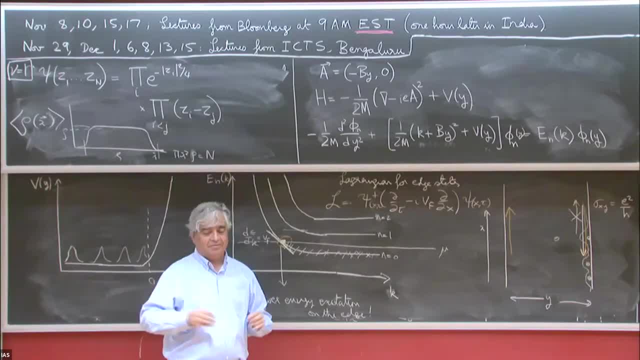 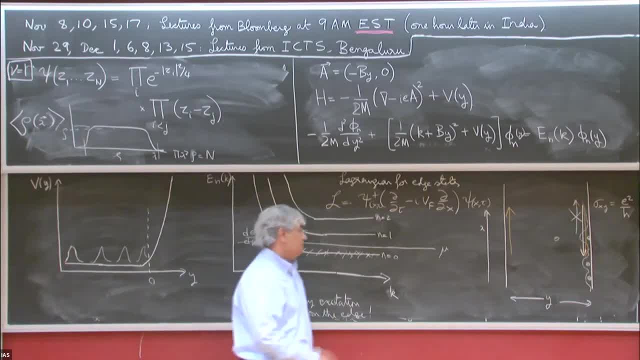 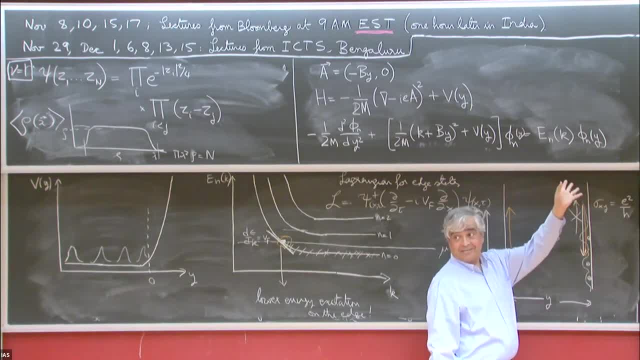 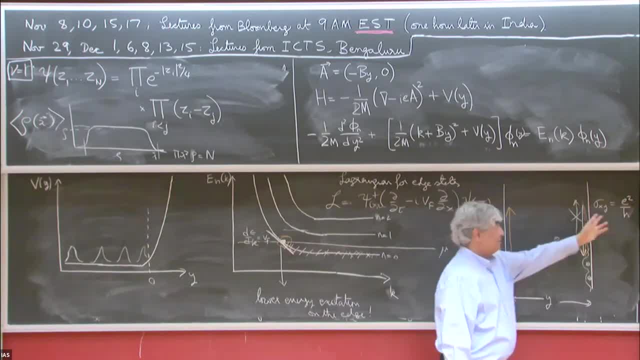 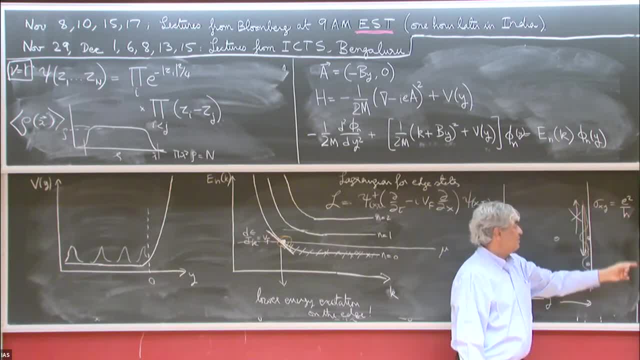 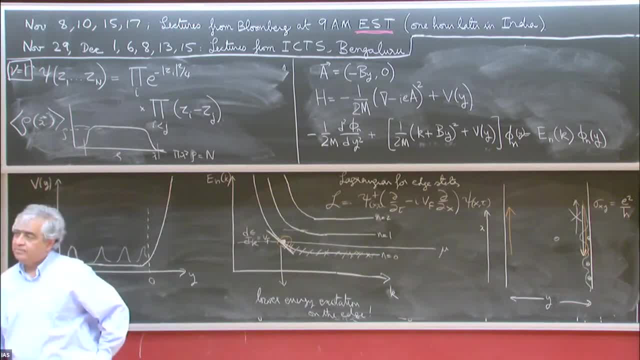 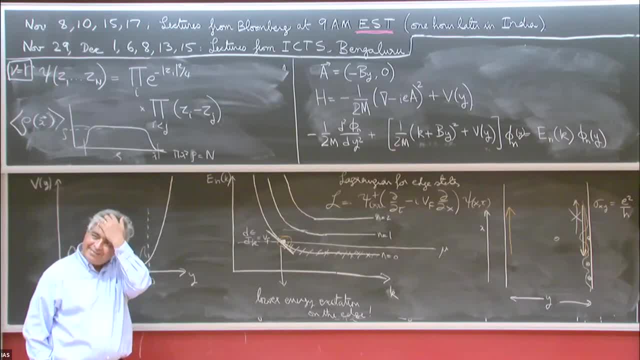 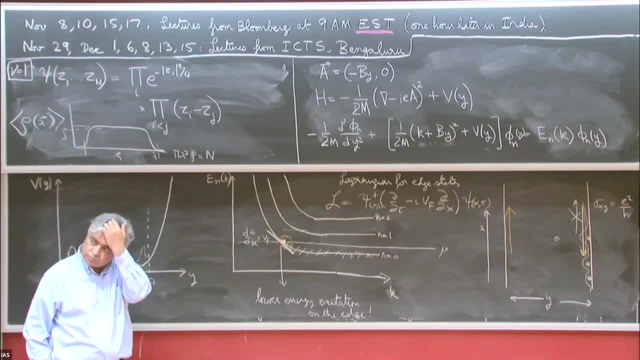 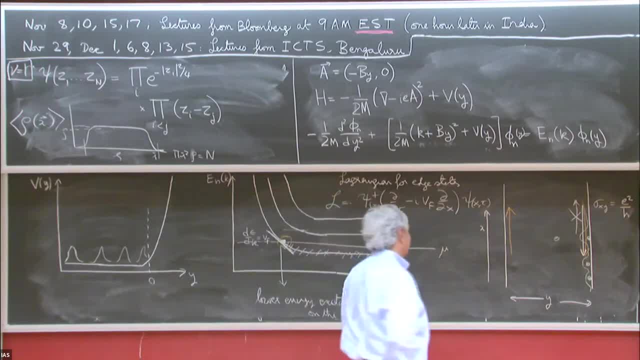 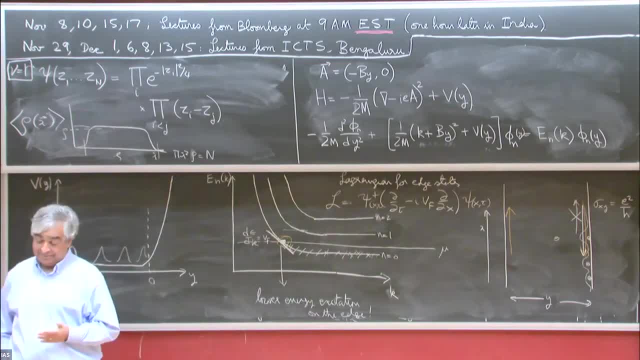 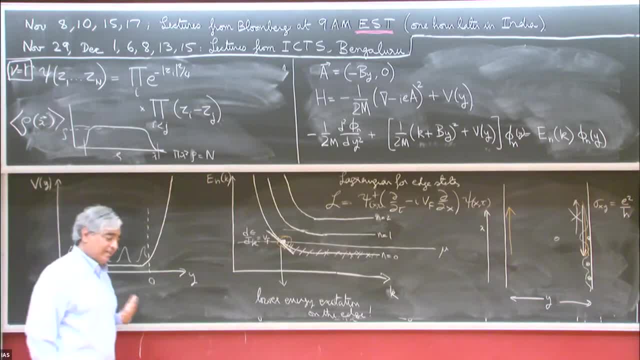 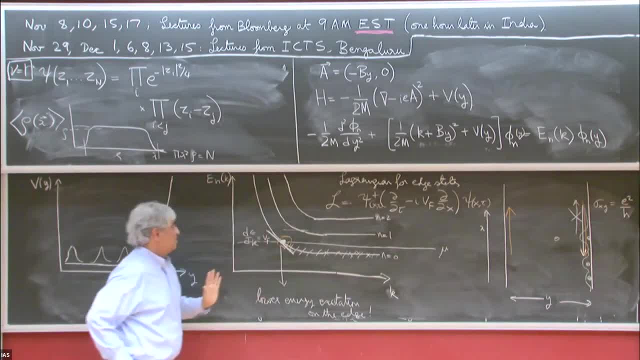 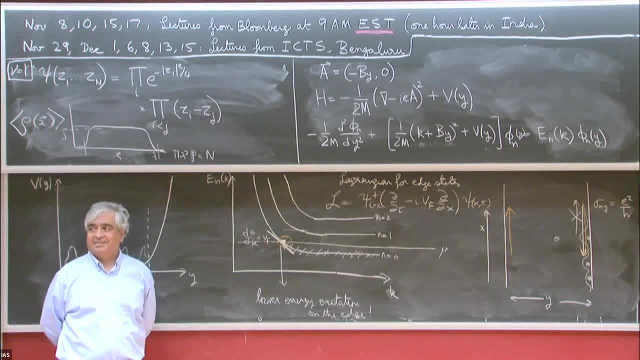 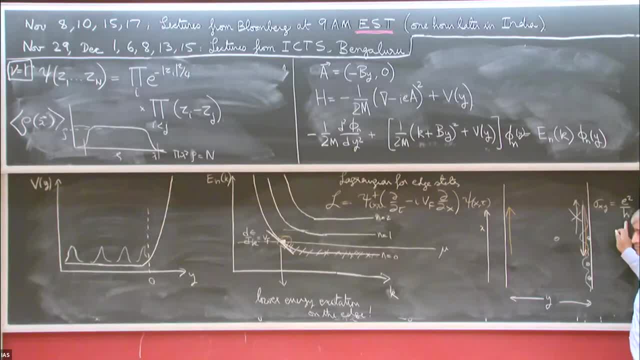 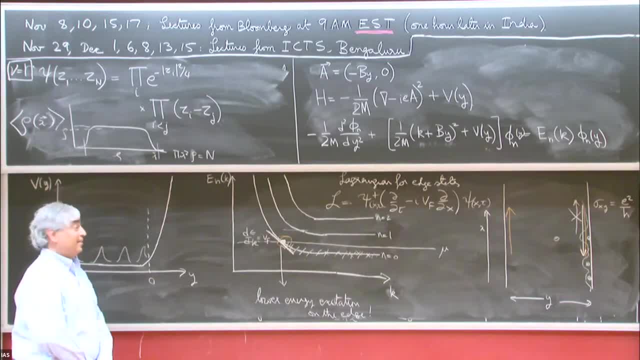 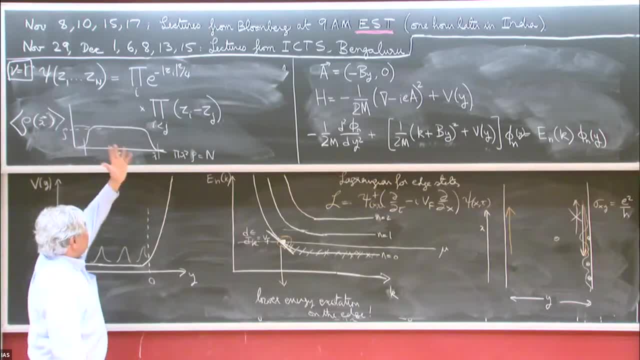 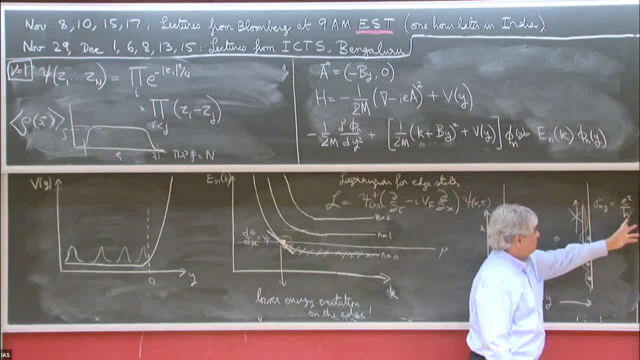 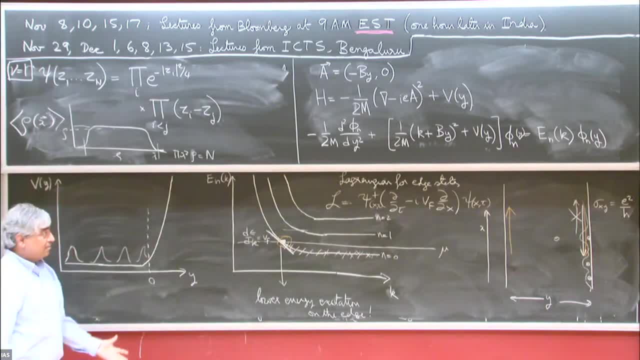 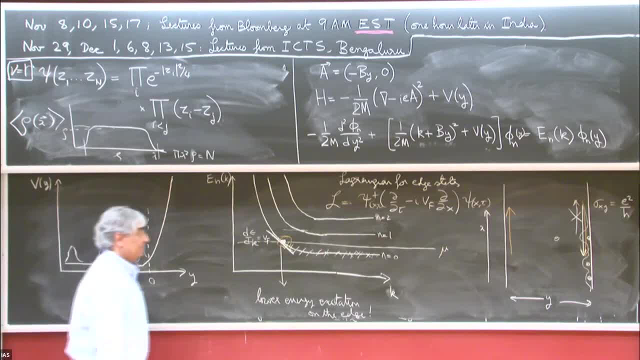 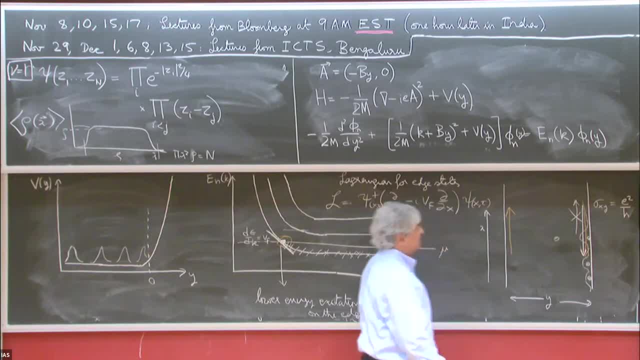 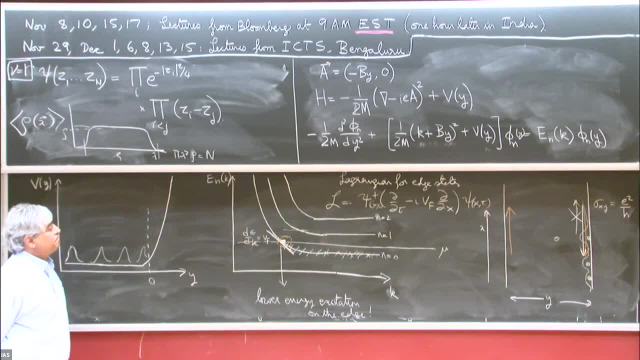 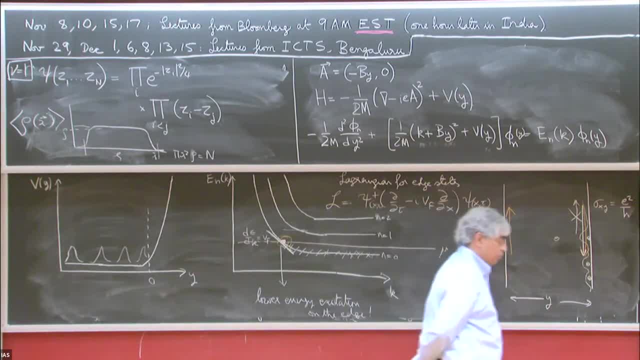 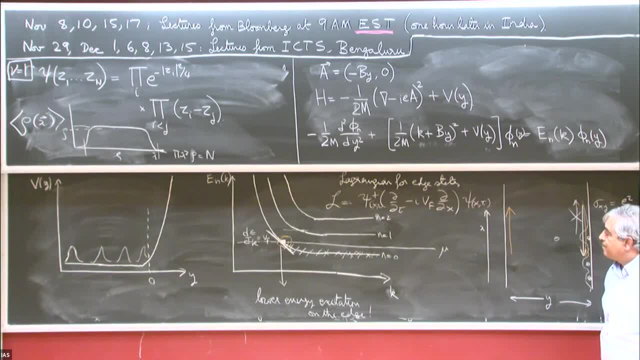 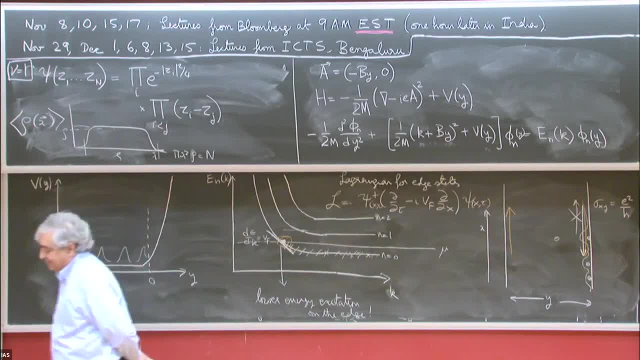 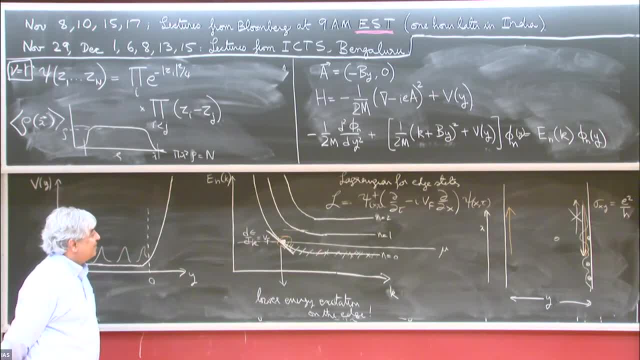 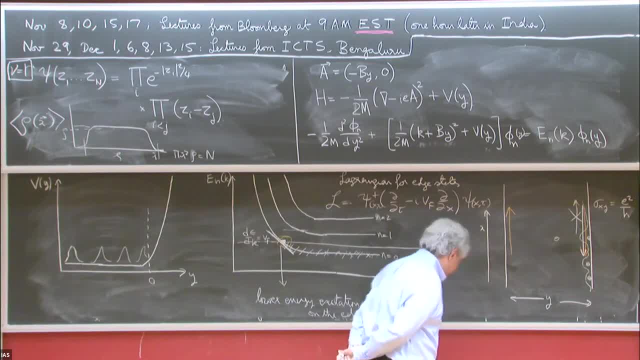 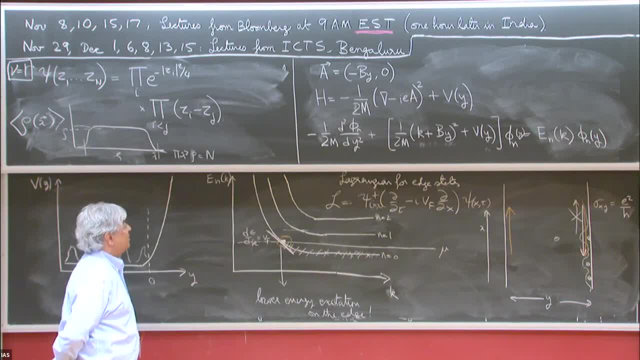 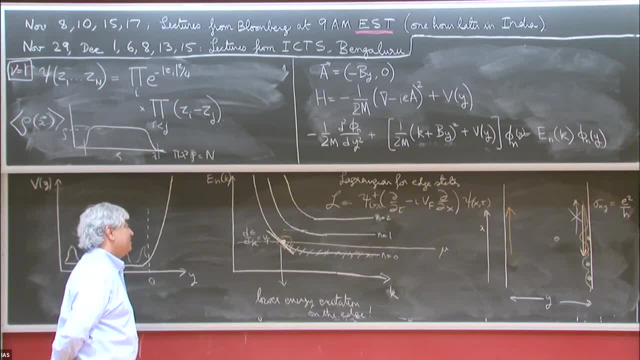 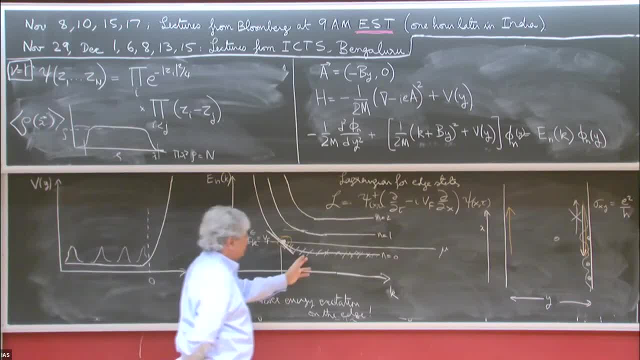 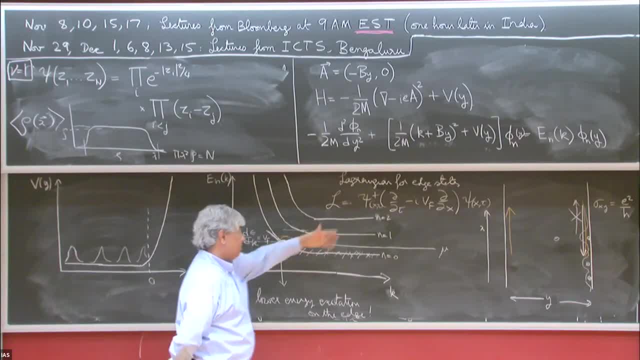 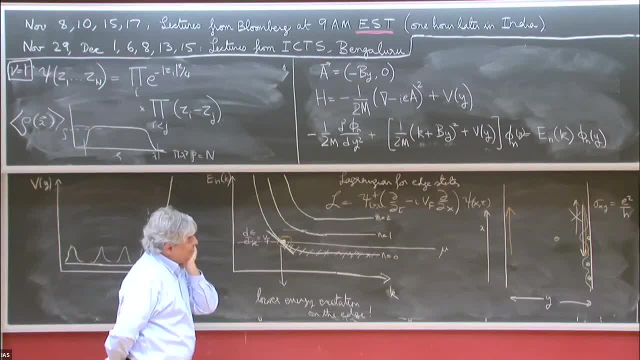 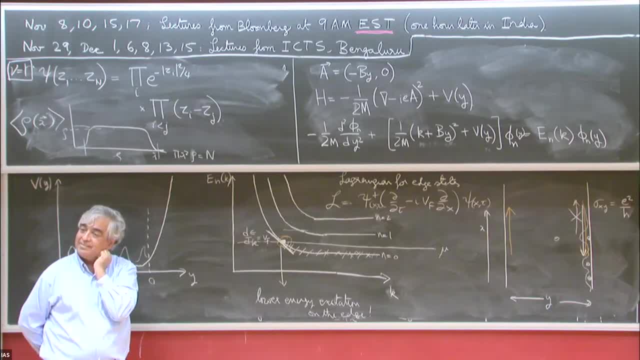 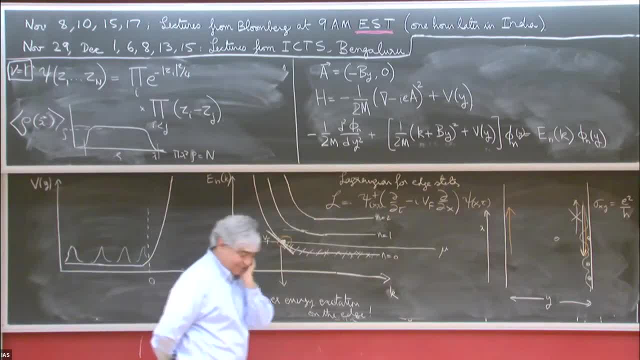 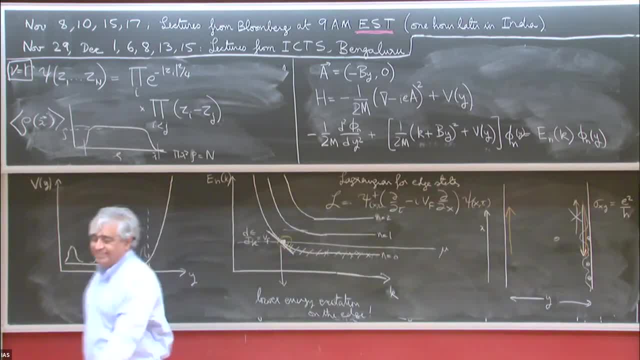 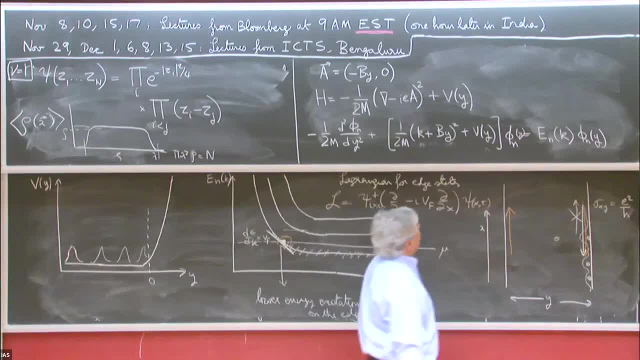 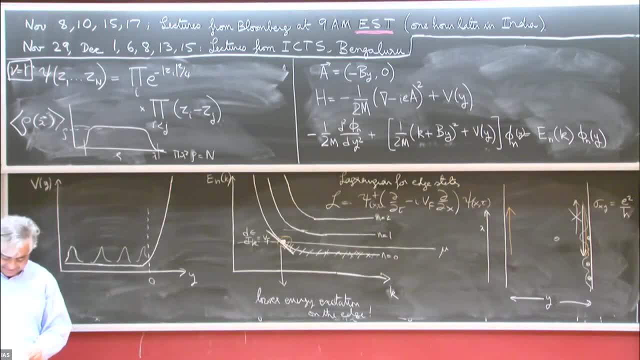 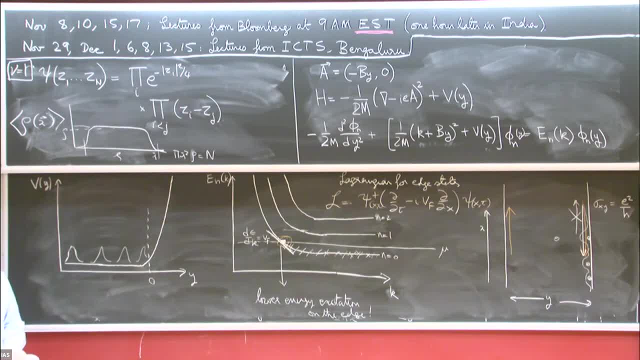 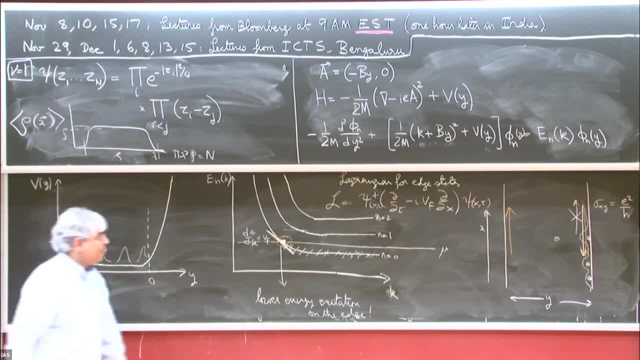 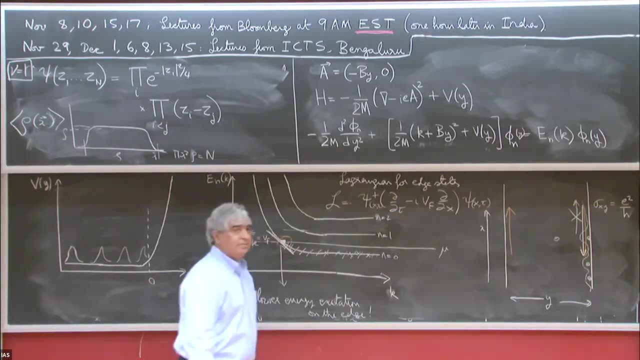 you can do that, but let's just look at some general features, so what this e n of k looks like. uh, uh, you know, is there a sense in which the current flows also in the bulk, or is it only, or is it always the case that it's only on the edge? 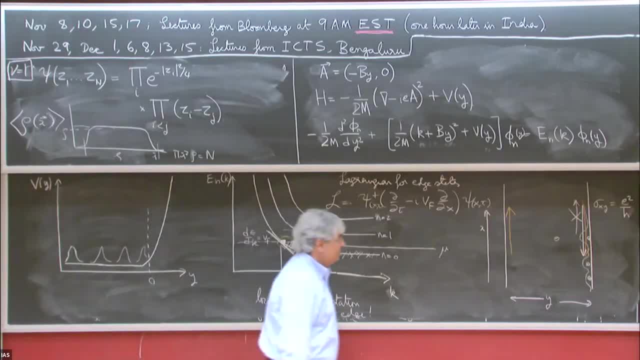 it's always on the edge. i mean you can measure the current. uh, you know, people can come in with there's is probes and see what the current is and you can see it's only on the edges. yeah, so there are states in the in the bulk that if you take any given state you'd see there's a current. but when? 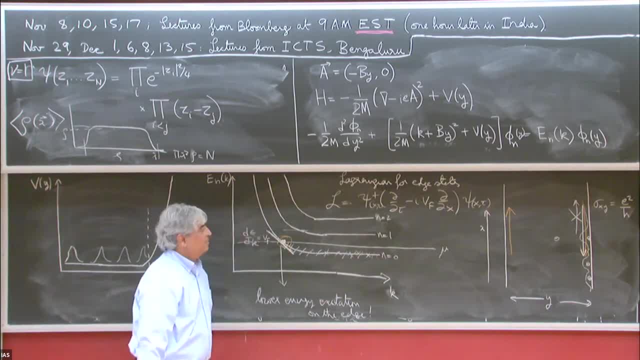 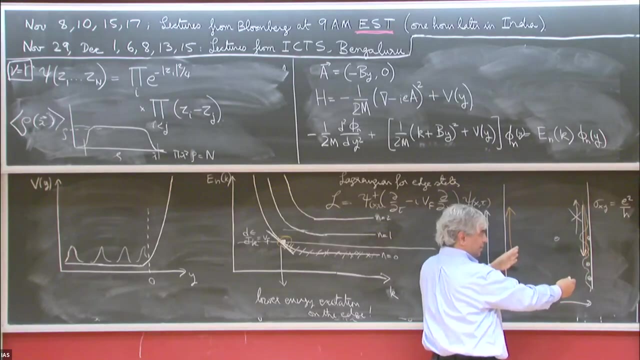 you sum over all of this occupied state, the net current is zero. I see, thank you so and in fact the whole conductivity is, you know, to drive a net current you have to have this, the current here if not exactly equal to the current there. so there's a difference and the net current that. 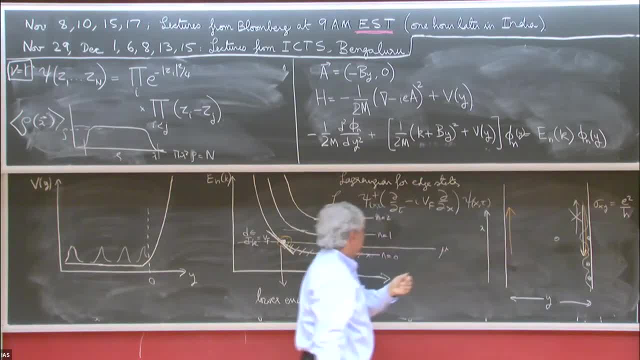 you will be driving. the sample is the difference of the left and right currents and from that, and using a few general arguments, you can then see why there's a whole voltage that will develop a character. so that's why the linear- in the end the linear conductance. 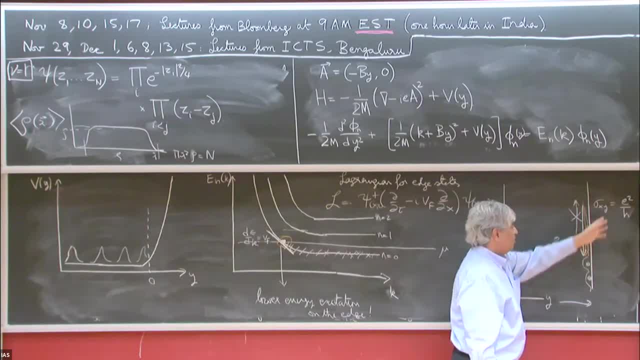 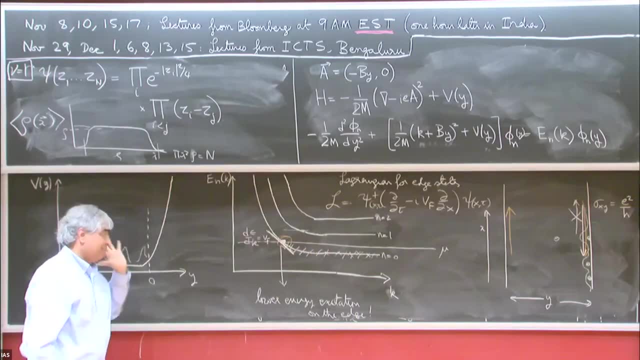 of this edge theory is, in fact, related to the hall conductance of the whole bar. so, yeah, there's a lot of interest on that, with the using the land of particular approach to all of this, and that's essentially exactly all you need for, for that is, you know, the, the various 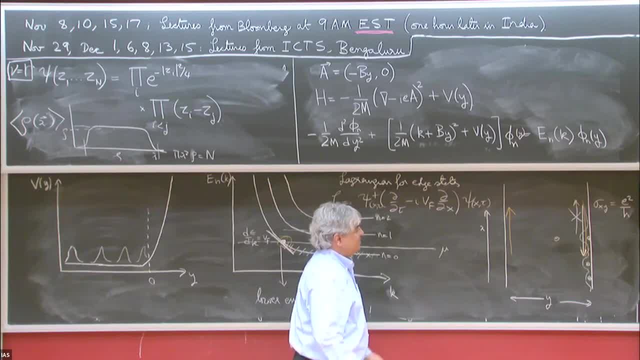 leads on your samples and at very low temperatures. the collision coefficients of all the edges. of course you can get, in some cases in fractions, quantum Hall states, very exotic edges. but you can get very exotic edges in some cases in fractions, quantum Hall states, very exotic edges which are non-trivial, conformable theories and yeah, so we'll get to those in a minute. 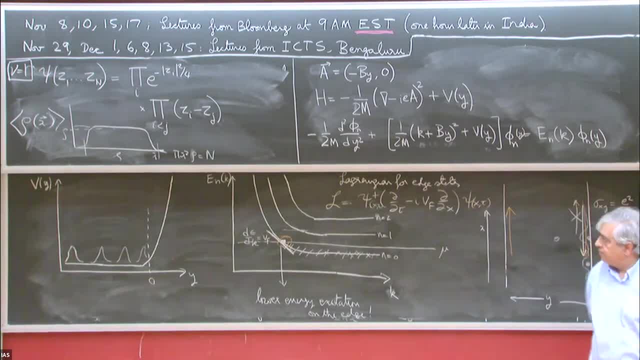 can you please say briefly what does one mean by an anomalous theory? or what does anomaly mean? i'm afraid i can't because i can't be breathing. but the more important reason, i'm not sure i understand it well enough to talk about this. maybe tom or nari want to attempt an answer to that. 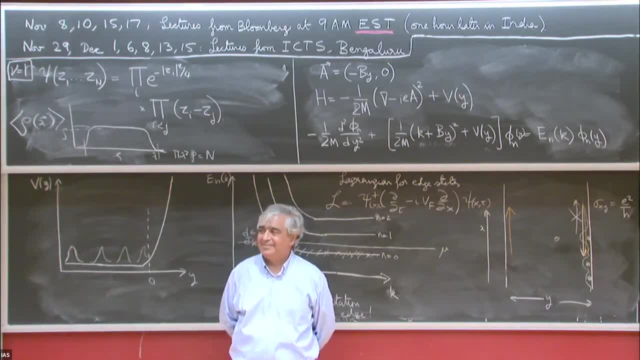 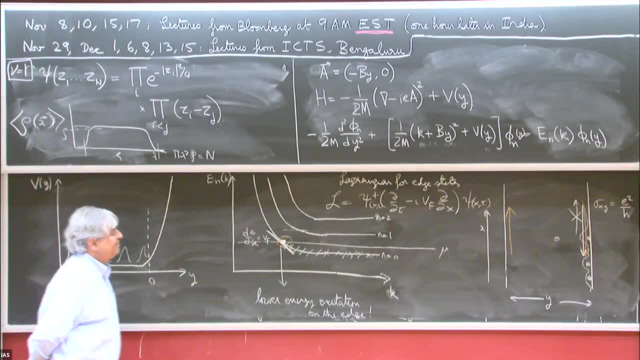 if you want to say something about that. yes, yes, in one word, if you just look at this Lagrangian that you wrote and you add the gauge field and you try to integrate out the fermions, this is just a determinant. it's straightforward to integrate it out, the result you get is not gauge variant. 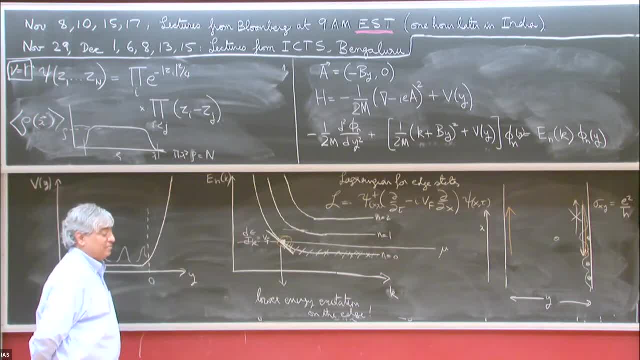 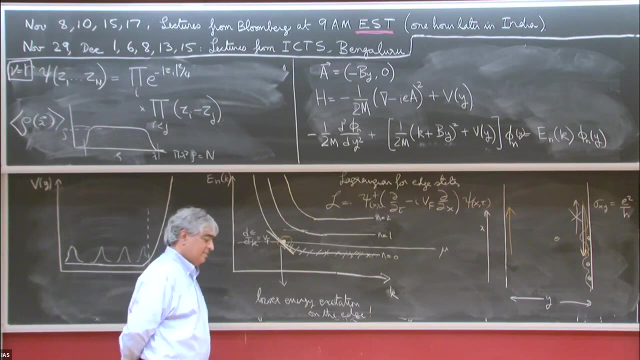 put an external gauge field, then the final theory will not be gauged in very respect to the external gauge field. Yeah, it's not an inconsistency in the theory. The theory is perfectly consistent. Okay, Yes, I do. I'm just going to suggest the following: Suppose you only have one edge: You apply an electric 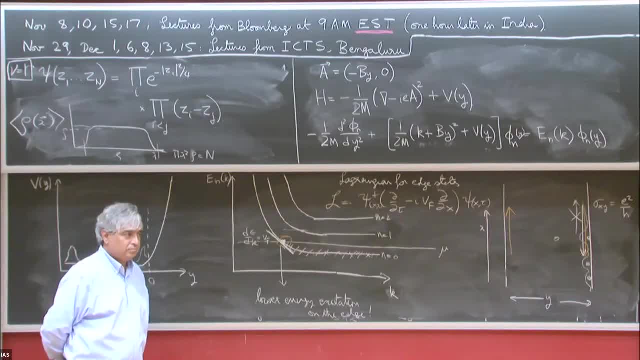 field which accelerates the electrons and makes the Fermi level go up, And if you have only this one band, it would change by that oxygen charge conservation. When the Fermi level goes up, the electron density goes up. Okay, All right. Okay, So I hope you could hear that. Okay, that's good, Thank you. 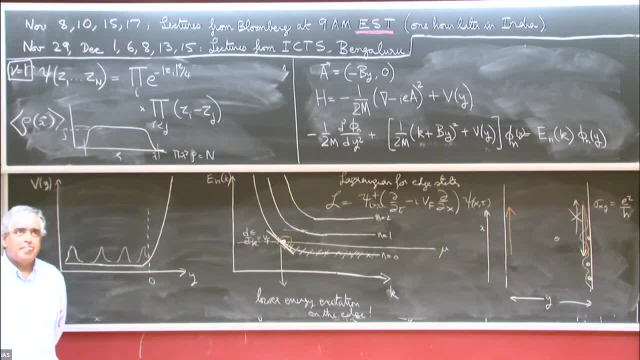 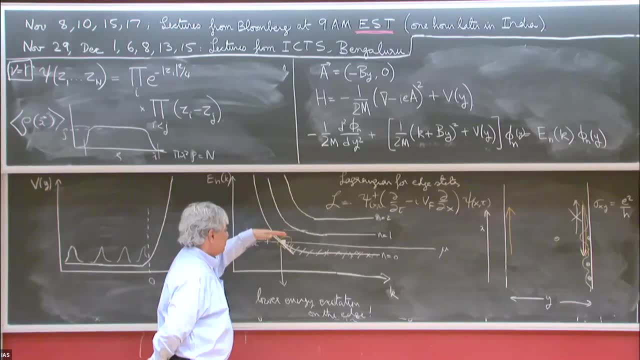 Actually I could not hear it well. So what Edward said was that if you apply an electric field, then the Fermi level will move up here over here And then therefore you get a net charge on the left edge. And the question is where that charge? 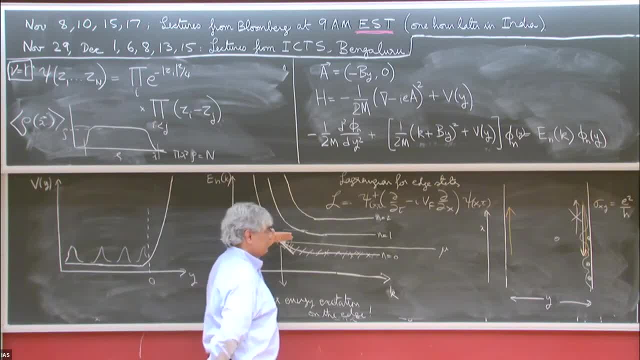 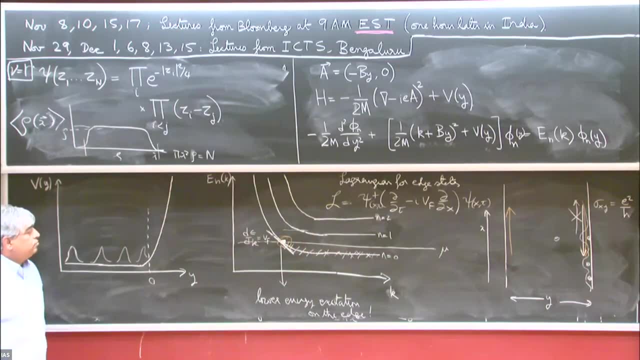 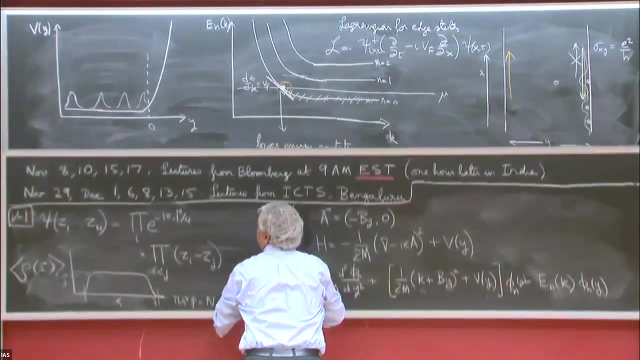 comes from. So you end up violating charge conservation. So the charge that you accumulate on one side has to come from the other side. Okay, Thank you. Okay, Right, So now let's just jump ahead to the fractions bottom half. Okay, 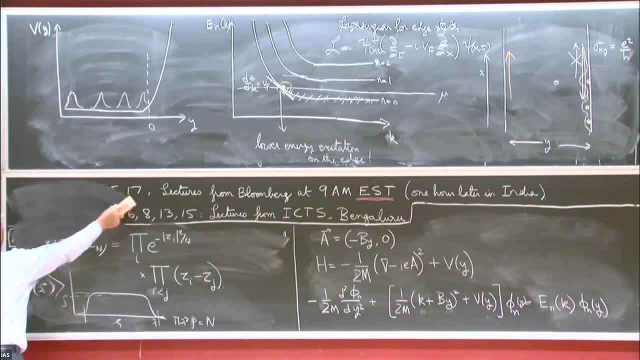 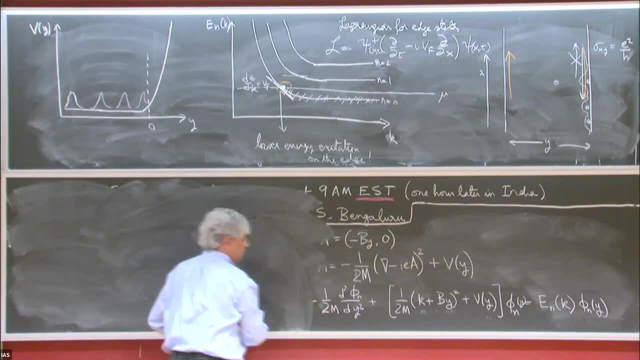 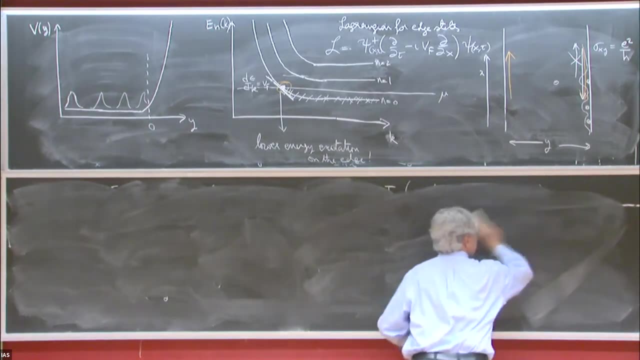 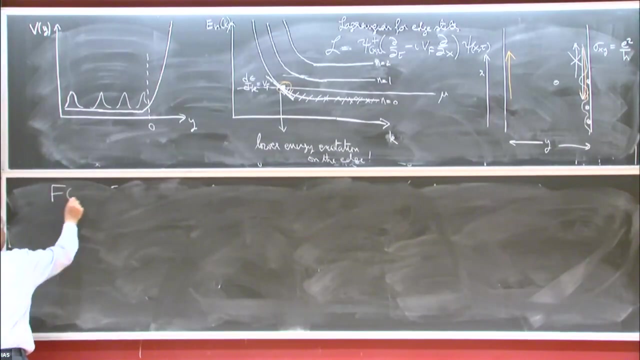 So I'm going to use the part-time approach. And this was this context you know, rather explicitly discussed by Jane very early on 1989, already around the time he wrote down the famous Jane states, which we'll also talk about. 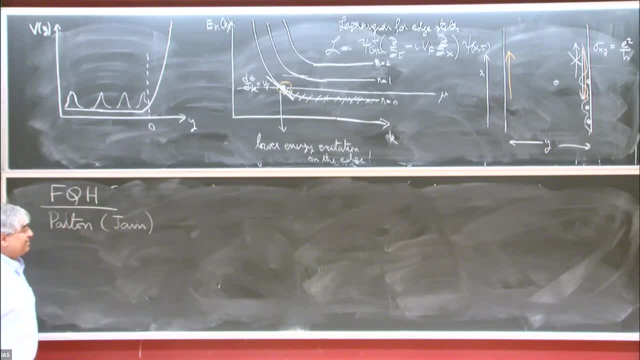 But strangely enough it hasn't been used much in the literature since then. With the benefit of hindsight, I think this is the cleanest way to do a lot of things. Much of the condensed matter literature uses flux, attachment, transformations and dualities, and they can be highly confusing and often are not entirely correct. 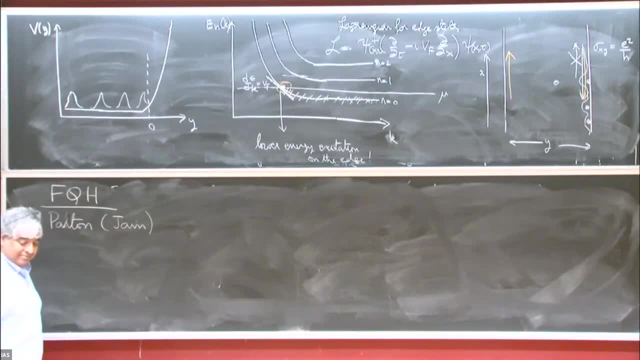 But this one, at least formally, at every stage, is well defined And it does actually give you a very compact description of the important quantum all states, particularly most of the ones that have been observed, So let me just discuss it. So what we're going to do, we're going to take our electron operator, which I'll call C and no spin here. 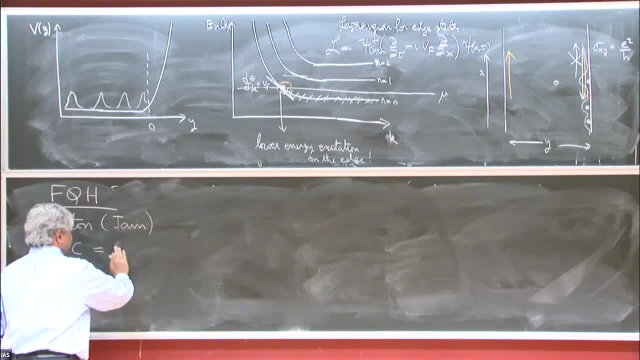 And I'm going to decompose it. And I'm going to decompose it into three fermions- That's hardly the partons- which are called Psi 1,, Psi 2, and Psi 3.. So you can imagine putting this on a lattice. 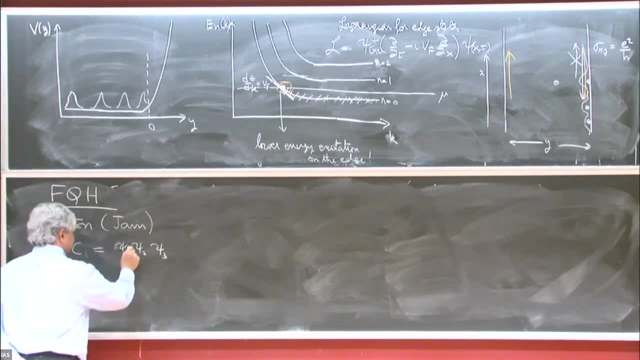 So you can put a site index if you want. Eventually I'll just work in the continuum And this is just a very simple thing. on each side of the lattice I have two states: I have the empty state And I have the filled state with one electron in it. 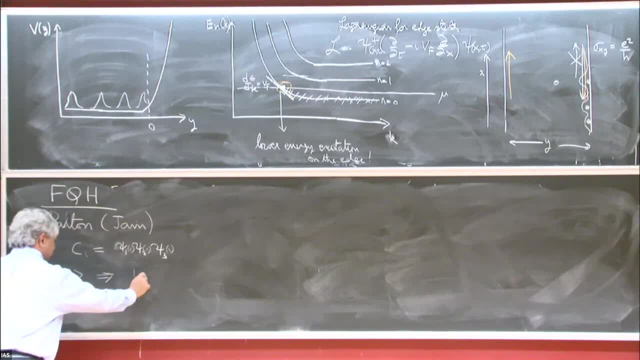 And that I'm going to just equate here also with the empty state. And this state I'm going to equate with Psi 1 dagger, Psi 2 dagger, Psi 3 dagger. So if you really had three partons, then they're independent. 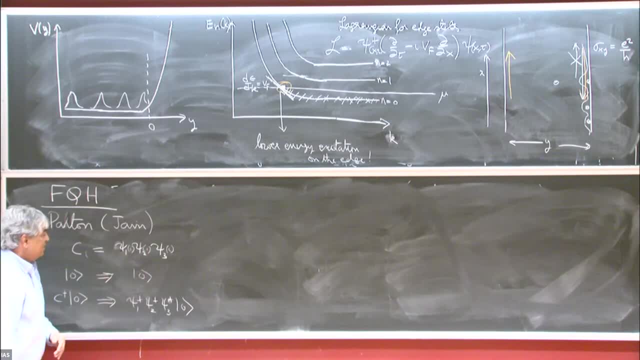 So I'm going to take the total number of states in my Hilbert space of eight on each side. I'm going to declare all the other states to be illegal and demand that these are the only two legal states. So it's sort of like a repetition code. 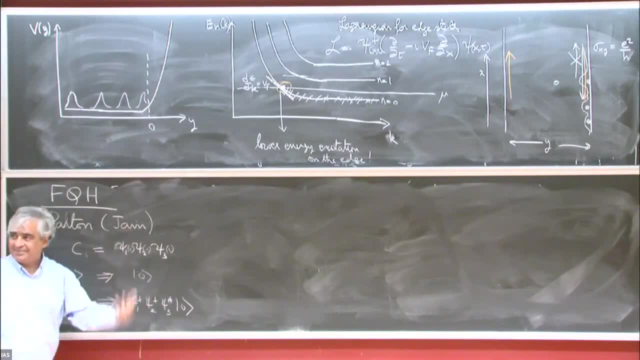 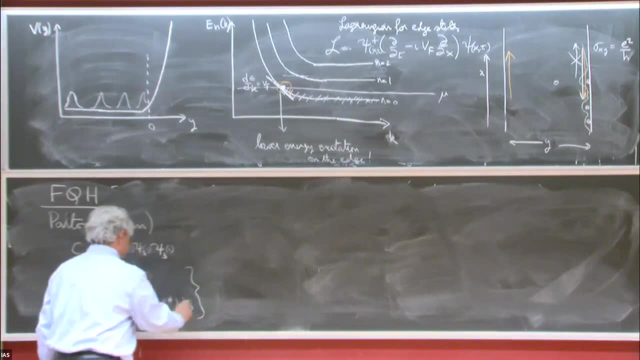 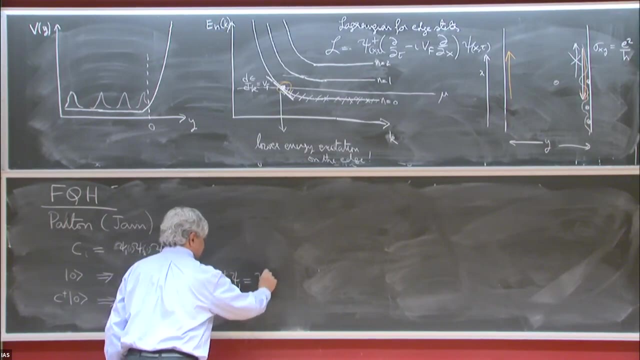 You're representing one by one, one one, That's all. And all of the states are not allowed. So if you want to get these two states only, then you have a constraint. And the constraint is very simple: Psi dagger 1, Psi 1 equals Psi dagger 2, Psi 2 equals Psi dagger 3, Psi 3.. 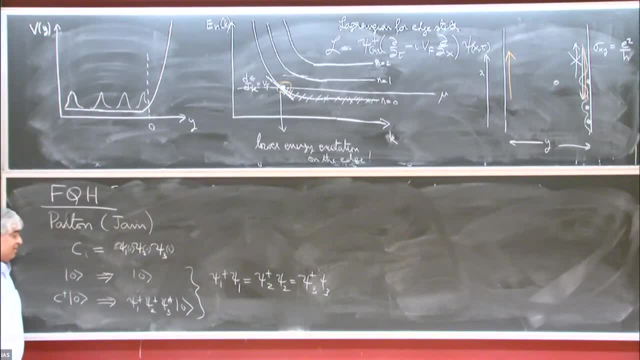 So if I impose these constraints exactly, then I will exactly restrict my eight states in the Hilbert space of the three partons to these two states. These are the only two states that satisfy both constraints, So I only need to impose two constraints. 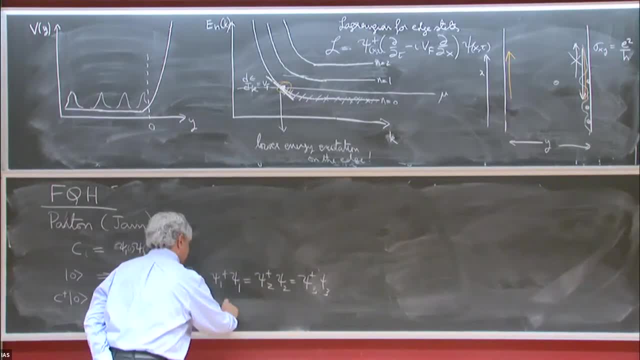 There are also other constraints which are implied by these. For example, like Psi 1, Psi 2 equals 0.. Or Psi dagger 1, Psi 2.. So these are implied by these, But you may want to impose them explicitly. 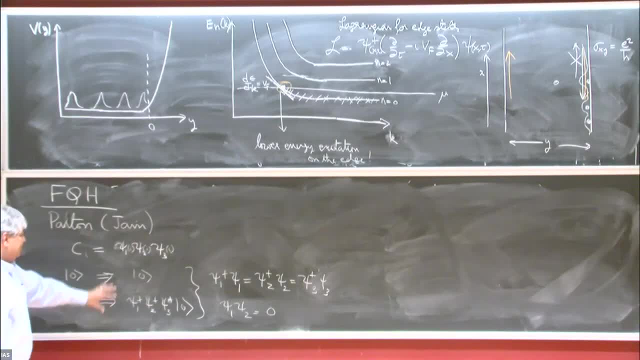 In particular. you can see that there's a certain SU symmetry here, And if you want to make everything SU invariant, then you'll probably want to impose those constraints too as you go along. We're not going to bother with that, because just imposing these two constraints is sufficient. 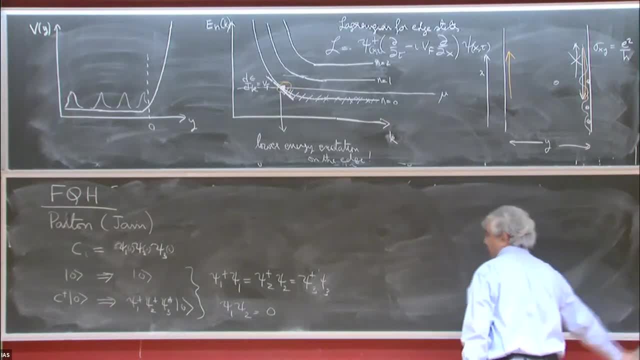 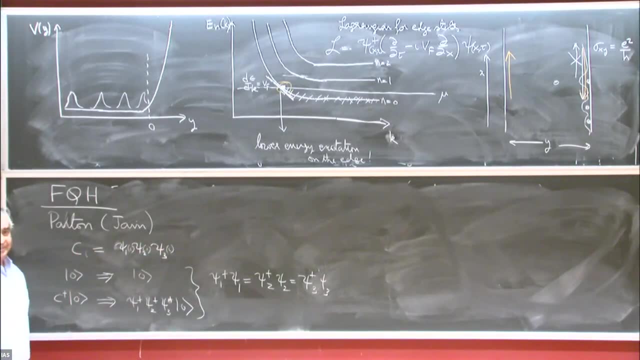 And so let's just stick to that And we're going to only work with the U gauge field that we might expect, rather than SU gauge fields. But if you insist, you could work with SU gauge fields And then you can get even more exotic states. 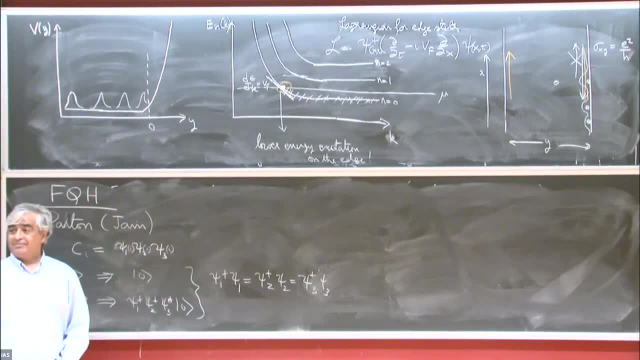 That would be important for certain non-obligation states, if you care about them, But at this point let's just stick to the? U. So now, the point, of course, here is that if you have this constraint, then you have a gauge field. 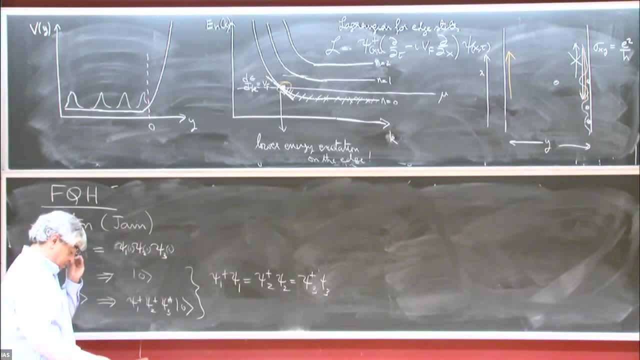 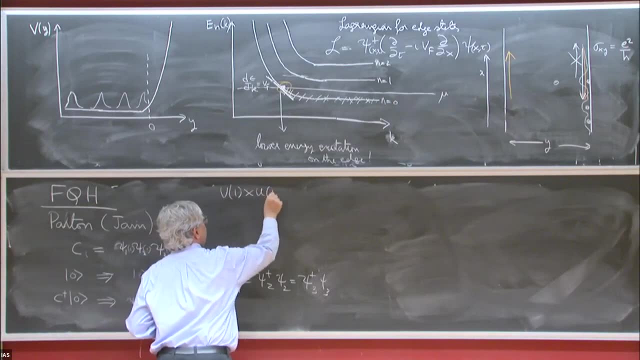 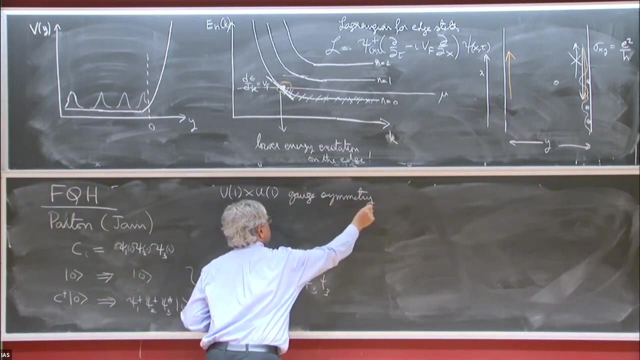 You have a gauge symmetry, Just like we had for the spins. So I now have two U gauge symmetry, U1 cross, U1 gauge symmetry, Which I will take to be Psi 1 goes to U, Psi 1. And Psi 2 goes to P2.. 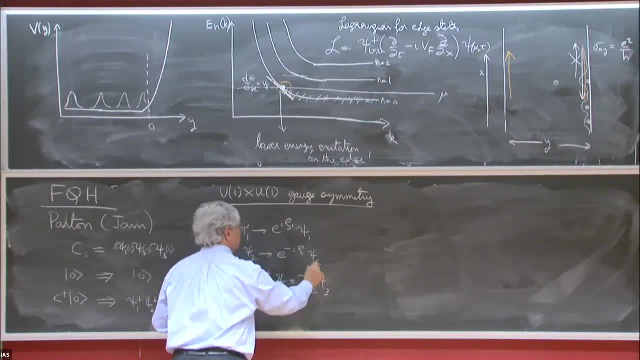 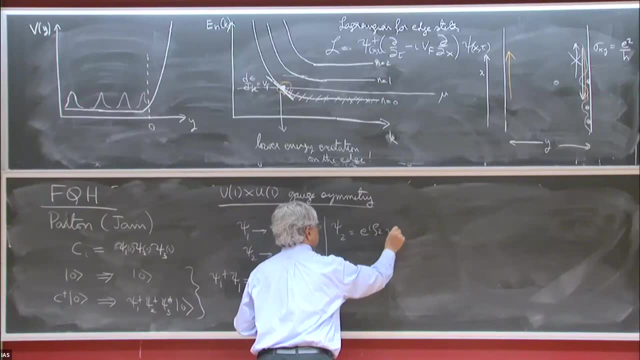 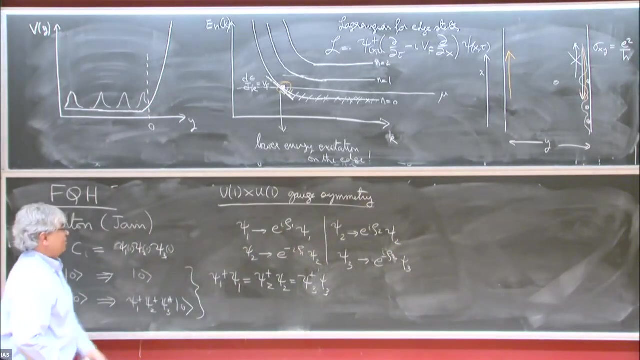 Minus I01 by 2. That's Psi 1. And the other one, And here will be Psi 3.. Oops, Okay. Well, if I could just assign Psi 1 to have a positive charge in the first gauge field. 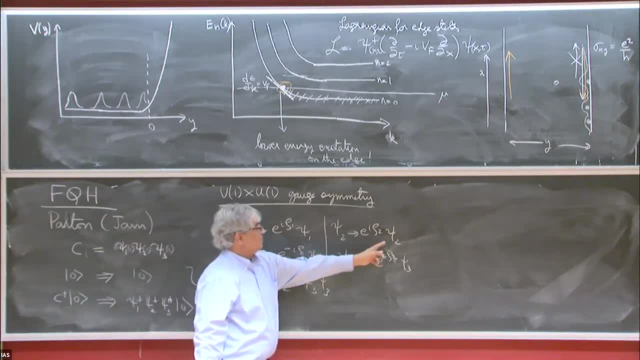 Then Psi 2 will have a negative charge And we'll get Psi 2 positive charge in the first gauge field And Psi 3 would have a negative charge. Of course, there's many ways of choosing it. Okay, There's one way. 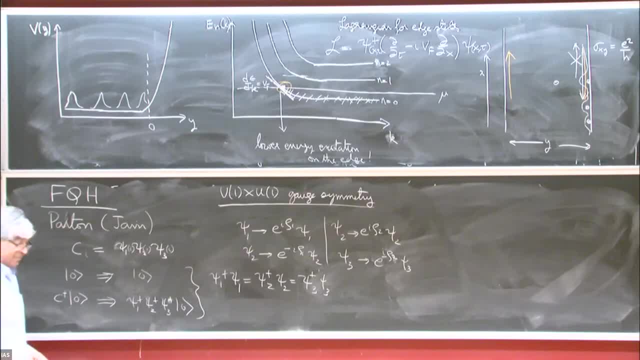 All right. So now, what you should really do- This is what we did for the spin system. Is you want to take this ansatz? Put it into your actual Lagrangian Or Hamiltonian For your threshold point of all states. 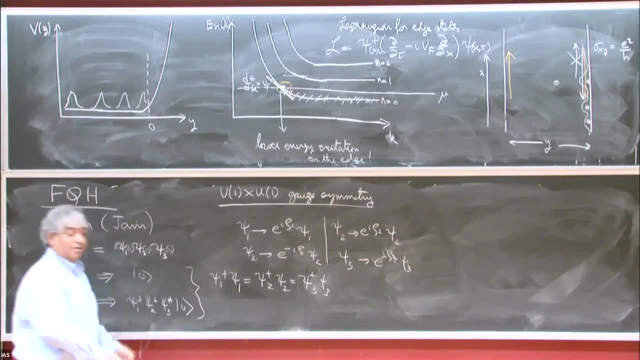 Or whatever, And then you'll get you know very complicated terms Like C, dagger C will become a 6 fermion term. Previously, the spin dot spin became a 4 fermion term. Here this is even more complicated: It's 6.. 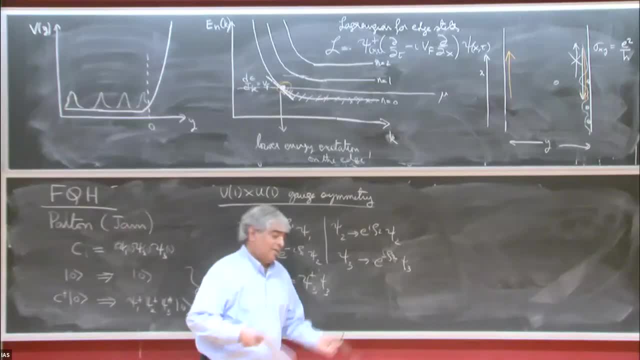 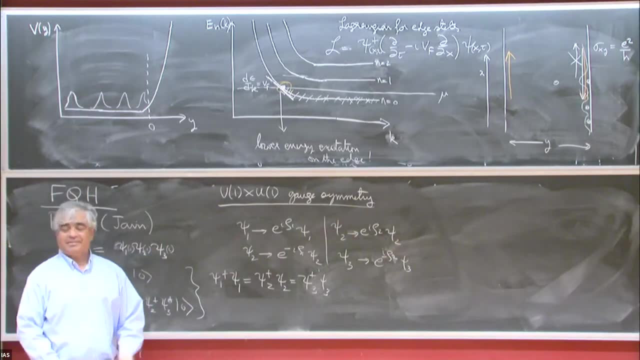 So you get some very complicated Lagrangian And then you imagine that you have some saddle point At which these gauge fields are not fluctuating too strongly. So you take some mean field saddle point And then you do all kinds of How about you're trying to wish decouplings? 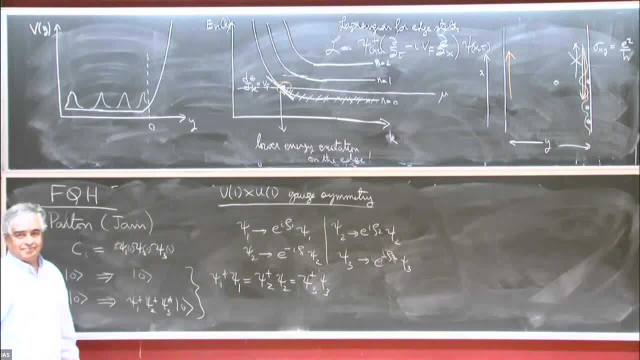 To write down a simple theory for the partons in the background of the saddle. Now, all of those steps We laboriously went through with the Z2 spin liquid anyways, And maybe partially for the chiral spin liquid. But hopefully you're all. 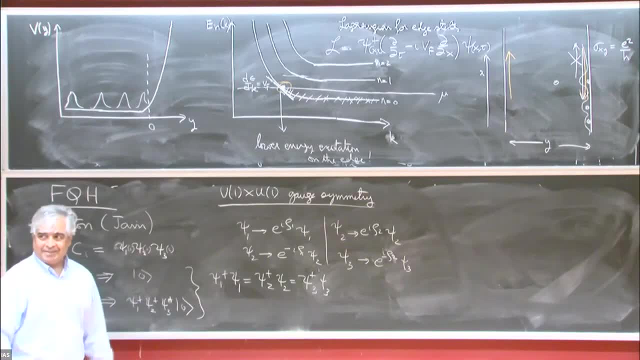 Exposited by now, And so we'll just skip all the steps And just write down What the general structure of the effect of Lagrangian should be, Just from gazing there. Okay, So in this case we are assuming that everything is. 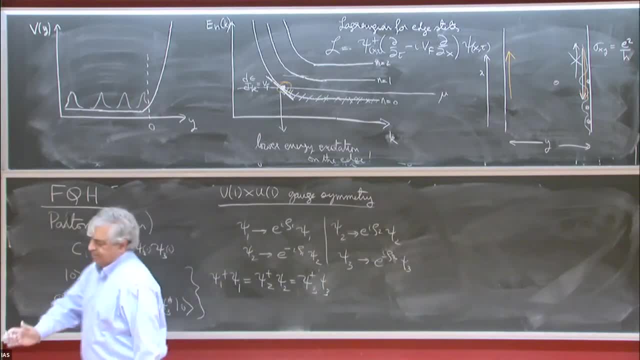 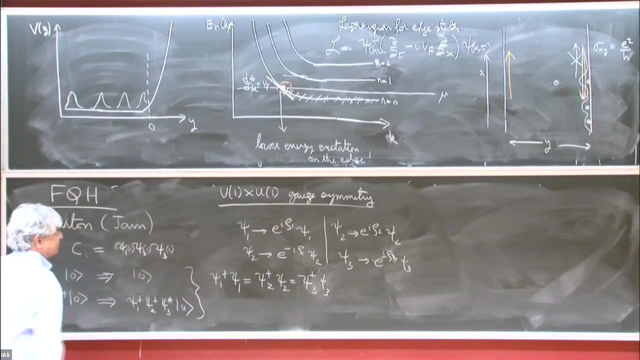 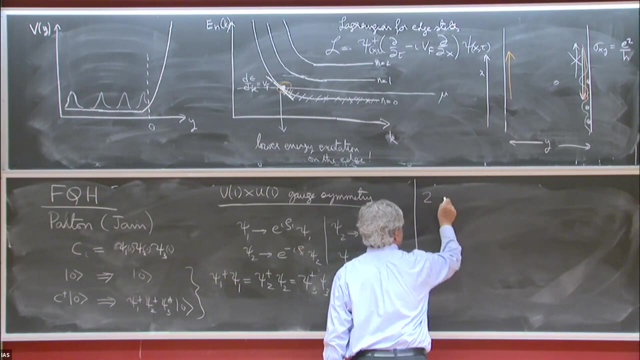 If you make this rigorous, you probably want a lattice. Well, let's assume everything is happening on a much longer scale. Everything is longer than on the lattice scale You used to define these states. So what would the theory look like? So I will have two gauge fields. 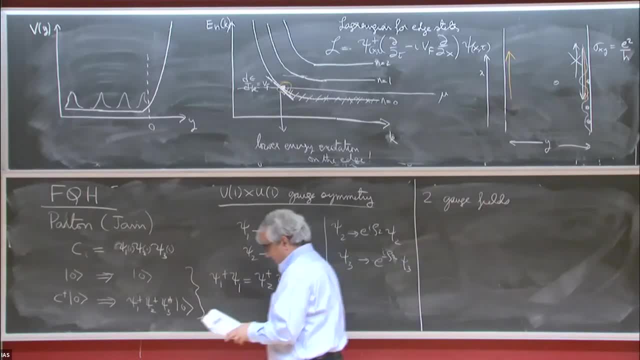 Sorry, Let me see. I'll use it in a minute. What did I call that? Oh, that's B, All right, Sorry. So I have two gauge fields, B1 and B2.. That's unfortunate notation, But small B will refer to gauge fields. 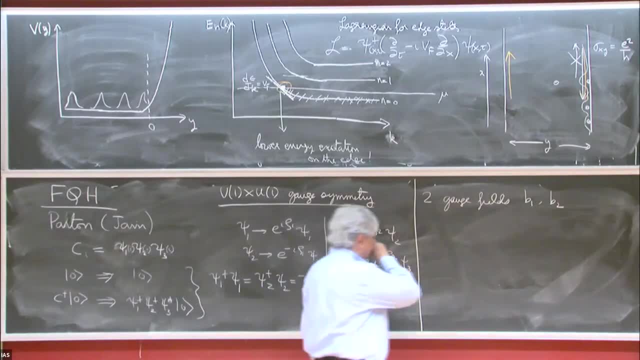 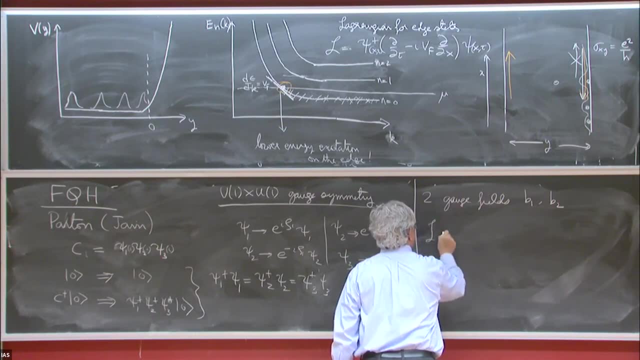 And big B will refer to magnetic fields. Okay, So what would the theory look like? So you would have, Let me, You know, Let me try to The spatial terms, The most important one. So we'll have B dagger. 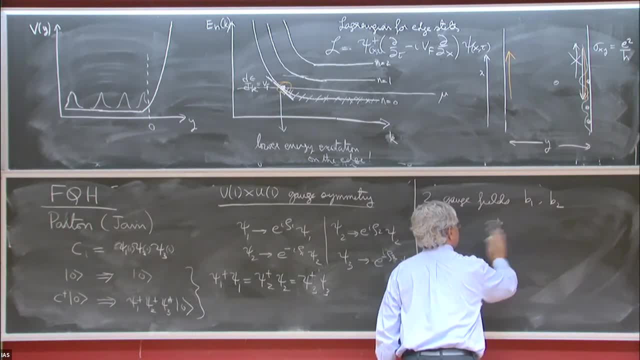 One, Oh sorry One, Over some coefficient Rad. Minus One has a charge, So minus IB one, And let's put the external field To act fully on On site One. So let's put the external field. 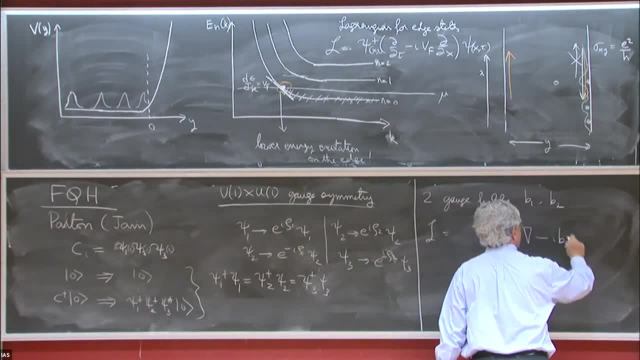 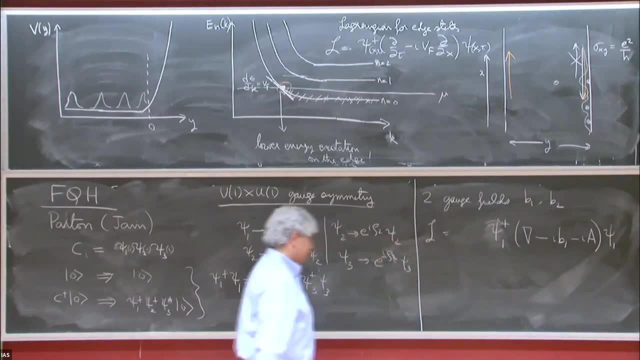 On To act fully on On site One. So let's put the external field On On site One. It's up to you Where it acts, But let's put it on site One, And then I'll have. 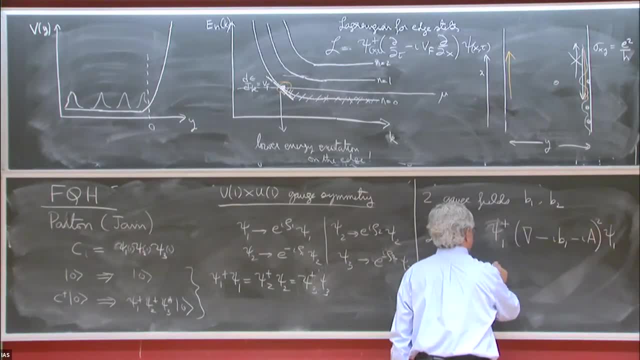 Side Diagon Two Of Rad Plus I B1.. Minus IB Two Side Two And I'll have Side Diagon Three Rad Minus IB Three B2.. 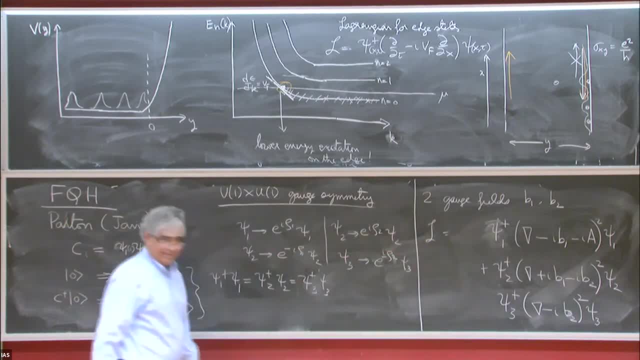 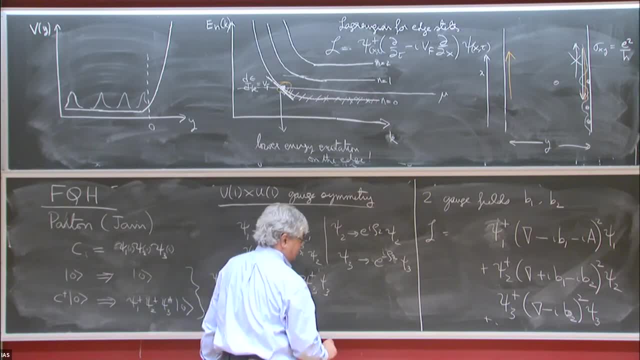 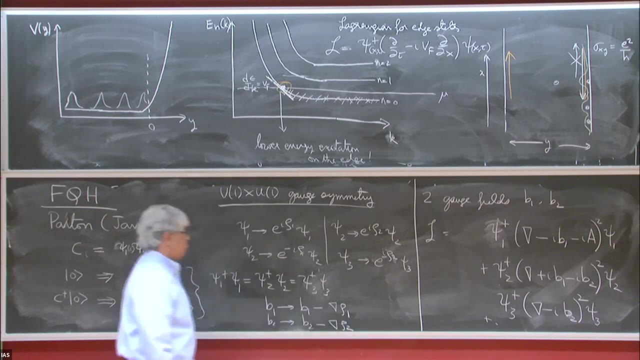 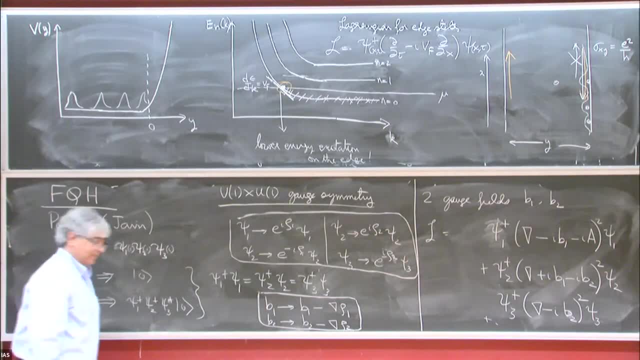 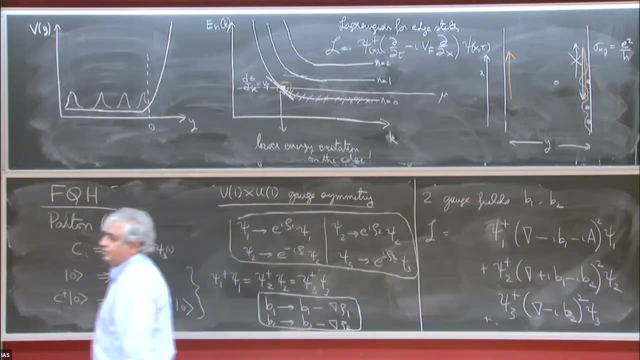 and you just write down all possible terms consistent with these gauge transformations. So, Subir, what you're saying is: no matter how I distribute the real charge among those three sides, you think we absorb it into the B field, Correct? You can redefine your V1 and V2. 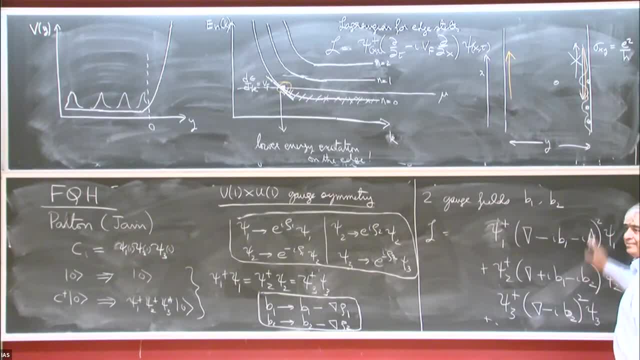 so that you can put the charge in where you want. So I just chose to put it there. I don't want to take fractions. Well, because these are compact gauge fields. in some cases that's important. So you don't want to put factors of two. 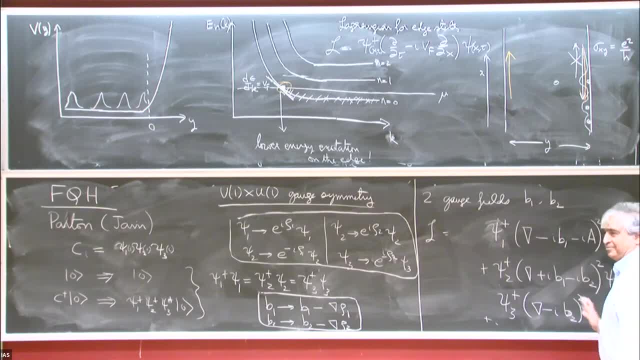 But with the external gauge field you could take fractions, but even that's a little uncomfortable. So if you You don't want to put a over three, a over three, a over three, and you have to keep track of the flux point. 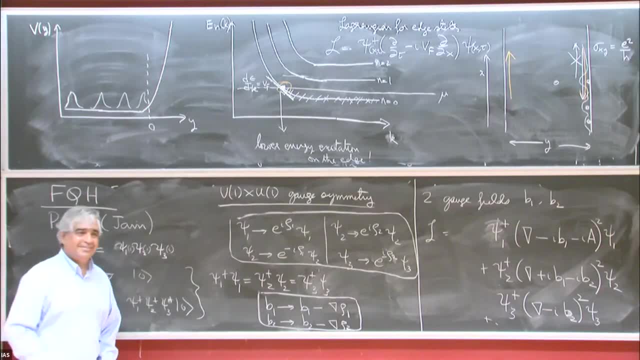 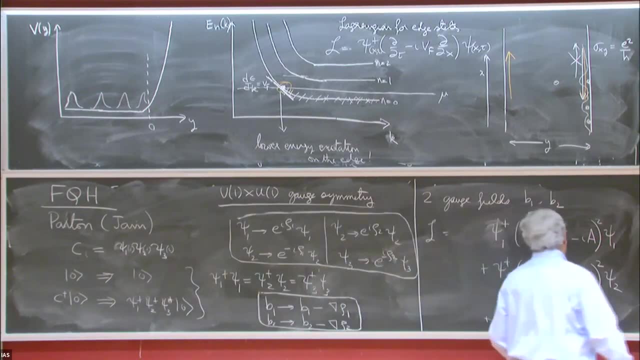 that's become the more careful, The better. to put it in one place: Okay, All right, so this is our theory, or this is just a general theory of electrons in any dimension? So far I haven't made any particular specialization. 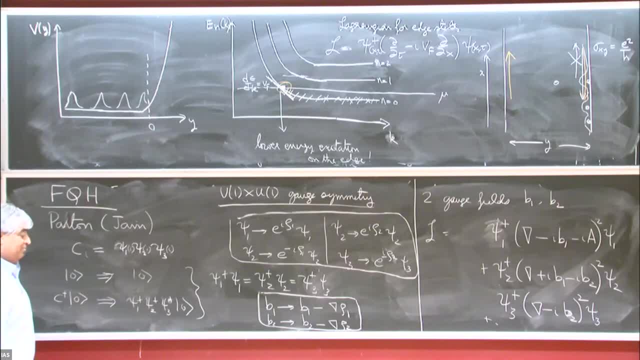 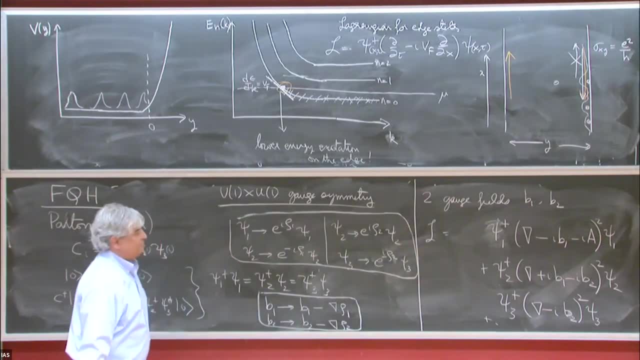 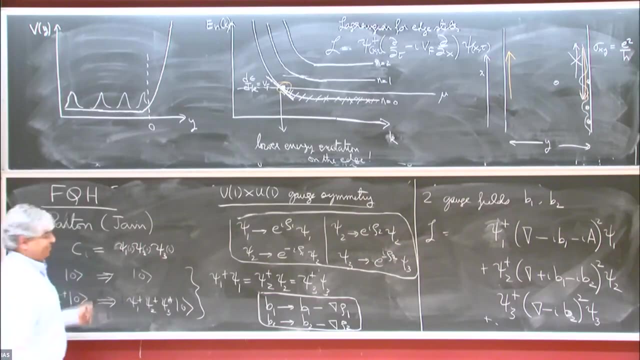 You could do this if you know wherever. You could always do this for any system, But of course, the question is: when is this a useful thing to do? When is this particular fractionalization something that's likely to happen? And I suppose that's probably why the Ponton method- 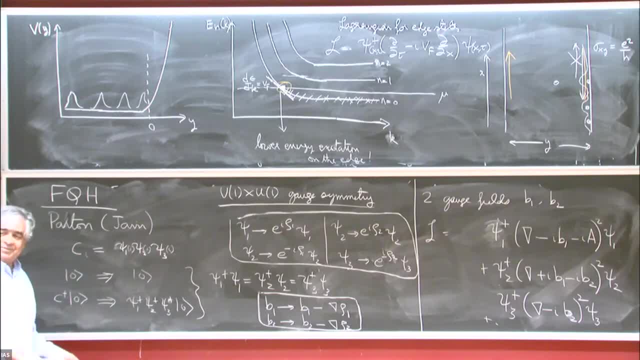 has been used as much. It's very powerful but it doesn't tell you when it's good to use it. Other methods are numerical methods, you know, somehow motivated from this particular Hamiltonian. But it's a good thing. But once others have motivated, 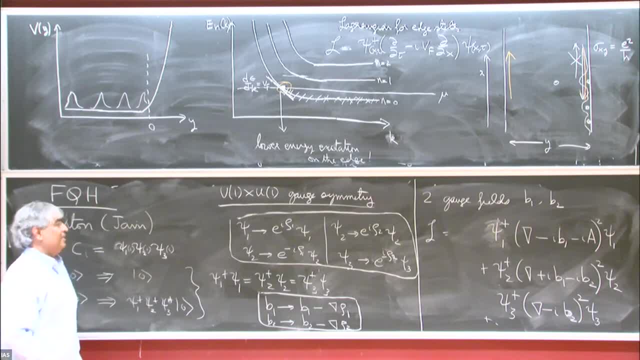 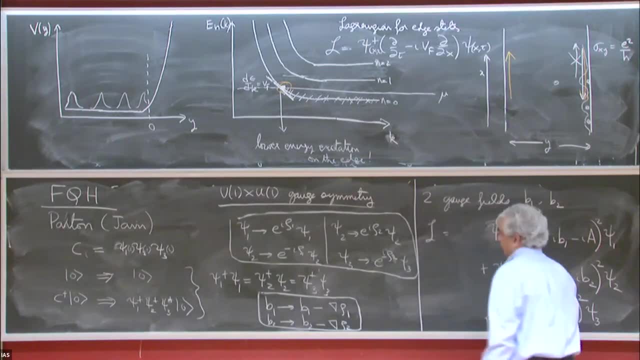 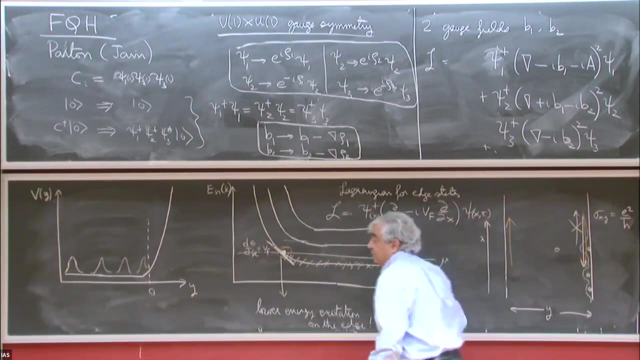 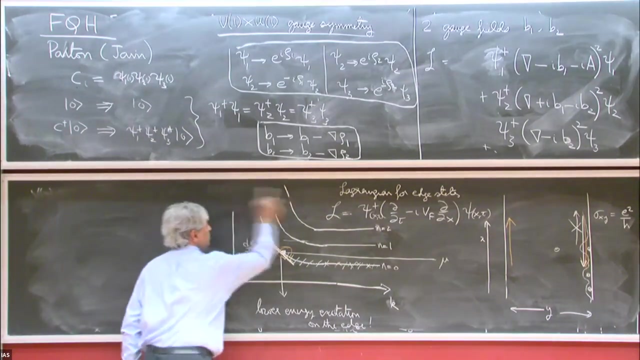 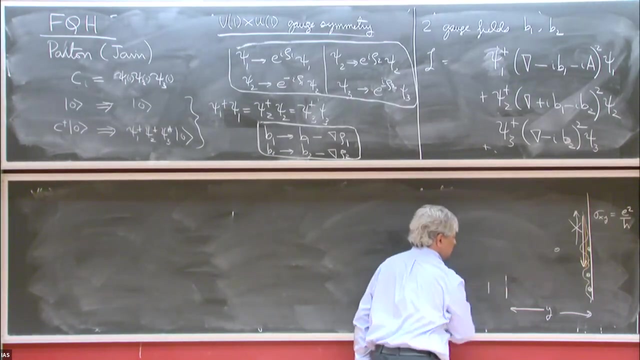 or experiments have seen a certain state. you can just go ahead and figure out what's the right part on description that will give me that state. So why do we use it? So we want to use this in the following situation: So we have an external, so we're going to be in two dimensions. 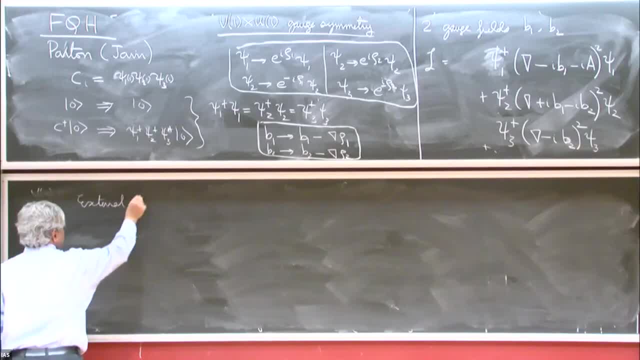 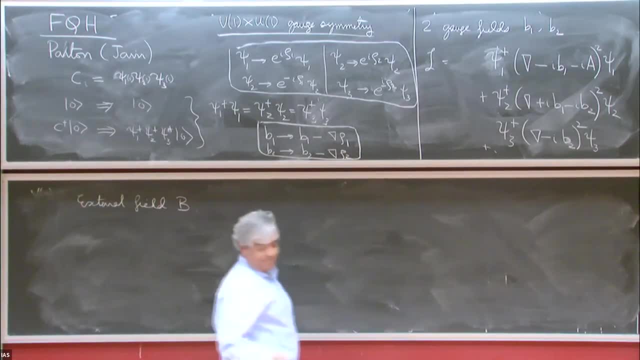 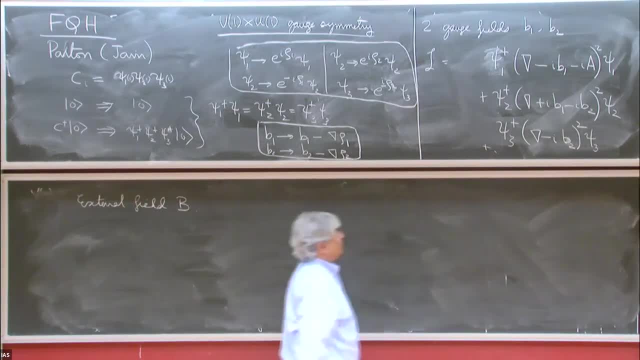 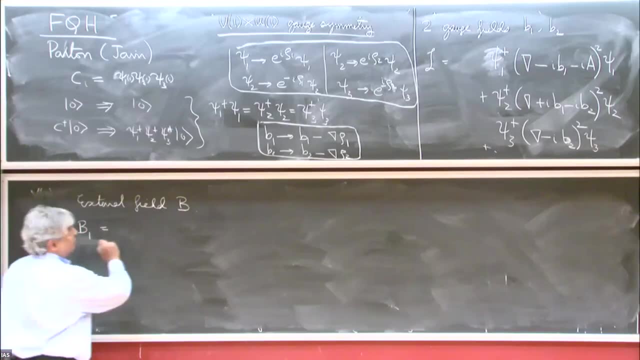 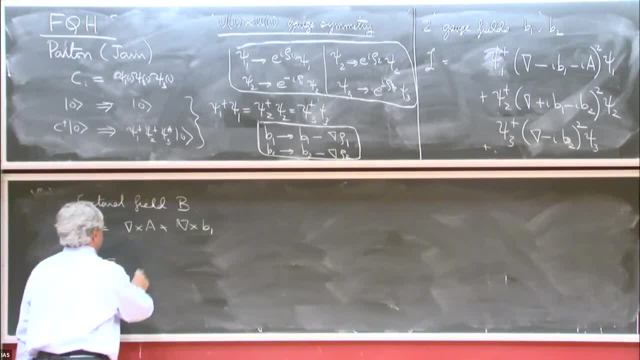 And parton two will experience a field B two, which will be delta cross A, sorry, delta cross B one. B two minus delta cross B one, So that's B one, And B three will be delta cross minus delta cross B two. 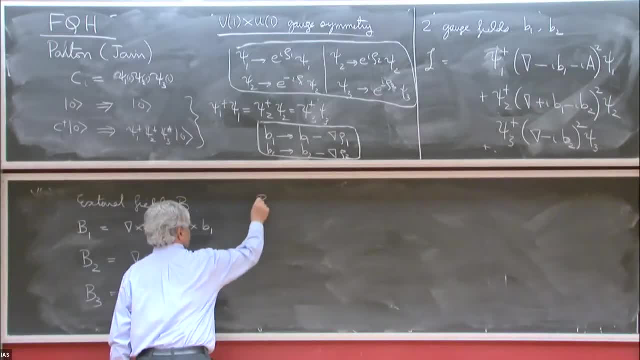 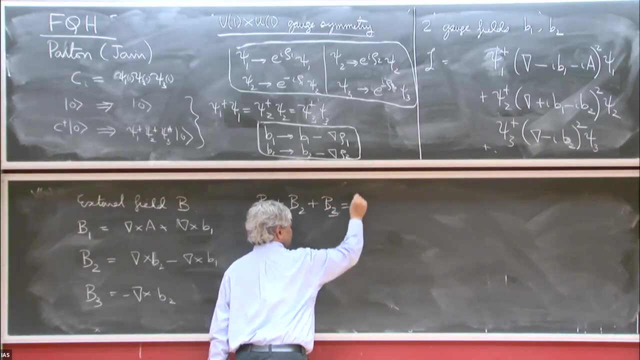 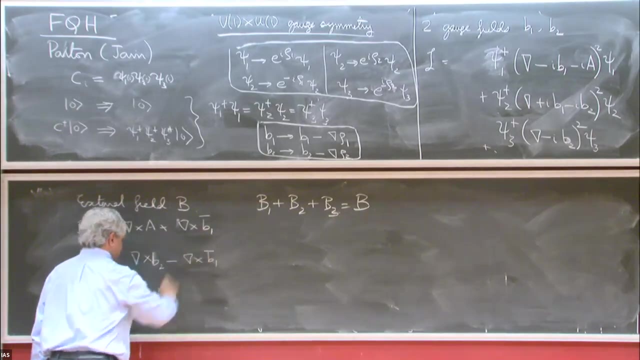 And of course now you should check that B one plus B two plus B three, the next field is equal to the external field. Each of the partons experience a next field. And just I'll put a bar here because we're going to imagine that these gauge fields have 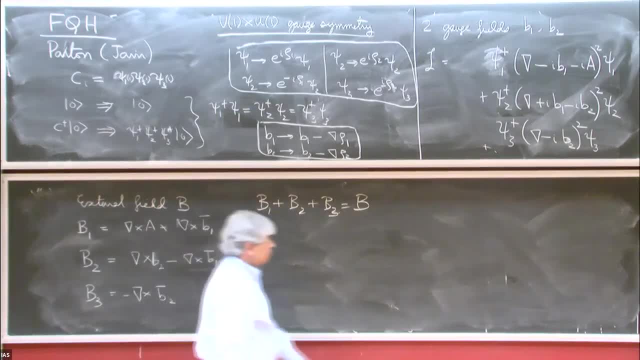 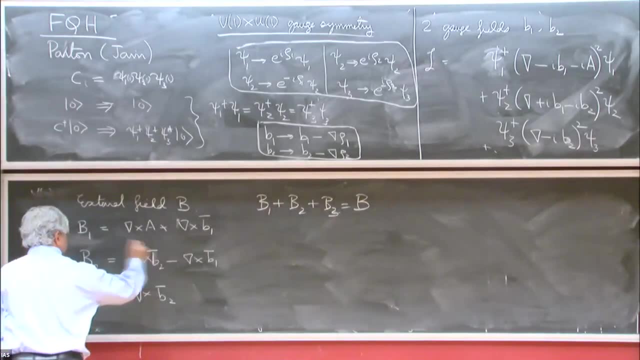 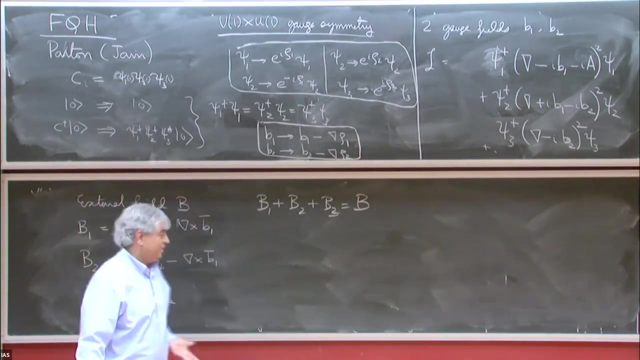 a non-zero expectation. Now you're on the saddle point. These are fluctuating fields here. This is their average value. Okay, So when should this be useful? Well, when it's useful is if the parton fluctuations are weak. And so where would the parton fluctuations be? 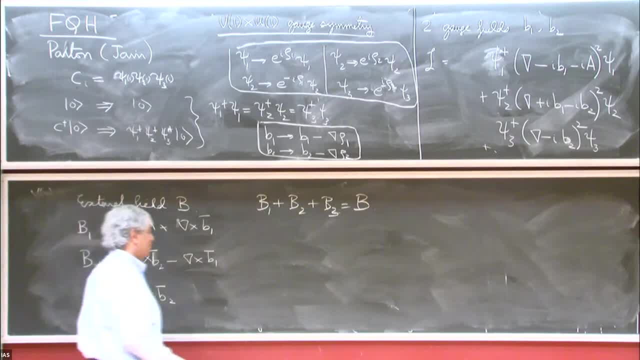 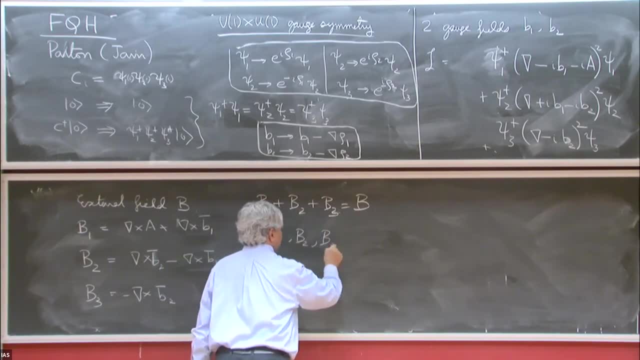 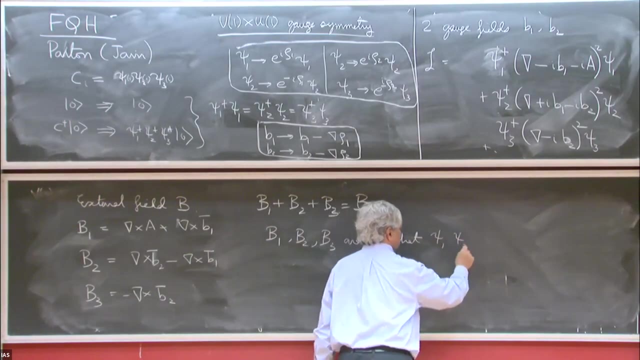 Well, if there's a gap to the parton exudation, So in a magnetic field. so what we require is B one, B two, B three, such that psi one, psi two, psi three occupy N one, N, two, N three Landau levels. 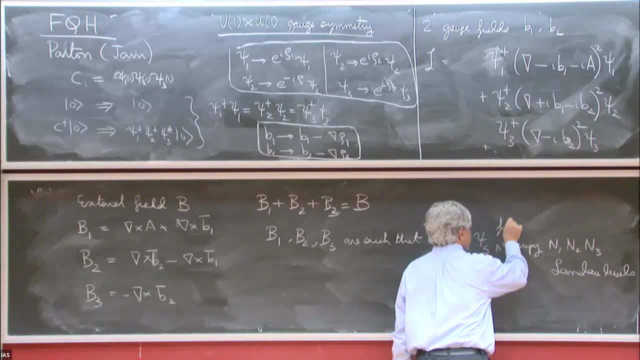 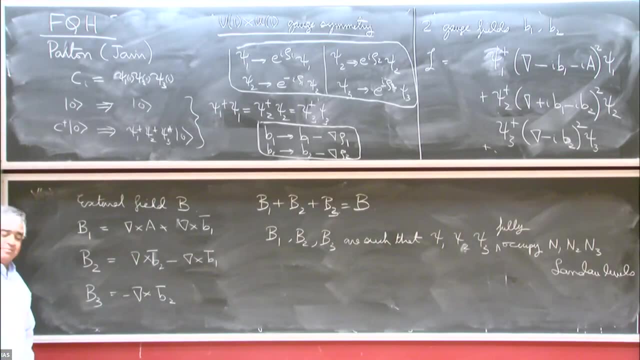 They fully occupy their own Landau levels. Okay, And then you will have a gap. So then the gap to all the excitation of psi one, psi two, psi three, and there's a hope that this very drastic decomposition is like stable. 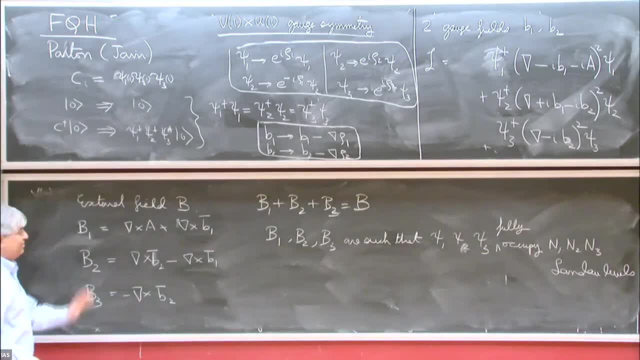 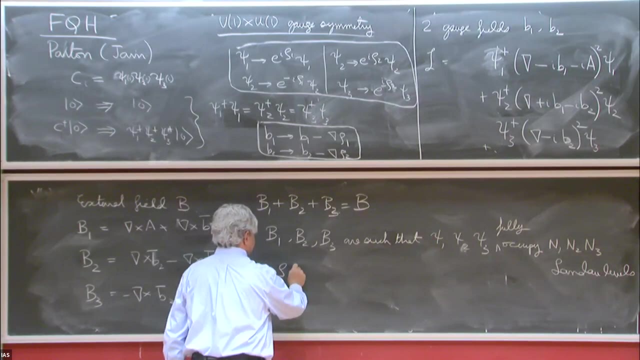 There's no gap with excitation anyway. You may have to worry about other things, but this is a good starting point. So what does this? so what does this imply? So now let me make sure I get this right. The density of the electrons, it's the same. 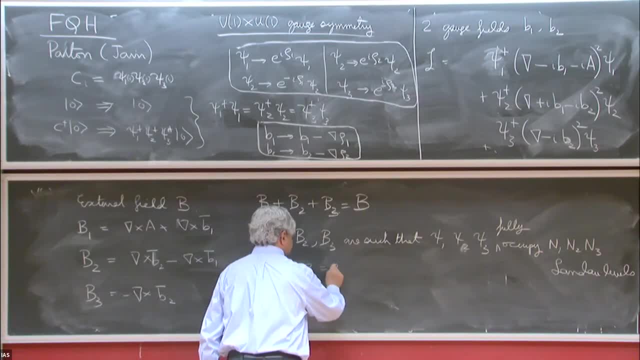 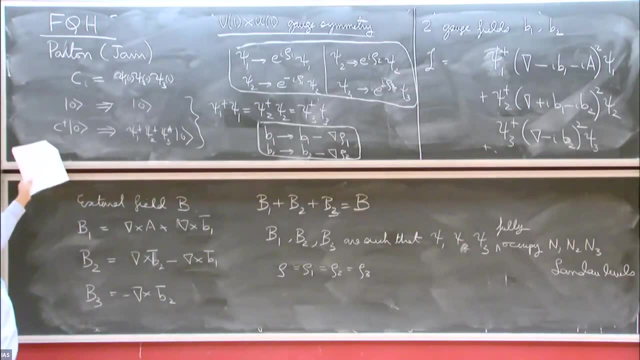 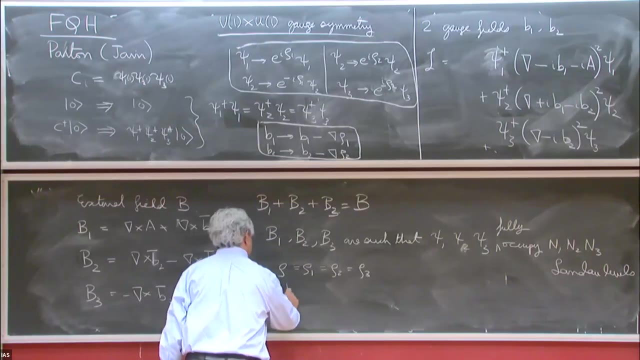 at the density of all. three of them have the same density because of the constraint. this constraint right here. the density of the electrons are the same against the side one cycle, side three. so the filling fractions of each of them, so one over nu, is equal to where did it go? 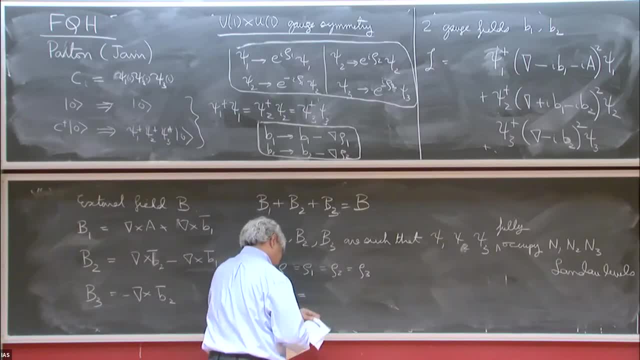 density: rho, one. so rho over b over phi naught. that's the filling fraction of this, filling fraction of the first fermion, which now is going to be n- it's going to be an integer- is rho, which is the same as rho, one over b, one over phi, one, so rho, one over b one. 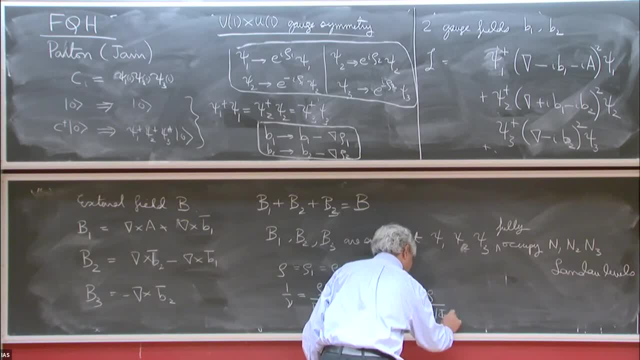 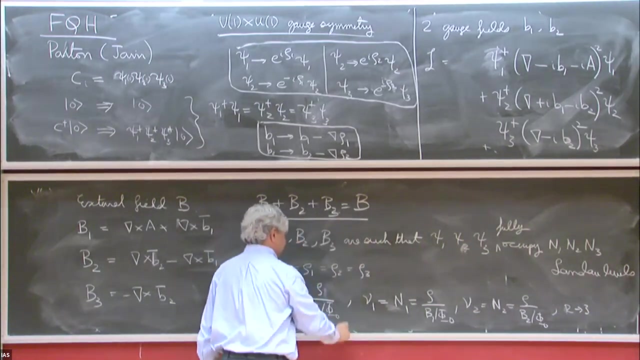 is the same as rho, one over phi one, and so on. nu, two will be an integer n, two, which will be rho over b, two over phi naught, and similarly, two goes to three. okay, so I have this equation here, I have these equations here, and you combine them and you get a very simple expression. 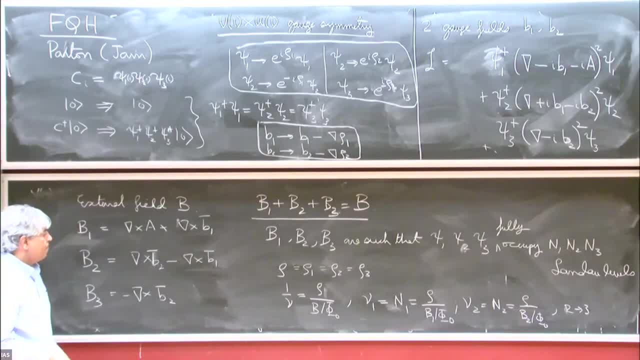 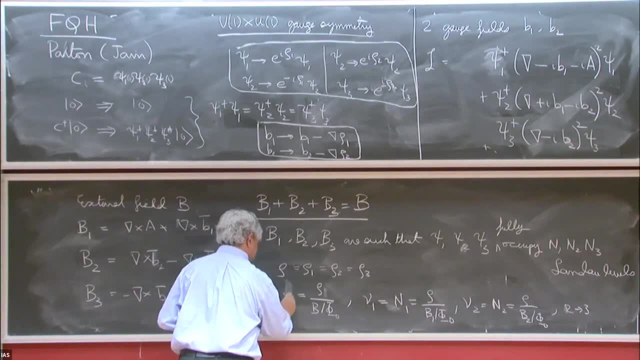 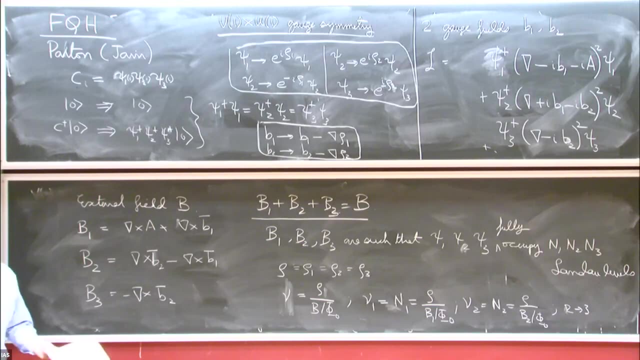 sorry, the first one is new. oh, thank you, this is new. the flux quanta are all the same. oh, yes, e is one. yeah, and h is one flux point at h over e, and so there may be factors of e that you have to carry through, but okay, e is one. 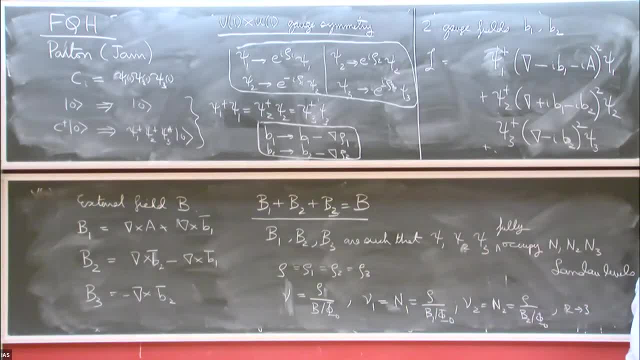 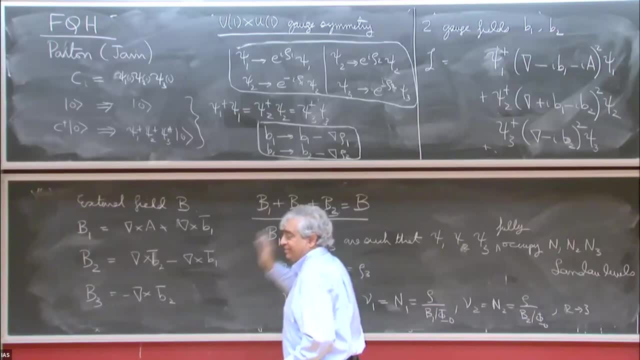 we can always measure p1 in units of e. okay, yeah, which is obviously what we're doing here too. we're just equating the internal free space. external field, for e equals one, all right, so if you combine all these relations, you get a very elegant looking relation for the filling fraction of the electrons. 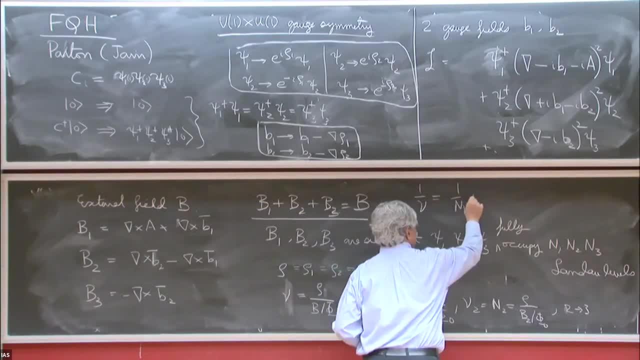 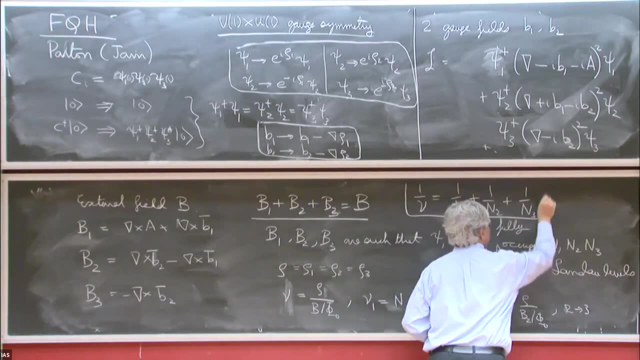 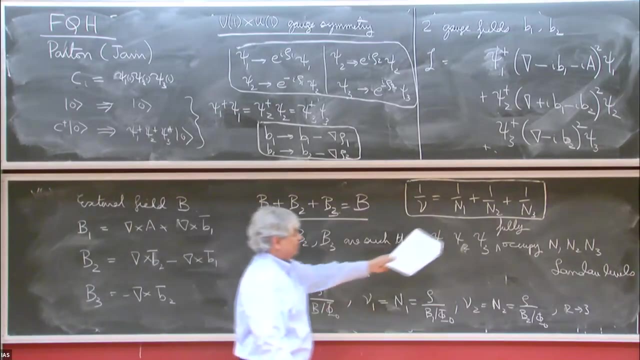 which is one over nu, is one over n one. one over n two. that's one over n two. so that's one over n two. so for this three-part non-construction to work, n one, n two and three are positive integers. okay, they can even be negative. 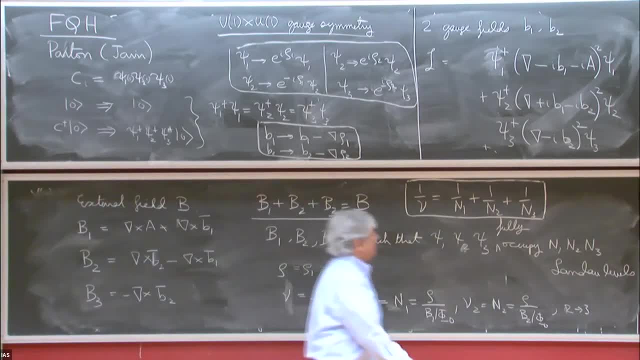 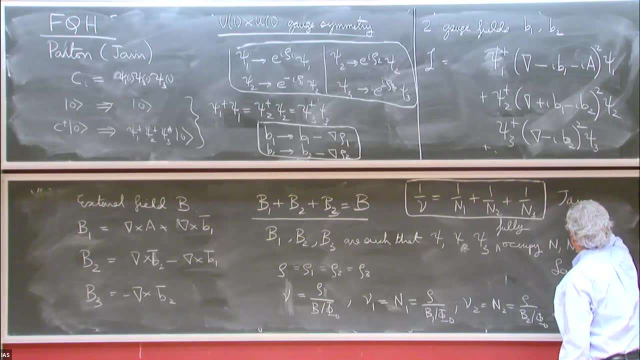 if you put the field in the other direction, we won't consider that. then this is the, the special filling fractions, and these are, you know, special case of what I call the jing fractions, and in fact, essentially all observed states are of this type. okay, all right, so that's it. so now we have a saddle point which has a gap. 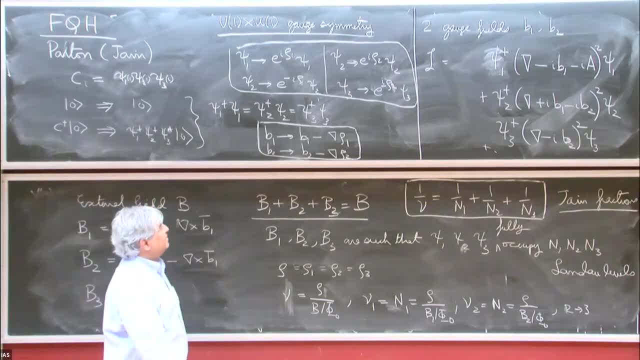 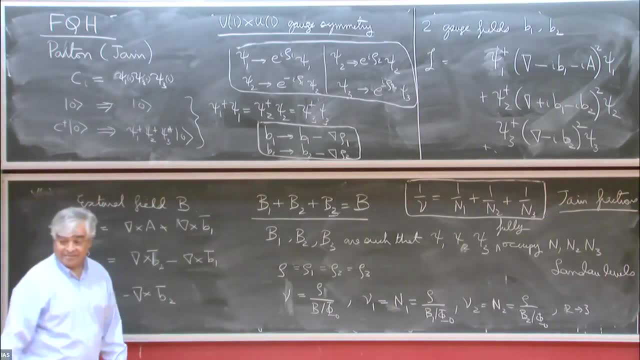 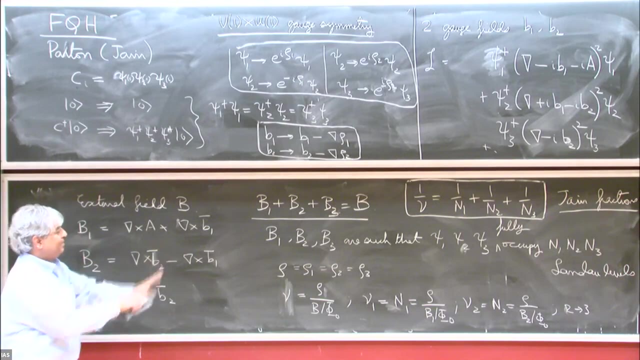 then we can do all kinds of fluctuations about it and you know you'll get transaxle theories, edge states, but we've done enough of all of that. in fact, the whole analysis will be identical to things we've already talked about, just the different cases of that, okay. 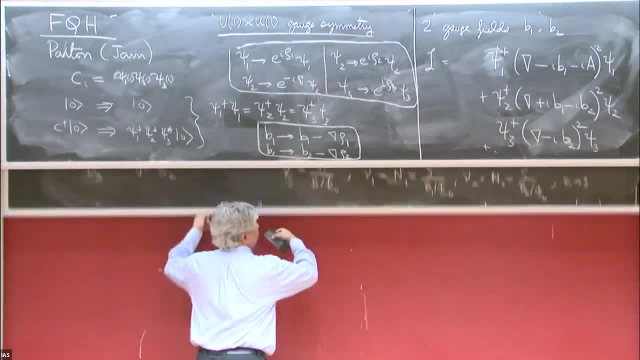 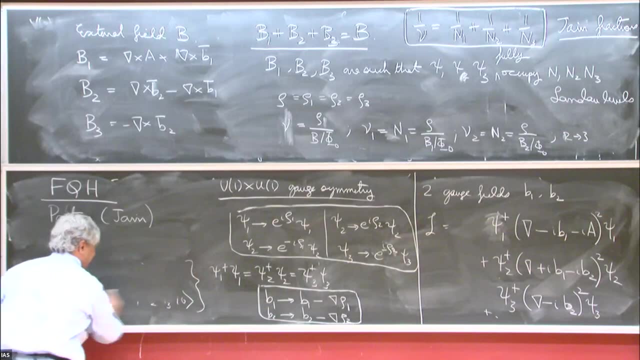 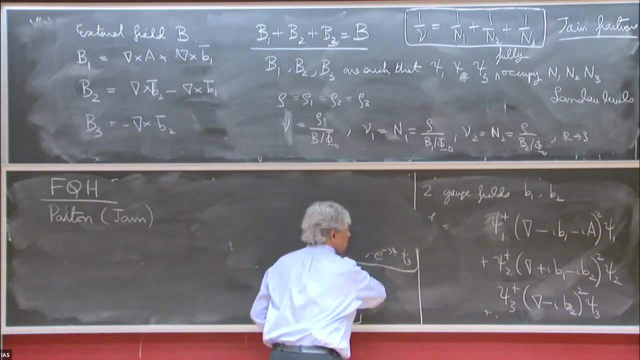 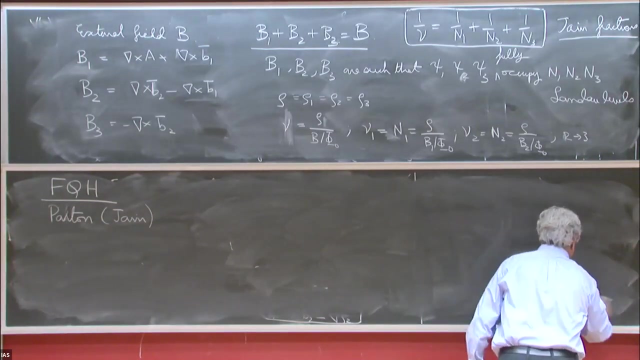 okay, so what's the simplest case? the simplest case is: n one equals one, equals two equals three, so all of them equal to one. is there a simple formula for the term simon's levels in terms of these integers? that you, yes, but i'm not perfect. 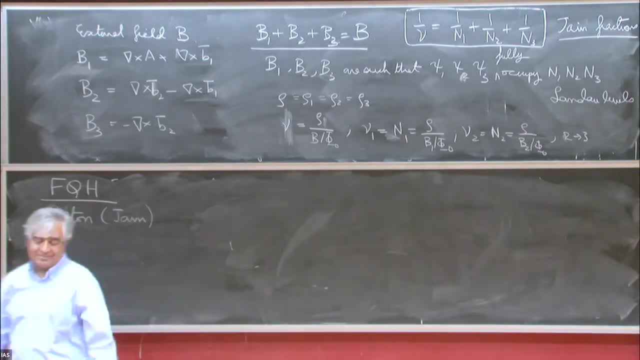 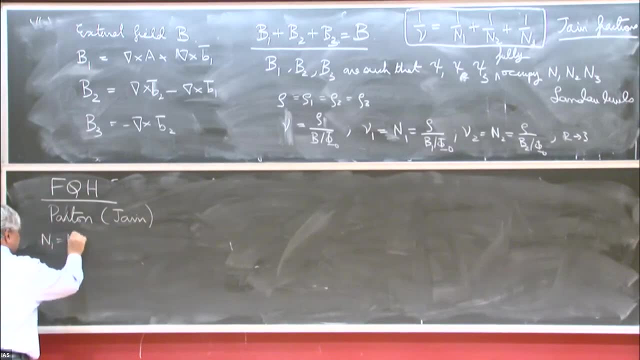 it's a bit of a mess. i think i've only done a special case, so we're going to look at the case first of all. the most important case is: n1 equals one equals n2 equals x3 equals one, when, of course, nu is one-third. that's the famous Laughlin state. 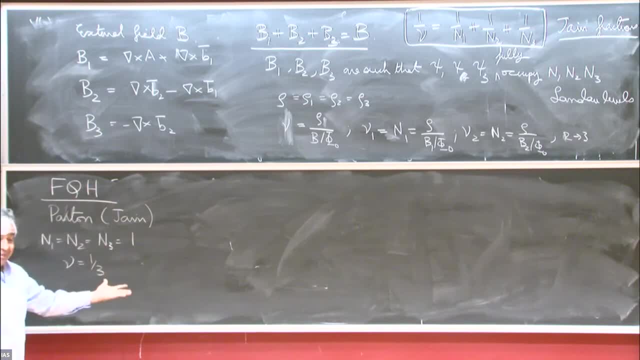 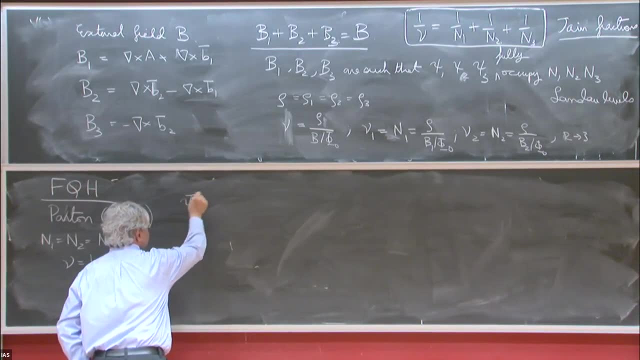 and now, to go back to the beginning of the lecture, i can write down the wave function of this state. so the wave function of the electrons, so this is the capital psi of z1 to zn- is the product of three wave functions. it's the product of, let me say, 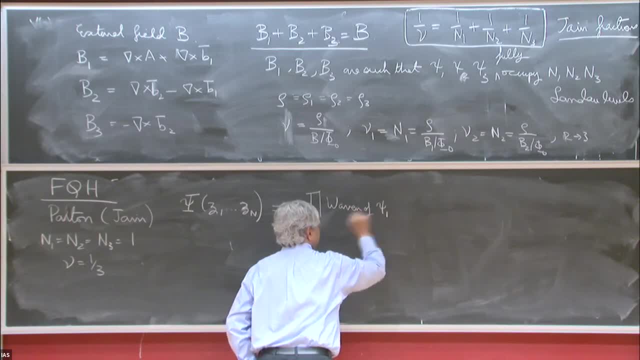 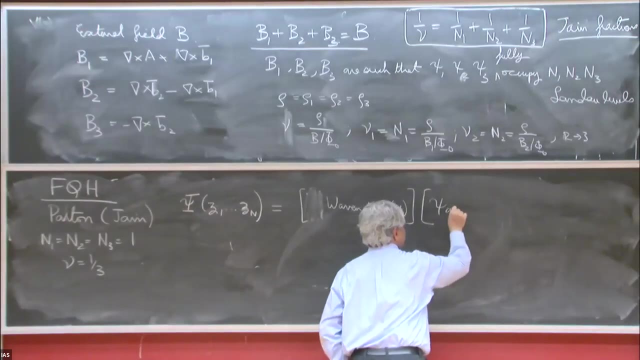 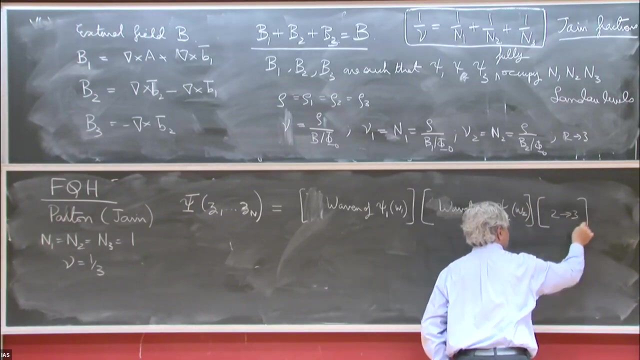 wave function of psi one, and this will have some coordinates and they call them w1, and similarly for the other ones, but the product is outside the function of the field. psi two, with coordinates w two, and two plus two, three. Okay now, what are these wave functions? Well, these wave functions, we already know that there was. 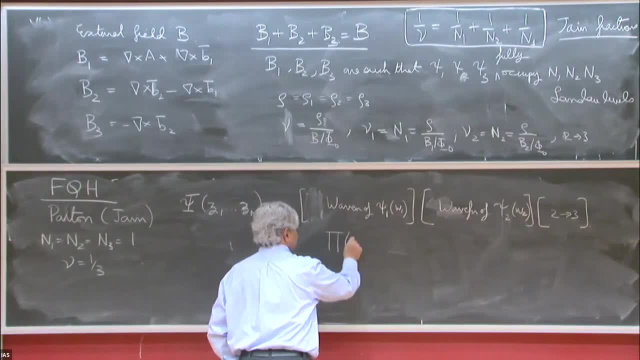 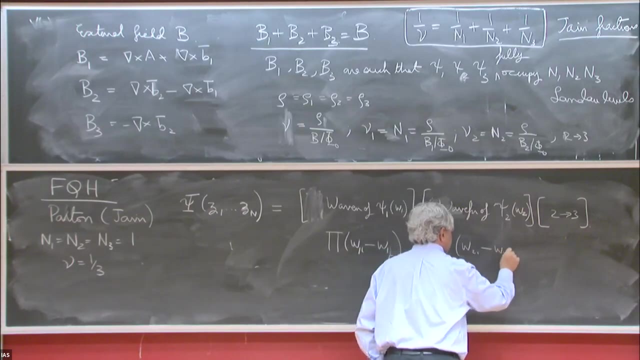 a landau level. So this is product of w one i minus w j. Let me not worry about the w one i minus w one j, and this will be product on w two i minus w two j, and this will be product of w three i. 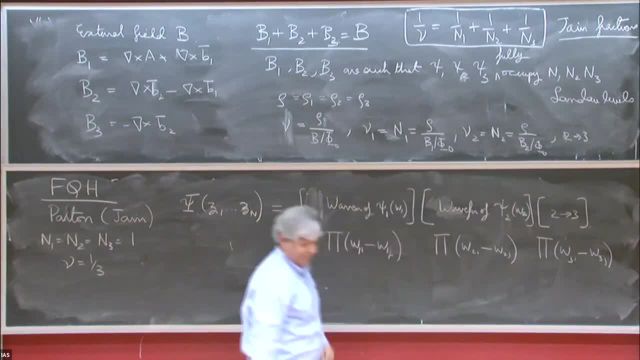 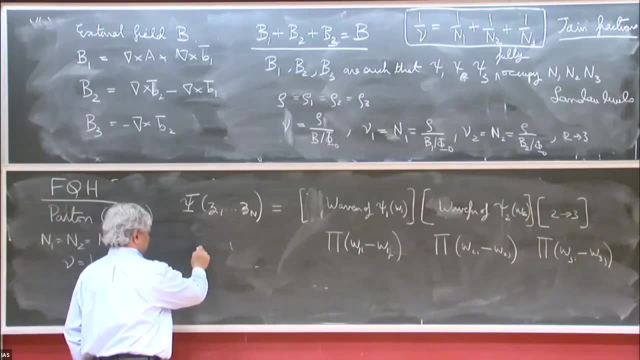 minus w three j, That's the fully filled landau levels, The vector bound between it. and then you have a constraint that the densities are the same. So we have the constraint that z i equals w one, i equals w two, i equals w three i. That's the original constraint that you 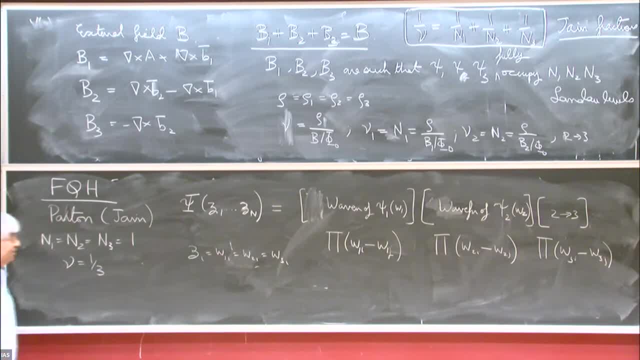 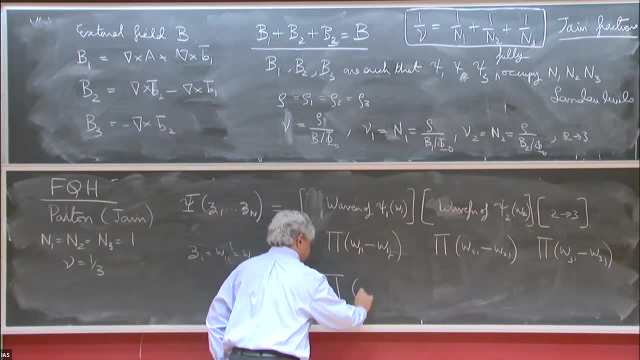 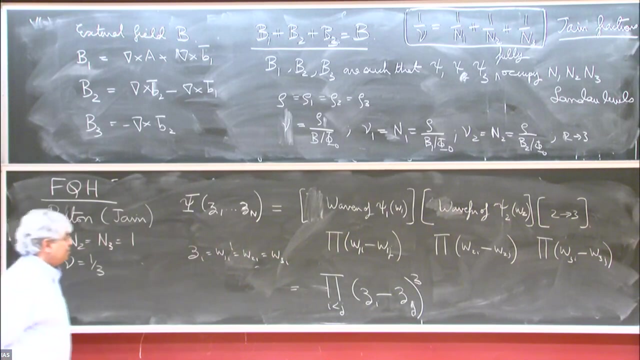 had. Then we started out the part on construction and of course then this is the famous landau, and i leave off the exponential factor. You could satisfy the constraint with extra phase factors, right? Well, these are the coordinates, The position of the particles, wherever they are. 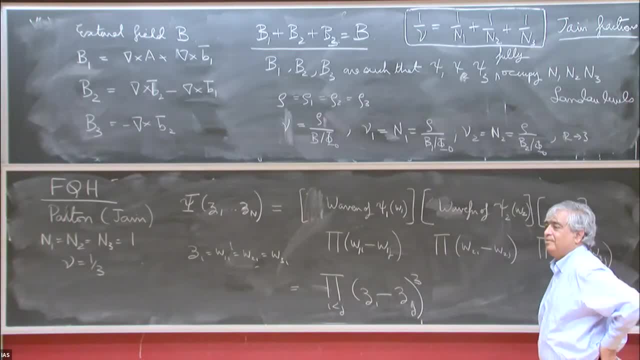 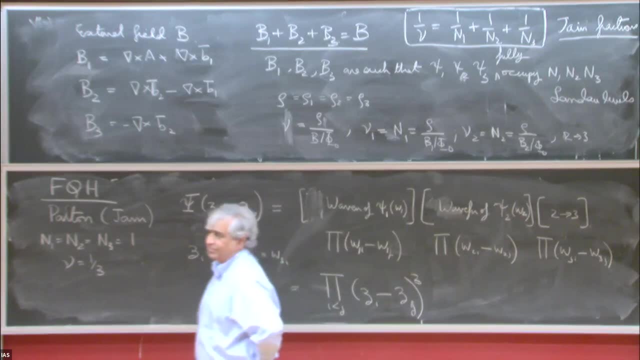 have to be the same, But the real constraint is that the density is the same. If you apply that at every point, then the coordinates in the first point does represent the coordinates of the particle. I'm kind of going back and forth with the second one. I'm just saying 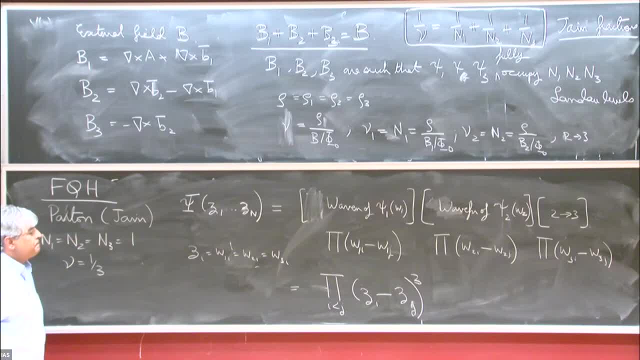 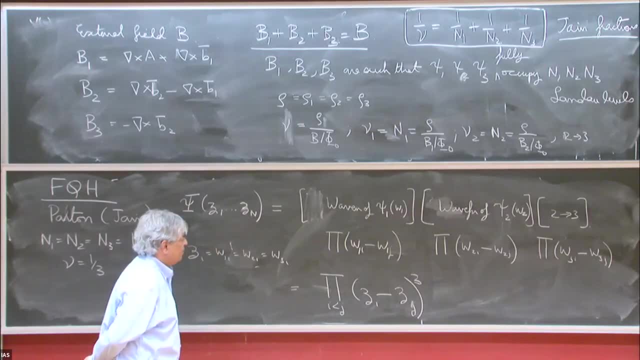 individual wave functions could have factors that would disappear when you enter the density. I'm not sure which factors you're referring to- Some things that appear up here. I think this is fine. I don't think there's any arbitrary less here. So that's of course the Loughlin wave function that started this whole. 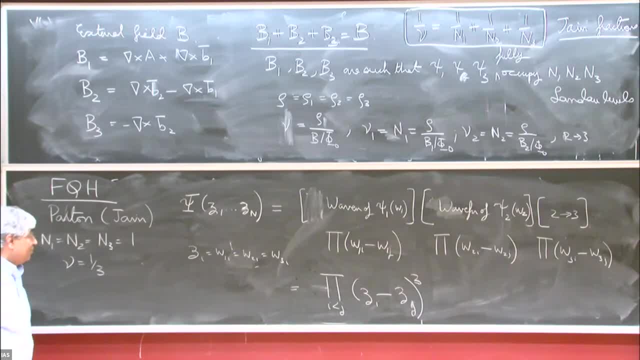 analysis and then later on, Jane pointed out that in fact this is one very simple way to think about it. But then the power of change approach, and after Loughlin's wave function, there was a very complicated theory- I should say, at least complicated for me- of what's called 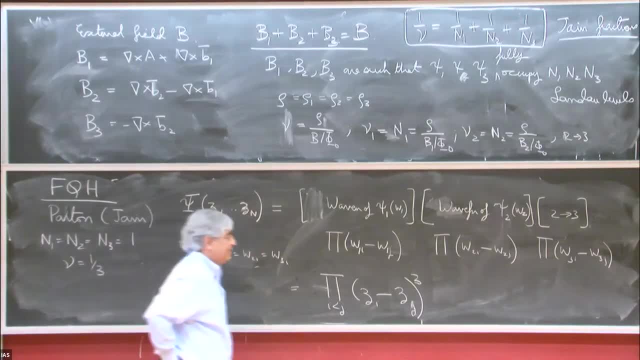 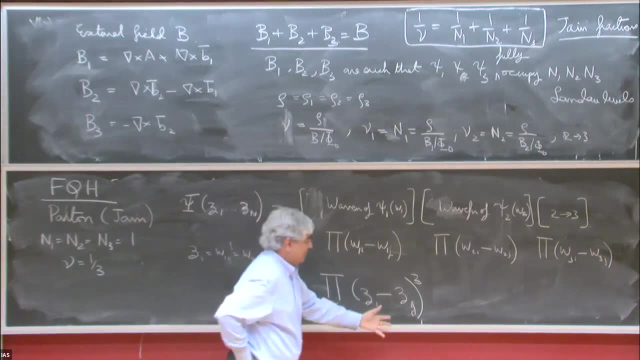 the hierarchy, because the experiments could be shown many other fractions, And so people developed a hierarchy and the basic idea of the hierarchy was: well, you have the Loughlin's state and it has certain quasi-particles which have fractional statistics. All of that is very 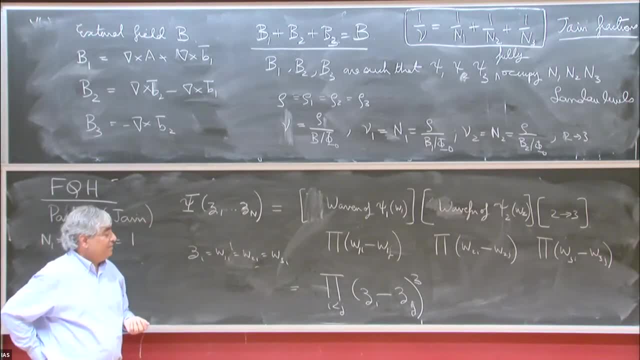 similar to the chiral spin liquid, And then those fractional statistic particles can form states of their own Fractional point of hold states and other density. So you get a finite density of quasi-particles about the Loughlin state and then you get higher. But the hierarchy 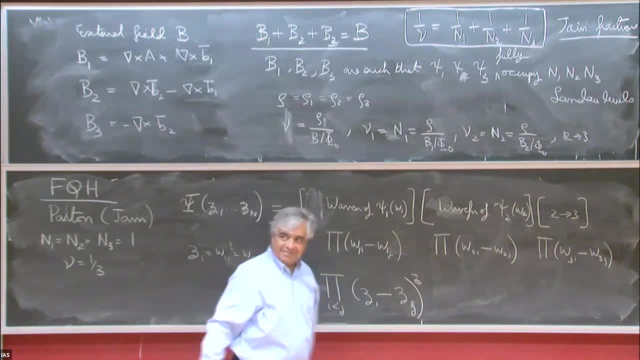 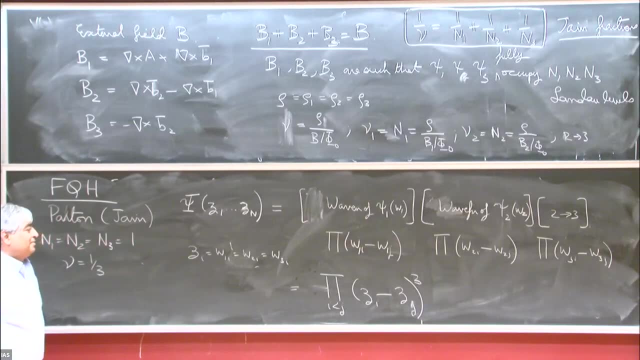 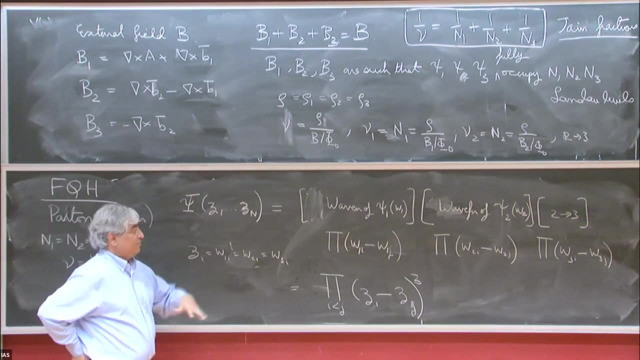 is nothing wrong with it, but it predicts all kinds of fractions- only a small fraction which are actually seen. And also there's the question that the hierarchy assumes- you know, the whole structure of the hierarchy, at least initially assumes- that the quasi-particles are dilute. But to get the higher, 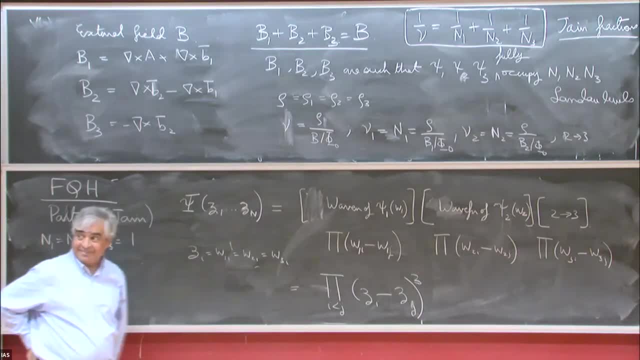 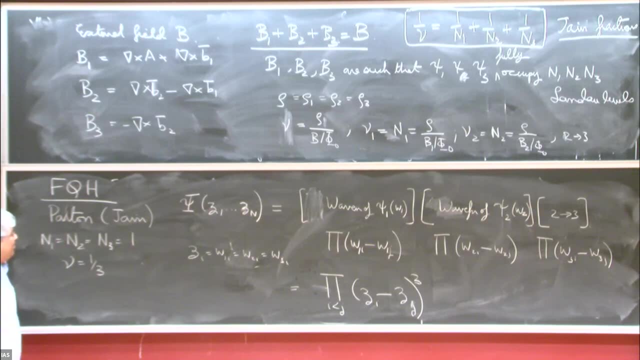 states in the hierarchy, you're making them quite dense. So should you really believe it? At least qualitatively you could, but quantitatively it may not be the right way to think about it, Anyway. so what Jane showed was that if you did this approach, in fact it was highly predictive in the 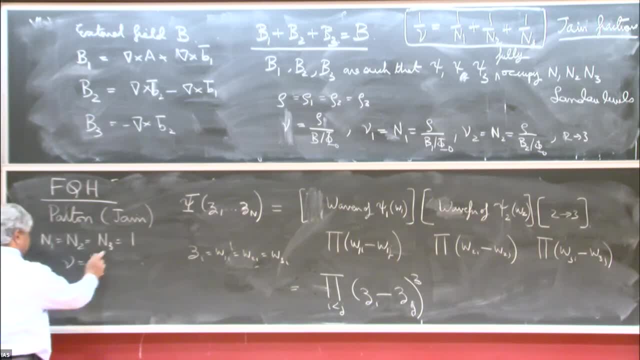 way that the most important fractions are the ones where you just take one of these integers and make them not equal to one. So, more precisely, the other important cases are: n1 equals one, n2 equals one and n3 equals n greater than one, So you put two of the 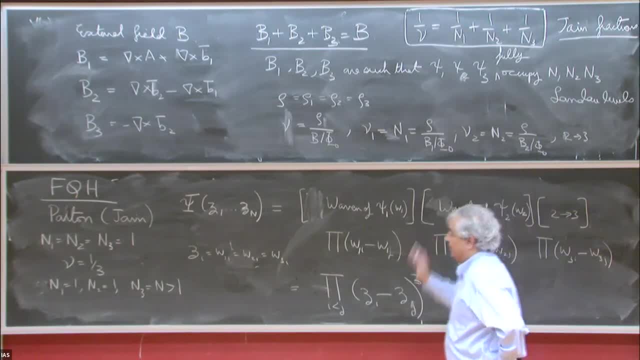 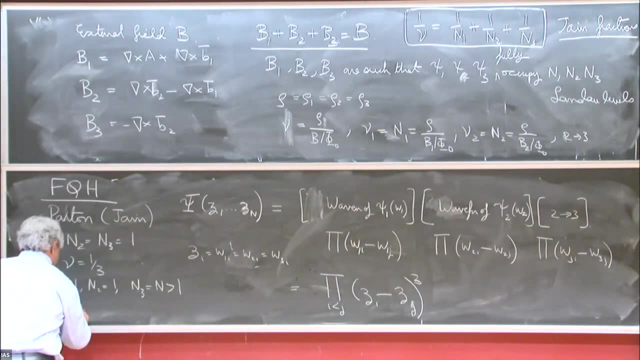 partons in the lowest landau level and the others in some higher landau level. Then you take that famous expression and work it out. You get: nu is equal to n over two, n plus one, And these are the by far the most important quantum model fractions. 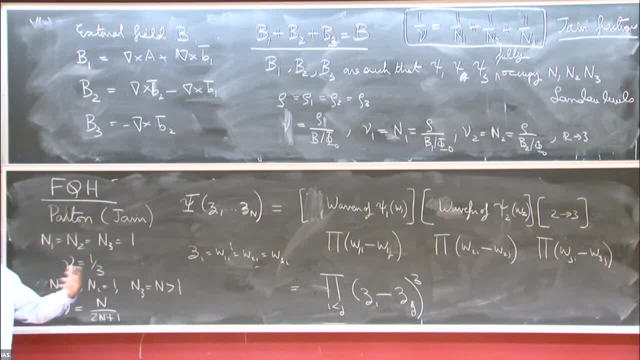 The next one will be n equals two, which will give you two-fifths after one-third and so on. Okay, so how much time I have, So probably I have to say a bit more next time. So now there's two of these to get nu equals one-fifth. do we go to five partons or do we get it? 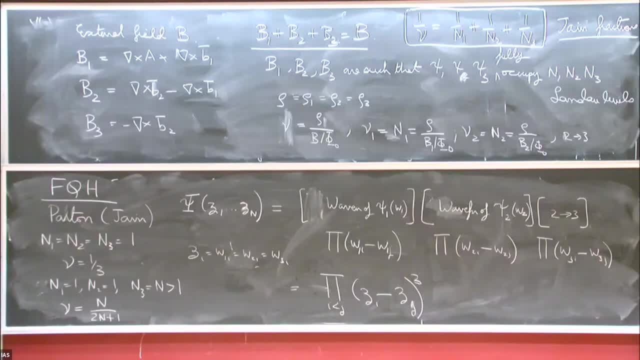 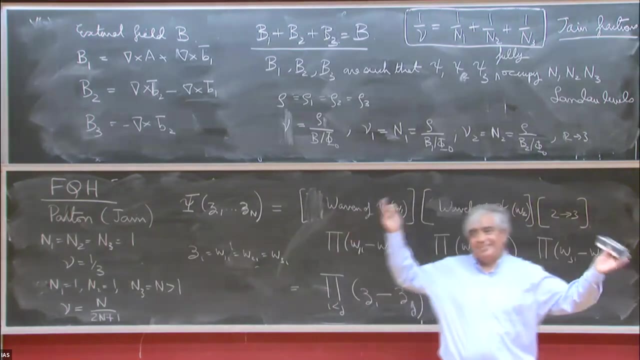 The one-fifth. yes, five partons, but that's a relatively hard fraction to see. It's pretty close to Weibner crystal, Most of the ones that you know. experiments are around. u equals one-half, Yeah, but in principle right. this also has its- you know- letter of possibilities. 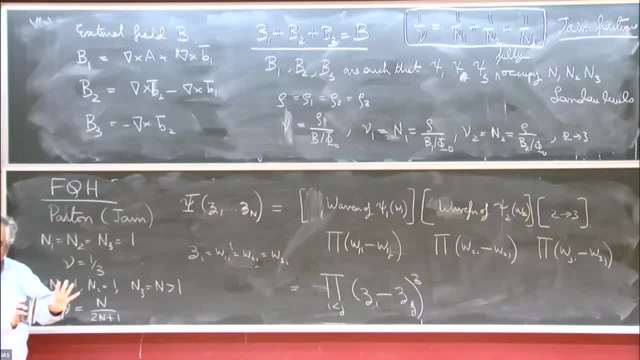 So what's nice is that the very simplest possibilities. that three is the smallest thing you could do And you can't go to one, then there's nothing to do. Three is the smallest allowed number And you just make one of them greater than one. 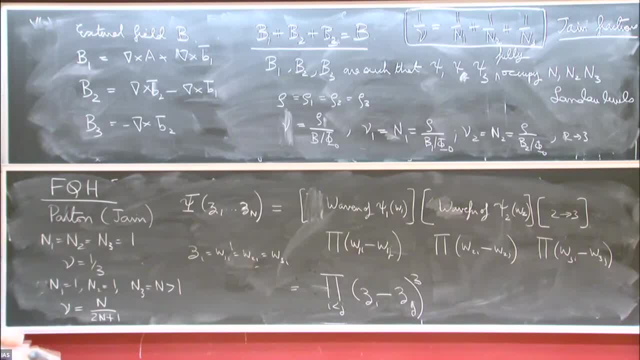 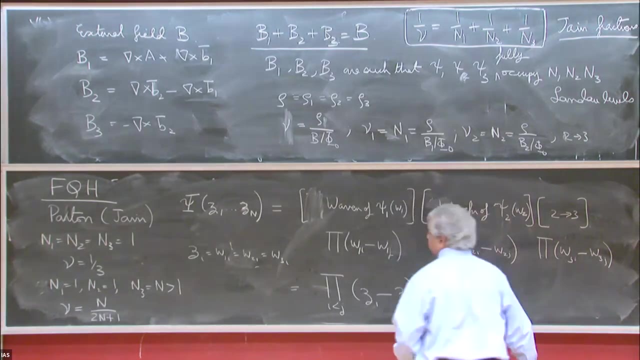 that's sufficient to give everything. So there's a certain economy here, But of course it's in fact all of the states in the hierarchy can also be obtained by this approach. Yeah Well, I have 15 minutes, So what should I talk about? 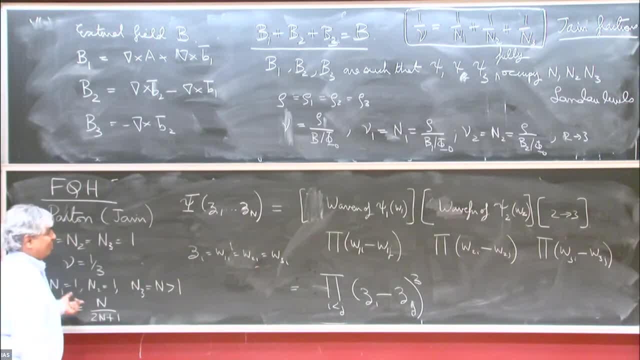 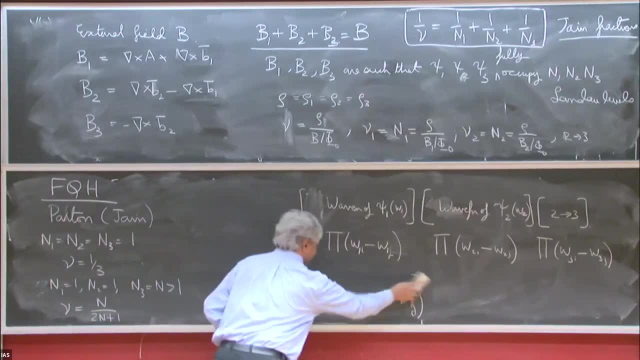 Okay, maybe I'll talk about edge states next time. Let me talk about one very important case, but there's a slightly different type of topology. So at this point, if you've been following my lecture so far, you just have to turn the crank. 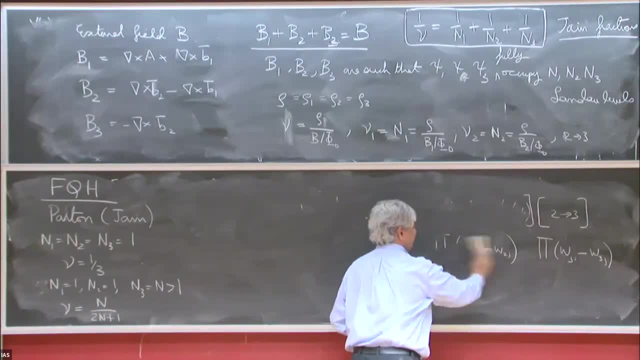 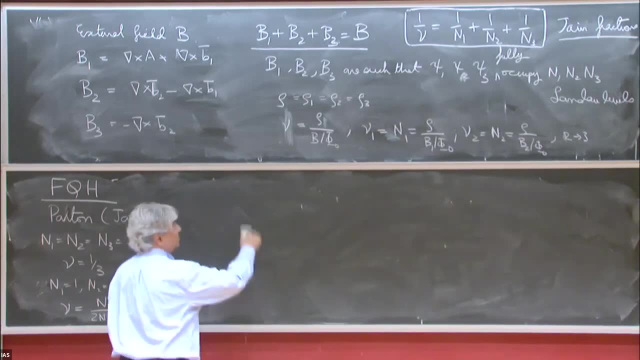 and do everything we did for the chiral: spin liquid and figure out the edge state theory, the statistics of the bulk quality particles and all of that, And just take that theory and you integrate out the fermions and look at the edge states. just repeating what we did. 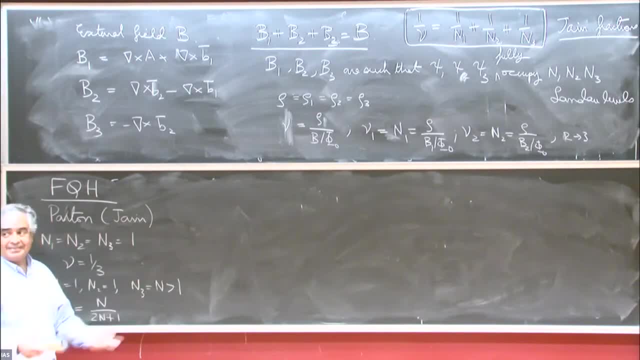 for the integer quantum Hall state, but now with this gauge fields and so on. But let me mention here- maybe I'll say a little bit about that next time and then we'll be done. But let me mention here another very interesting case where you get some new types of states. 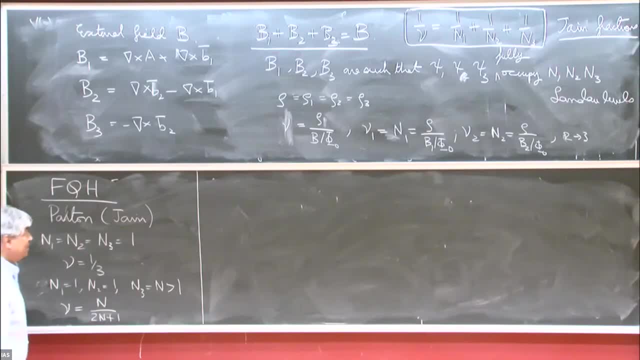 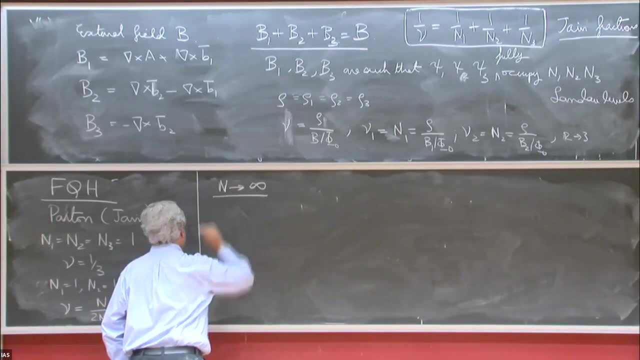 which have no analog, really what we've talked about so far. So the one case is N goes to infinity, Or that take the N goes to infinity And so your new then becomes one half. So what this means is that the side three fermions. 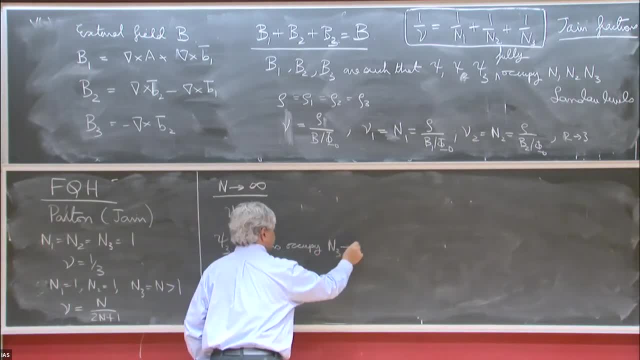 occupy N3, infinity Landau levels. And what does that mean? Well, really, if you look at this formula here, if you're filling integers going to infinity, well, the way it goes to infinity for a fixed density is your B field is going to zero. 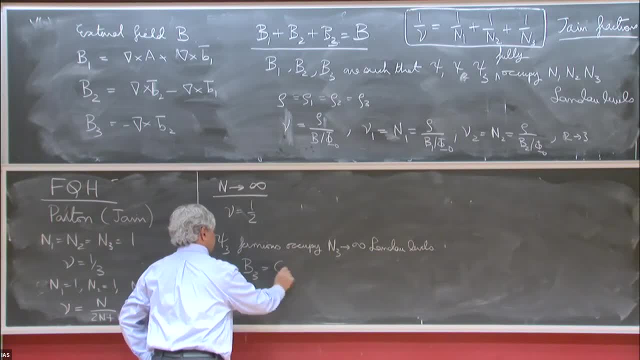 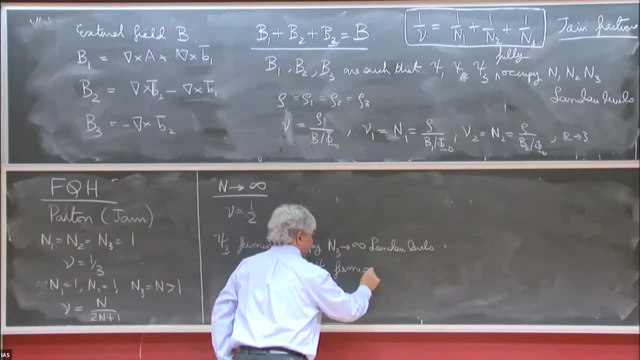 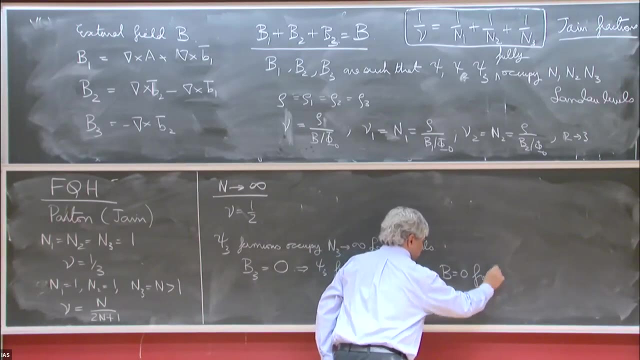 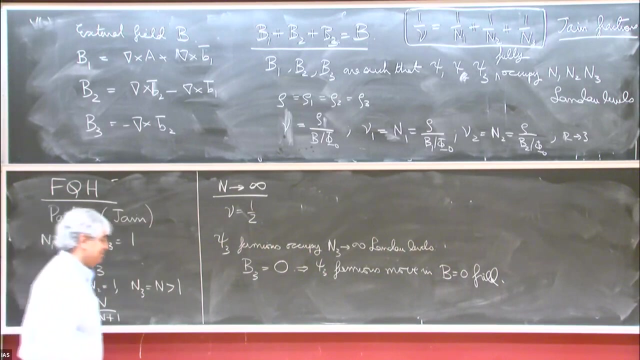 So that means B3 is zero. And so the side three fermions move in zero field, And so the side three fermions move in zero field. This is a whole new ball game. What do fermions, when they move in zero field, do? 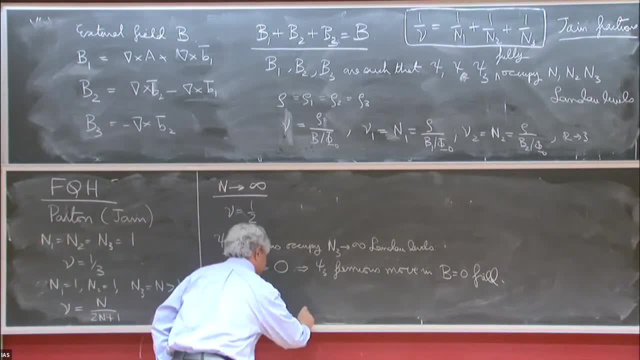 They form a Fermi surface. That was chapter one of the course. So we would expect the side three fermions to not fill Landau levels but will form a Fermi surface. So this is some Fermi vector here. KX and KY. 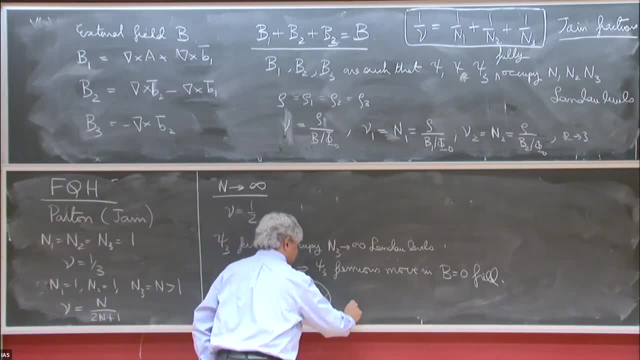 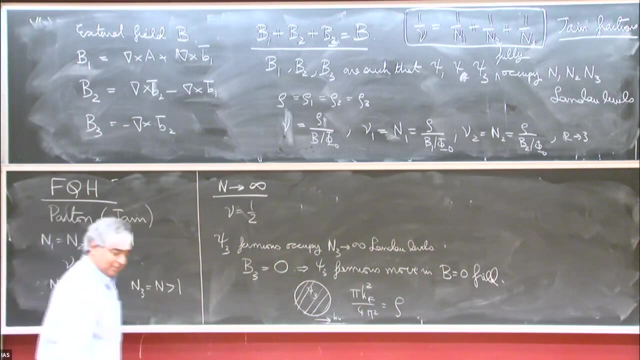 And the volume enclosed by the Fermi surface. these are spinless. Well, that's pi KF squared four. pi squared is going to equal the density of electrons, because the density of electrons will equal the density of side three fermions. So this is potentially a dangerous thing. 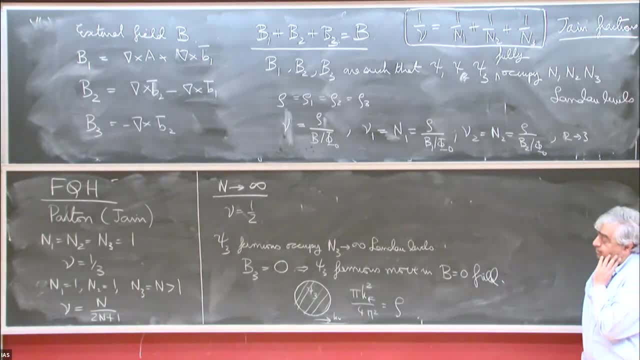 with the logic of what we've been talking about, in the sense that the side three fermions will no longer have a gap. So now you can take a fermion from inside the Fermi surface and put it outside with arbitrary low energy, And so it's a gapless state. 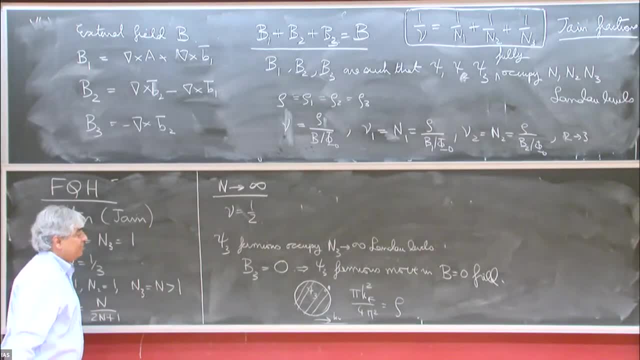 unlike all the states we've talked about before, where the piece in the bottom had a gap, This doesn't have a gap in the bottom. Okay, but now there's actually quite a lot of good evidence that this state is seen in experiments. They help in the restate. 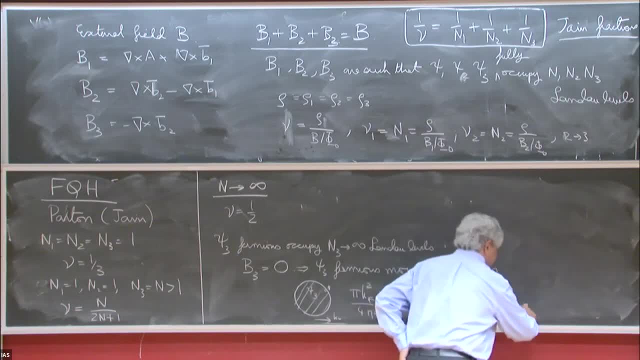 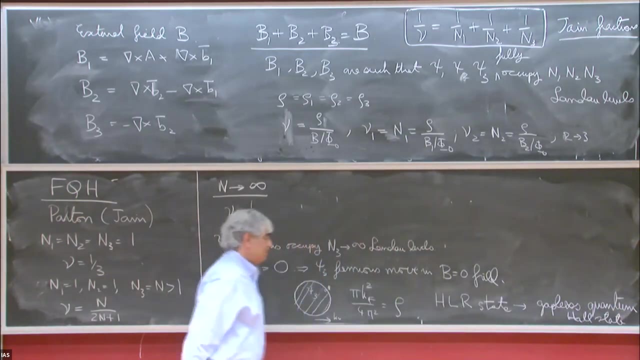 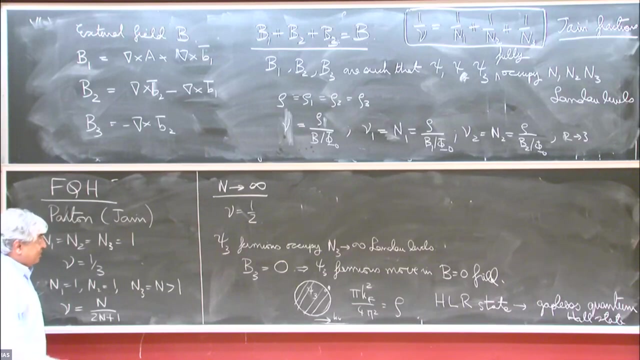 So the HLR state and it's a gapless formal state. Well, the whole procedure of edge states and so on doesn't really quite work here because you have gapless expectations in the bulk. But nevertheless the gauge field approach has seen a lot of, in fact does work. 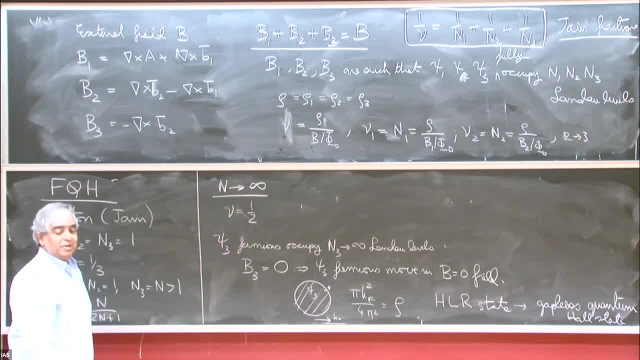 As we understand today, the gauge fields do have very strong effects now on the bulk and they change the spectrum of these particles And you get what we call a non-Fermi liquid. It's not a Fermi liquid like we started off with. 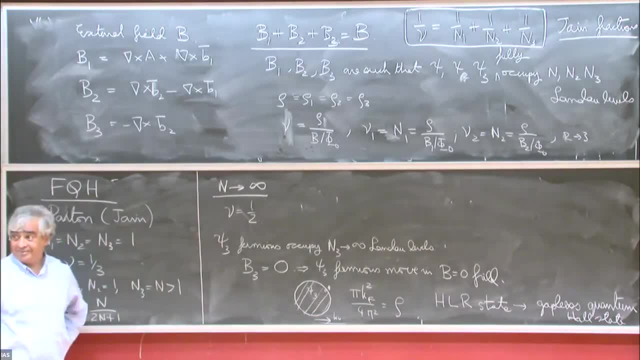 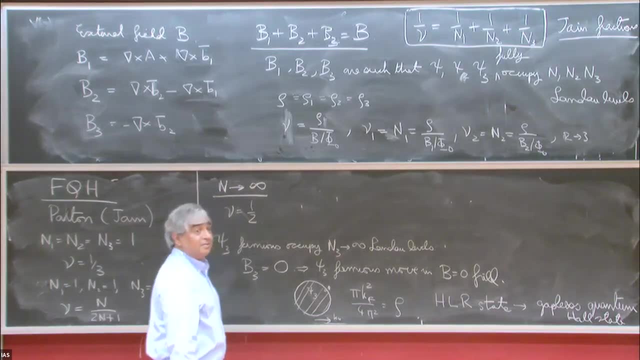 And this is a topic that I will cover towards the end of the course. So, but this is one way. you get a problem of fermions coupled to a gauge field. The gauge field here is what you call B2? Yes, so what will happen is: yeah. 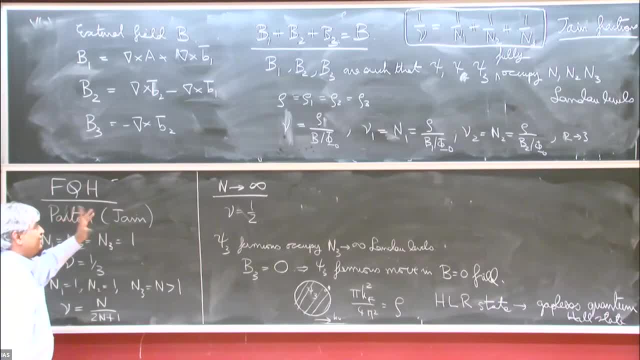 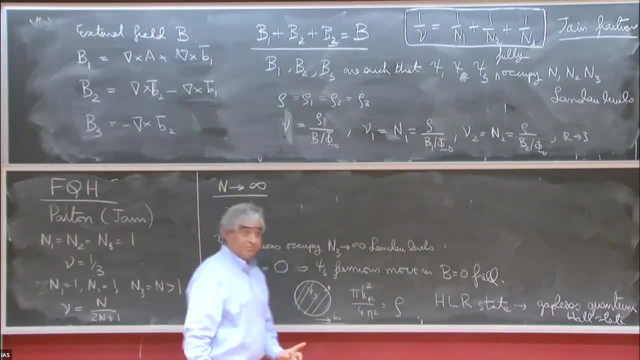 the B1, you can integrate it out Now if you okay. so this is another important point. In reality, there's really two gauge fields: B1 and B2. And they have- B1- will have a Chen-Simons term. 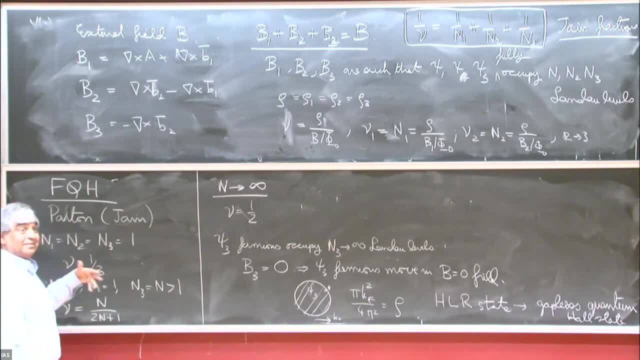 that you can get from integrating out N1, the psi one and psi two fermions. Now if you integrate out B2, which formally you can, then you'll end up getting Chen-Simons term with the improperly quantized in the bulk. 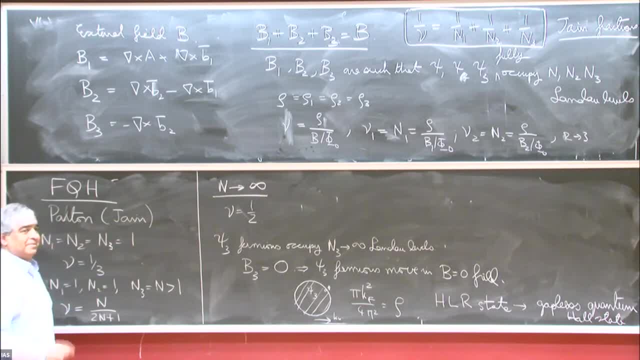 So if you want to work with just one gauge field, then you have a Chen-Simons term that's not properly quantized. But you can fix that, as you and others have shown, by keeping more than one gauge field. This formalism automatically gives you: 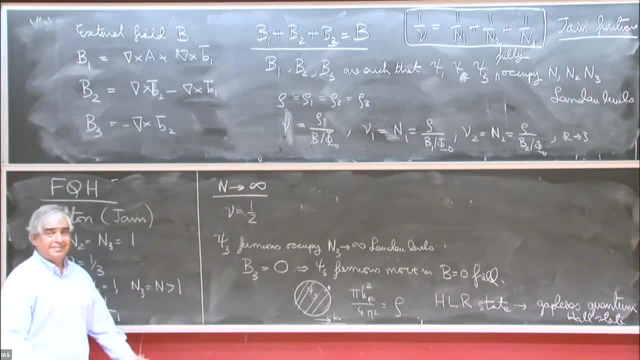 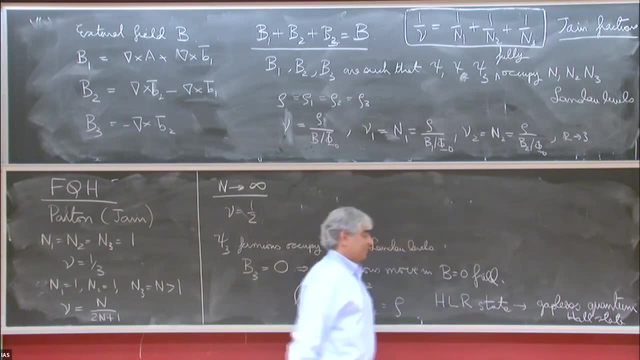 the right number of gauge fields. you need to get everything properly quantized. Well, so this problem: since there's no charge, there's no gap in the bulk. maybe it's not such a big sin to just work with one gauge field, because you never have eight states or anything like that. 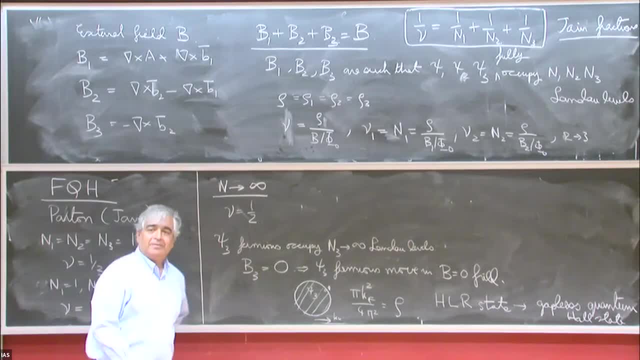 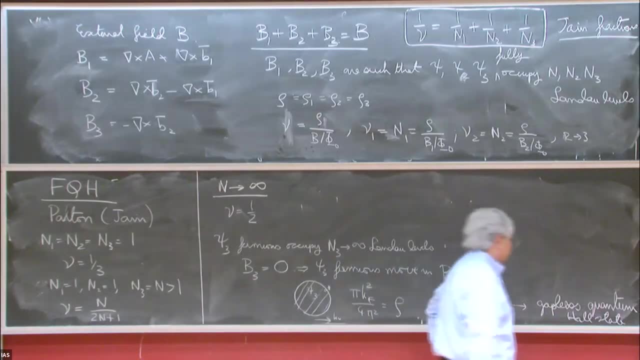 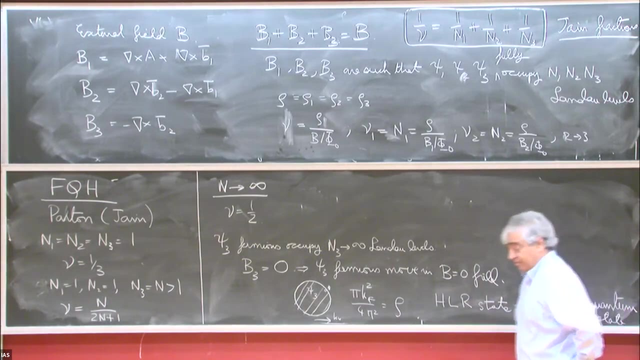 Everything's really in the bulk. I don't know. did you disagree with that? No, Okay, All right, great, Okay. So you have fermions in a zero magnetic field here which claim you form a Fermi surface, And then you see some you know. 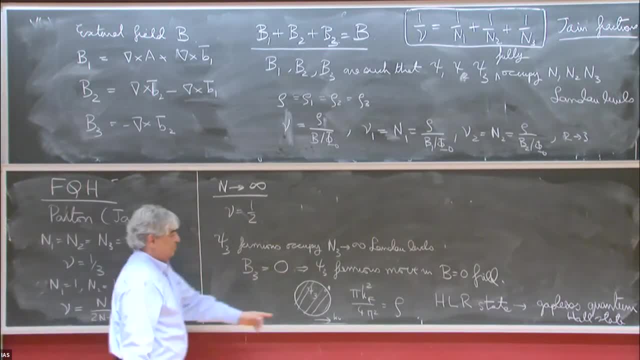 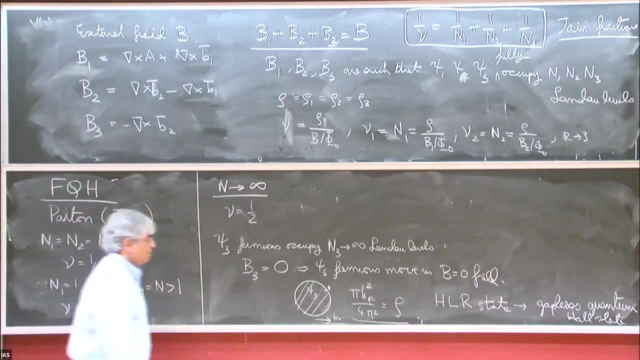 there are very good indication, in fact, of this particular Fermi wave vector that measured in various experiments, In fact here at Princeton by Mansour Shagan, it's observed to be okay, rather accurately, an observation on this state. Sorry, the Fermi, how do you see the Fermi vector? 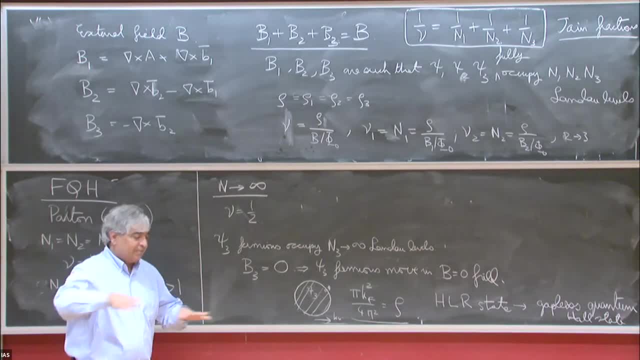 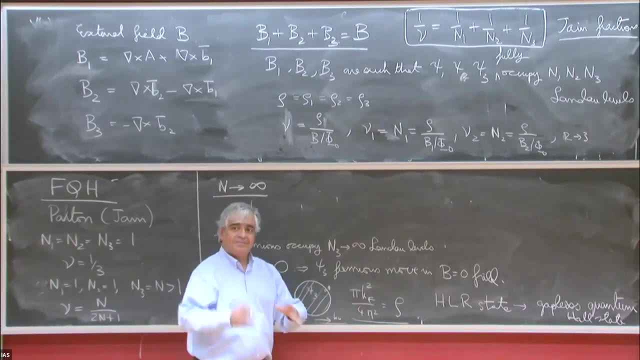 So you have to put an external perturbation which oscillates in space And if it has a wavelength which matches this gap, you observe some sort of resonance. So you do a surface acoustic wave which has a certain wavelength and the wavelength of the wave matches this wave vector. 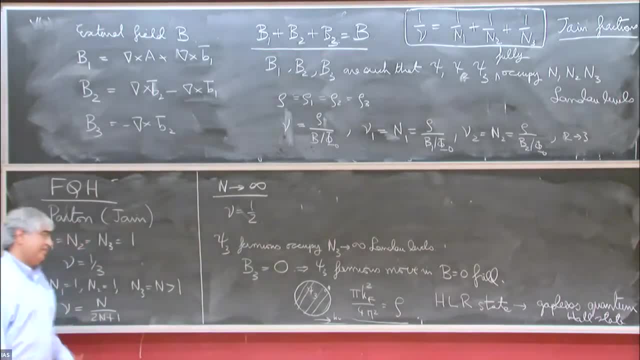 you see, and that's good, You can see the response and so on. Yeah, they're very clever experiments and you can. the point is that these KFs are relatively small because the density in this 2D electron gases is quite small. 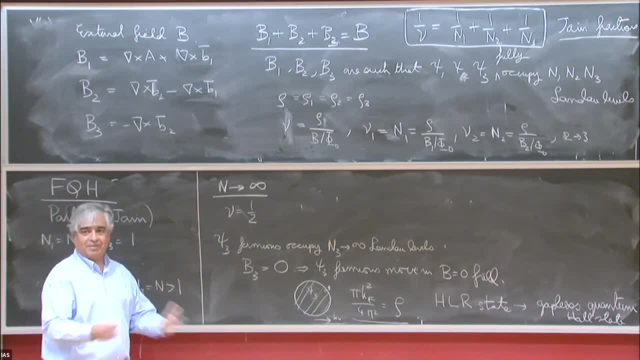 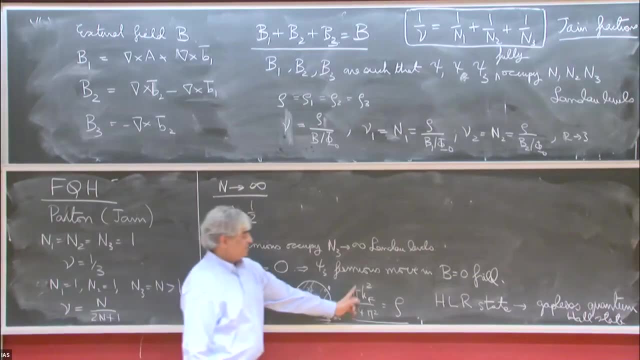 For a KF and an electron gas. in the real material. that kind of experiment would be impossible because the KF is way too large, The wavelengths are very short, But these densities, these wave vectors are, you know, thousands of atomic spaces, so it's easy to measure them. 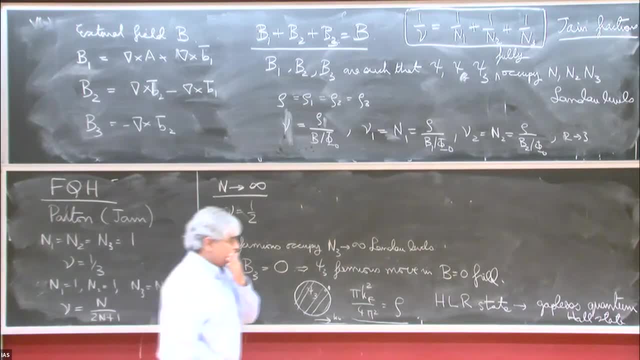 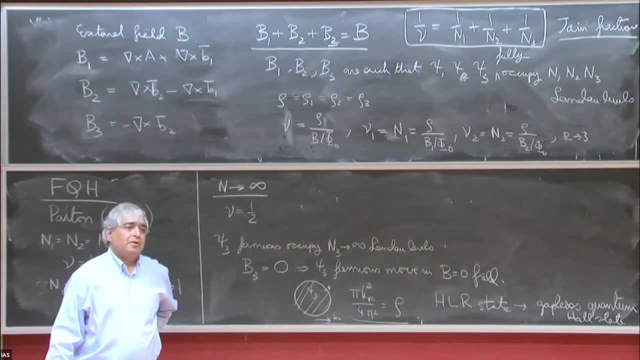 Because of the way these two Degs are created. Maybe 100, sorry, That's driven by the applied physical dynamics, right, Yes, but also the way you create these two Degs is by doping- doping gallium arsenide, and the dopant density is rather low. It's a very small set of dopants, so the density of the electron gas is small. And then you need that also to fill an integer number of Landau levels, because if you took the electronic densities that you would get in the crystal-like cuprates. I think you would need hundreds of Tesla- No one can achieve those- to get anywhere close to the quantum origin. So all of those go together to make this experiment possible. the low density and relatively small magnetic fields that you need to impose to see highly quantum effects. 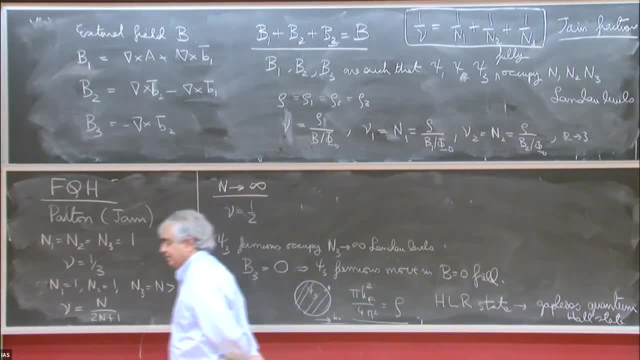 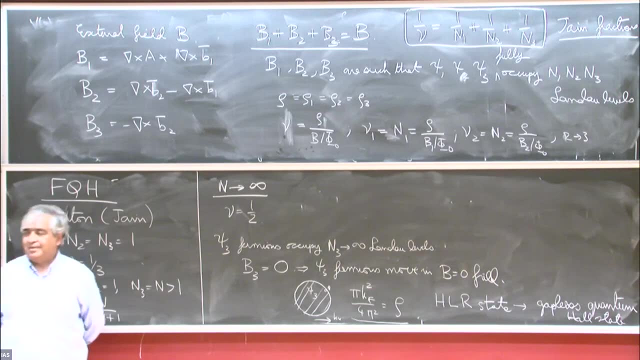 Did I understand-? Yes, said that the Fermi liquid picture of this stage is not exactly correct because the interactions are important, Absolutely yeah, So that's right. So that's a good question. So what do I mean by a Fermi surface? 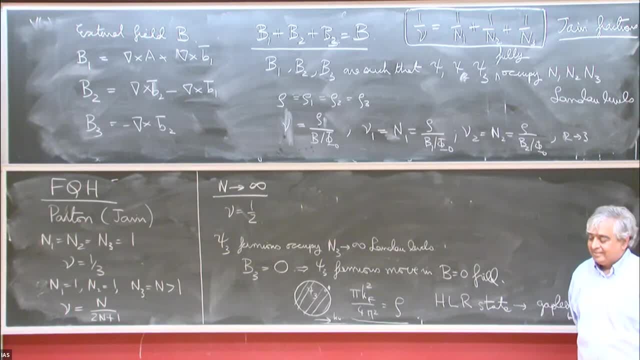 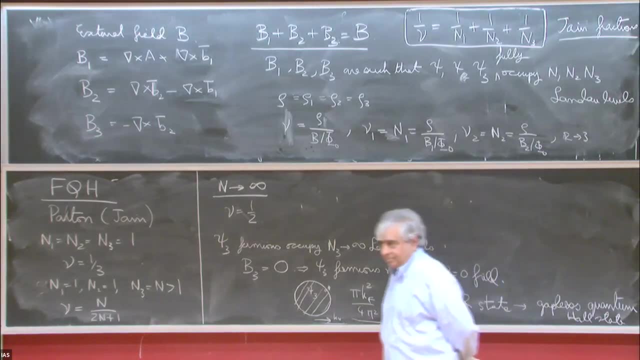 Well, we introduced a Fermi surface for a free electron gas as a jump in the momentum distribution function. Then we found it's also specified for an interacting gas. It's just the size of the jump becomes smaller. In this case there is no jump in the electron momentum. 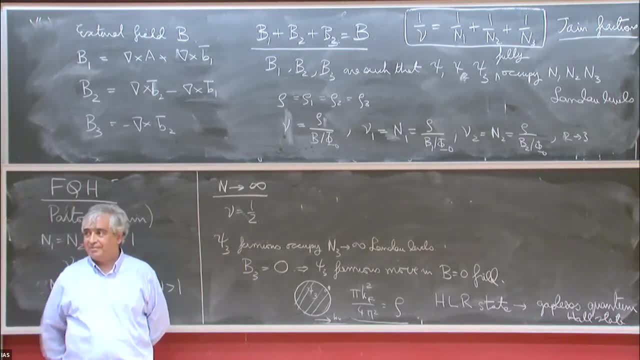 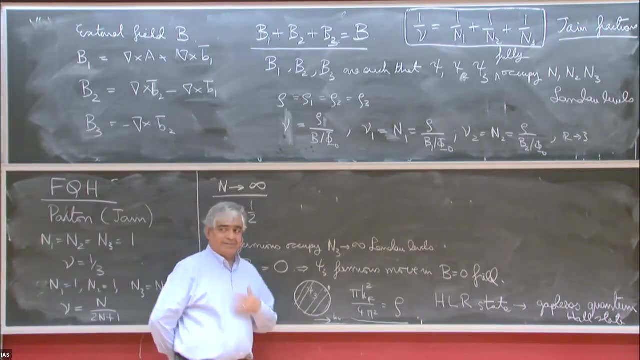 distribution function. But there is a kink, There's a non-analyticity. So what happens is that, roughly speaking, the gauge fields leads to a breakdown of the quasi-particle idea in energy space, sort of very much like the SYK model. 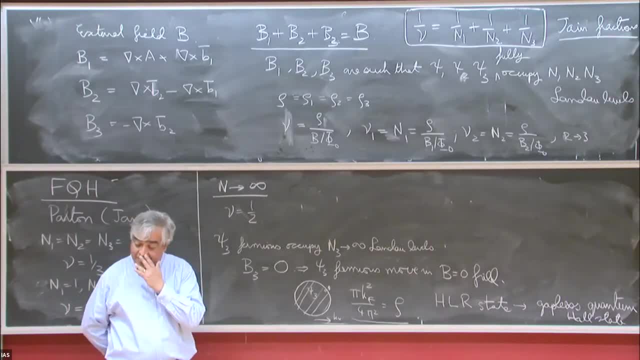 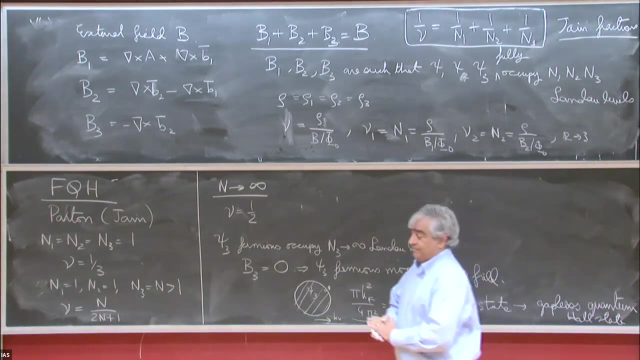 You get no quasi-particle excitations, But nevertheless there's a sharp and momentum space. The idea of a Fermi surface is still well-defined, Because what happens is you have these excitations that are not well-defined, but they do have a definite charge. 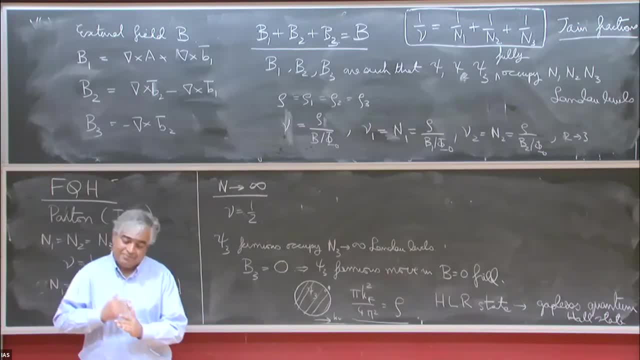 They're either quasi-particles or quasi-holes, And the locus of points in momentum space where your excitation change from quasi-hole-like to quasi-particle-like is the Fermi surface. Even though there are no particles, the Fermi surface is sharp. 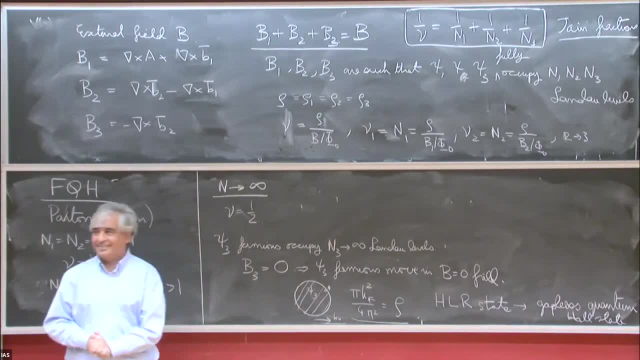 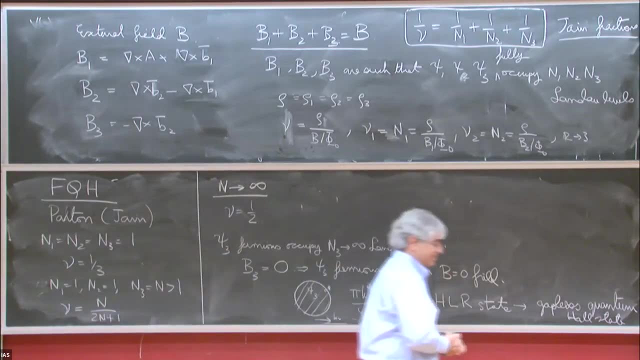 Yeah, This is going to be a topic that I will say much more about. Oh, you're very good. Yes, That's why I want to move on to other things. to eventually get to this: Yeah, I once heard that this state is supposed. 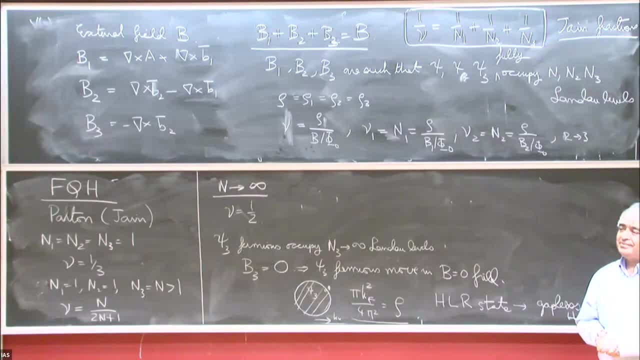 to be described by a prefab-free, massless fermion. Is that the No? Well, I mean you can make an approximation and just treat it as free, but no, Ultimately the quasi-particles are, I mean, OK. 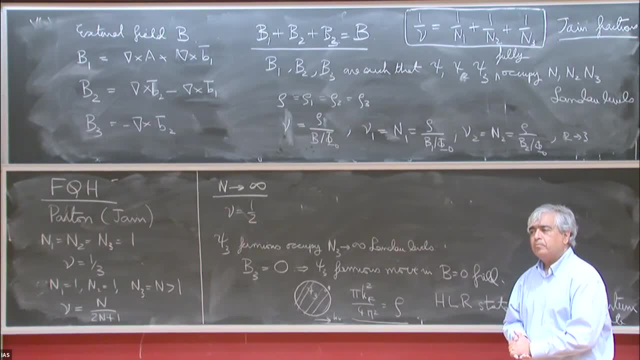 Right, It's a statement that there was some CFT and then the CFT was that of a free fermion. Maybe I'm just remembering? No, I don't think so. This is definitely. The closest thing to this is an SYK model, actually. 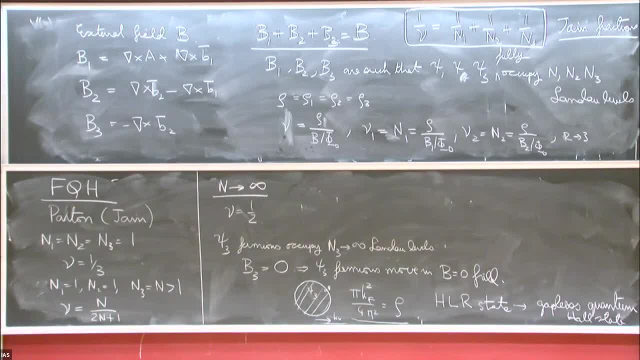 It's strongly interacting, as strongly interacting as the SYK model, But it nevertheless has some sharp structure in momentum space which you can investigate experimentally. OK, Well, I guess I will have to talk more about it, But what I wanted to talk about next, which is also a lot of fun, 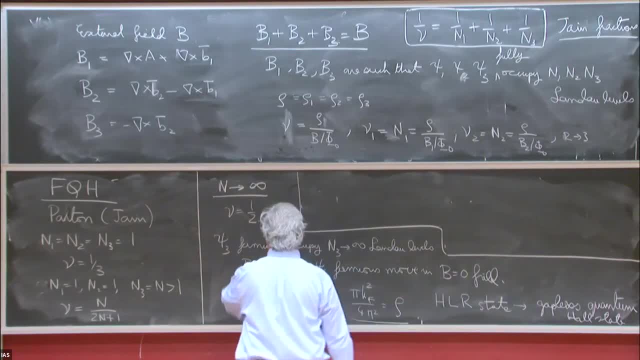 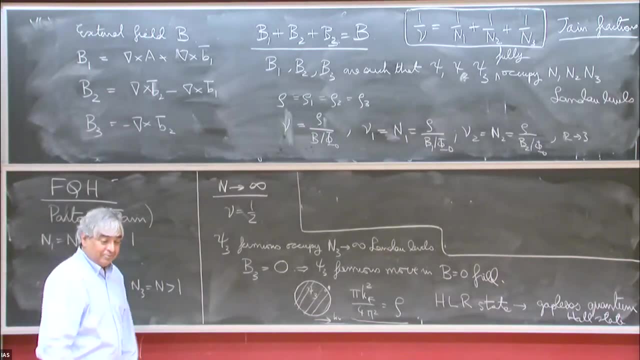 but it's something we can do next time. So another possibility for fermions. We go back to the beginning of the course. We said: fermions form a Fermi surface, Great, But what else do they do? Well, they form superfluids, superconductors. 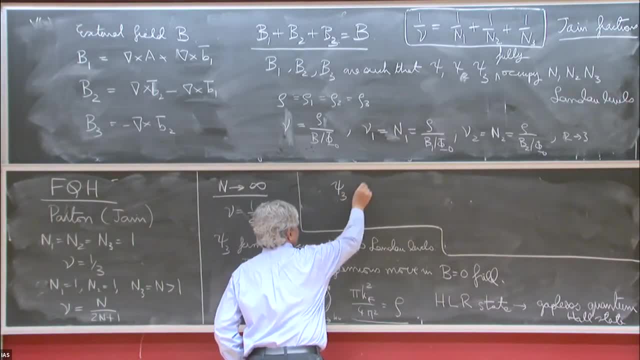 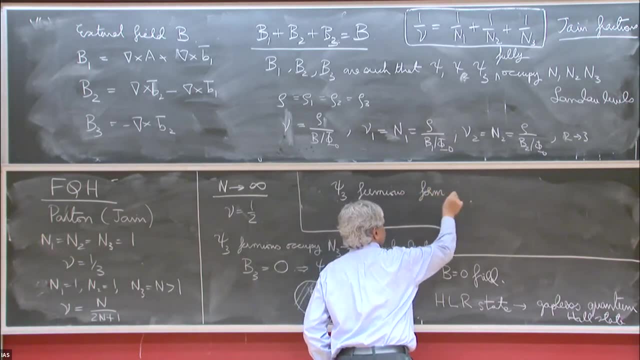 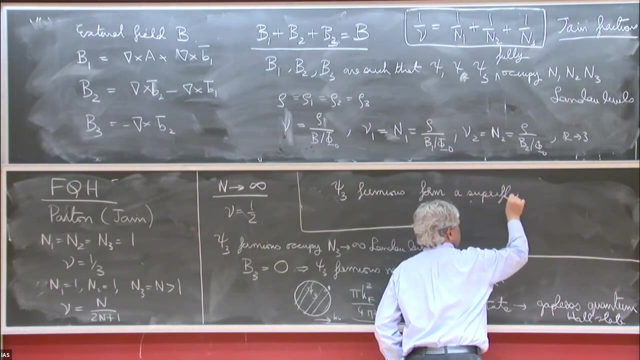 So what can happen in this case is that SIK-3 fermions form. let me call it a superfluid, because from a superfluid which means that psi 3 of p, then the condensate of psi 3 of minus p. 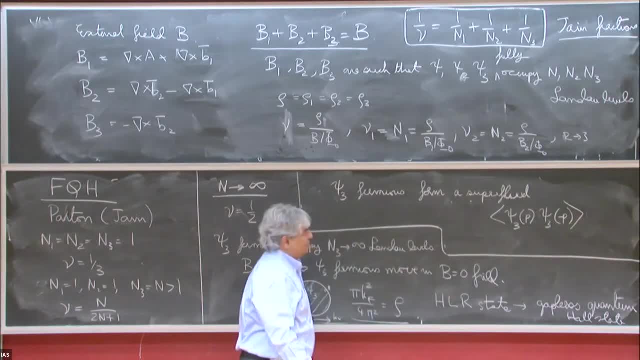 which is not equal to 0. Now, since there's no spin, this has to be an odd function of p. So it's not a d-wave superconductor, which is even function of momentum, It has to be a p-wave superconductor. 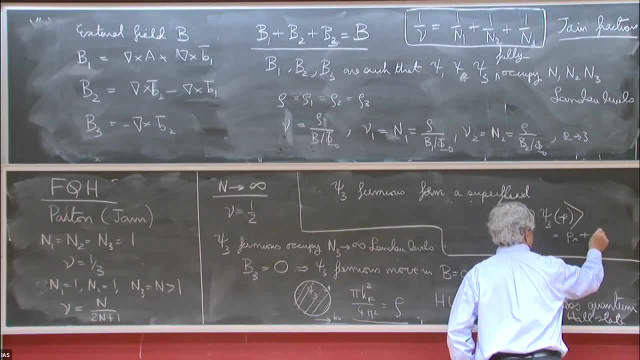 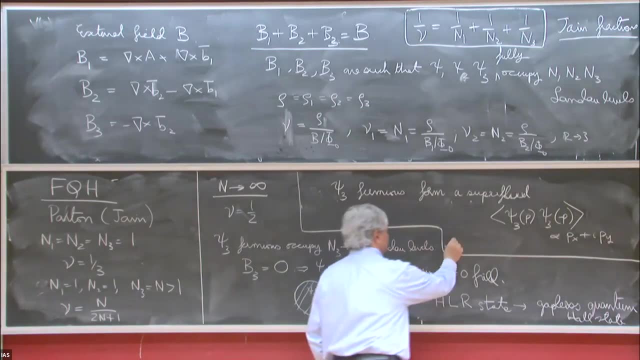 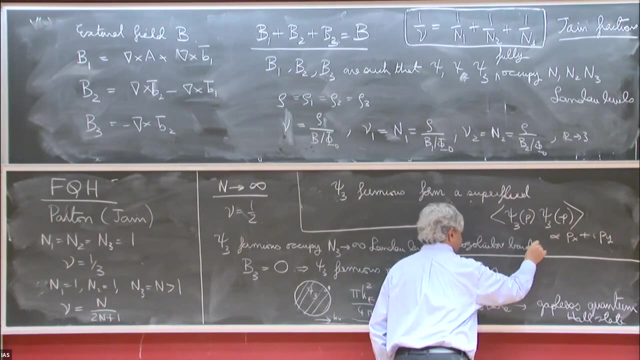 And, in particular, if you take what's called a px plus i, pi, p-y superconductor, which is of this form, then the Pocahontas bonds of this superconductor, which, again, you determine them exactly like we've done in previous chapters. 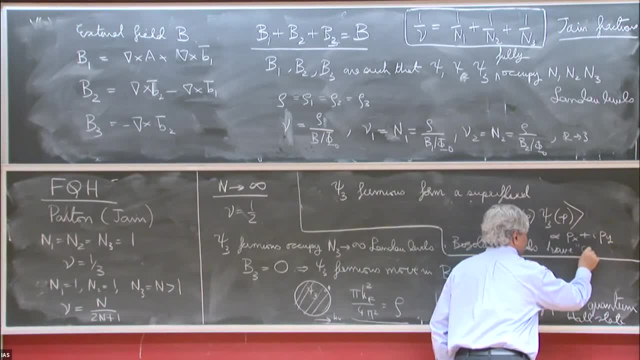 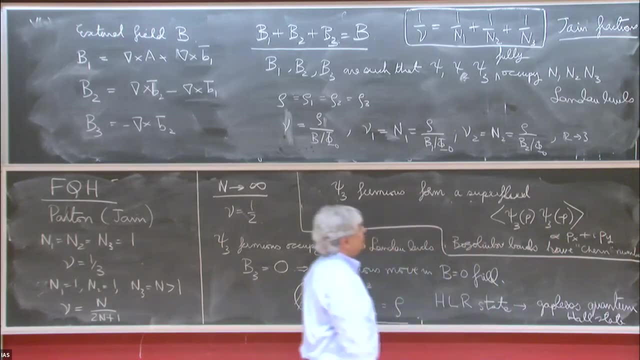 they turn out to have a Chern number. I'll put Chern in quotes, But it's really like half a Chern number. I'll talk about this next time. So now you get a different type of topological state where you have pairing of these fermions. 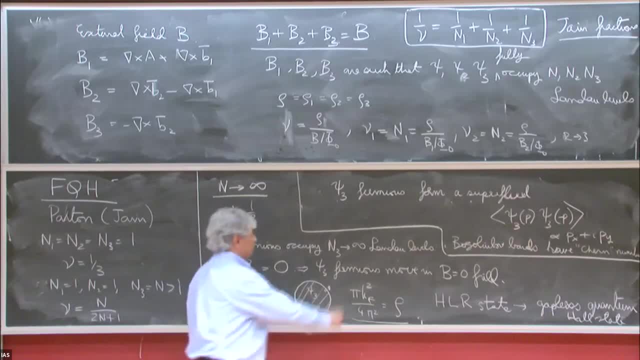 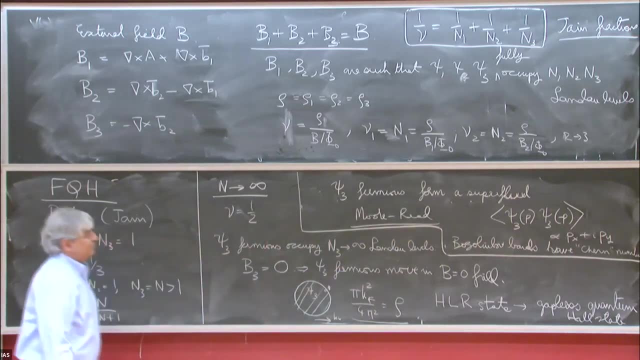 and the bands have a Chern number And that's what leads to non-abelian state, in this case the Mori state. OK, and you can get again. you put this in and you just go through all the tricks you have learned. 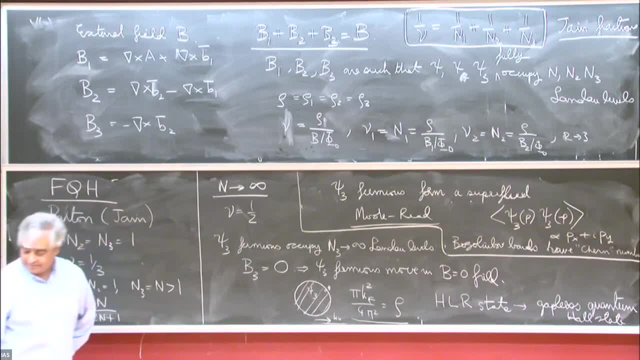 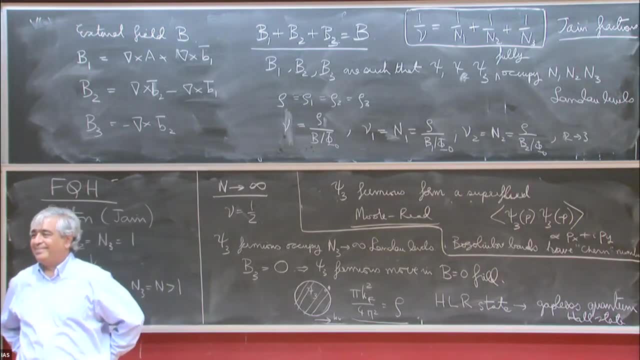 You've got the Pocahontas bonds, You will get all the right properties in the Mori state. I'll say a bit more about that next time. What determines whether it's superconducting or not? OK, it's definitely not a superconductor. 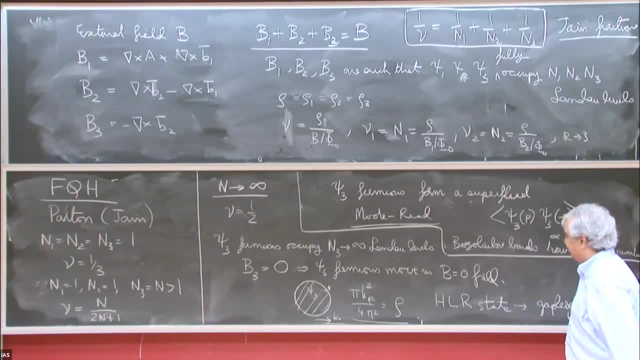 in the sense that you won't see a persistent parent. Yeah, yeah, These things count as a parent, right? Yes, You know, again, that depends on detail. So there's some interaction between the fermions. It depends on which Landau level you're in. 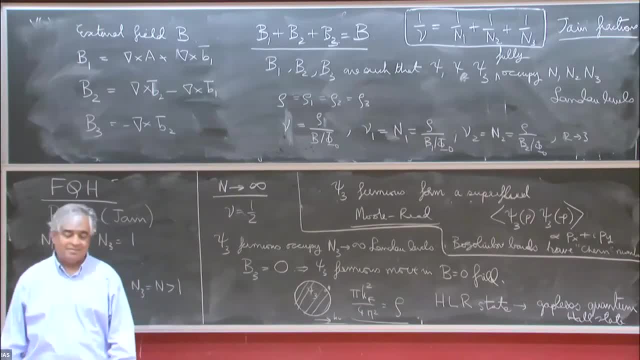 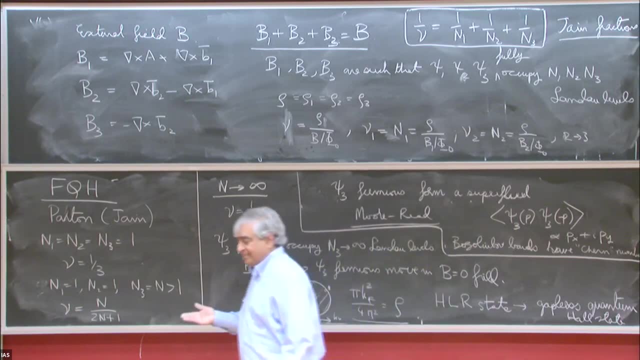 Depends on everything. OK, Is there an attractor? Is there an attractive interaction? Is there an attractor? Well, so there is something called the BCS instability that we learned about, which applies for S-wave pairing. when you have time, reversal symmetry, where 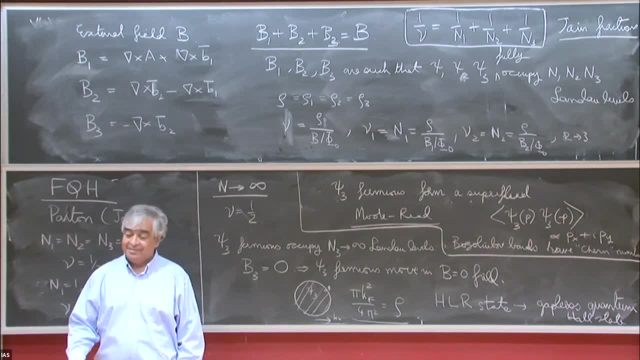 no matter how weak the attraction, as long as there's one, there's an instability to a superconductor state. There's no such theorem here, but when you have broken time, reversal, So you need some appropriate interaction. So OK, and in fact it seems to happen in certain situations. 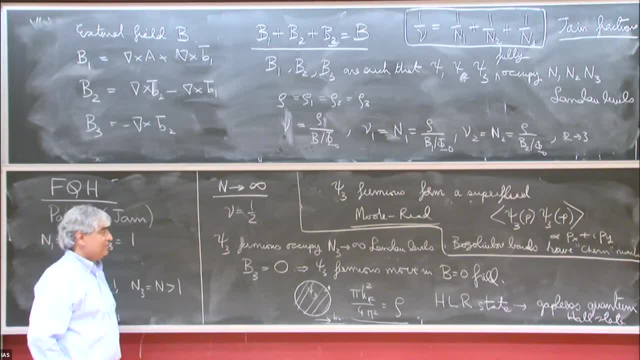 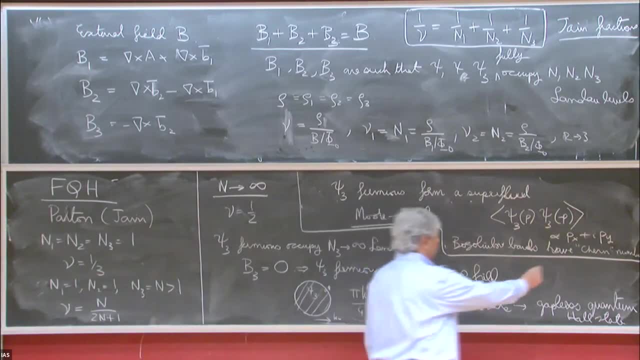 not just in Gallimard site, but also in graphene in recent years. We do see. so this is now a regular fractal quantum Hall state in the sense that it's gapped. So this is a gapped FQH. 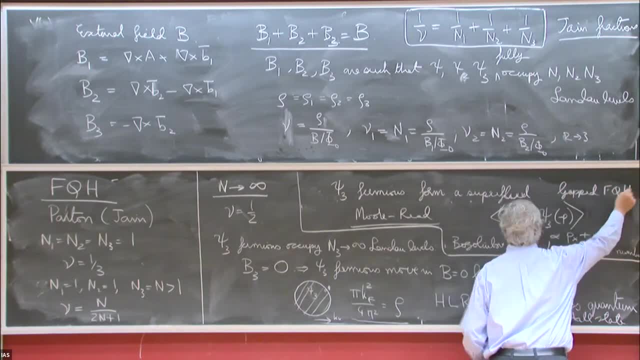 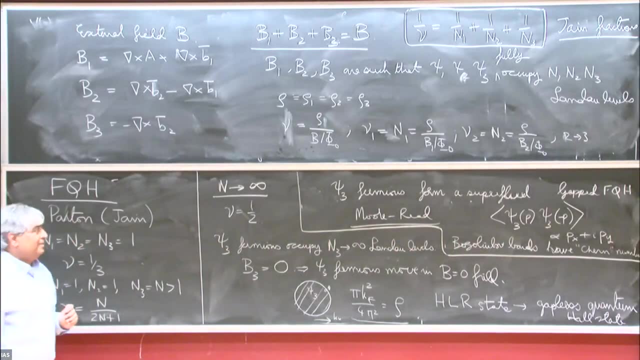 It's fully gapped. There will be edge states and the edge states, because of this boggle of churn number, have Majorana fermions. They're not complex, They're not complex, But when they're real, because of this pairing, essentially, 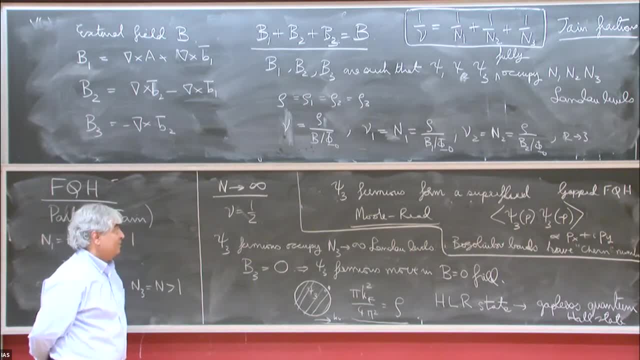 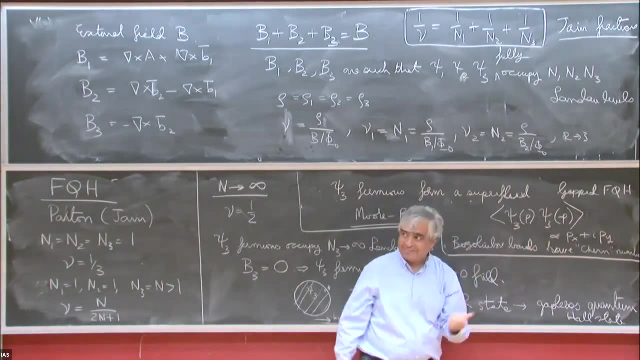 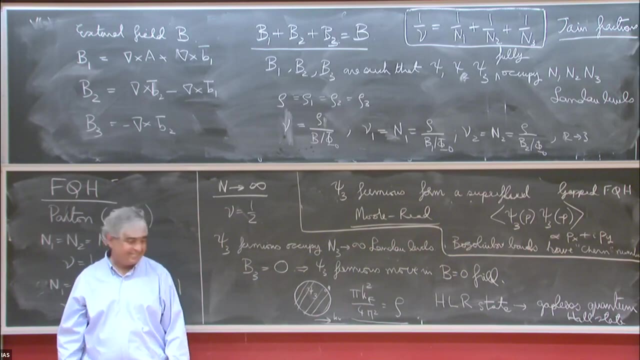 And the Majorana fermions is what leads ultimately to more to, not into. the non-abelian statistics appear from the fact that once you have a superfluid, you also have a vortex. So the vortex in the superfluid is a non-abelian quasi particle. 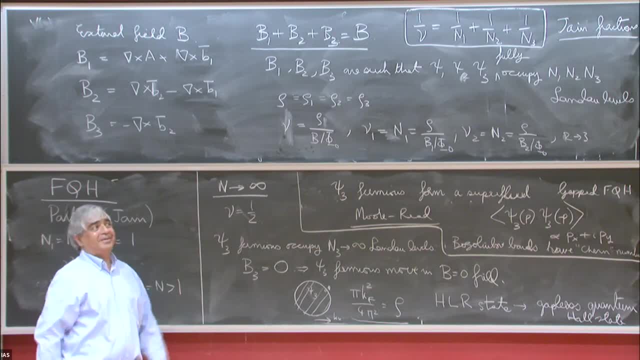 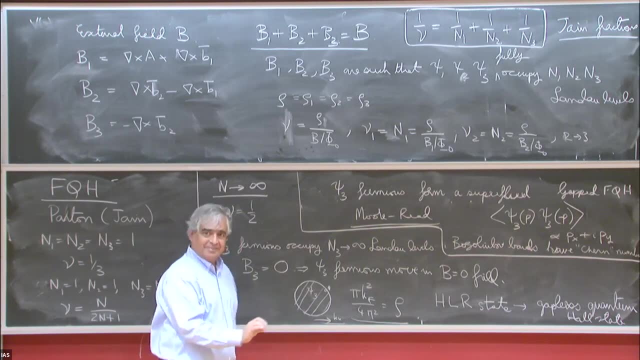 How's the state being observed experimentally? Yeah, well, OK, There is a fractional quantum Hall state observed at nu equals 1, half The more. reach state is the simplest possibility, but there are three or four others, And I'm not an expert on this. 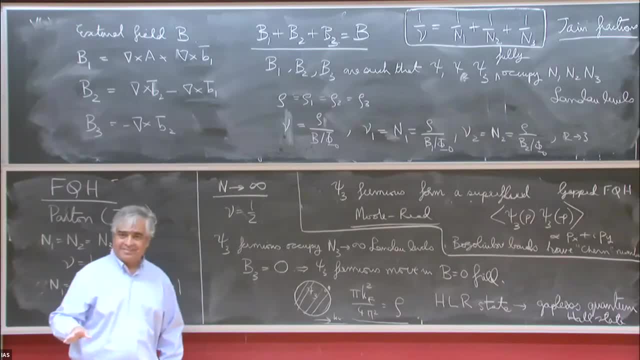 This is a topic of very hard current research. I don't think it's particularly been decided which is the right one. It may be more read, It could be something else I see. So some materials will give you the new 1 half. 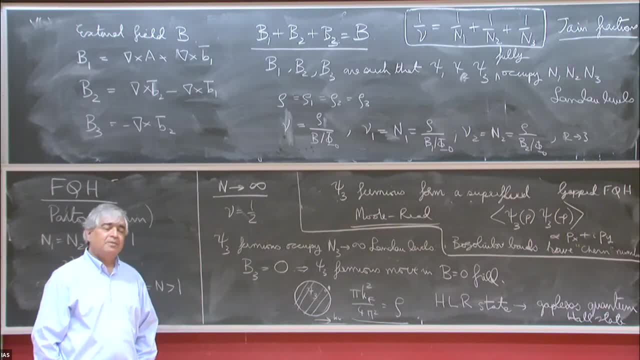 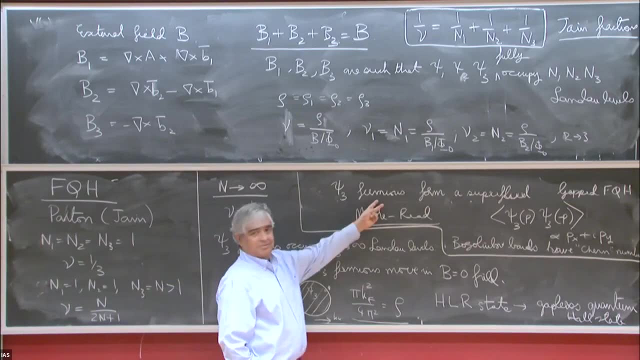 that you said before we mastered. Yeah, Other materials will give you the new one. Yeah, I mean, it could also be that if you went to very low temperatures, every material will go to this. For some temperature range you can ignore the pairing. 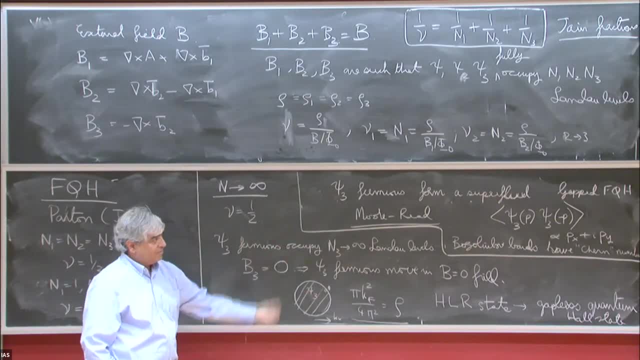 and you can see the HLR state, But at low enough temperatures it could well be. everything will be compared and somewhat tangled. But yeah, there are a bunch of other states, more complicated states, which have also had Majorana edge states. 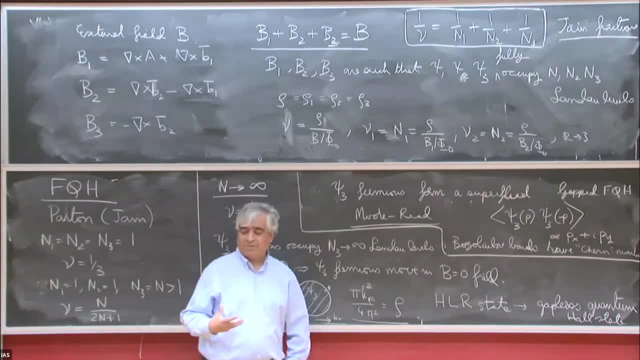 And there's evidence for a piece of Majorana edge, Because that gives you a half quantized thermal conductance, which has been seen. Yeah, It's been seen. But there are also other edge states coming from the side 1 and side 2 fermions. 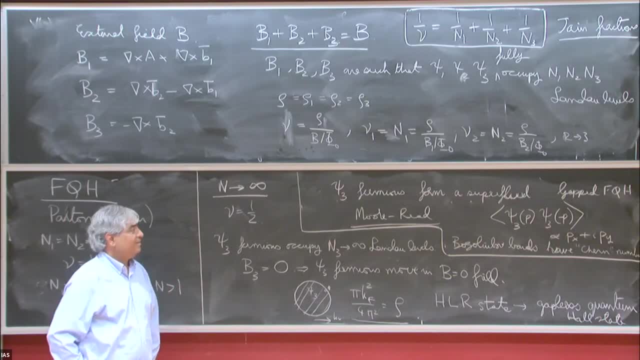 So in this case it's more complicated. You've got a lot of stuff going on And there are other states- I am not an expert by that any means, But I think the current status is not yet clear which one of them has been seen. 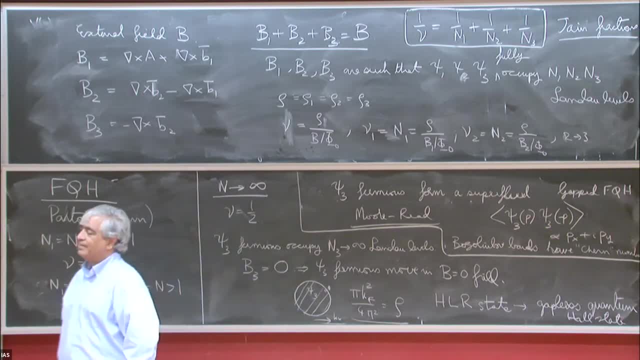 I know that a short while ago I saw a paper that talked about the half integer thermal conductivity. Yeah, And I asked Greg whether this was proof that they found more reach state And he said no, Yeah, OK, So he's being honest. 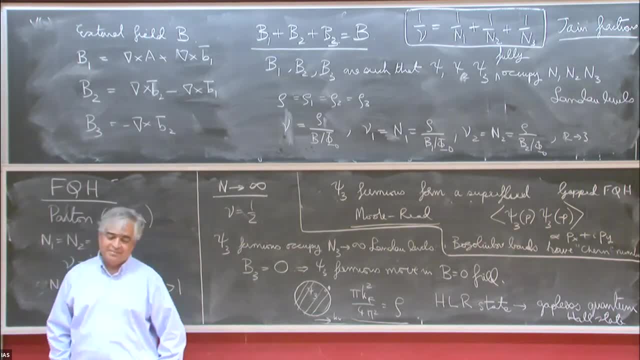 That's correct. Yeah, That's my understanding too. Yeah, There's also analogs of the pairing in spin liquids, where you take a Z to spin liquid and you pair this epsilon particles in this P plus IP state And that's the of non-abelian state, which is similar. 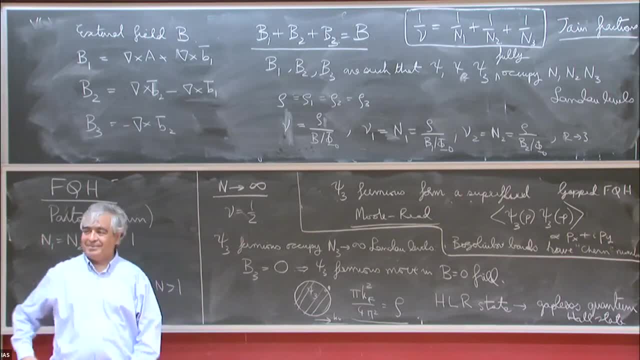 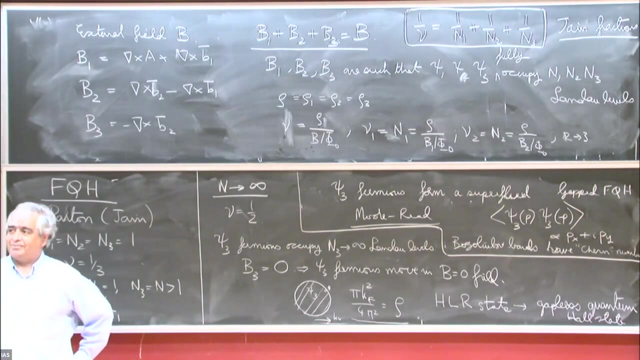 But its edge states are slightly different. Yeah, But everything can be very compacted, At least these ones. The more complicated ones- maybe I'm not sure how to get them from the part of those People- are very fancy conformal ways. 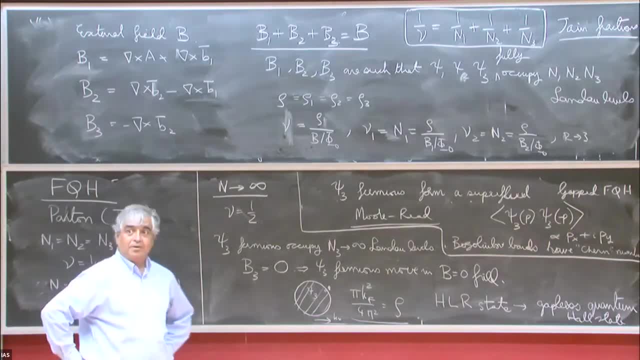 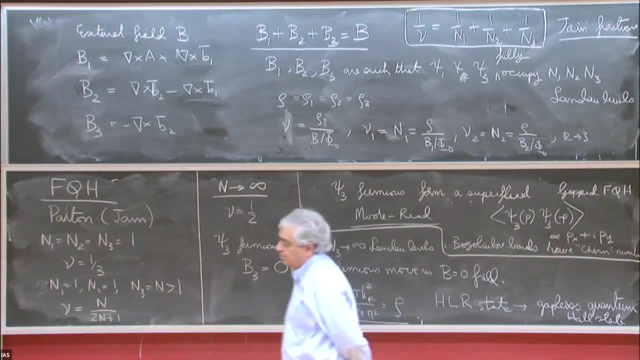 of thinking about it. OK, yes, go ahead. I just wanted to make a comment. slash question. Sure, When you hear you said that the size fill of Ni Landau levels, Yes, I was confused for a bit, But in the spirit of your derivation, 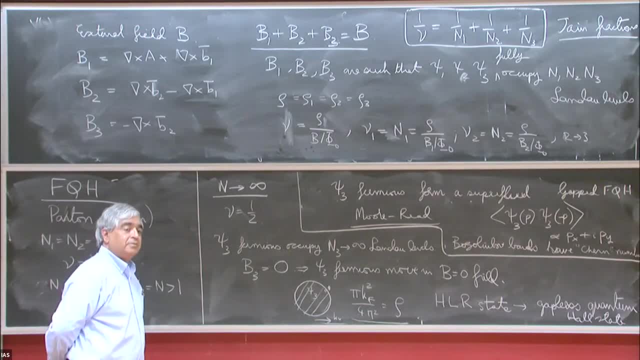 you could say that if you did this mean field theory without the Hamiltonian for the size, which would have turn numbers, Yes, Ni's could be interpreted as the turn numbers of those filled bands. Correct, And that would answer Tom's question about what. 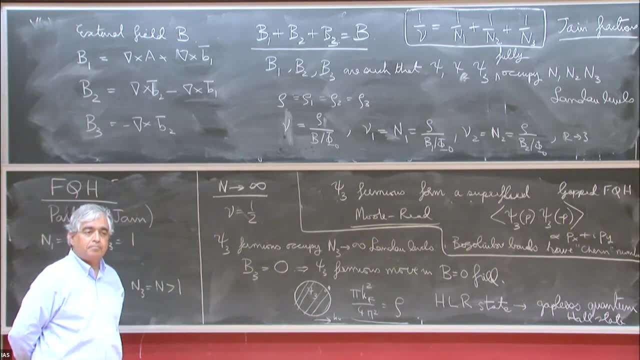 the turn Simons levels are, because we would deduce them in precisely the way you said the other day, from the numbers of filled bands and from the gauge fields that coupled to each species of Yes, Yes, sure, And I think that's correct. 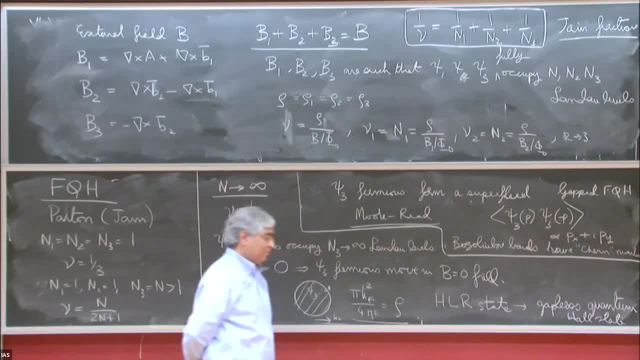 But I guess I was thinking about: well, what if you get to some physical response? The actual positive particle statistics is a bit more complicated, And how would they couple to the external magnetic field and so on? Yes, But yeah, I think you're right. 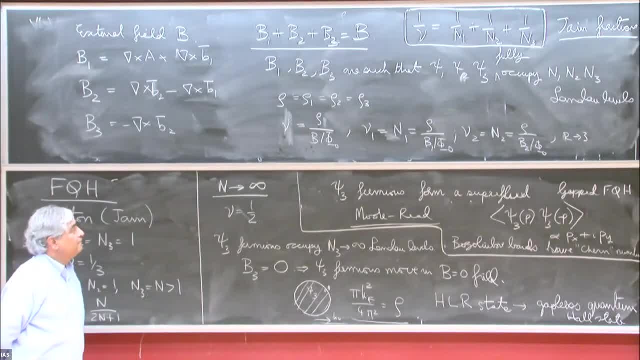 Yes, sure you're right. I guess I'm saying that the turn Simons levels would be like Ni for the Di Yes, correct? Yeah, If you put it on a lattice, I mean, that's effectively what happens on spin systems on a lattice. 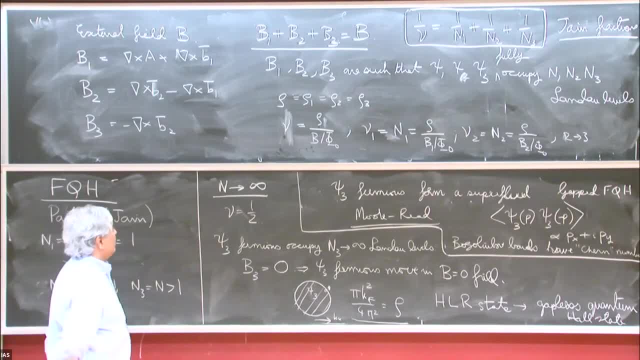 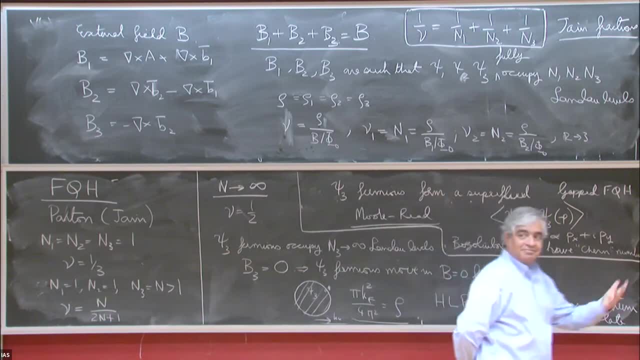 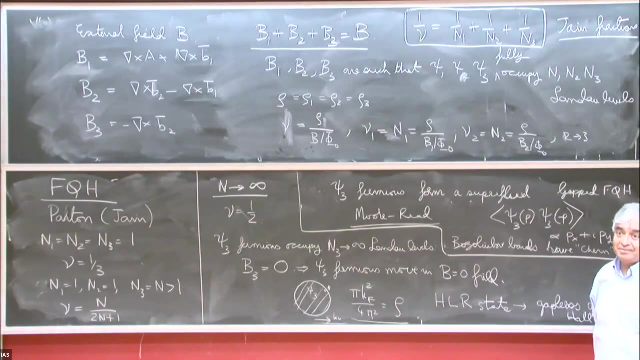 Yeah, So there's OK, there may be a plus 1.. Sorry, Yeah, and the way I wrote it is correct. So N1 is just the turn number. Yeah, So everything can go to turn insulators. We just replace the integers N with turn numbers. 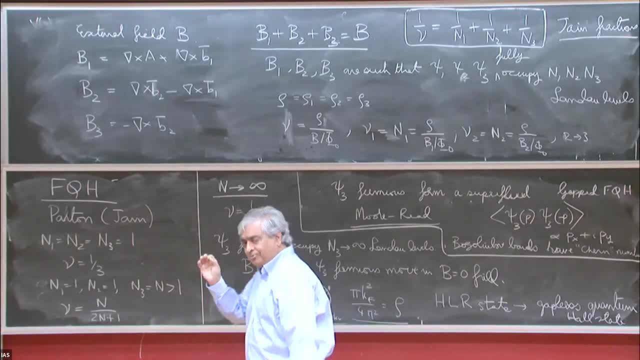 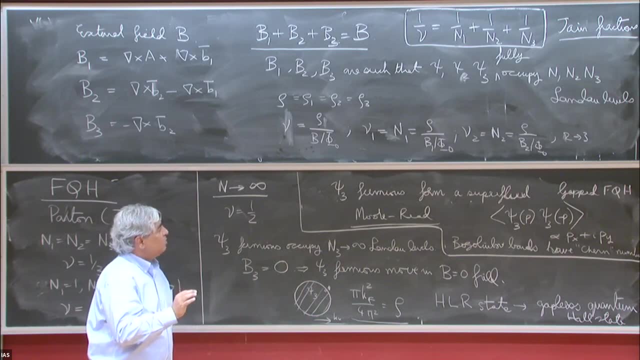 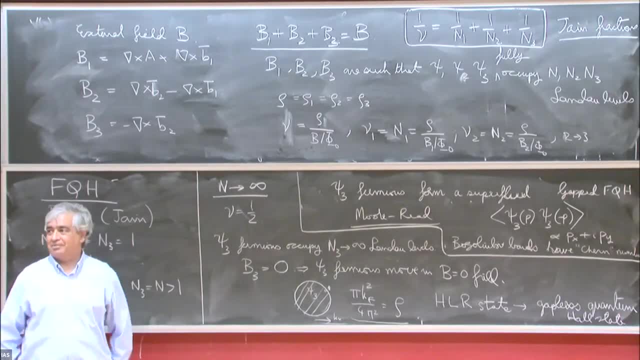 The number of edge states for each of them would be N1,, N2, and N3 also, which you can also see from the Halbrin picture. You get N levels going to the edge. OK, I've gone way over. 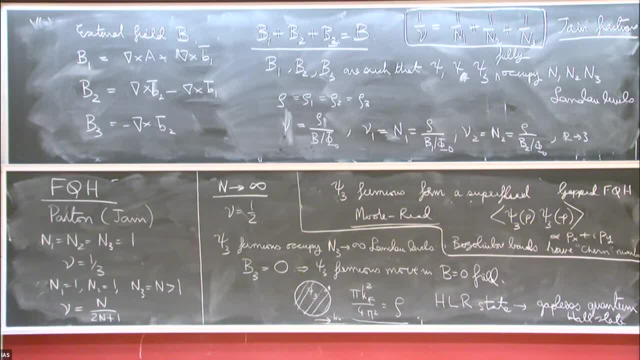 So, all right, just a few more things to say, and then we'll move on to other topics. next time, N being infinity just means that psi 3 happens to have a Banditism. it turns in, So it says Yes. 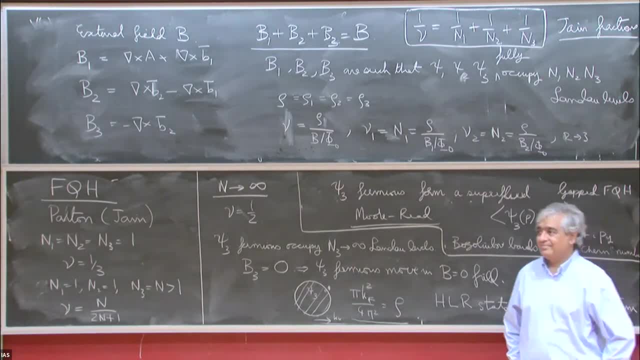 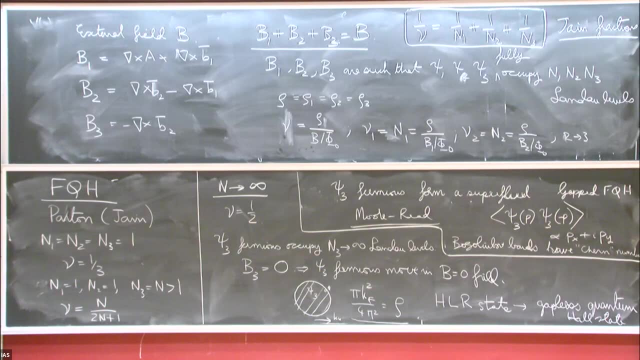 Yes, right, Yeah, Yeah, Yes, Yes, Yes, Excuse me, Yes, Yes, quick. there's an envelope with kiara's name on it in the princeton records office. just, uh, mentioned offhand. uh, yeah, there was an analog to codes of the um. 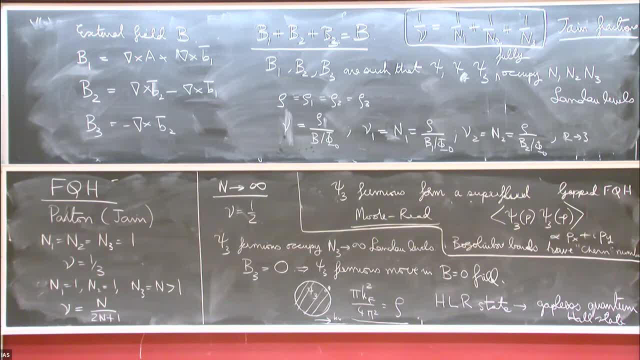 with that. i don't know much about a throwaway. okay, yeah, i mean it looks like that. right, you have to take one and replace by one, one one. yeah, it looks like a code. of course, people looked at codes, quantum codes, in turn, simon system, i don't know. it's like. i think there may be some relation, but you know also all these. 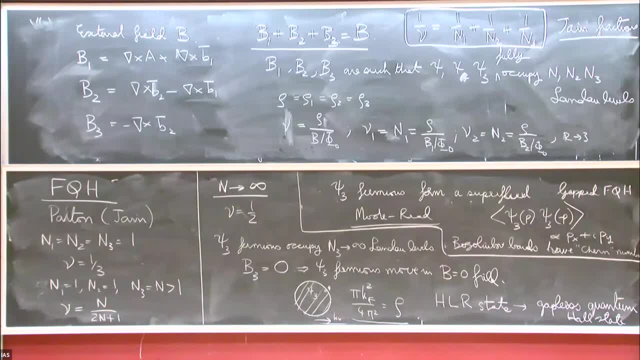 gauge fields. part-time construction is very much related to tensor networks. they're also, you know, with extra degrees of freedom, which are all related to code. so, yeah, there may be a way of unifying it more. okay, i was wondering if there was more to it than that there could be, but i'm not aware. 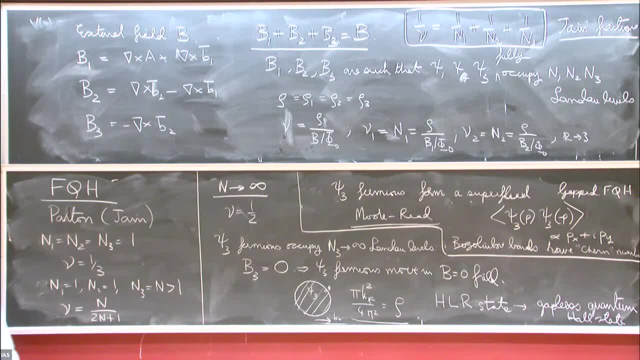 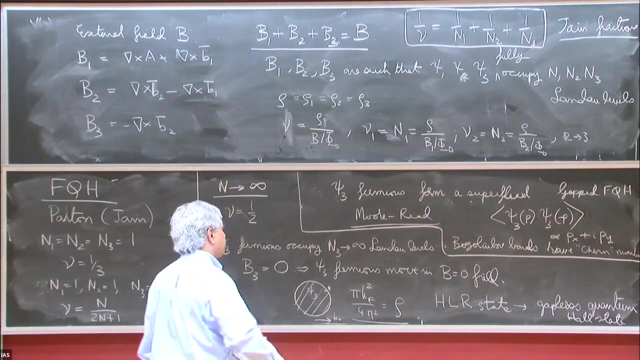 i think there could be. i mean the, the, uh, the gate conditions are really are stabilizer conditions actually. is that right? forcing the, the code subspace? yes, yes, exactly, oh, okay, now i know what a stabilizer. yes, and they commute with everything else, right, okay, yes.